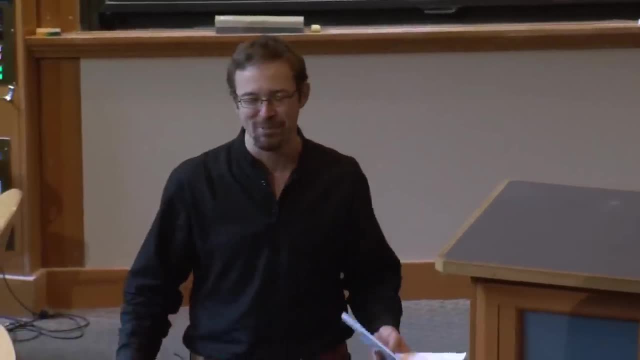 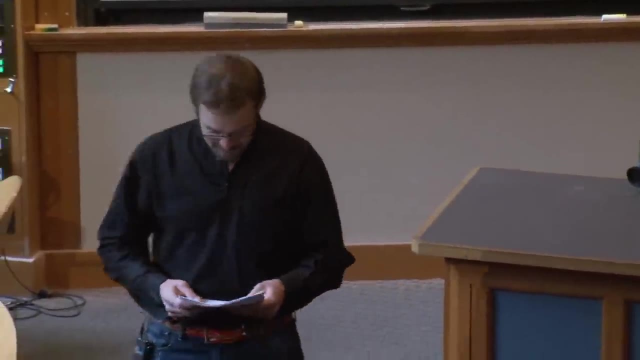 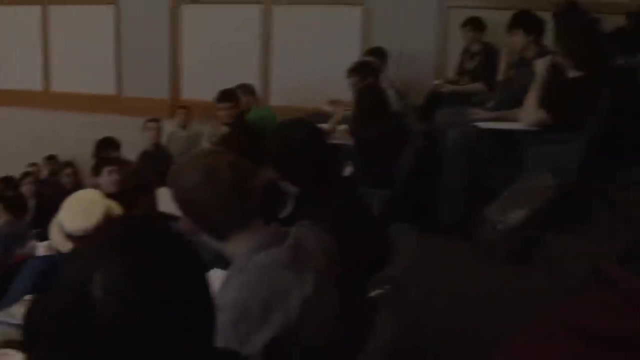 I met quantum mechanics 20 years ago. I just realized that last night. It was kind of depressing. So, old friend, It's also my most powerful tool, So I'm pretty psyched about it. Our recitation instructors are Barton Zwibach, yay. 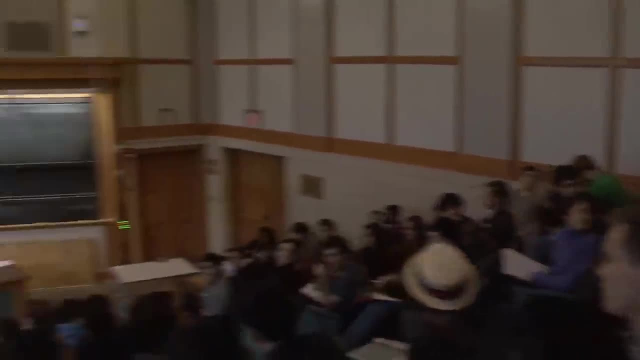 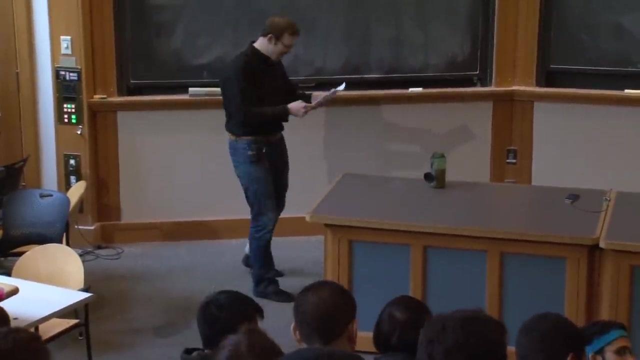 and Matt Evans. yay, OK, Matt's new to the department, so welcome him, Hi. So he just started his faculty position, which is pretty awesome, And our TA is Paolo. Glorioso Paolo, are you here? Hey, there you are. 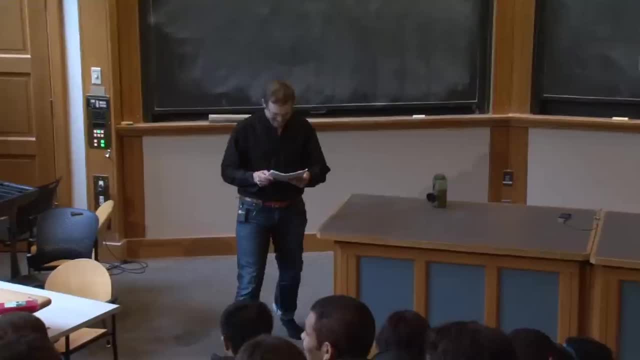 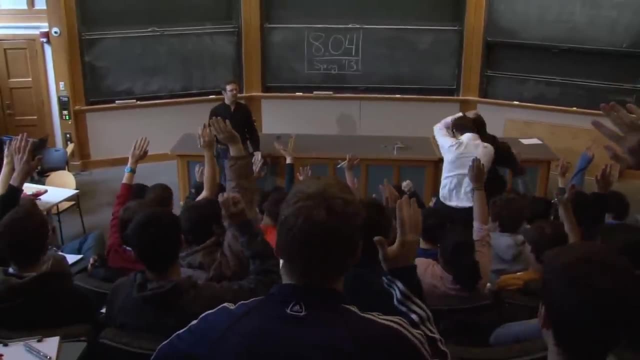 OK, so he's a person to send all complaints to. So, just out of curiosity, how many of y'all are course, eight, Oh awesome. How many of y'all are, I don't know, 18? Solid Six. 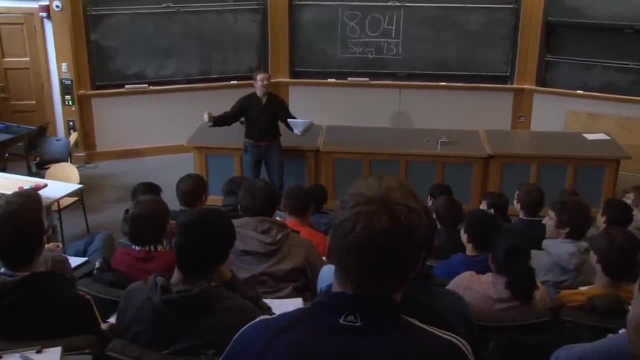 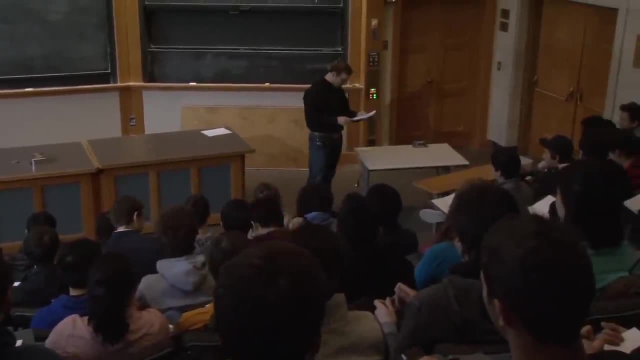 Excellent Nine: No one. This is the first year we haven't had anyone course nine. That's a shame. So last year one of the best students was a course nine student. So two practical things to know. The first thing is everything that we put out. 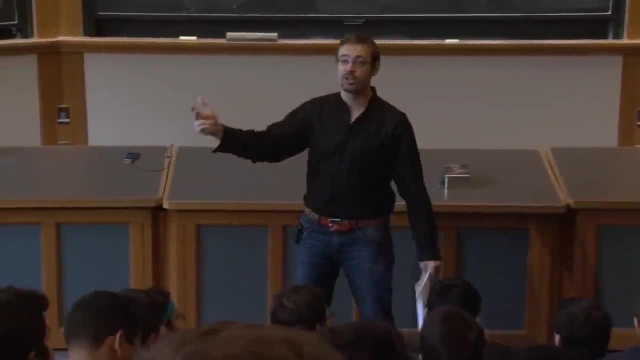 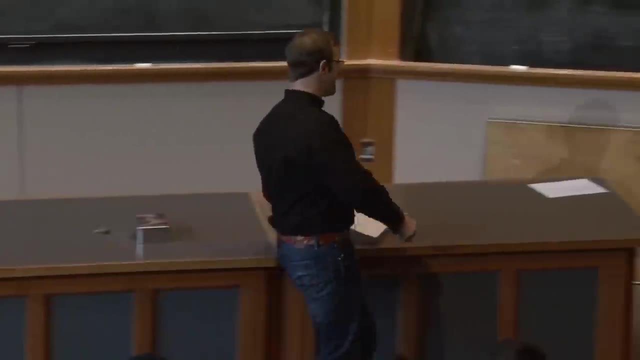 will be on the Stellar website: Lecture notes, homeworks, exams. everything is going to be done through Stellar, including your grades. The second thing is that, as you may notice, there are rather more lights than usual. I'm wearing a mic. 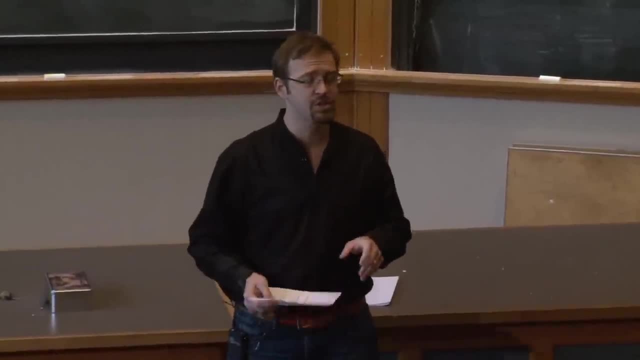 And there are these signs up. We're going to be videotaping this course for the lectures for OCW, And if you don't want to, you know you don't want to do it, but if you're happy with that, cool. 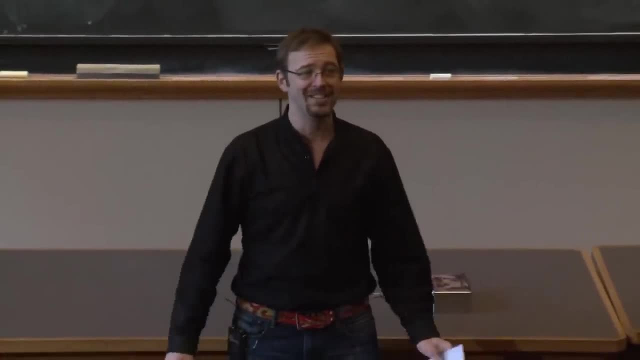 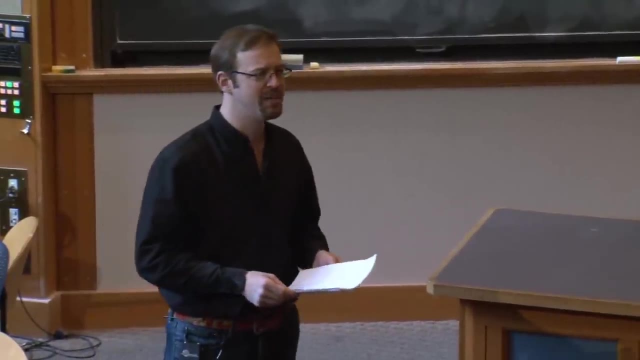 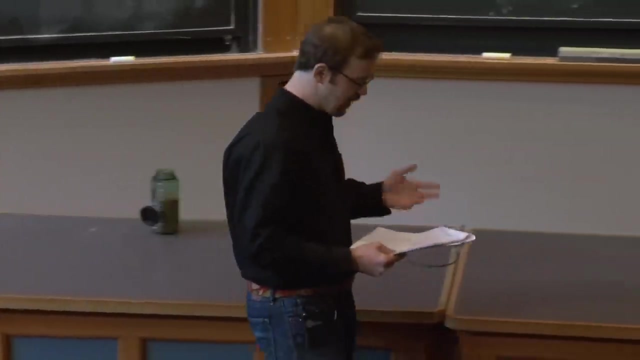 If not, just sit on the sides and you won't appear anywhere on video. Sadly I can't do that, But you're welcome to if you like. But hopefully that should not play a meaningful role in any of the lectures, So I'm going to, OK. 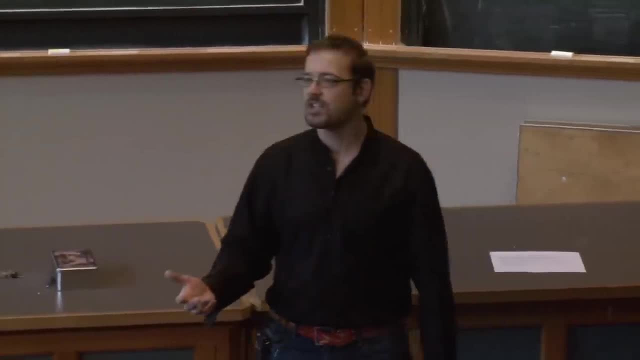 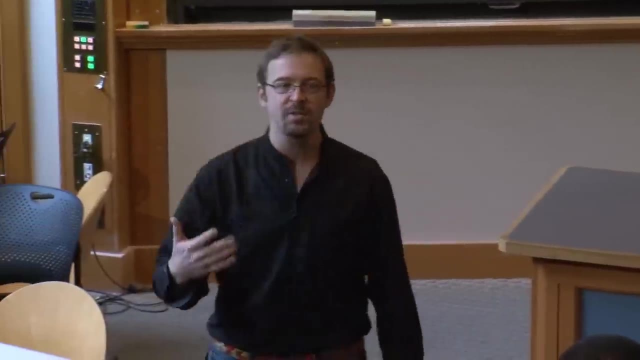 So the goal of 804 is for you to learn quantum mechanics. And by learn quantum mechanics I don't mean learn how to do calculations, although that's an important and critical thing. I mean learn some intuition. I want you to develop some intuition. 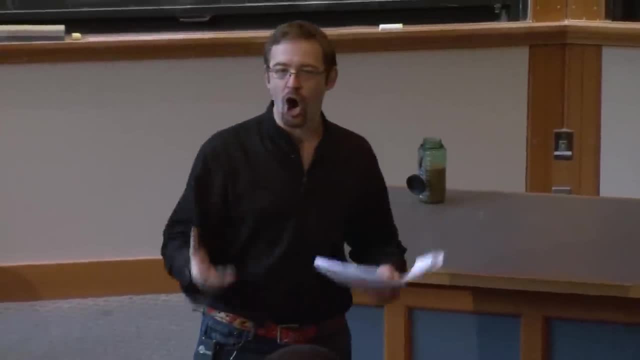 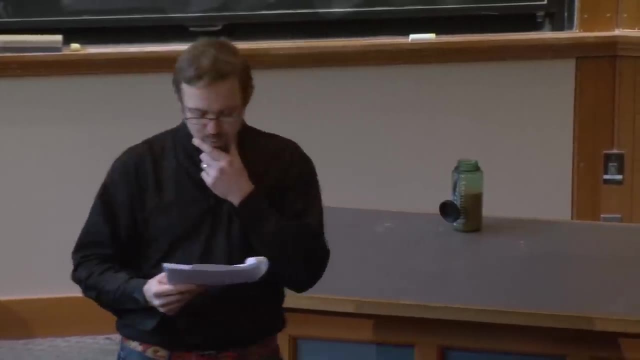 for quantum phenomena. Now, quantum mechanics is not hard. It has a reputation as being a hard topic. It is not a super hard topic. It does, however, require so, in particular, everyone in this room. I'm totally positive. 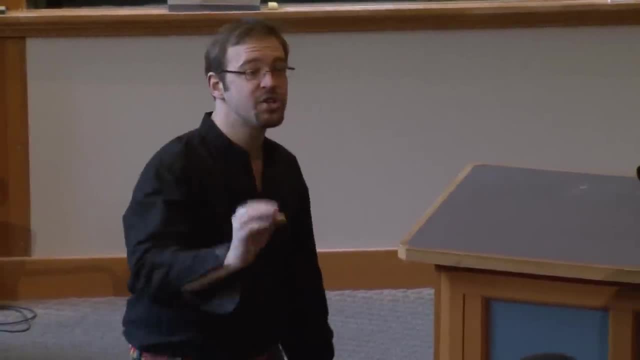 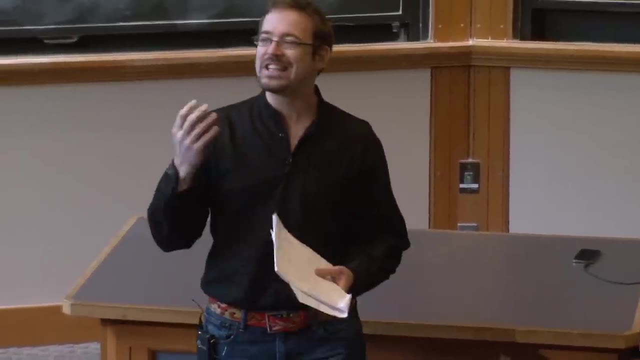 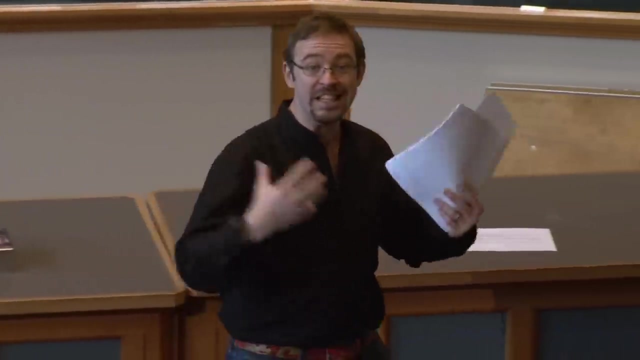 can learn quantum mechanics, It does require concerted effort. It's not a trivial topic And in order to really develop a good intuition, the essential thing is to solve problems. So the way you develop a new intuition is by solving problems and by dealing 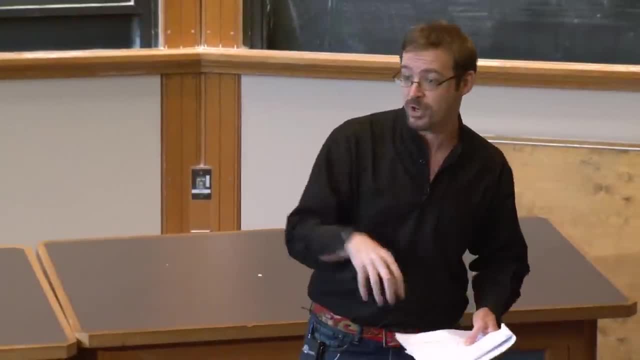 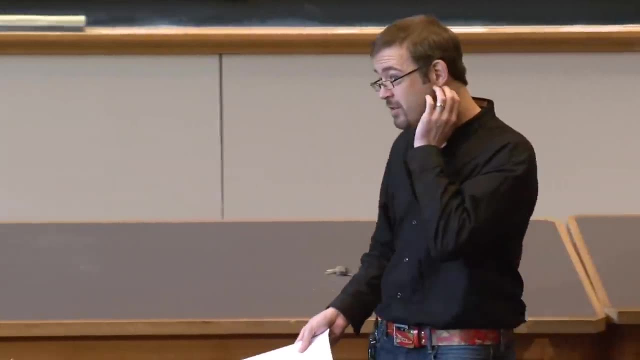 with new situations, new contexts, new regimes, which is what we're going to do in 804.. It's essential that you work hard on the problem sets. So your job is to devote yourself to the problem sets. My job is to convince you at the end of every lecture. 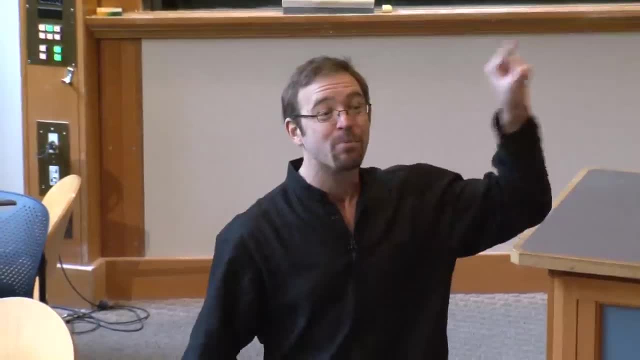 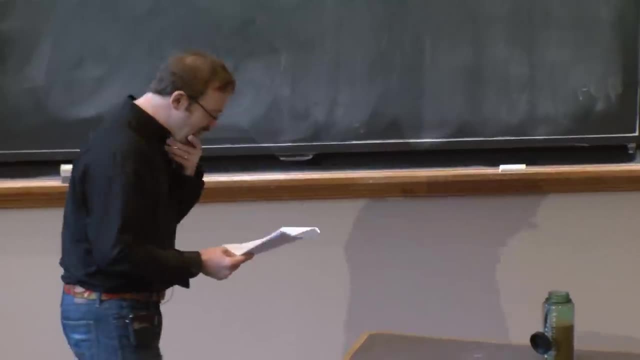 that the most interesting thing you could possibly do when you leave is the problem set. So you decide who has the harder job. OK, So the workload is not so bad. So we have problem sets due. They're due in the physics box, in the usual places. 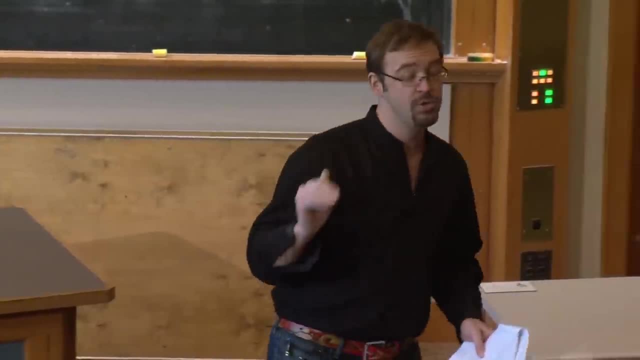 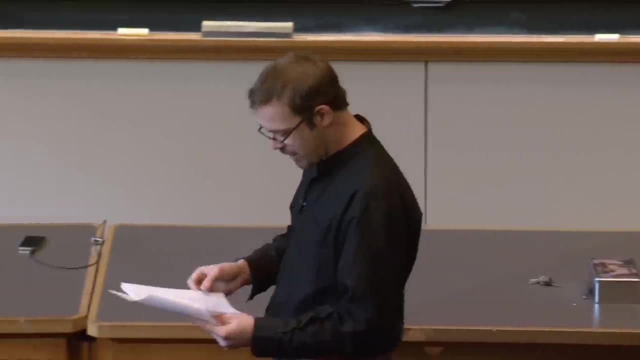 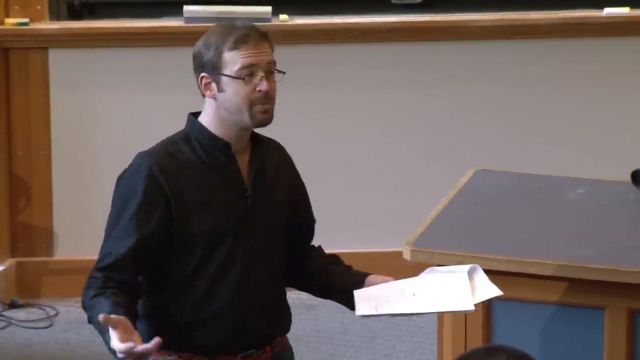 by lecture by 11 AM sharp on Tuesdays every week. Late work? no, not so much, But we will drop one problem set to make up for unanticipated events. We'll return the graded problem sets a week later in recitation. 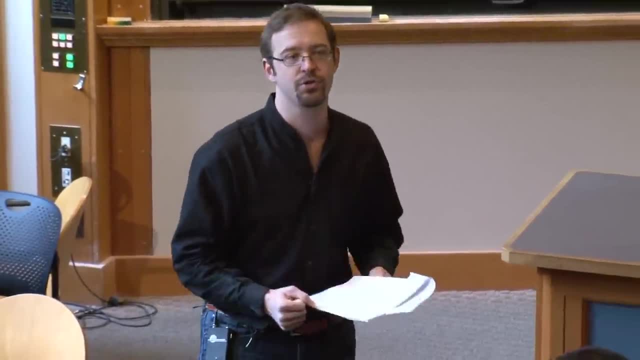 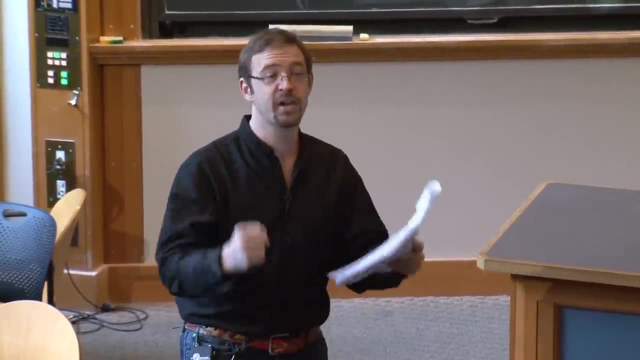 Should be easy. I strongly, strongly encourage you. I strongly encourage you to collaborate with other students on your problem sets. You will learn more. They will learn more. It will be more efficient. Work together, However. write up your problem set yourself. 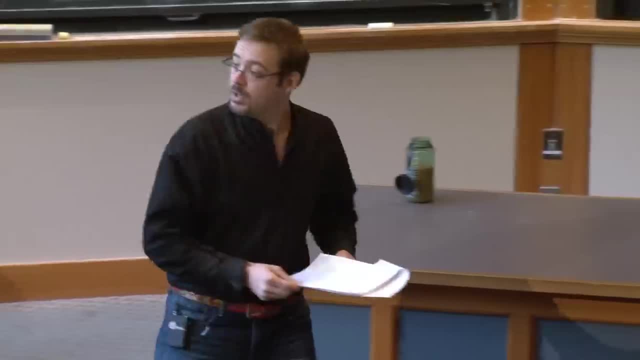 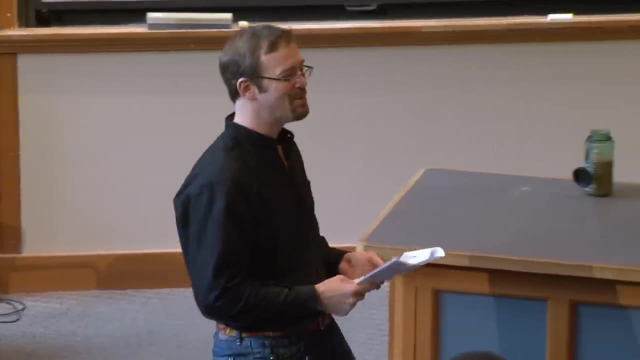 OK, That's the best way for you to develop and test your understanding. There will be two midterms dates to be announced and one final. I guess we could have multiple, but that would be a little exciting. We're going to use clickers, and clickers will be required. 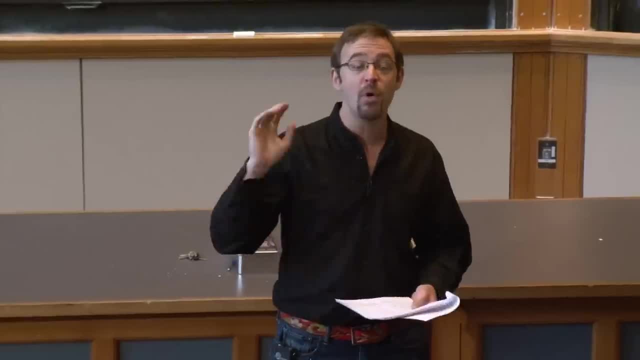 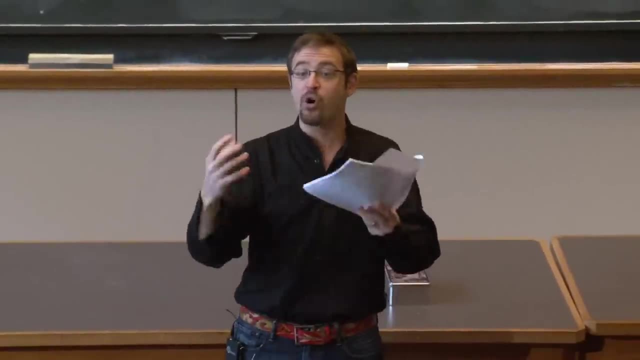 We're not going to take attendance, but we're going to take attendance. We're going to take attendance, We're going to take attendance. The answer is: you're going to get a small contribution to your overall grade And we'll use them most importantly. 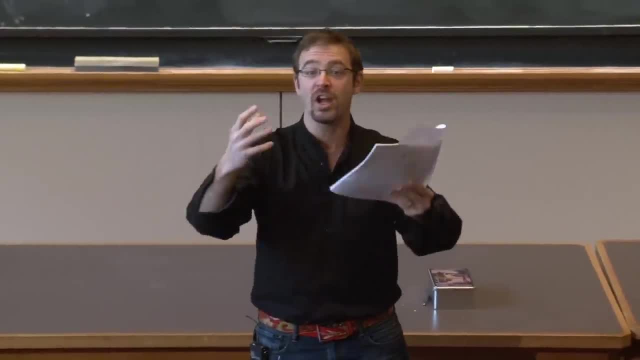 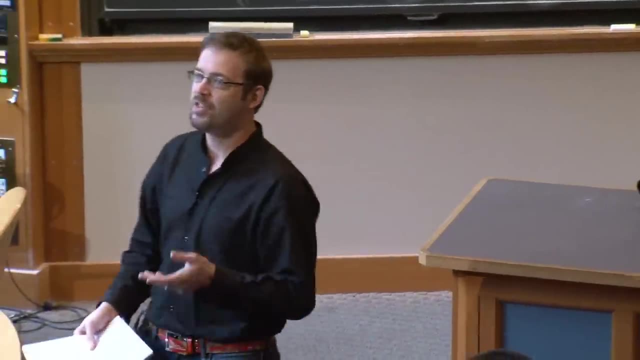 for non-graded but just participation, concept questions and the occasional in-class quiz to probe your knowledge. This is mostly so that you have a real time measure of your own conceptual understanding of the material. This has been enormously valuable And something I want to say just right off. 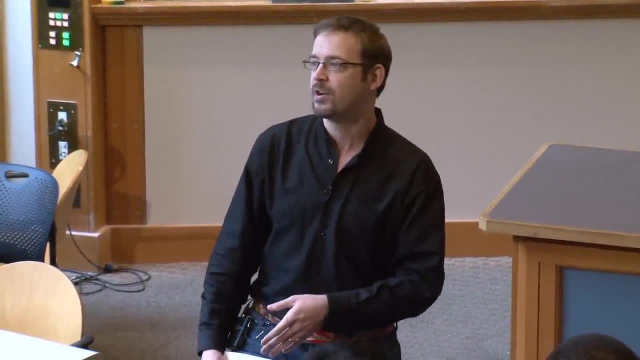 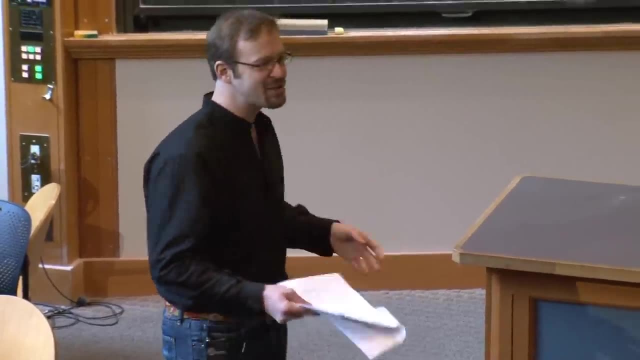 is that the way I've organized this class is not so much based on teaching what actually makes you learn better, And clickers are an excellent example of that. So this is mostly a standard lecture course, but there will be clickers used. 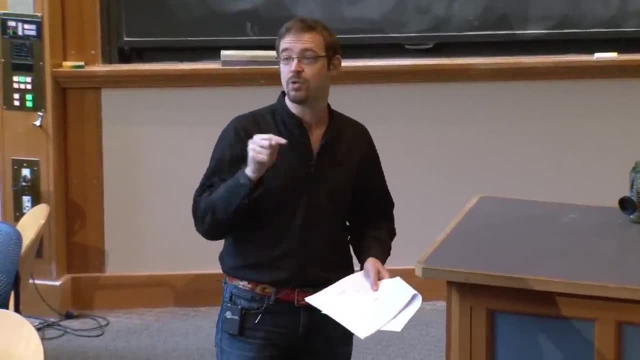 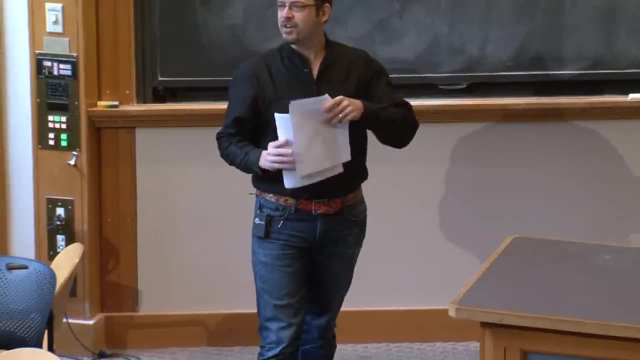 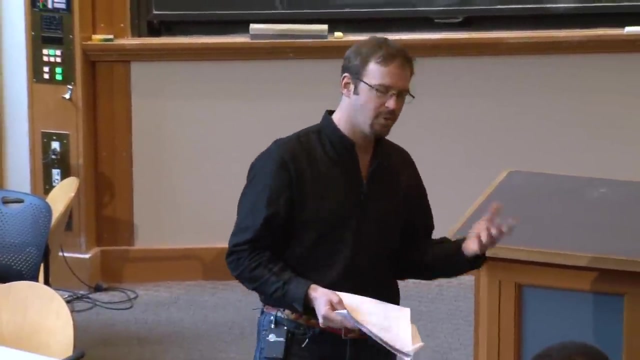 So by next week I need you all to have clickers and I need you all to register them on the TSG website. So I haven't chosen a specific textbook and this is discussed on the Stellar web page. There are a set of textbooks, four textbooks. 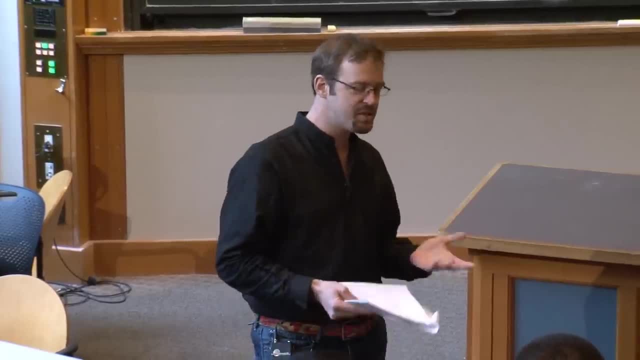 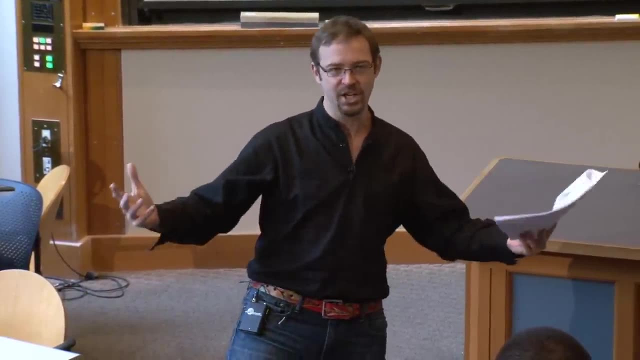 that I strongly recommend and a set of others that are nice references. The reason for this is twofold. First off, there are two languages that are canonically used for quantum mechanics. One is called wave mechanics and the language, the mathematical language, is partial differential. 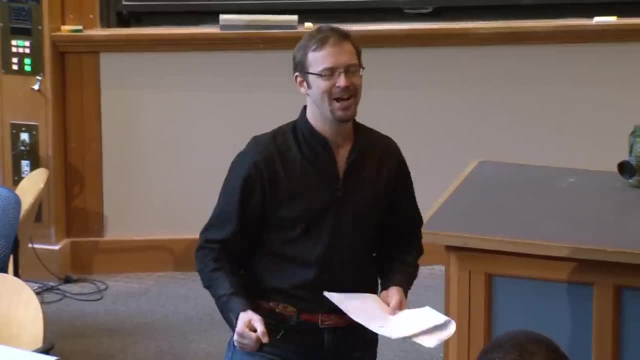 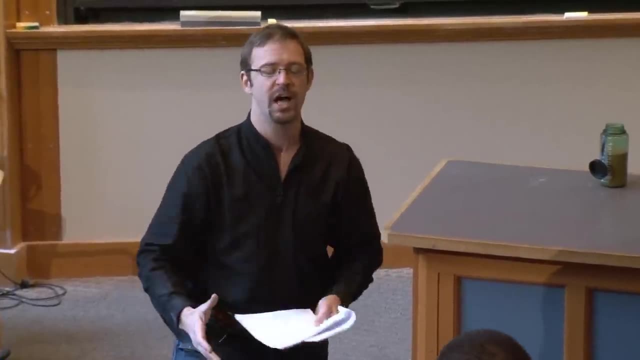 equations, The other is matrix mechanics. They have big names And the language. there is linear algebra And different books emphasize different aspects and use different languages And they also try to aim at different problems. Some books are aimed towards people who are interested in materials science. 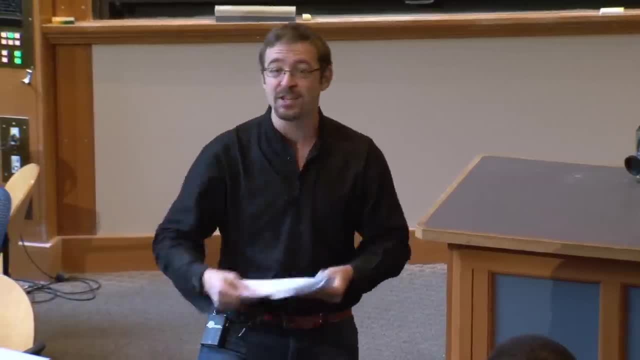 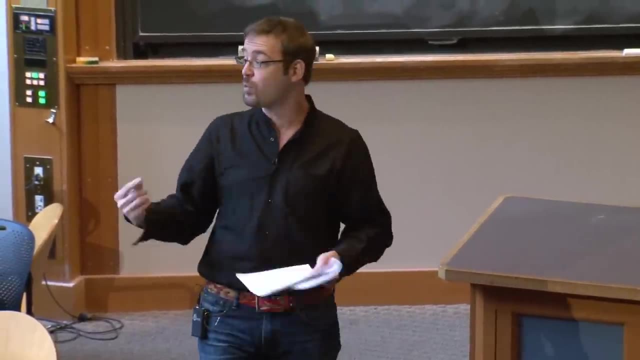 Ty opportunities And others are aim at different problems. Ty opportunities, some books that are aimed towards people interested in philosophy, And, depending on what you want, get the book that's suited to you And every week I'll be providing with your problem. 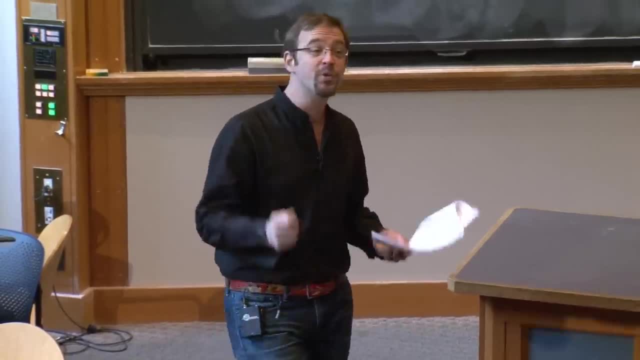 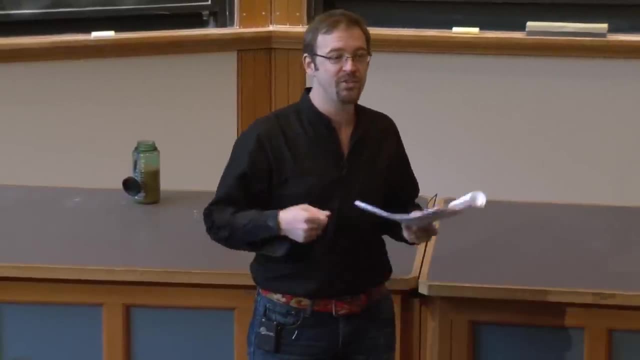 sets readings from each of the recommended texts. So what I really encourage you to do is find a group of people to work with every week and make sure that you've got all the books covered between you. This will give you as much access to the text. 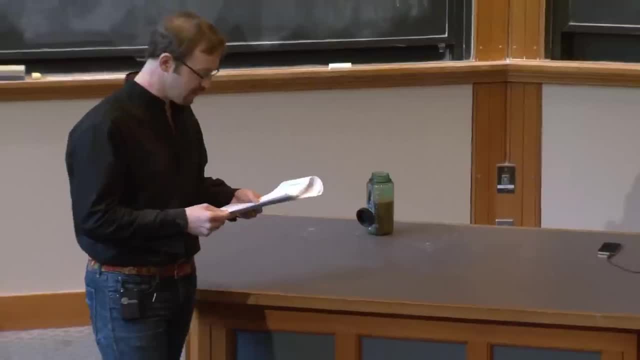 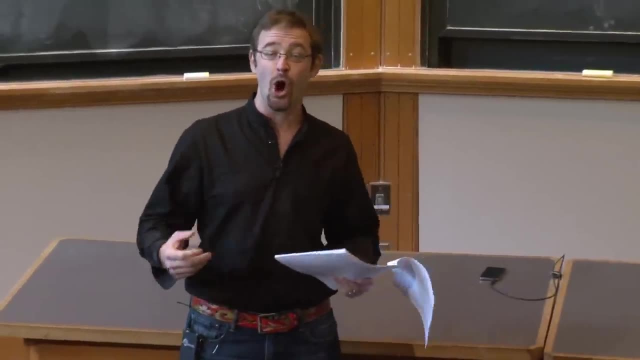 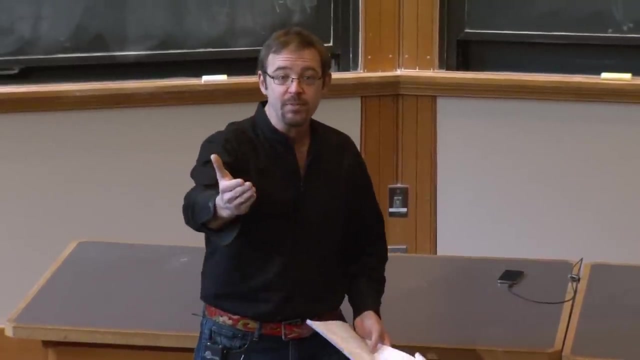 as possible without forcing you to buy four books, which I would discourage you from doing So. finally, I guess the last thing to say is: if this stuff were totally trivial, you wouldn't need to be here. So ask questions If you're confused about something. 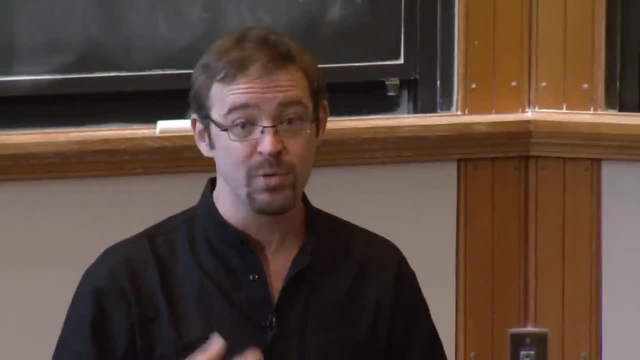 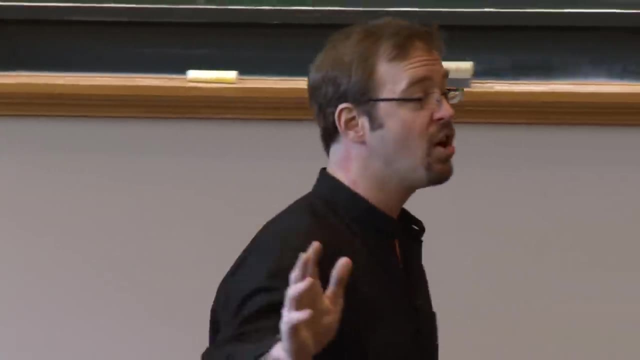 lots of other people in the class are also going to be confused, And if I'm not answering your question without you asking, then no one's getting the point. So ask questions, Don't hesitate to interrupt. Just raise your hand and I will do my best to call on you. 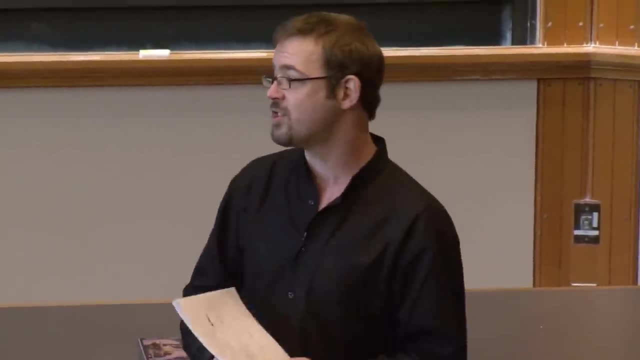 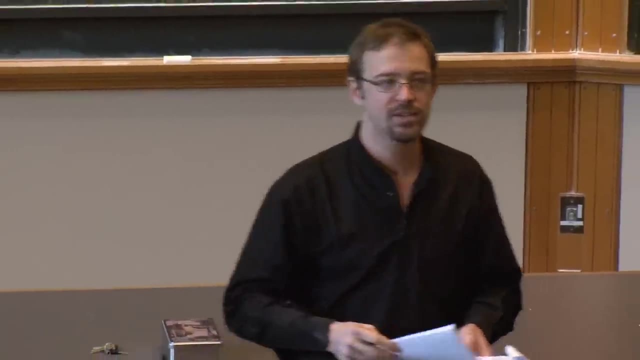 And this is true both in lecture- Also go to office hours And recitations, ask questions. I promise there's no such thing as a terrible question. Someone else will also be confused. So it's very valuable to me and everyone else. 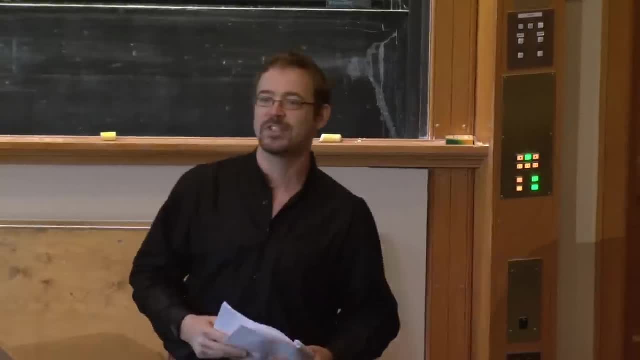 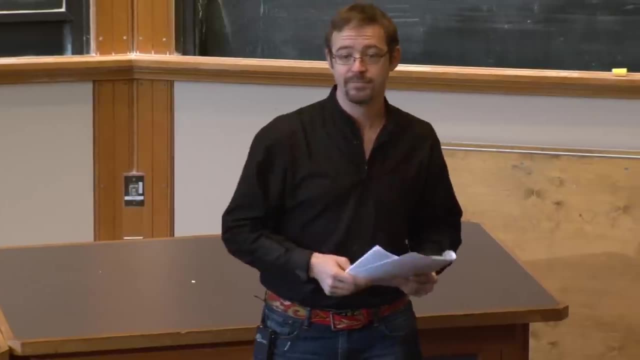 OK, So before I get going on the actual physics content of the class, are there any other practical questions? Yeah, What did you say was the lateness policy? Lateness policy: No late work is accepted whatsoever. So you're saying there's like a makeup for it? 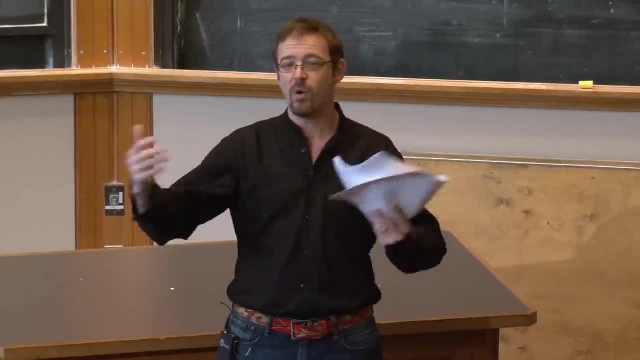 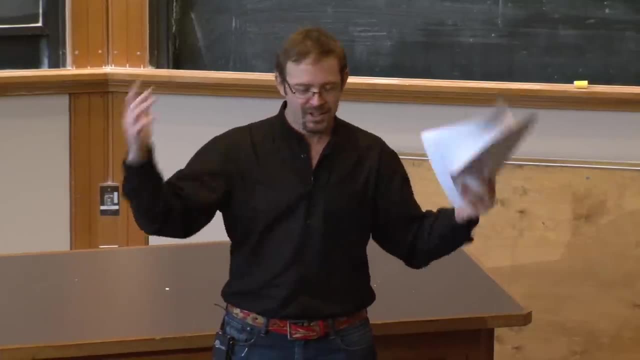 There is. So the deal is Given that every once in a while you're going to be walking to school and your leg is going to fall off, or a dog's going to jump out and eat your person standing next to you. whatever things happen, 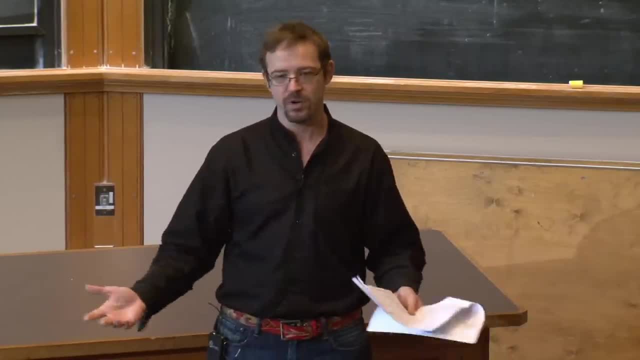 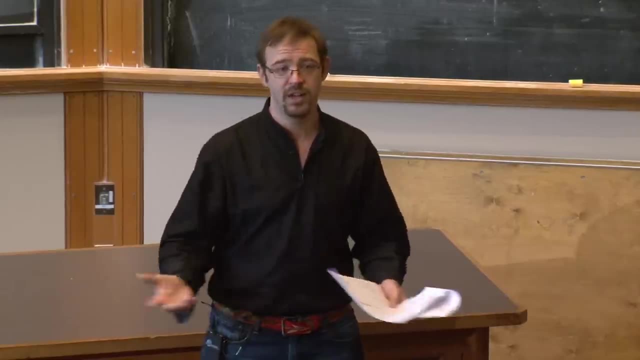 So we will drop your lowest problem set score without any questions. At the end of the semester, we'll just drop your lowest score And if you turn them all in, great Whatever, your lowest score was fine. If you missed one, then gone. 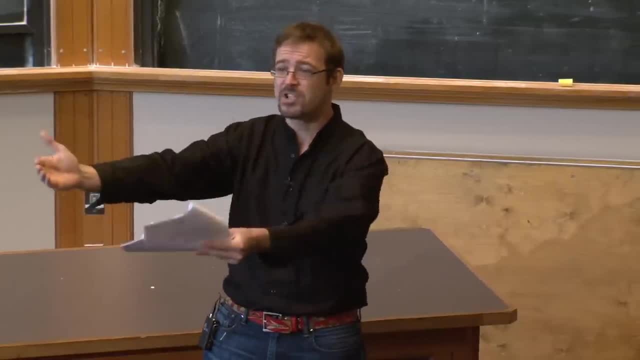 On the other hand, if you know, next week I'm going to be attacked by a rabid squirrel. it's going to be horrible. I don't want to have to worry about my problem set. OK. OK, Could we work this out? 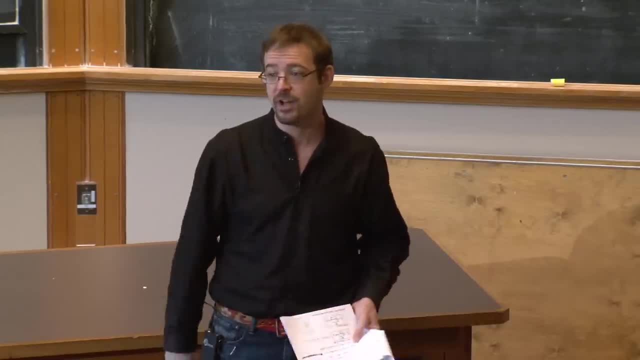 So if you know ahead of time, come to us. But you need to do that well ahead of time. the night before doesn't count. OK, Yeah, Would we be able to watch the videos? You know? that's an excellent question. 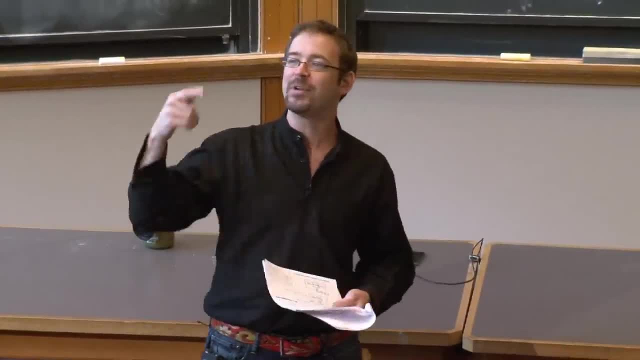 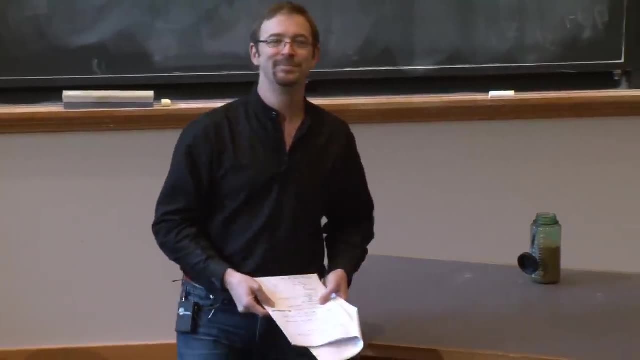 I don't know. I don't think so. I think it's going to happen at the end of the semester. Yeah, OK, So no, You'll be able to watch them later on the OCW website. Other questions? Yeah? 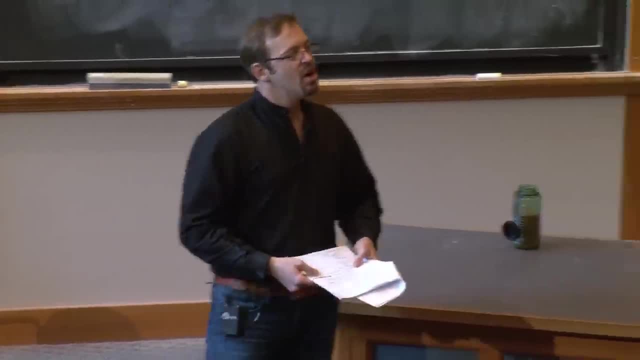 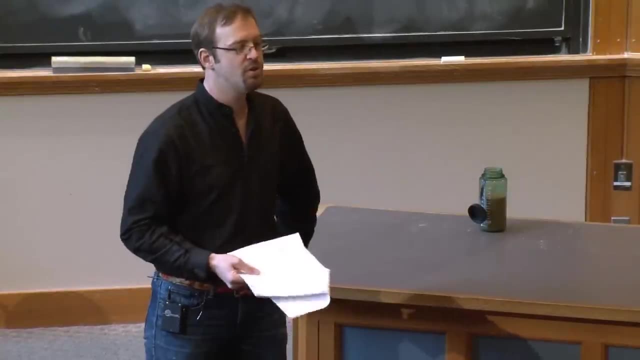 Do you have any other videos that you recommend, Like other courses on YouTube? Oh, that's an interesting question. I don't know off the top of my head, but if you send me an email I'll presume, because I do know several other lecture series. 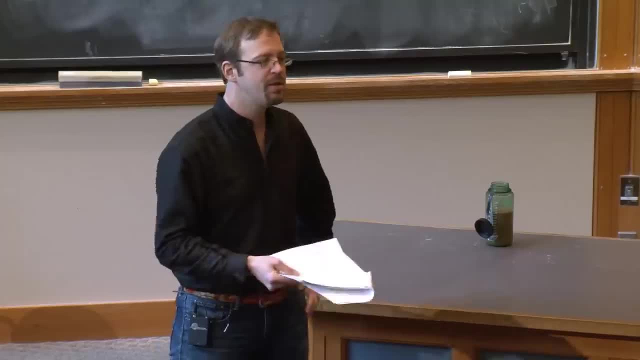 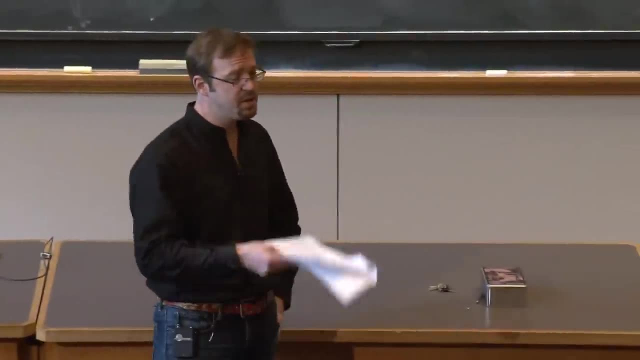 that I like very much, but I don't know if they're available on YouTube or publicly, So send me an email and I'll check. Yeah, How about the reading assignments? Reading assignments on the problem set every week will be listed. There will be equivalent reading from every textbook. 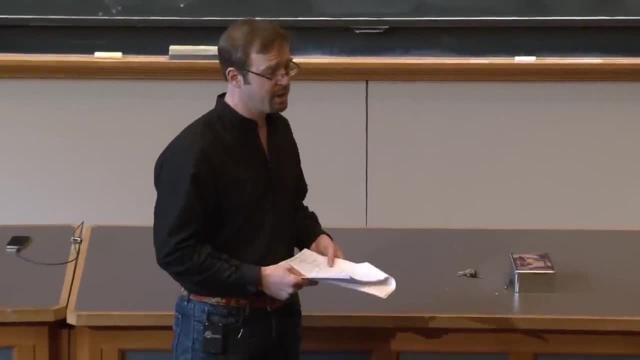 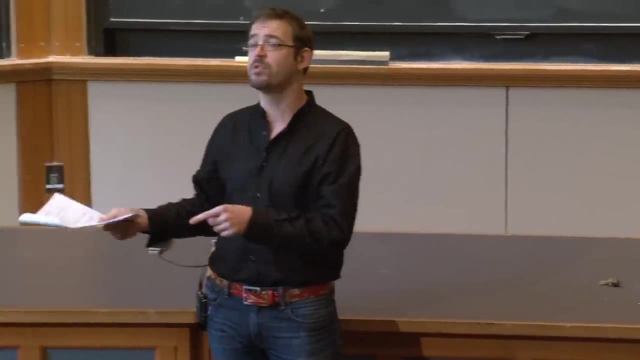 And if there is something missing, like if no textbook covers something, I'll post a separate reading Every once in a while, I'll post auxiliary readings and they'll be available on the Stellar website. So, for example, on your problem set, which is first one. 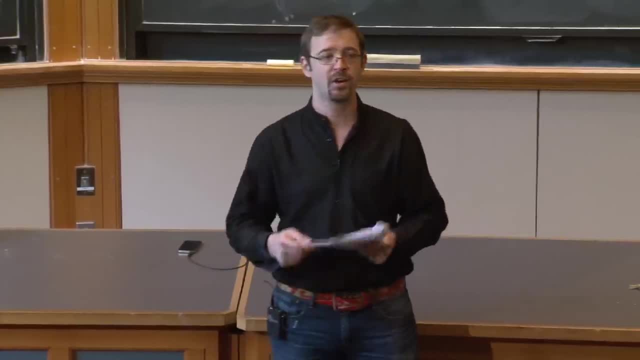 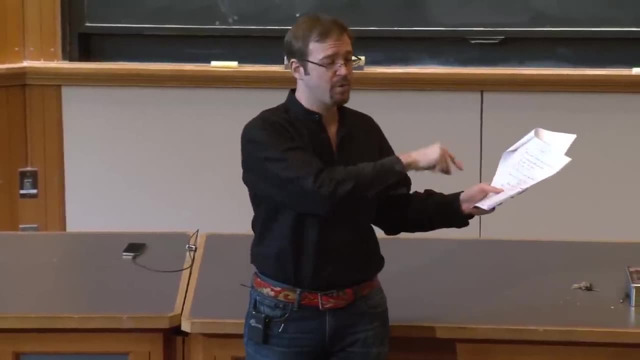 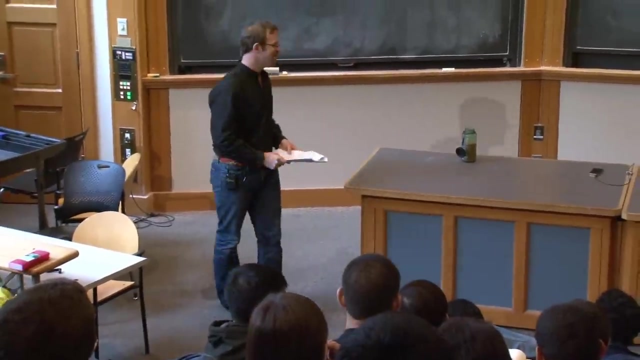 was posted will be available immediately after a lecture on the Stellar website. There are three papers that it refers to, or two, and they're posted on the Stellar website and linked from the problem set. Cool Others, OK. So the first lecture, the content. 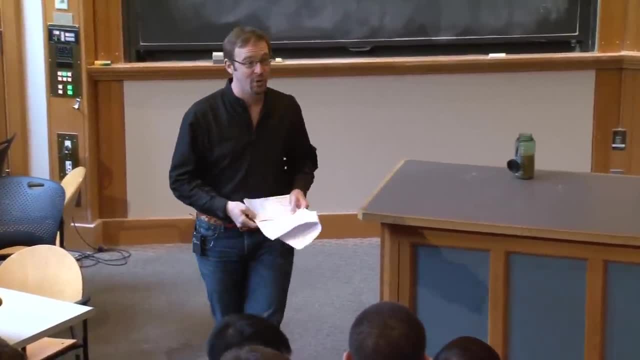 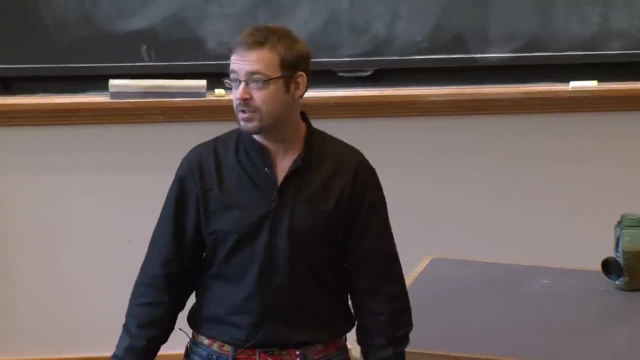 of the physics of the first lecture is relatively stand-up. It's going to be an introduction to a basic idea that is going to haunt, plague and charm us through the rest of the semester. OK, The logic of this lecture is based. 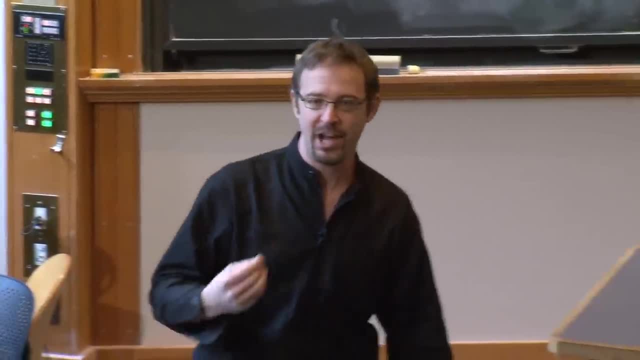 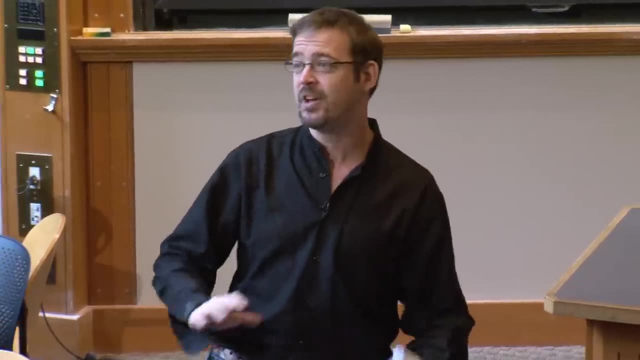 on a very beautiful discussion in the first few chapters of a book by David Albert called Quantum Mechanics and Experience. It's a book for philosophers, but the first few chapters are a really lovely introduction at a non-technical level and I encourage you to take a look at them. 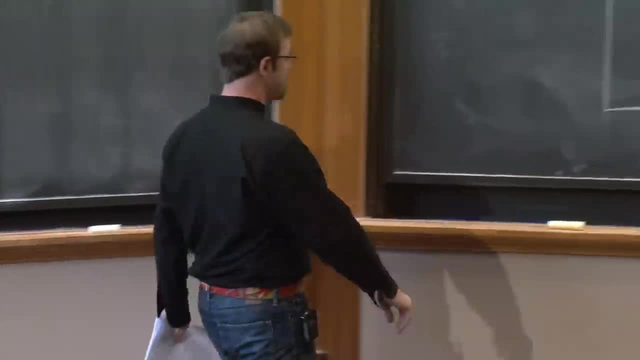 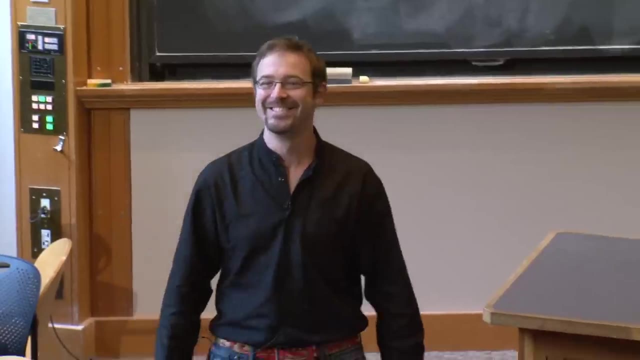 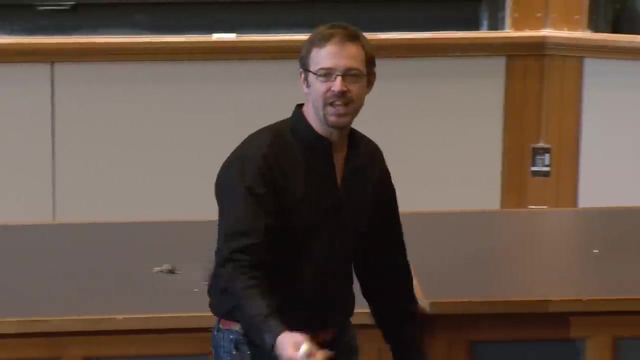 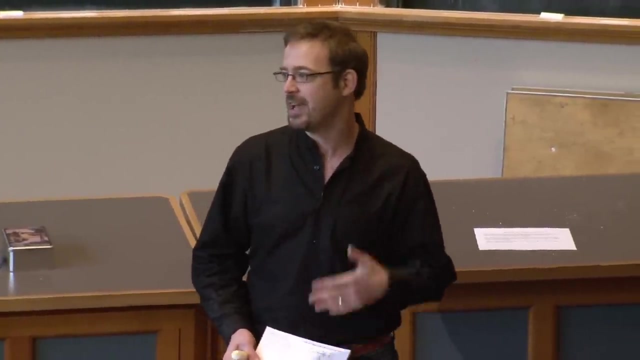 because they're very lovely. But it's to be sure, OK, Sure, Straight up physics. OK, Ready, I love this stuff. So today I want to describe to you a particular set of experiments. Now, to my mind, these are the most unsettling experiments. 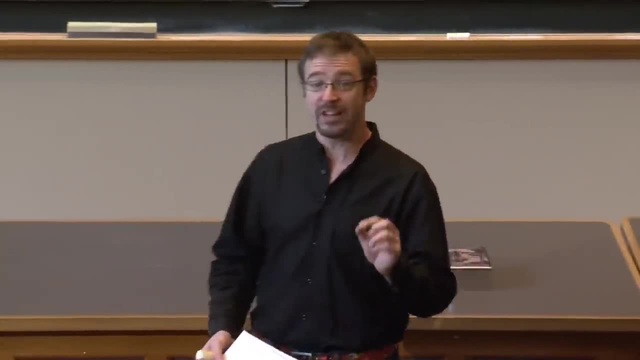 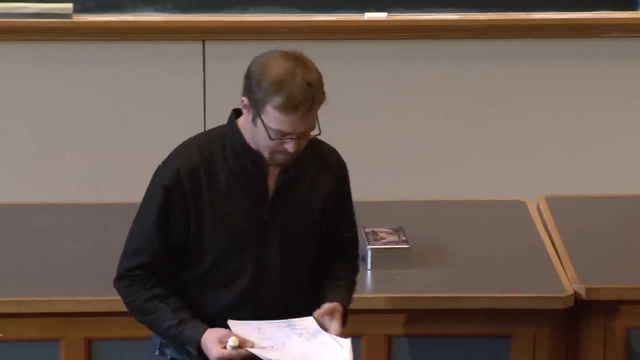 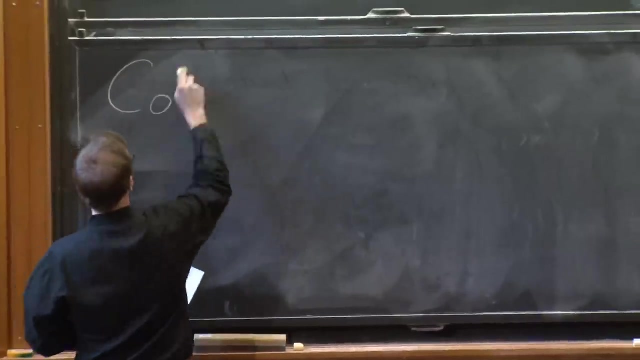 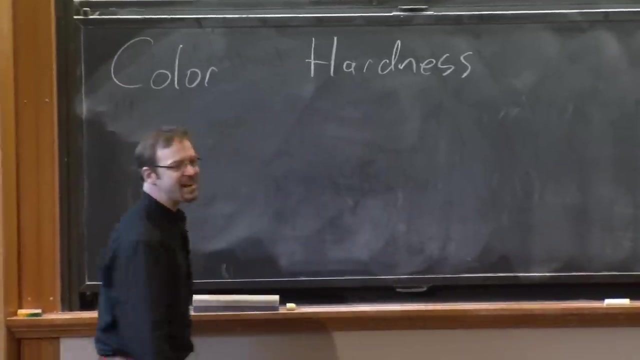 ever done. These experiments involve electrons. They have been performed and the results, as I will describe them, are true. I'm going to focus on two properties of electrons. I will call them color and hardness, And these are not the technical names. 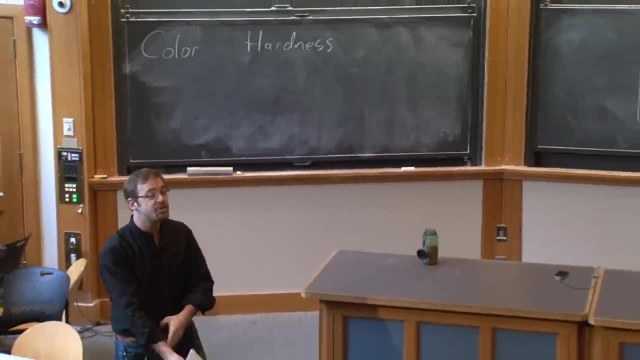 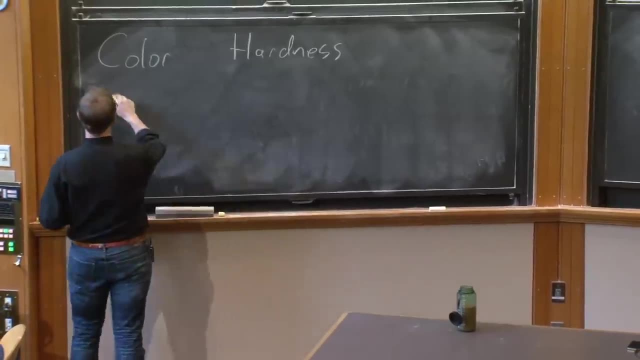 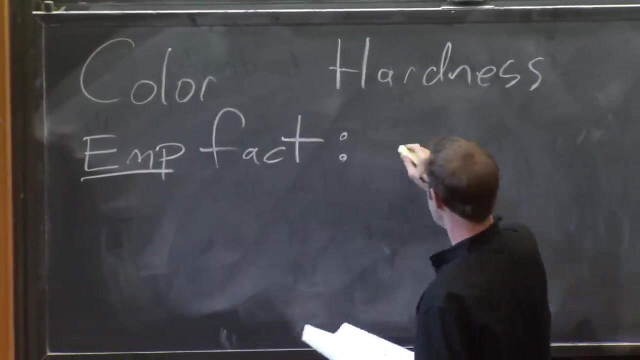 We'll learn the technical names for these properties later on in the semester, But to avoid distracting you by preconceived notions of what these things mean, I'm going to use ambiguous labels. color and hardness, And the empirical fact Is that every electron that's ever been observed 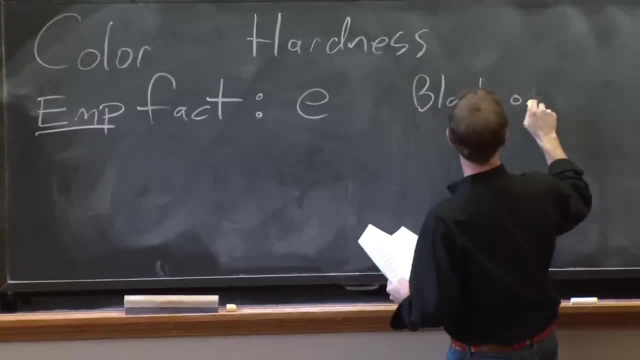 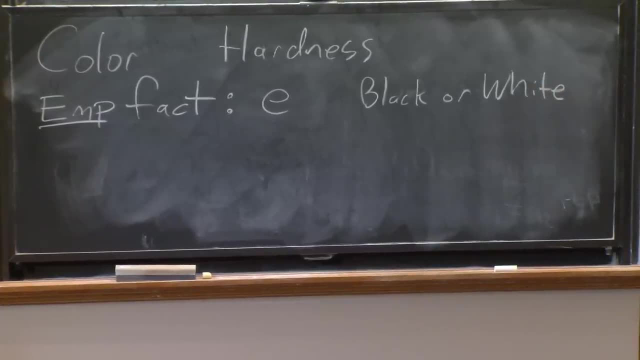 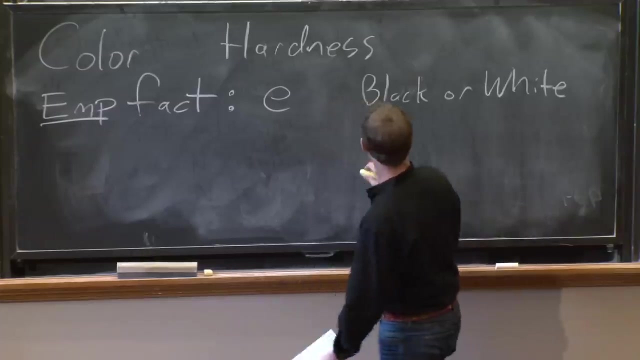 is either black or white and no other color. We've never seen a blue electron. There are no green electrons. No one has ever found a fluorescent electron. They're either black or they are white. It is a binary property. Secondly, their hardness is either hard or soft. 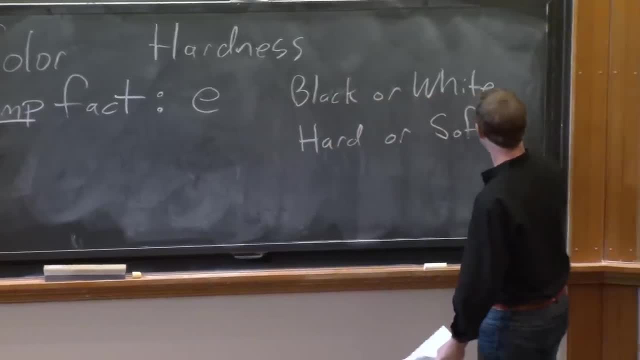 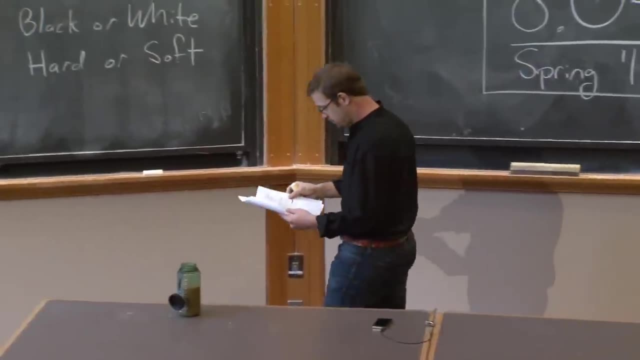 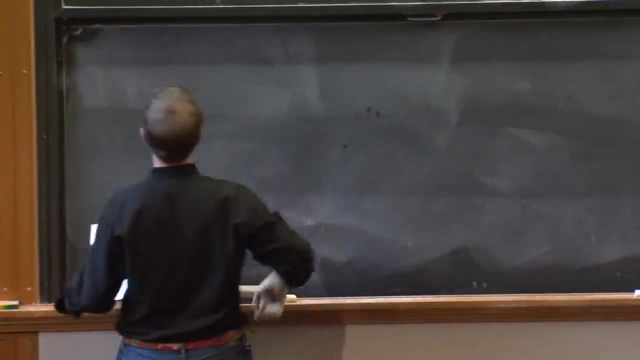 OK, They are never squishy. No one's ever found one that dribbles. They're either hard or they are soft Binary properties. OK Now, what I mean by this is that it is possible to build a device which measures the color and the hardness. 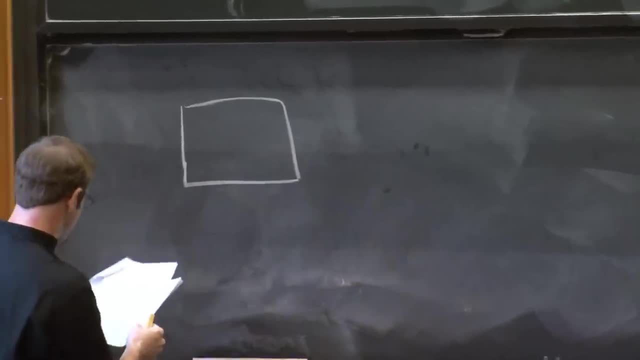 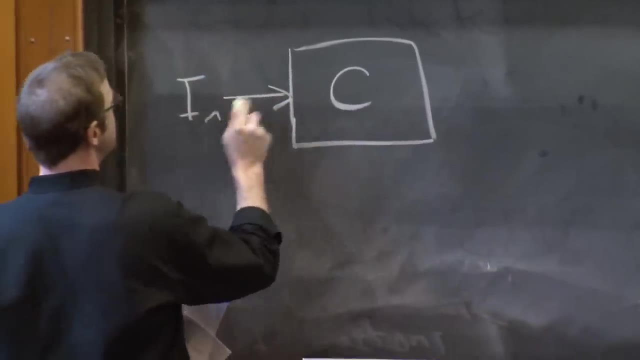 In particular, it is possible to build a box, which I will call a color box, that measures the color, And the way it works is this: It has three apertures, an in-port and two out-ports, one which sends out black electrons. 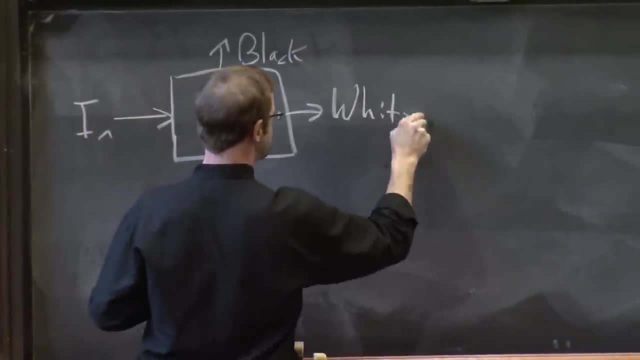 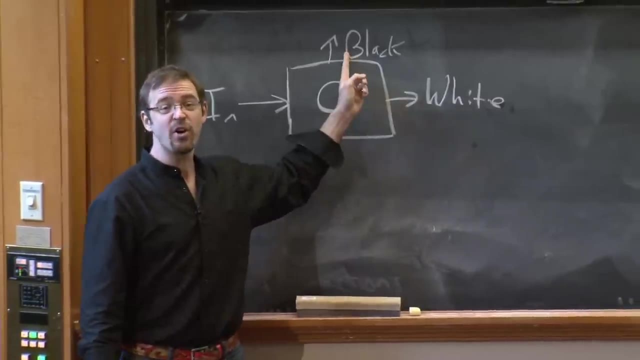 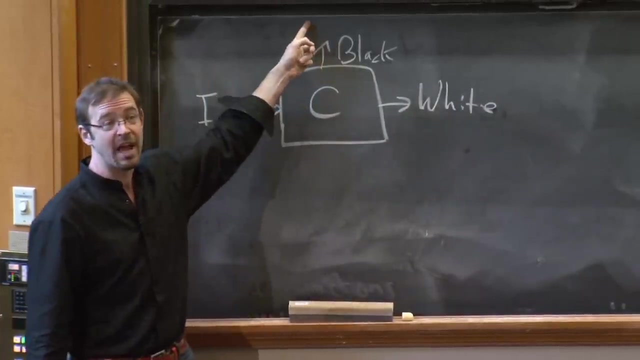 and one which sends out white electrons. And the utility of this box is that the color can be inferred from the position. If you find the electron over here, it is a white electron. If you find the electron here, it is a black electron. 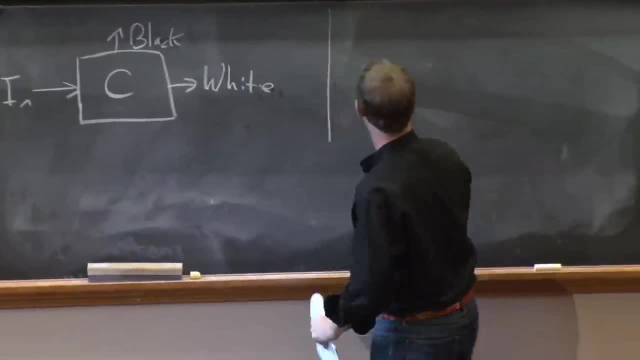 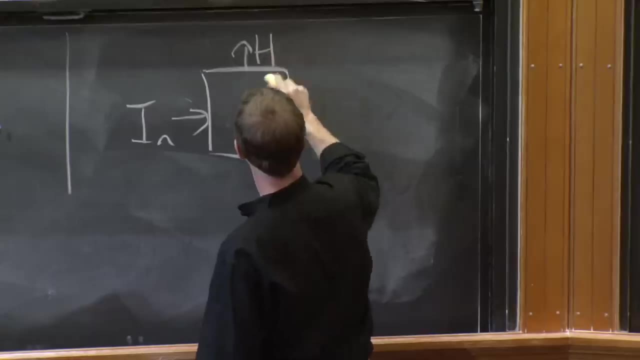 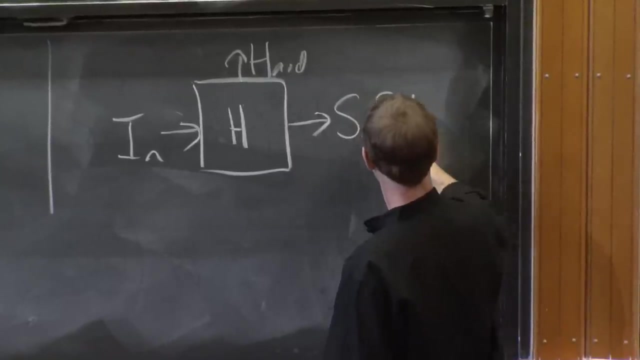 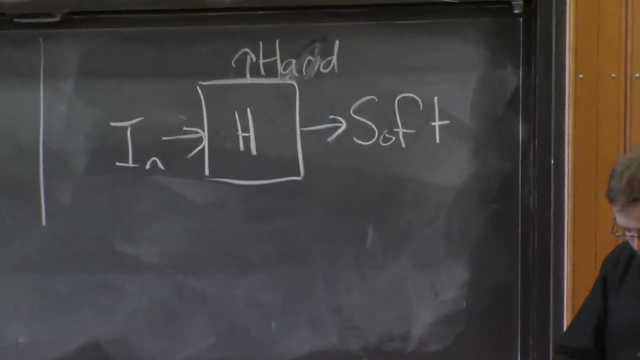 Cool. Similarly, We can build a hardness box which again has three apertures: an in-port, and hard electrons come out this port, and soft electrons come out this port. OK, Now, if you want, you're free to imagine. 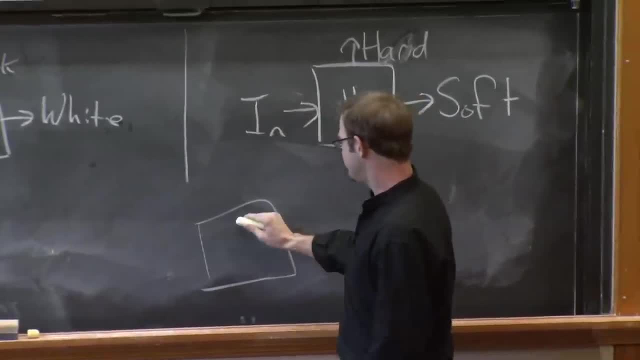 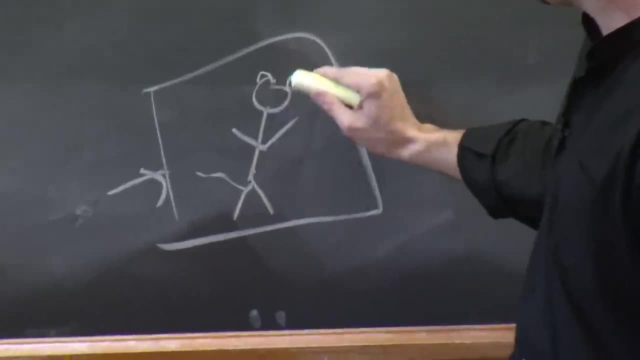 that these boxes are built by putting you know a monkey inside And you send in an electron And the monkey you know, with ears, looks at the electron and says: you know, it's a hard electron that sends it out. 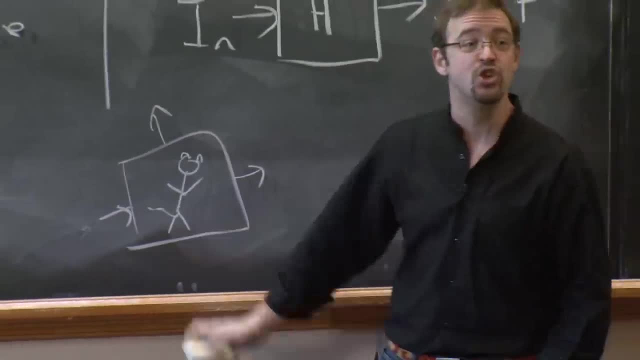 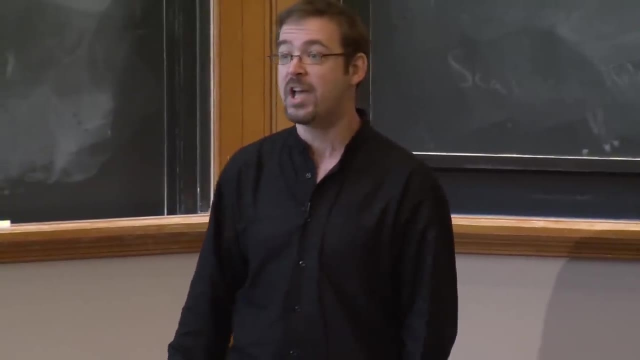 one way, or it's a soft electron that sends out the other. The workings inside do not matter And in particular later in the semester, I will describe in considerable detail the workings inside this apparatus. And here's something I want to emphasize to you. 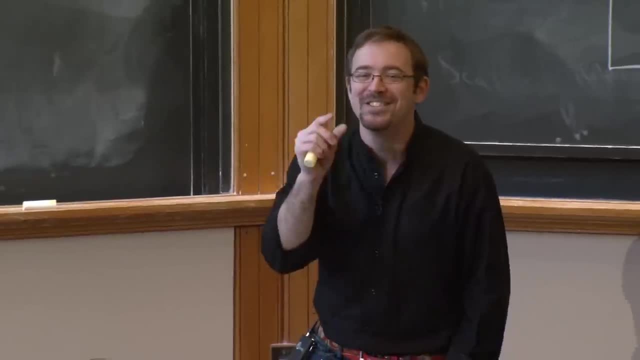 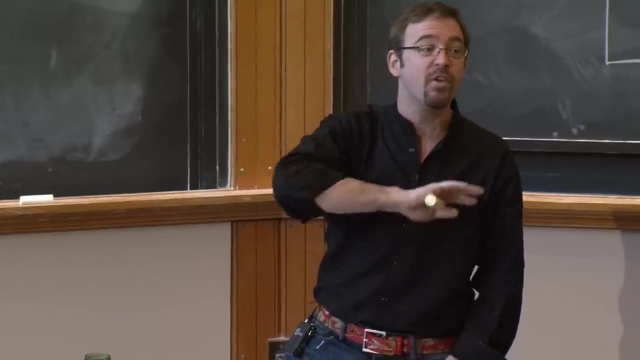 It can be built in principle using monkeys, hyper-intelligent monkeys that can see electrons. It can also be built using magnets and silver atoms. It can be done with neutrons. It can be done with all sorts of different technologies, And they all give precisely the same results. 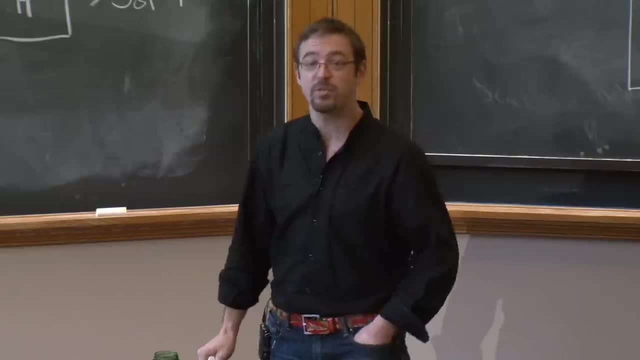 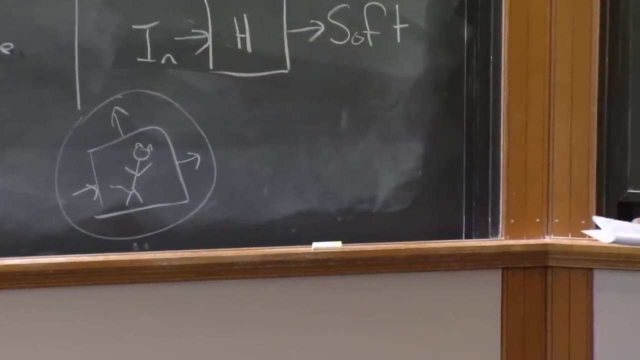 as I'm about to describe. OK, They all give precisely the same results, So it does not matter what's inside, But if you want a little idea, you can imagine putting a monkey inside a hyper-intelligent monkey. I don't know. 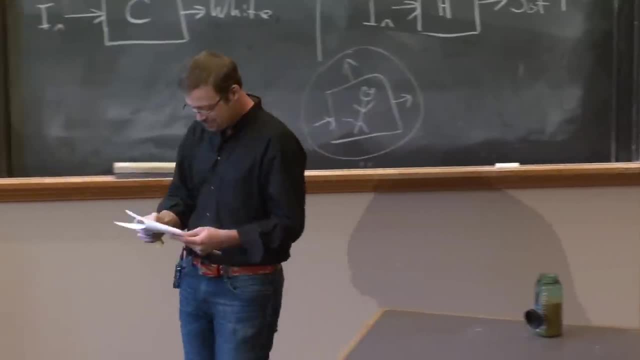 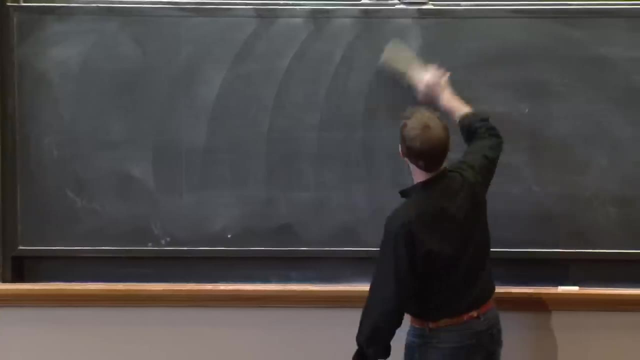 It sounds good, So I'm going to call it yeah. So a key property of these hardness boxes and color boxes is that they are repeatable, And here's what I mean by that. If I send in an electron and I find 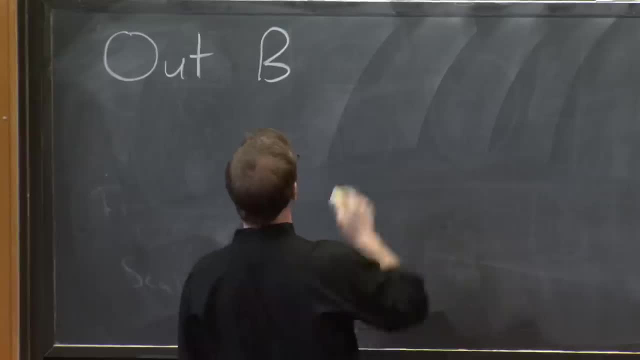 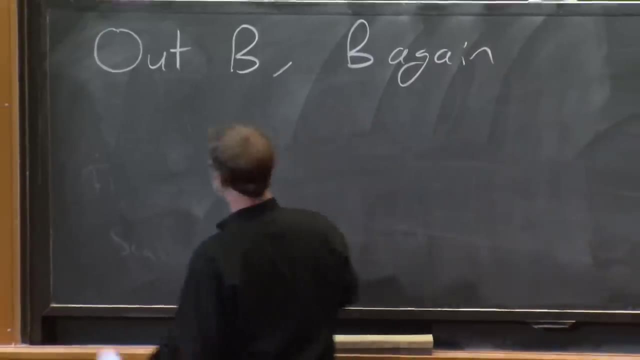 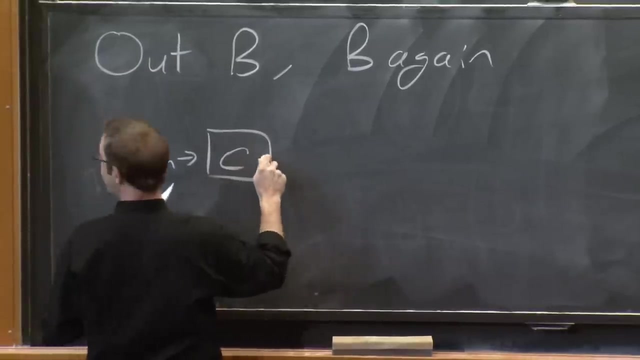 that it comes out of a color box black and then I send it in again. then if I send it into another color box it comes out black again. So in diagrams, if I send in some random electron to a color box and I discover that it comes, 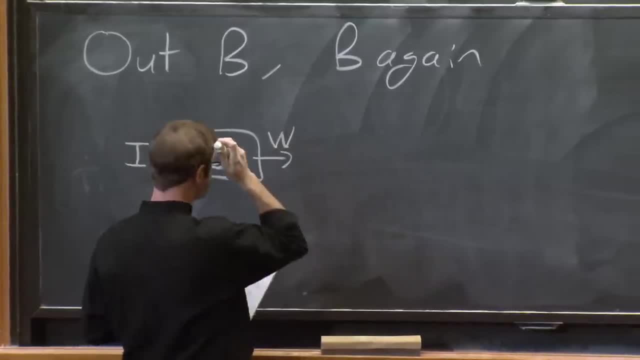 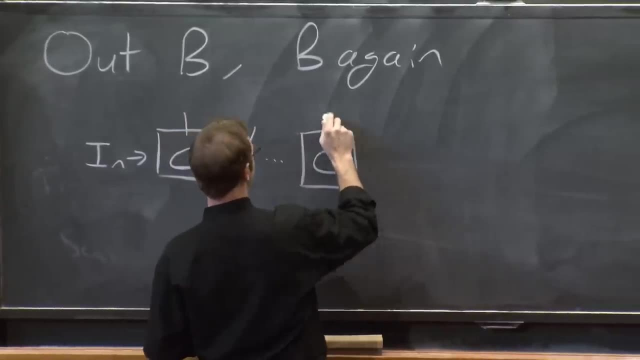 out, let's say the white aperture, and so here's dot dot dot, and I take the ones that come out of the white aperture and I send them into a color box again. then, with 100% confidence, 100% of the time, the electron coming out. 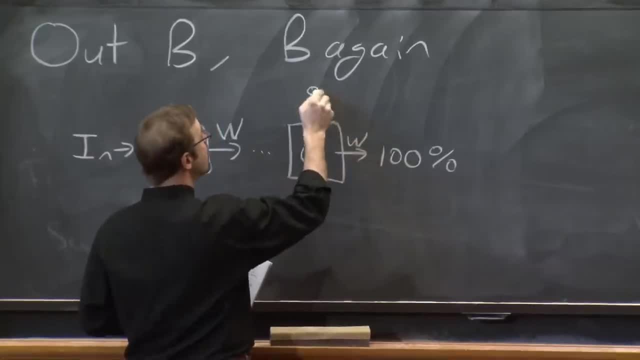 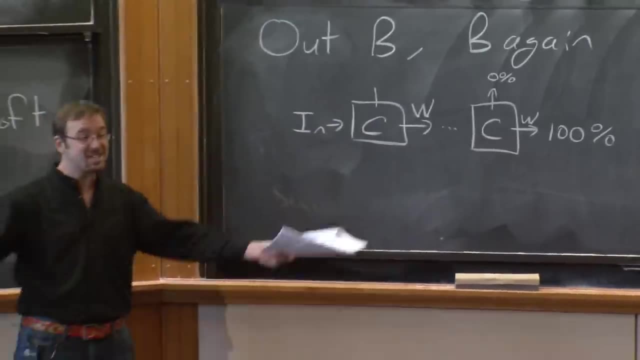 of the white incident on the color box will come out the white aperture again, And 0% of the time will it come out the black aperture. So this is a persistent property. You notice that it's white. You measure it again, it's still white. 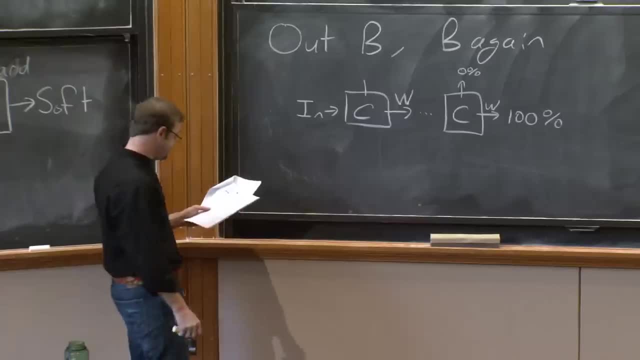 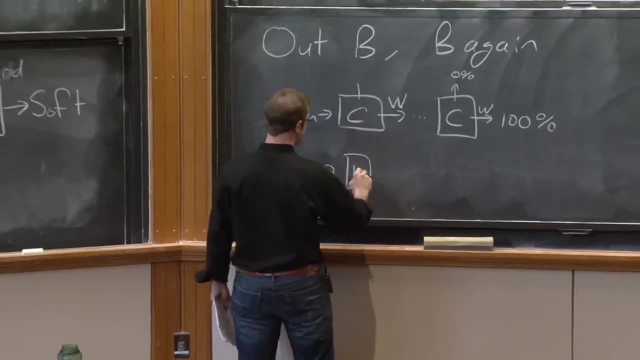 Do it a little bit later It's still white. It's a persistent property. Ditto the hardness. If I send in a bunch of electrons into a hardness box, here's an important thing. Well, send them into a hardness box. 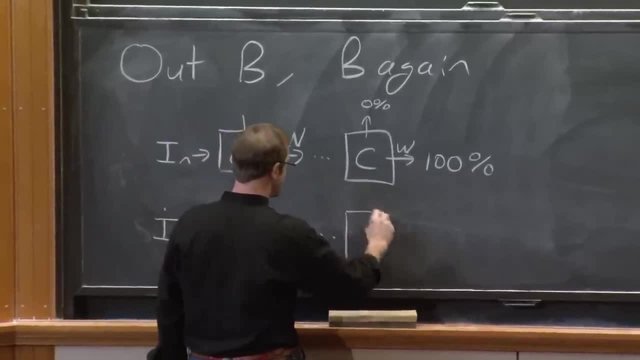 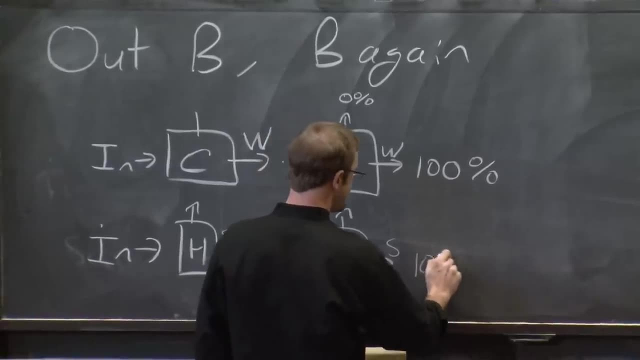 and I take out the ones that come out soft and I send them again into a hardness box and they come out soft. They will come out soft with 100% confidence, 100% of the time. Never do they come out the hard aperture. 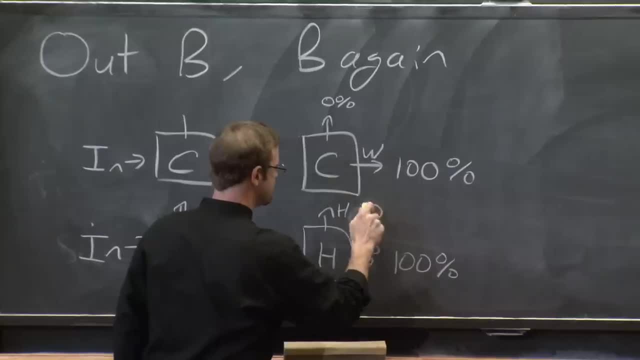 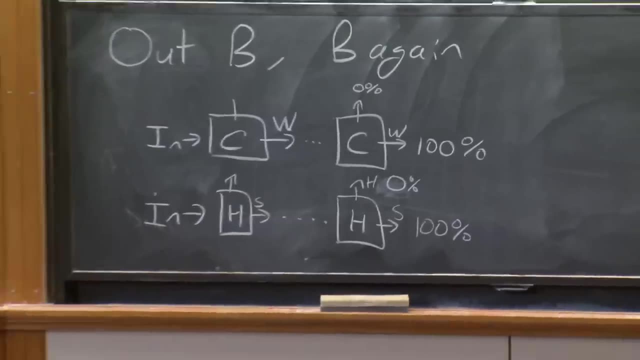 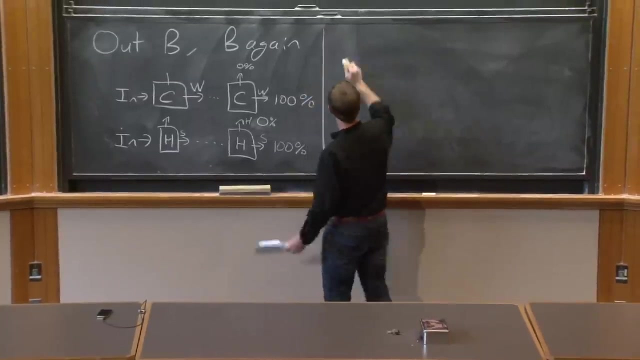 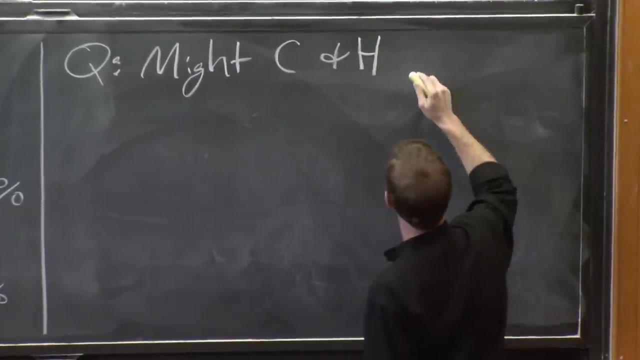 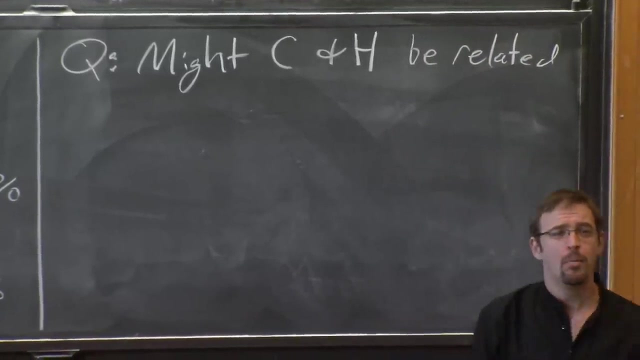 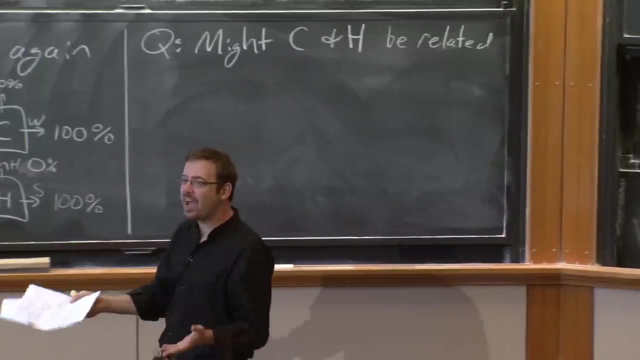 OK, Any questions at this point? So here's a natural question: Might the color and the hardness of an electron be related? And more precisely, Might they be correlated? Might knowing the color infer something about the hardness? So, for example, so being male and being a bachelor. 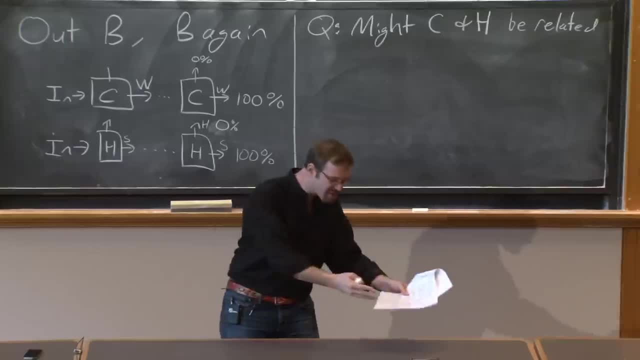 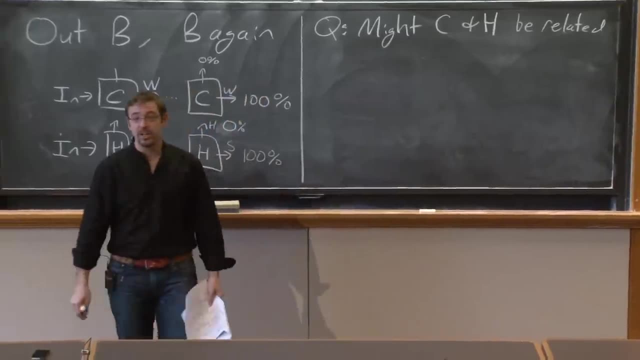 are correlated properties, Because if you're male, you don't know if you're a bachelor or not, But if you're a bachelor you're male. That's the definition of the word. So is it possible that color and hardness are similarly correlated? 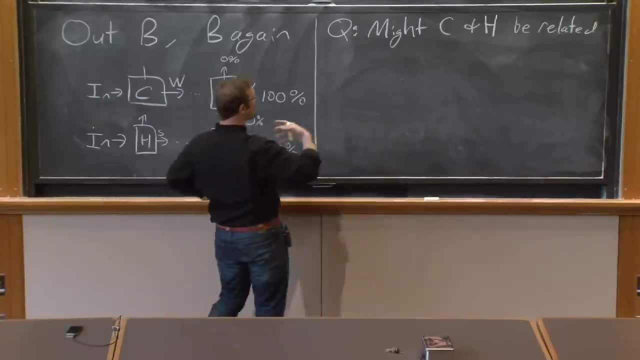 So I don't know. There are lots of good examples Wearing a red shirt and beaming down to the surface and making it back to the inner world, Making it back to the Enterprise later after the away team returns. Correlated right. 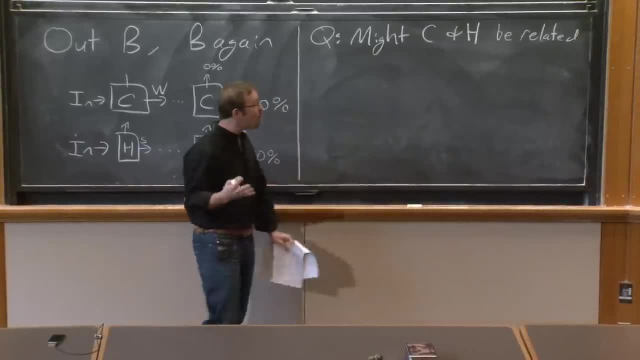 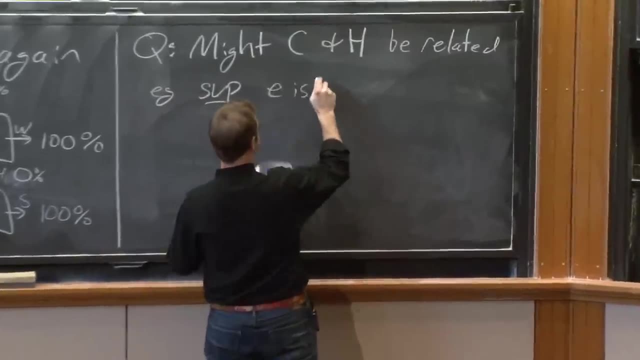 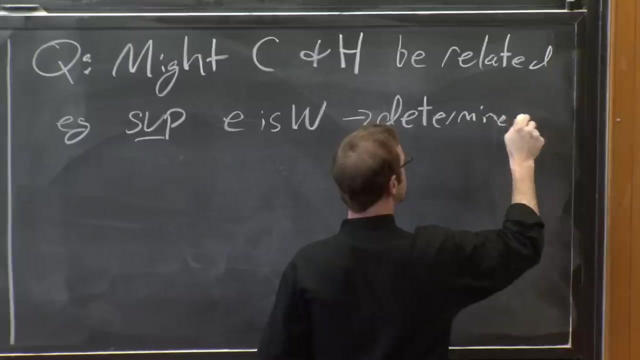 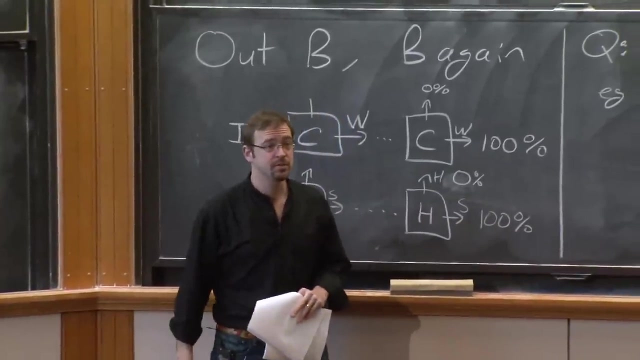 Negatively, but correlated. So the question is: suppose, eg suppose we know that an electron is white, does that determine the hardness? So we can answer this question by using our boxes. Yeah, So here's what I'm going to do. 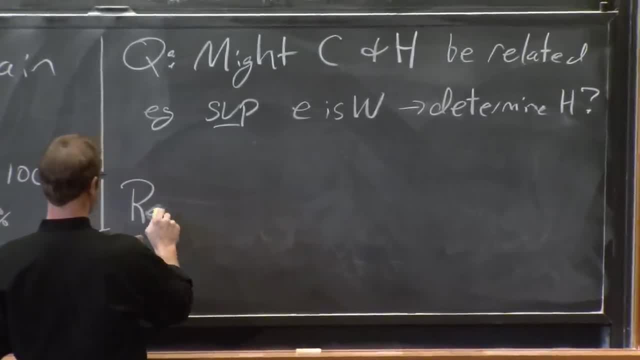 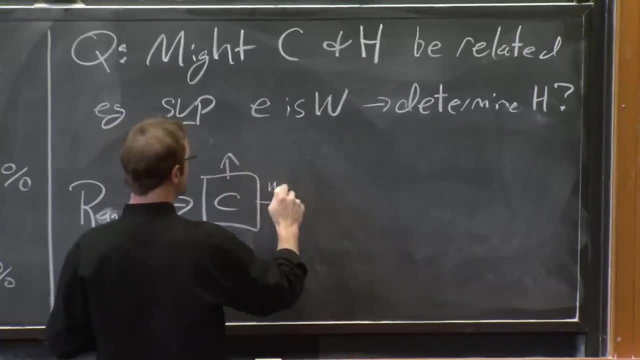 I'm going to take some random set of electrons- That's not random, Random- And I'm going to send them into a color box And I'm going to take the electrons that come out, the wide aperture. And here's a useful fact. 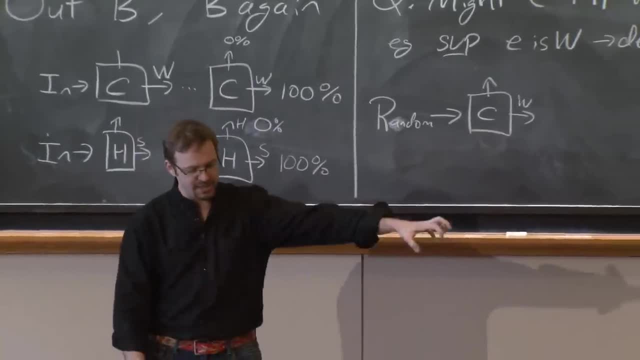 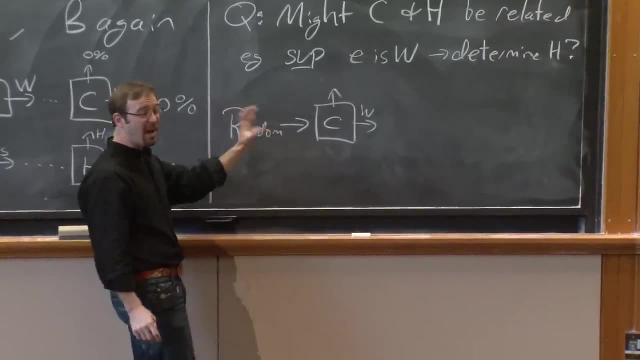 When I say random, here's operationally what I mean. I take some piece of material, I scrape it, I pull off some electrons and they're totally randomly chosen from the material and I send them in. If I send a random pile of electrons, 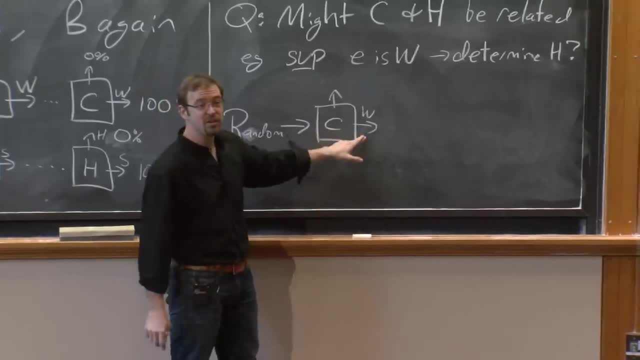 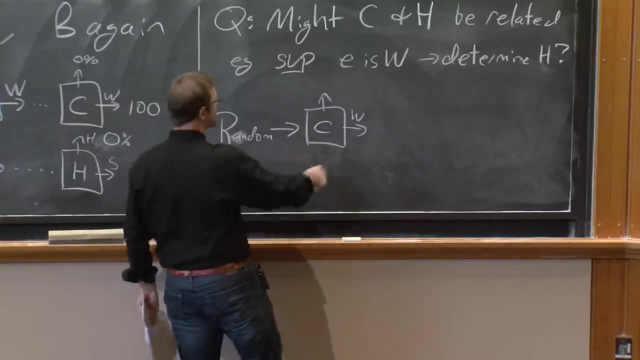 into a color box. useful thing to know. they come out about half and half. It's just some random assortment. Some of them are white, some of them come out black. Suppose I send some random collection of electrons into a color box and I take those which 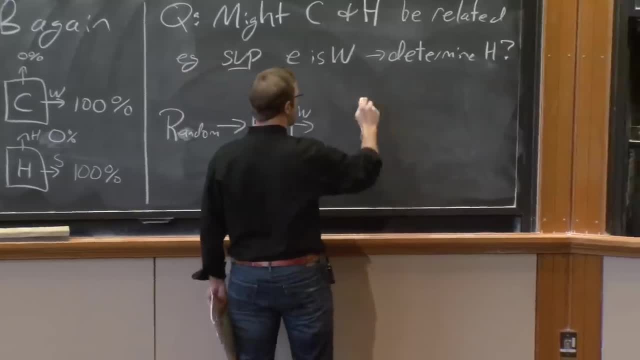 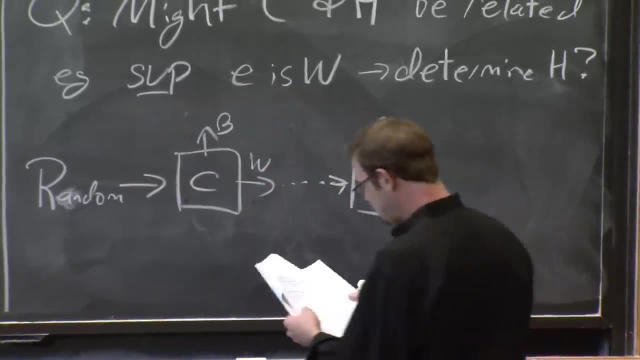 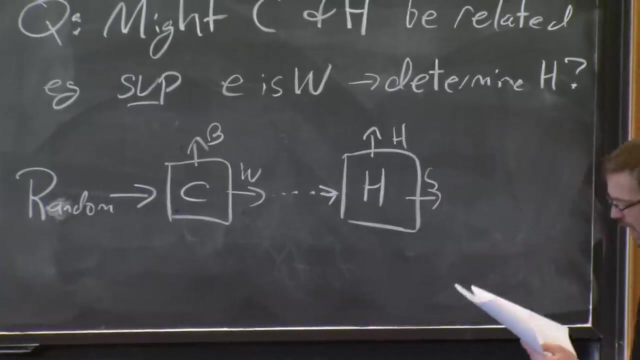 come out the wide aperture, And I want to know: does white determine hardness? So I can do that check by then, sending these white electrons into a hardness box and seeing what comes out, And what we find is that 50% of the white which 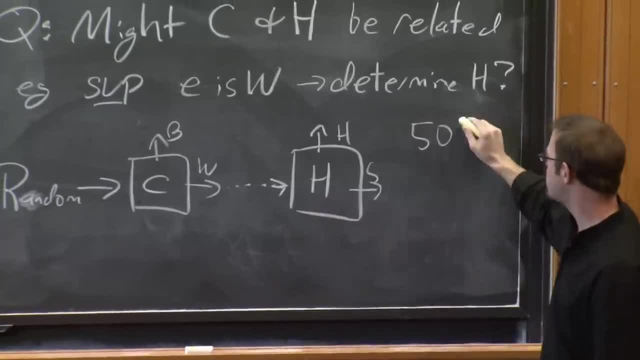 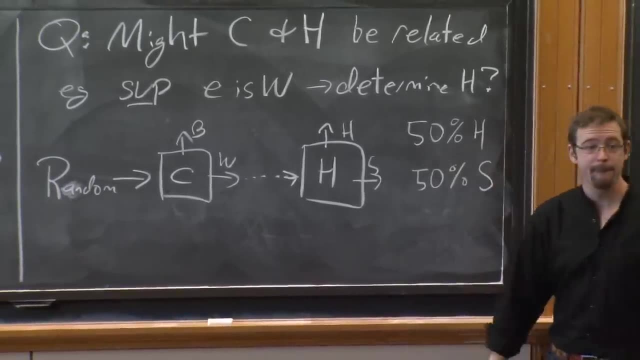 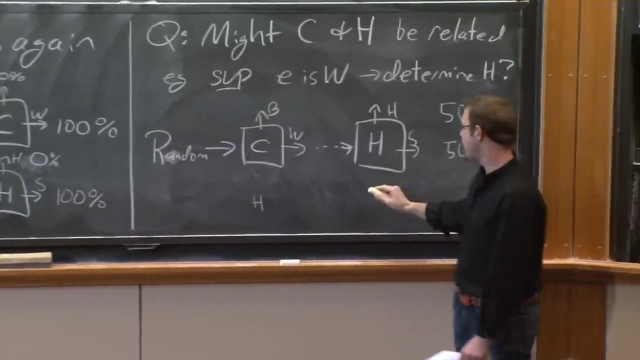 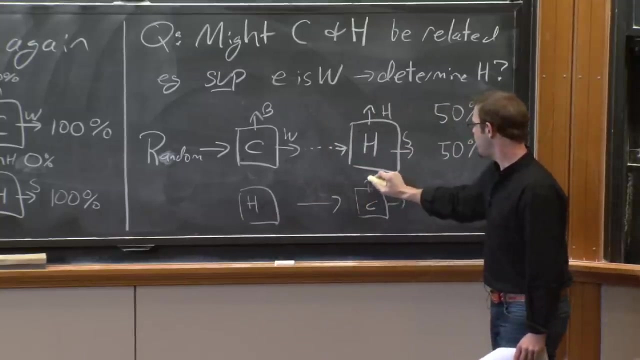 is 50% of those electrons incident on the hardness box come out hard And 50% come out soft And ditto. if we reverse this, If we take hardness and take, for example, a soft electron and send it into a color box, we again get 50-50.. 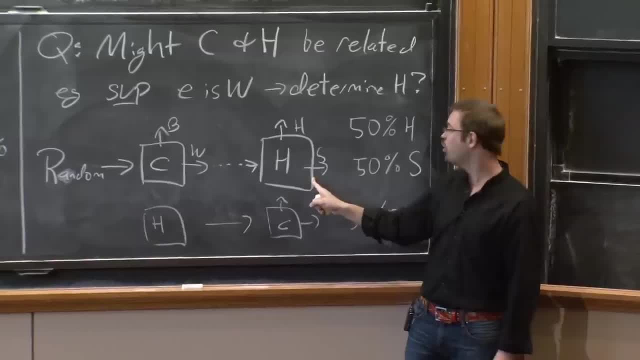 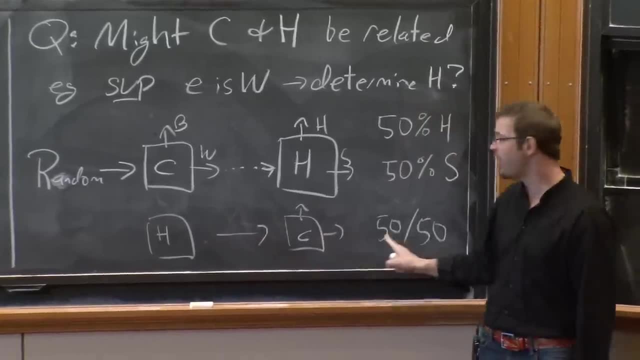 OK. So if you take a white electron, you send it into a hardness box, you're at even odds. You're at chance as to whether it's going to come out hard or soft. And similarly, if you send a soft electron into a color box, 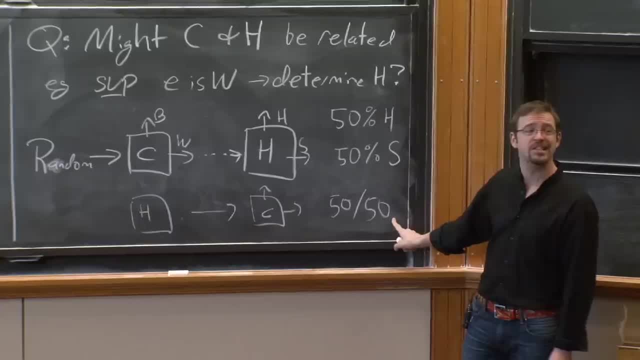 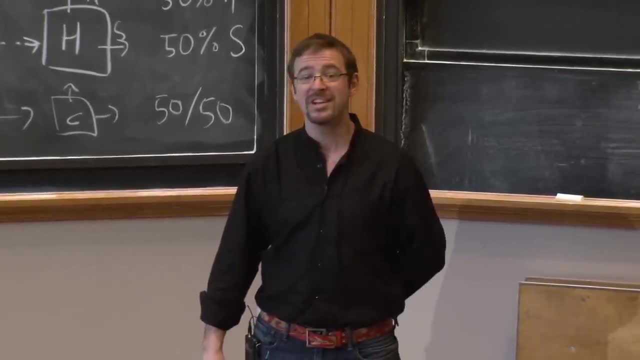 even odds, it's going to come out black or white, OK. So knowing the hardness does not give you any information about the color, and knowing the color does not give you any information about the hardness. Cool, These are independent facts, independent properties. 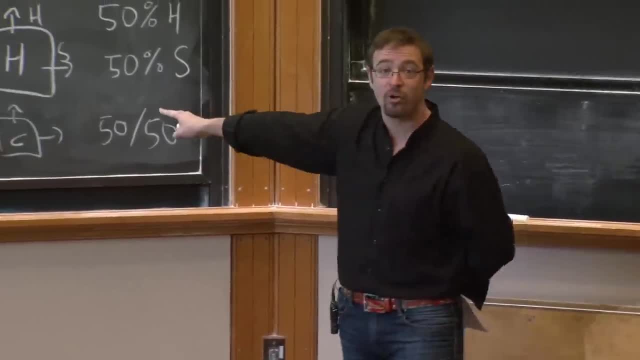 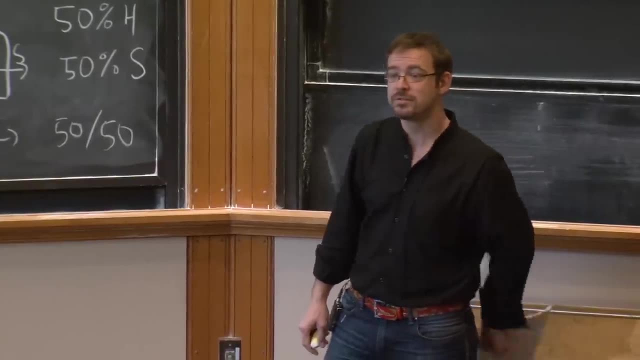 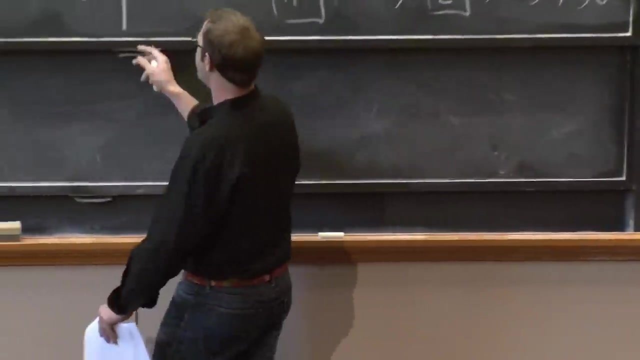 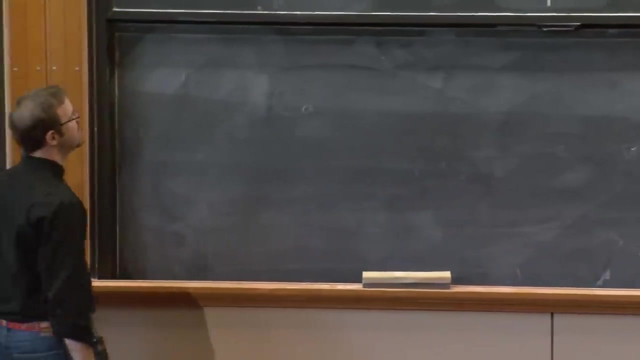 They're not correlated in this sense, in precisely this operational sense. OK, Cool Questions. OK, So measuring the color gives zero predictive power for the hardness and measuring the hardness gives zero predictive power for the color, And from that I will say that these properties 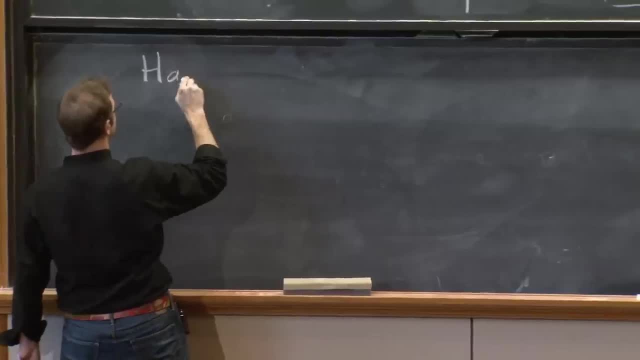 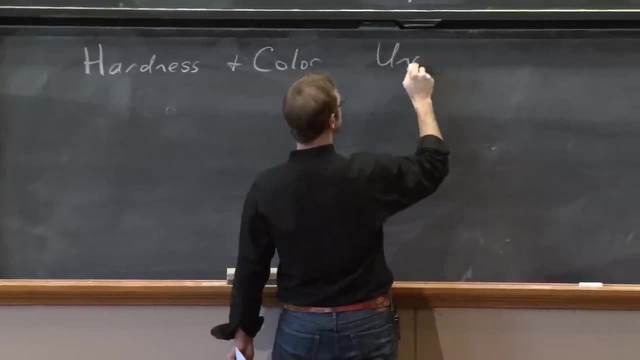 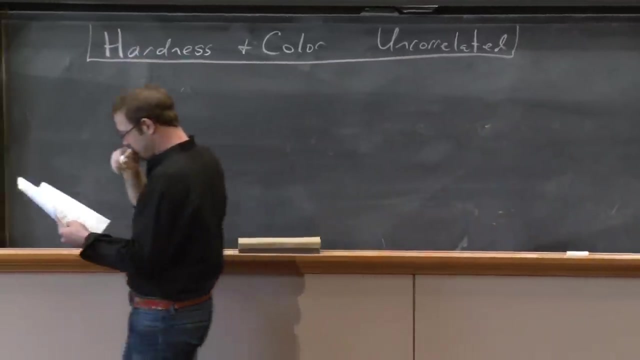 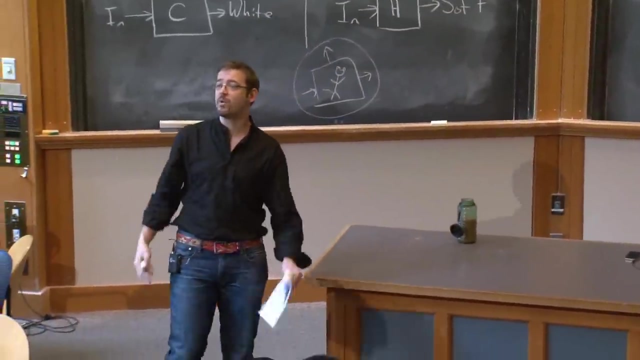 are uncorrelated. So H, hardness and color Are in this sense uncorrelated. So, using these properties of the color and hardness boxes, I want to run a few more experiments. I want to probe these properties of color and hardness. 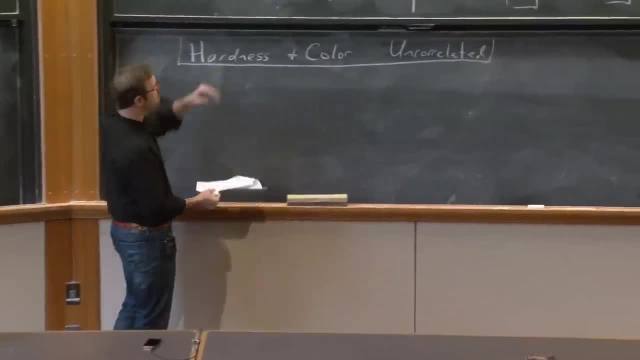 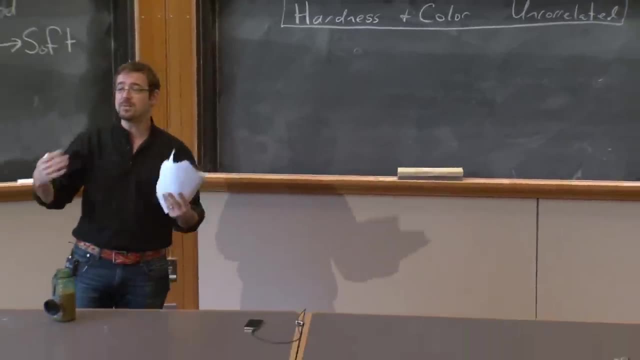 a little more And, in particular, knowing these results allows us to make predictions, to predict the results for a set of very simple experiments. Now, what we're going to do for the next bit is we're going to run some simple experiments And we're going to make predictions. 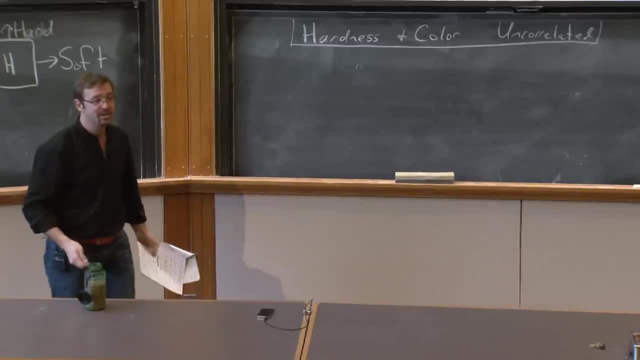 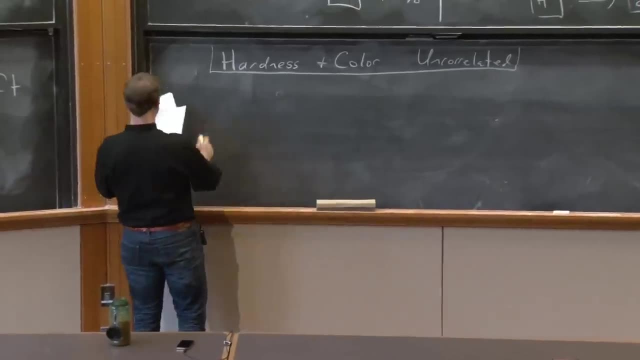 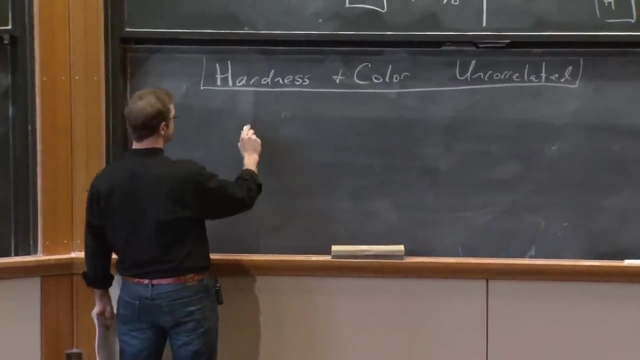 And then those simple experiments are going to lead us to more complicated experiments, But let's make sure we understand the simple ones first. So, for example, let's take this last experiment, color hardness, And let's add a color box. One more, monkey. 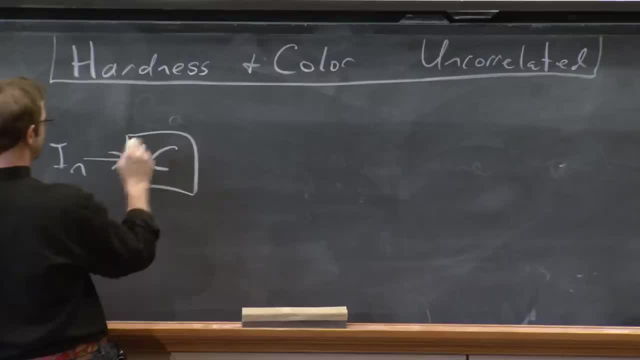 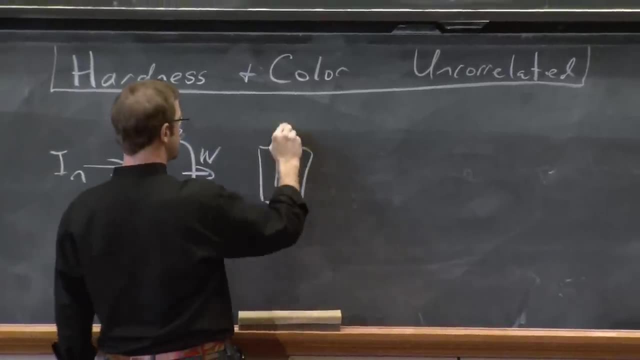 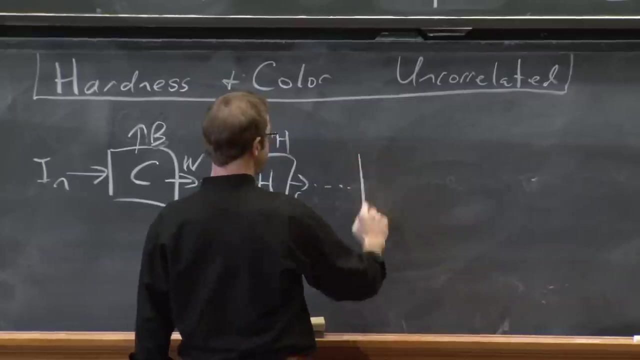 So color in, And we take those that come out the white aperture And we send them into a hardness box, Hard, soft. And we take those electrons which come out the soft aperture And now let's send these again into a color box. 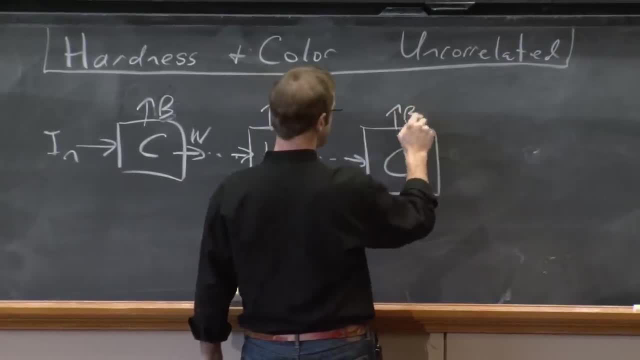 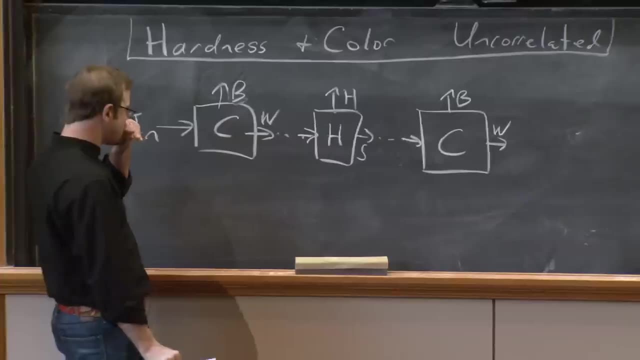 So it's easy to see what to predict: Black, white. So you can imagine a monkey inside this going aha. You look at it, You inspect: It comes out white. Here, you look at it and inspect It comes out soft. 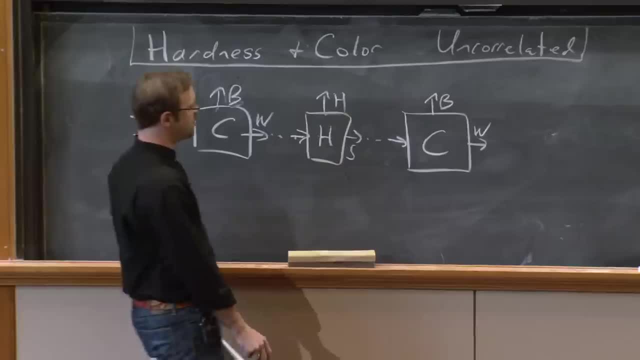 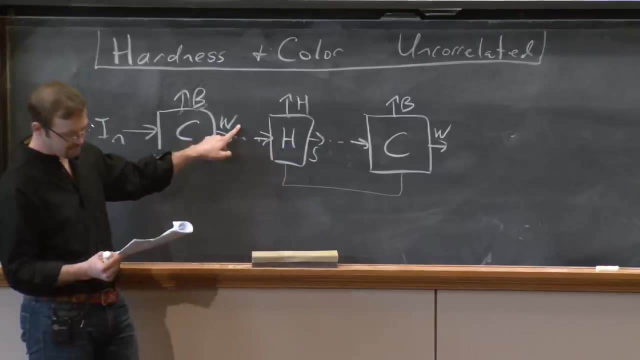 And you send it into the color box, And what do you expect to happen? Well, let's think about the logic here. Anything reaching the hardness box must have been measured to be white. And we just did the experiment that if you send a white, 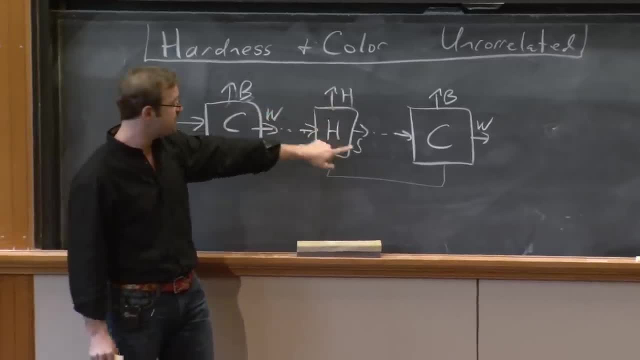 electron into a hardness box: 50% of the time it comes out, a hard aperture And 50% of the time it comes out, the soft aperture. So now we take that 50% of electrons that comes out, the soft aperture, which? 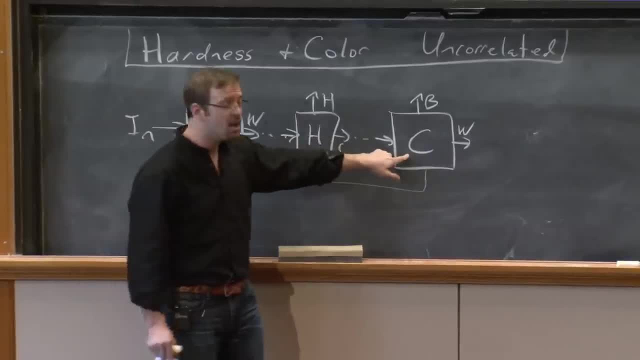 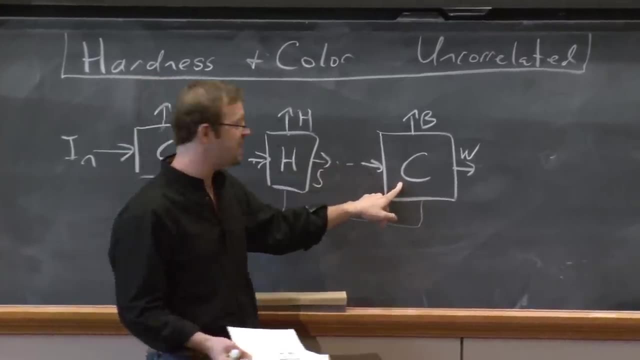 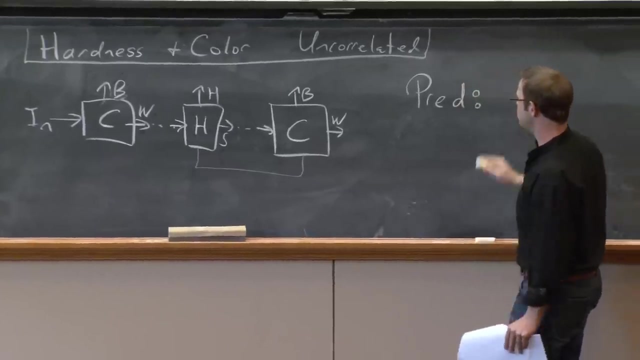 have previously been observed to be white and soft. And then we send them into a color box And what happens? They're white. Well, since color's repeatable, the natural expectation is that, of course, it comes out white. So our prediction, a natural prediction here, 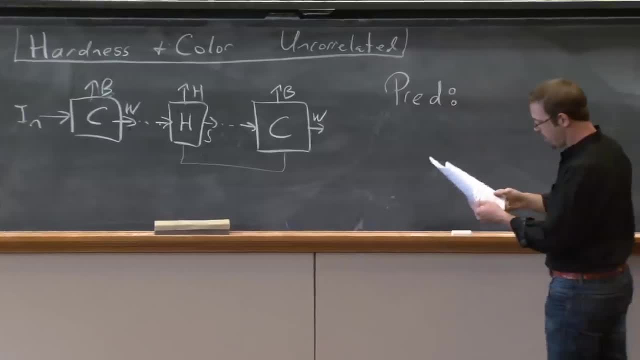 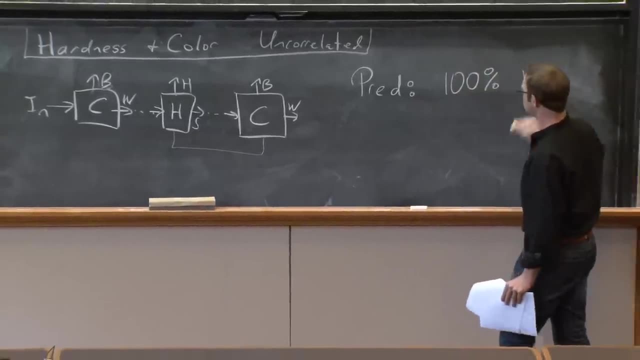 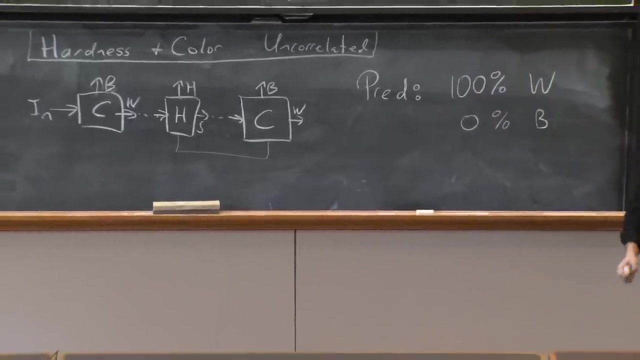 is that, of those electrons that are incident on this color box, 100% should come out white And 0% should come out black. Does that seem like a reasonable? Let's just make sure that we're all agreeing, So let's vote. 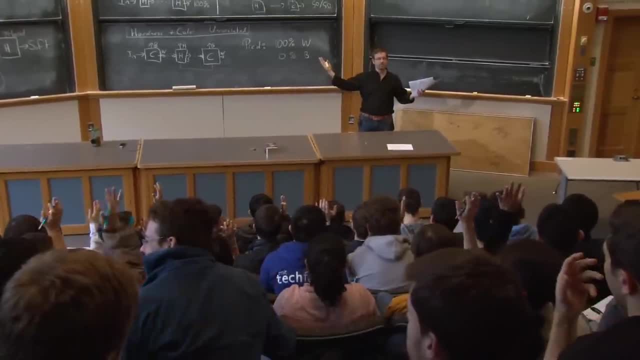 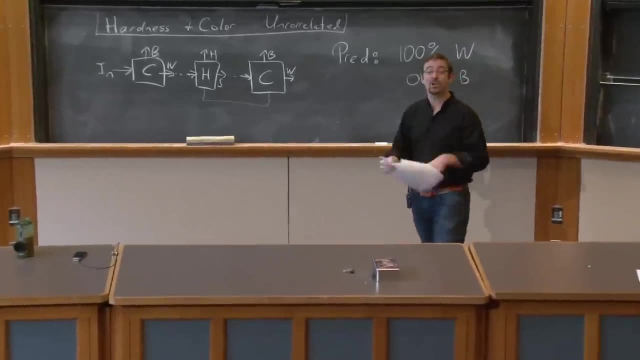 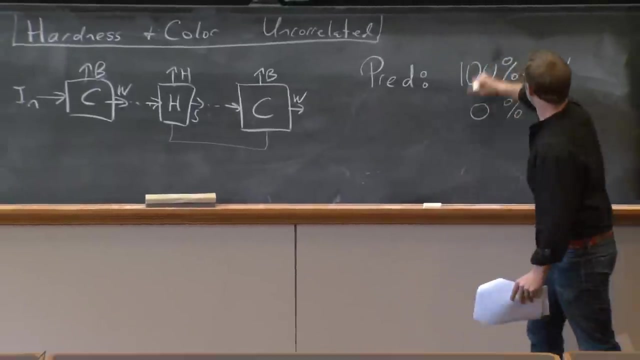 How many people think this is probably correct? OK good. How many people think this is probably wrong? OK good, That's reassuring, Except you're all wrong, right? In fact, what happens is half of these electrons exit white. 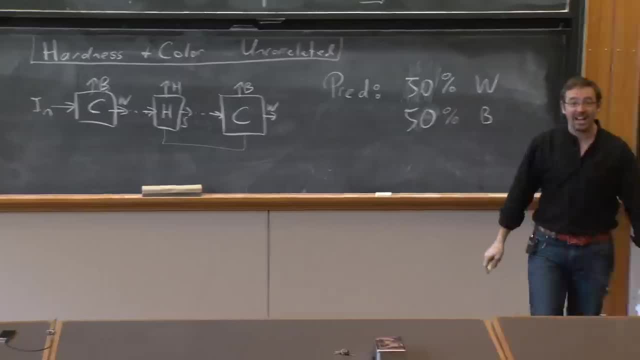 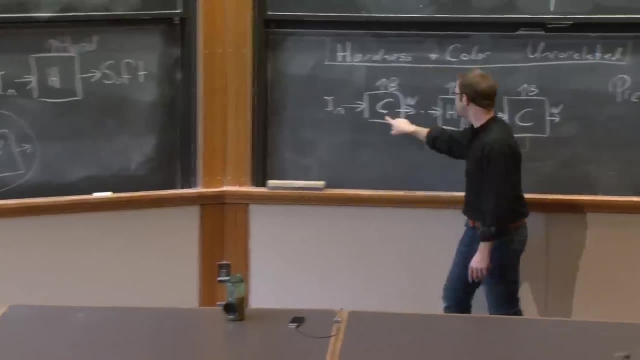 50% And 50% exit black. So let's think about what's going on here. This is really kind of troubling. We've said already that knowing the color doesn't predict the hardness, And yet this electron, which was previously 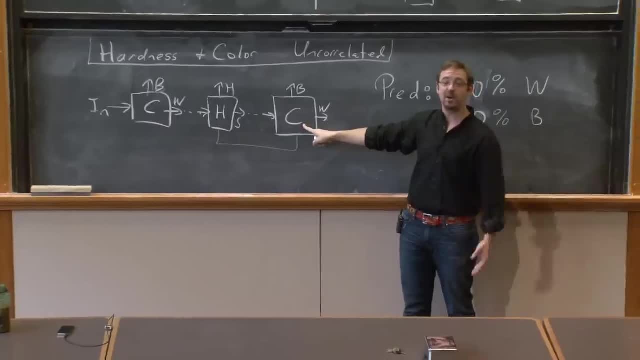 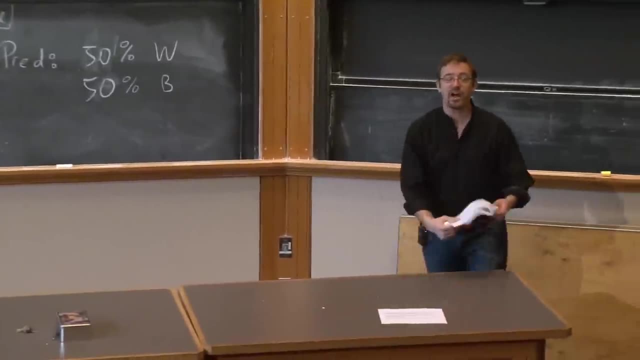 measured to be white. now, when subsequently measured, sometimes it comes out white, Sometimes it comes out black, 50%, 50% of the time. So that's surprising. What that tells you is: you can't think of electron as a little ball that has black and soft written on it. 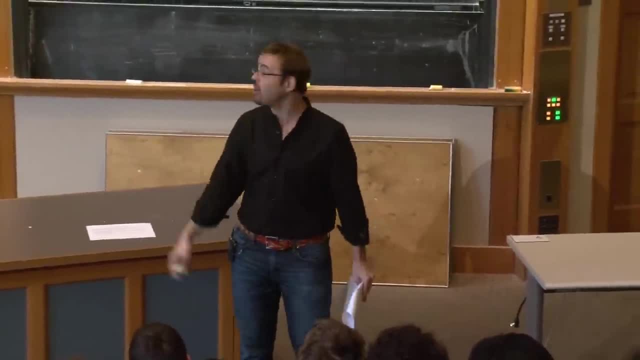 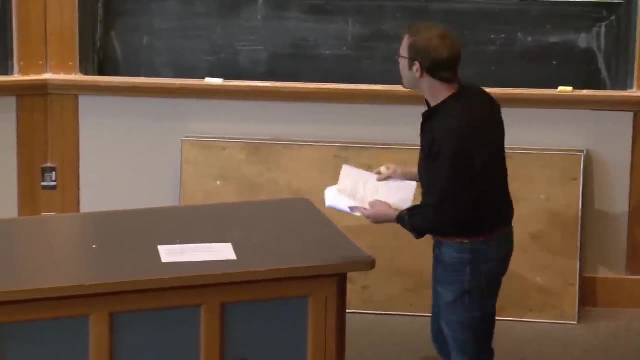 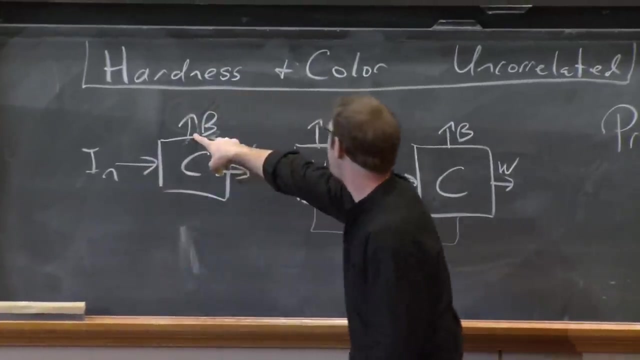 You can't, because apparently that black and soft isn't a persistent thing, Although it's persistent in the sense that once it's black, it stays black. So what's going on here? Now? I should emphasize that the same thing happens if I had changed this to taking the black electrons. 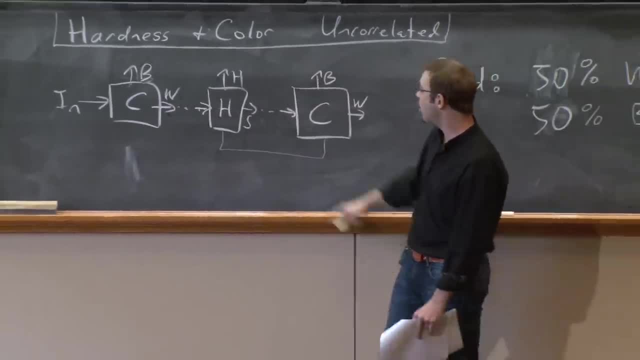 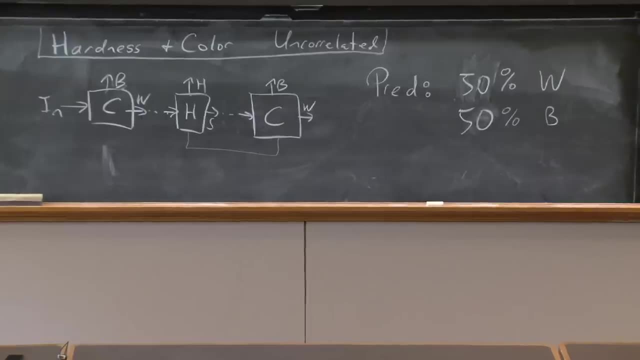 and throwing in a hardness and picking soft and then measure the color. Or if I had used the hard electrons, Any of those combinations, any of these ports would have given the same results: 50, 50. It is not persistent in this sense. 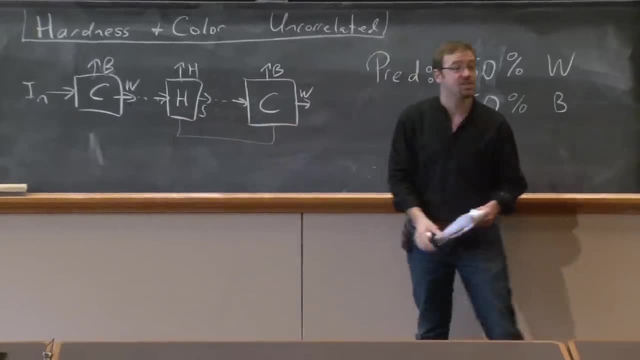 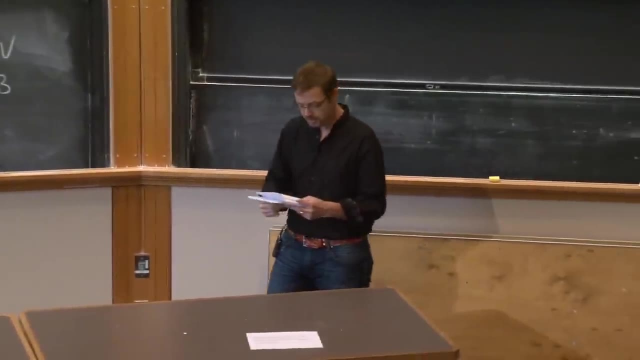 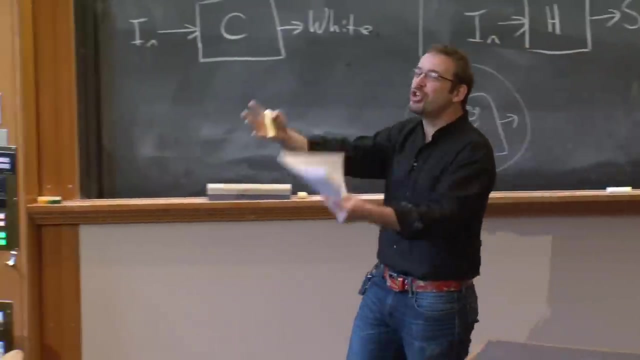 Apparently, the presence of the hardness box tampers with the color somehow, So it's not quite as trivial as that hyper-intelligent monkey. Something else is going on in here, So this is suspicious. So here's the first natural move. The first natural move is: oh look. 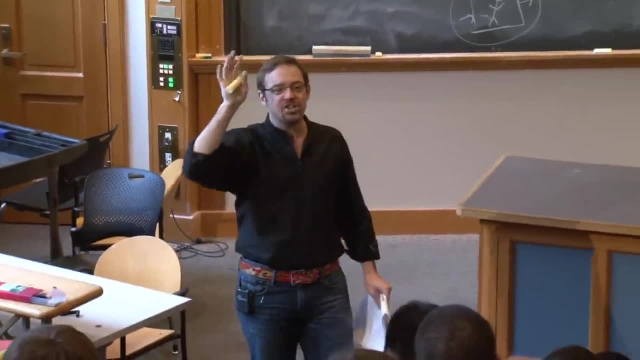 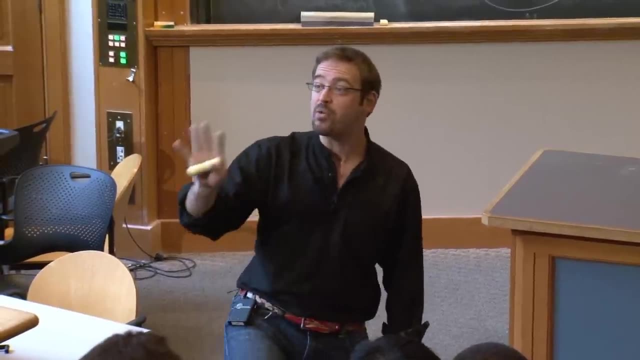 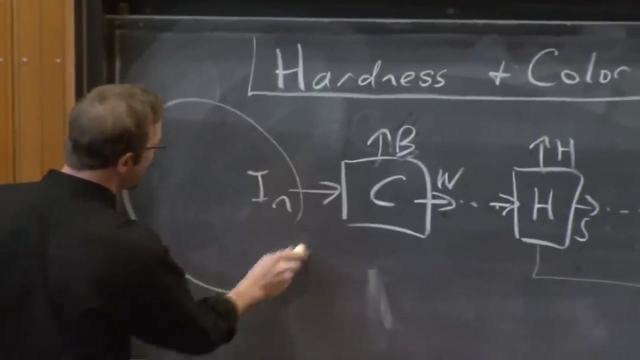 surely there's some additional property of the electron that we just haven't measured yet that determines whether it comes out the second color box, black or white. There's got to be some property that determines this, And so people have spent a tremendous amount of time. 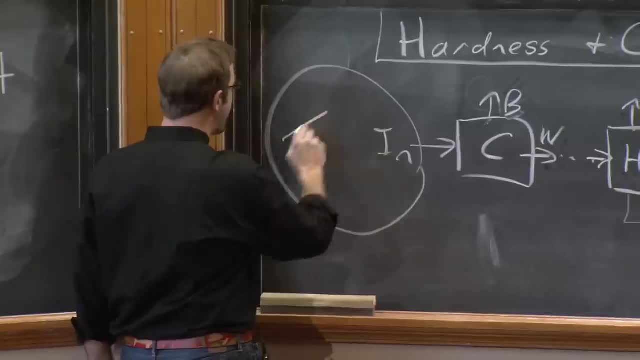 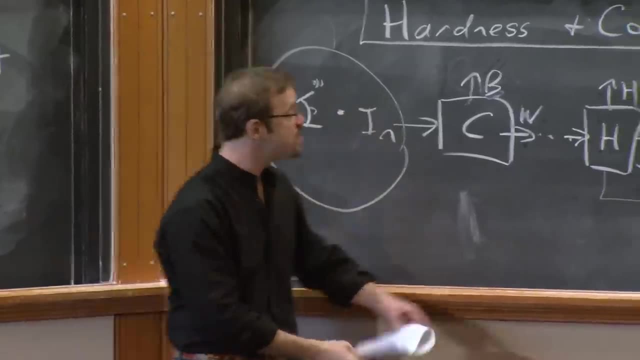 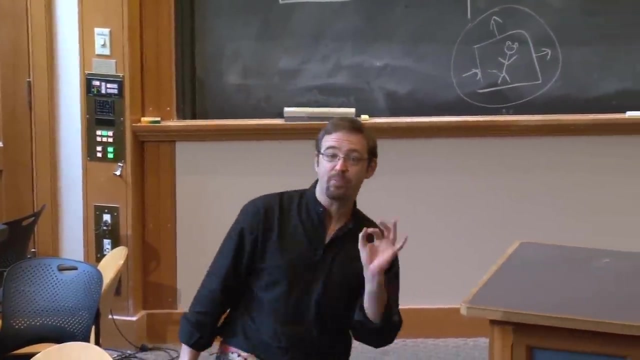 and energy, looking at these initial electrons and looking with great care to see whether there's any sort of feature of these incident electrons which determines which port they come out of. And the shocker is, no one's ever found such a property. No one has ever found a property which 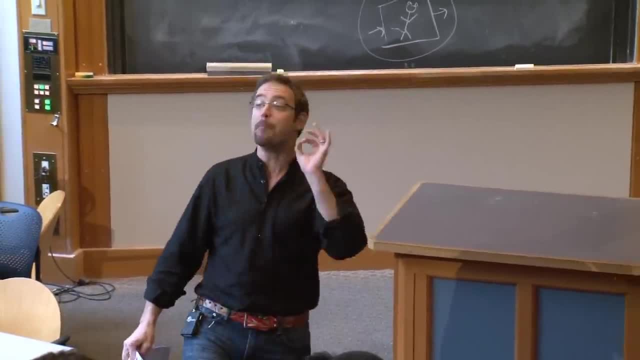 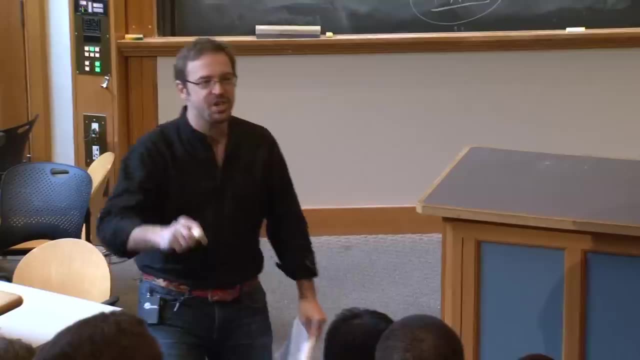 determines which port it comes out of. As far as we can tell, it is completely random. Those that flip and those that don't are indistinguishable at the beginning. And let me just emphasize- it's not like we're not looking. 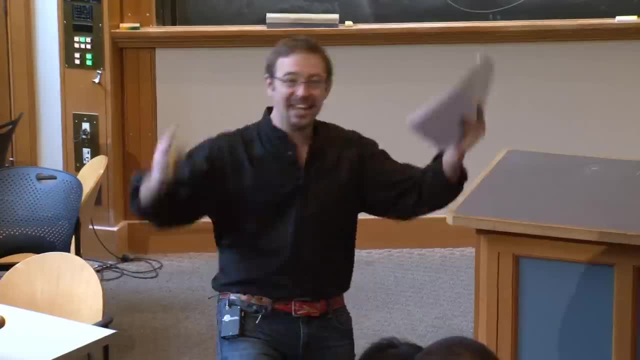 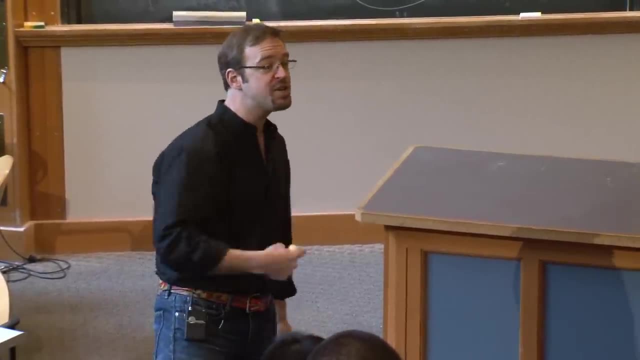 If anyone found such a property, fame, notoriety, subverting quantum mechanics, Nobel Prize. people have looked And there is none that anyone's been able to find And, as we'll see later on, using Bell's inequality we can more or less nail that such things don't exist. 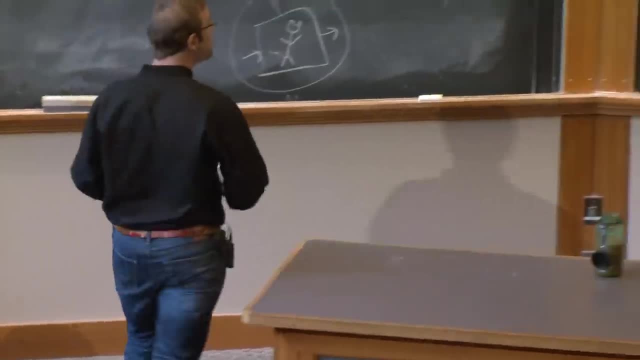 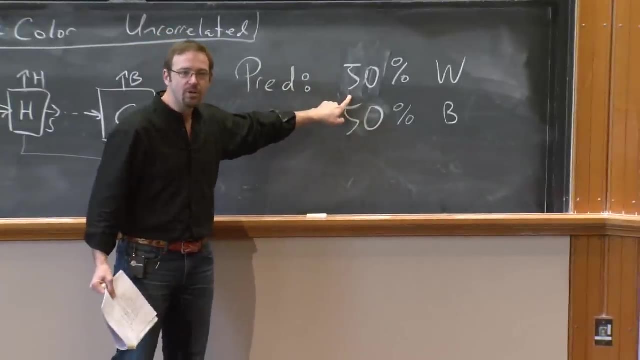 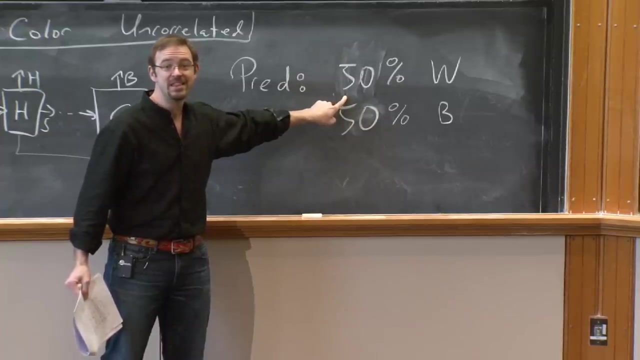 Such a feature doesn't exist, But this tells us something really disturbing. This tells us- And this is the first real shocker- that there is something intrinsically unpredictable, non-deterministic and random about physical processes that we observe in a laboratory. 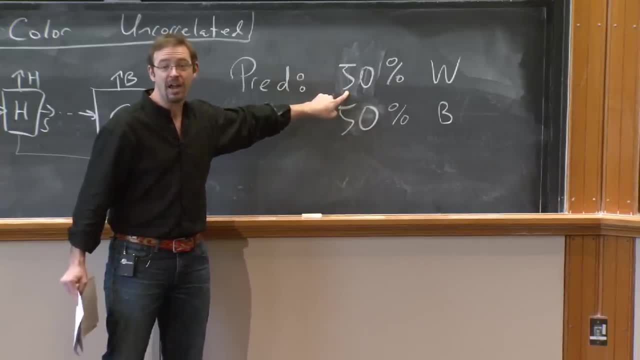 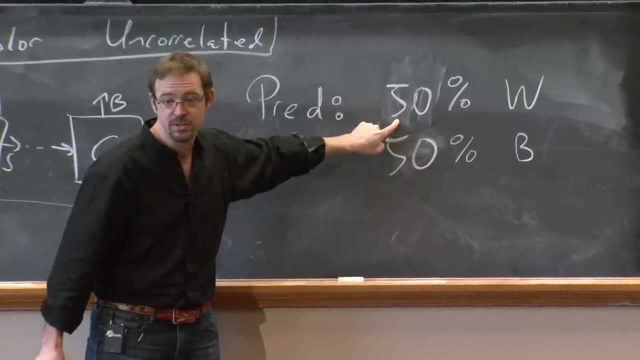 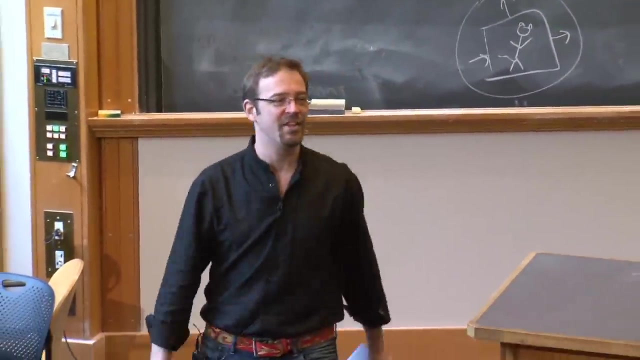 There's no way to determine a priori whether it will come out black or white from the second box. Probability in this experiment is forced upon us by observations. OK, Well, there's another way to come at this. You could say: look, you ran this experiment, that's fine. 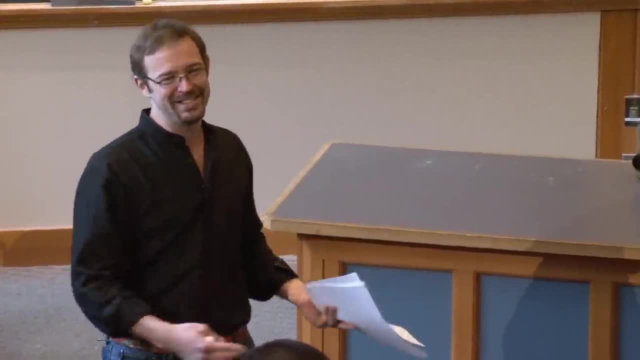 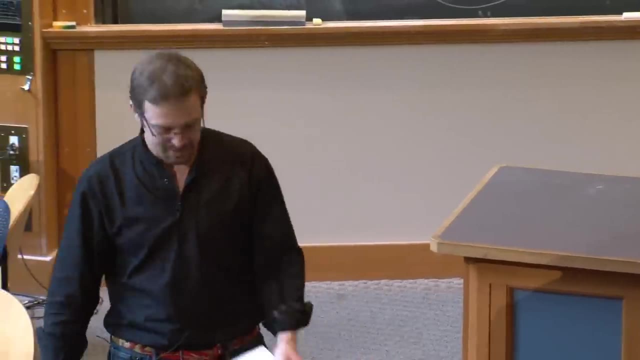 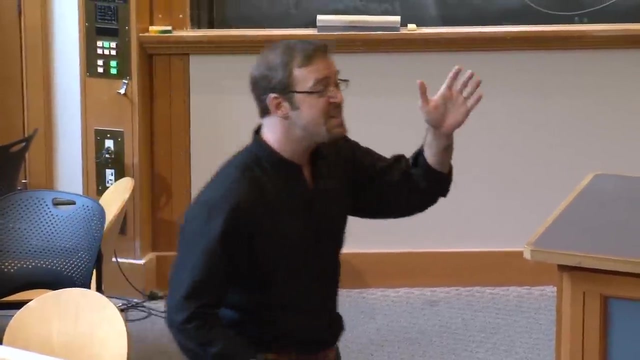 But look, I've met the guy who built these boxes And look, he's just some guy And he just didn't do a very good job. The boxes are just badly built. So here's the way to defeat that argument. No, we've built these things out of different materials. 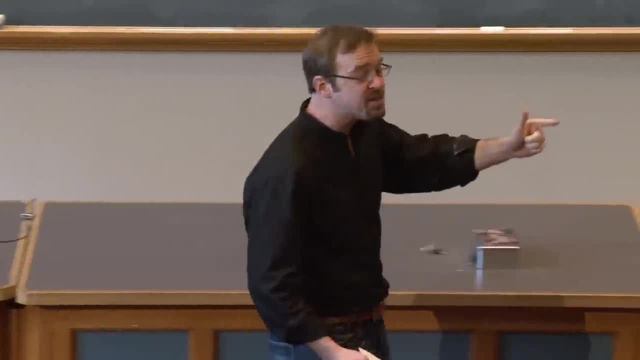 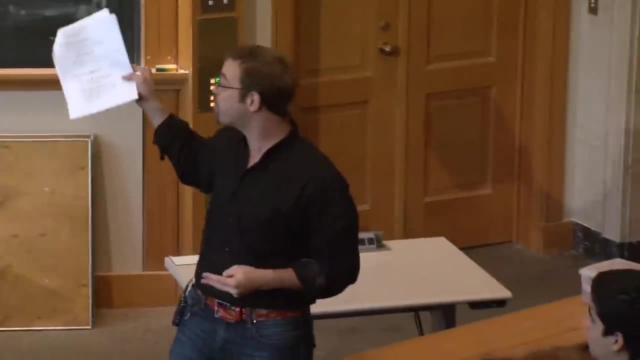 using different technologies: using electrons, using neutrons, using buckyballs, C60.. Seriously, It's been done, OK, We've done this experiment And this property does not change. It is persistent. And the thing that's most upsetting to me, 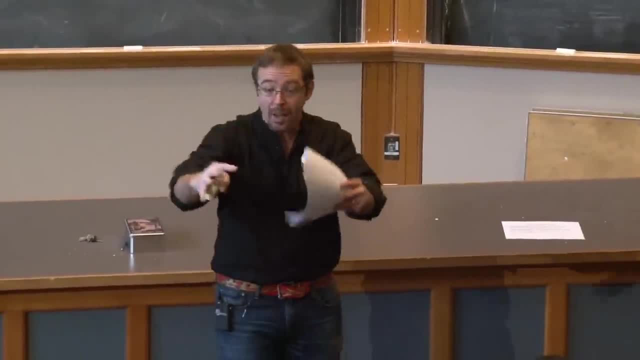 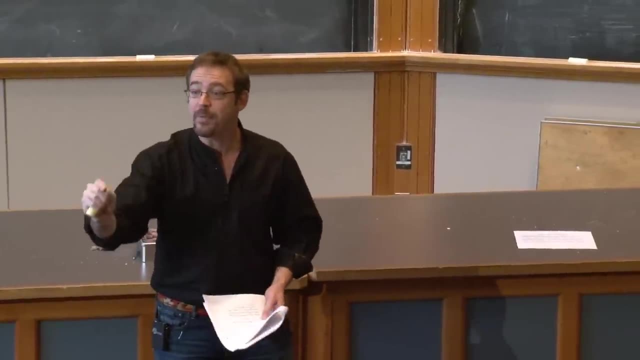 is that not only do we get the same results independent of what objects we use to run the experiment, we cannot change the probability away from 50-50 at all to within experimental tolerances We cannot change, no matter how we build the boxes. 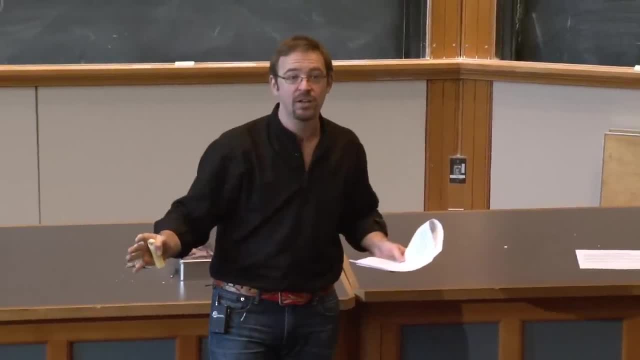 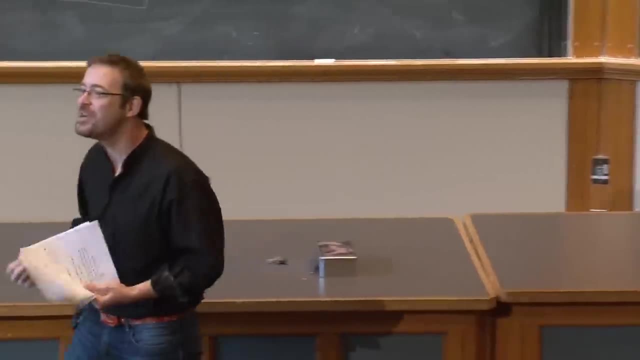 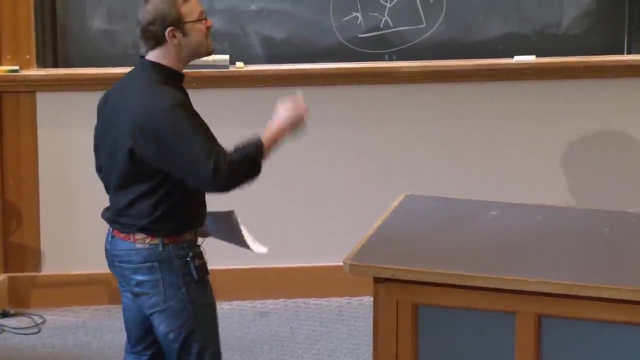 we cannot change the probability by part in 100.. OK, 50-50.. And to anyone who grew up with determinism from Newton, this should hurt, This should feel wrong, But it's a property of the real world And our job is going to be to deal with it. 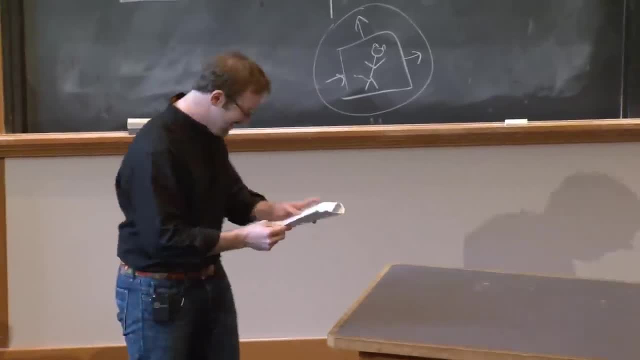 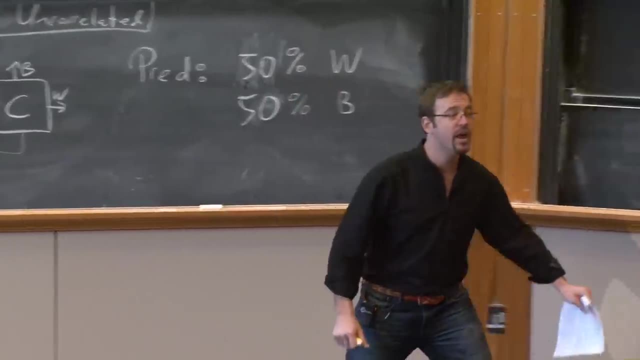 Rather, your job is going to be to deal with it, because I went through this already. So here's a curious consequence. Any questions before I cruise? OK, So here's a curious consequence. Here's a curious consequence of this series of experiments. 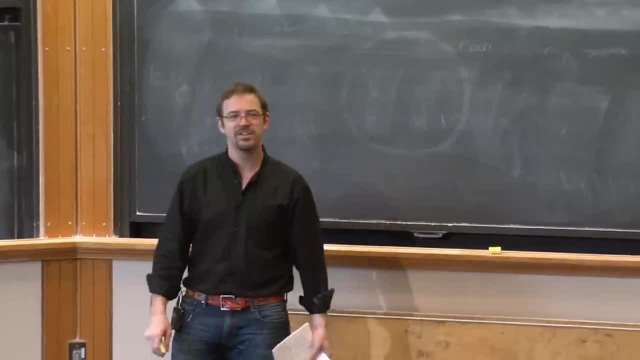 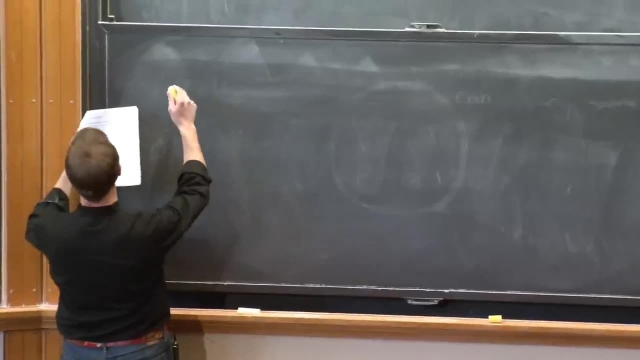 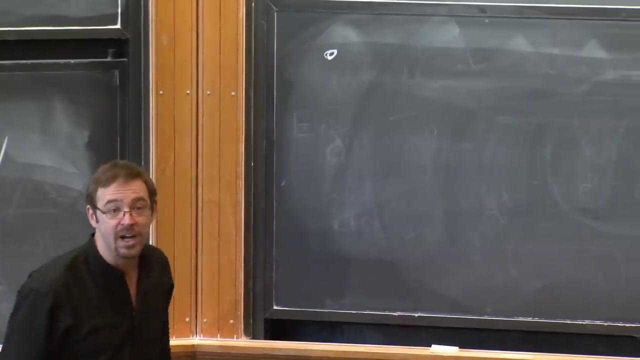 Here's something you can't do. Are you guys old enough where you can't do this on television? Oh Jesus, This is so sad. OK, So here's something you can't do. We cannot build. It is impossible to build a reliable color and hardness. 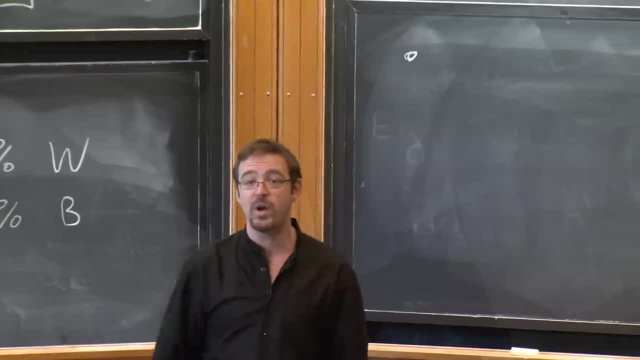 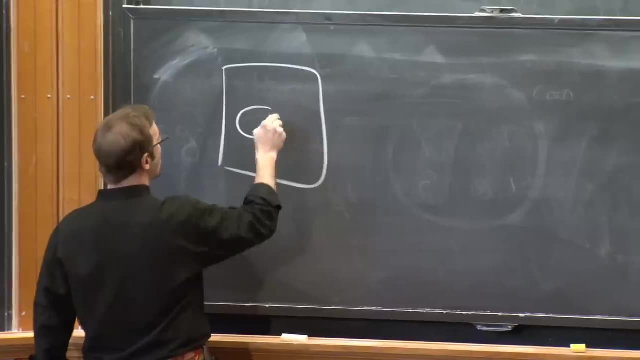 box. We've built a box that tells you what color it is. We've built a box that tells you what hardness it is, But you cannot build a meaningful box that tells you what color and hardness an electron is. So, in particular, what would this magical box be? 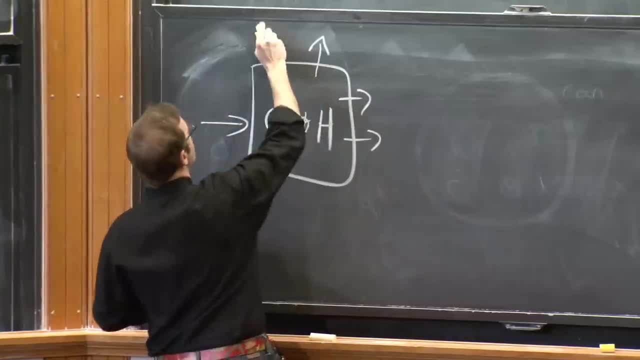 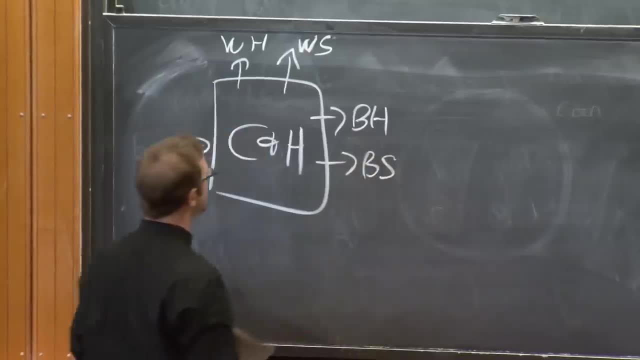 It would have four ports And its ports would say: well, one is white and hard, and one is white and soft, and one is black and hard and one is black and soft. So you can imagine how you might try to build a color and 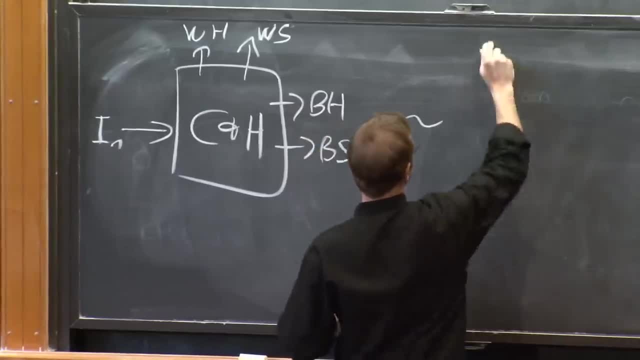 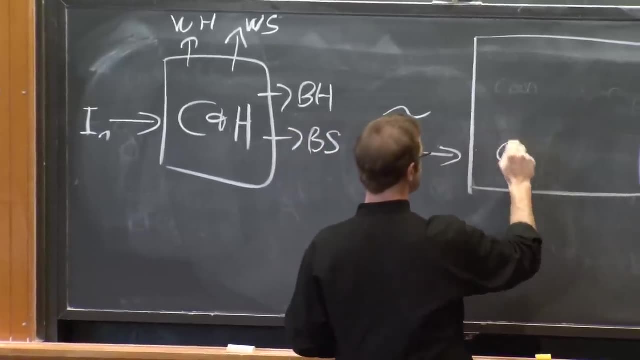 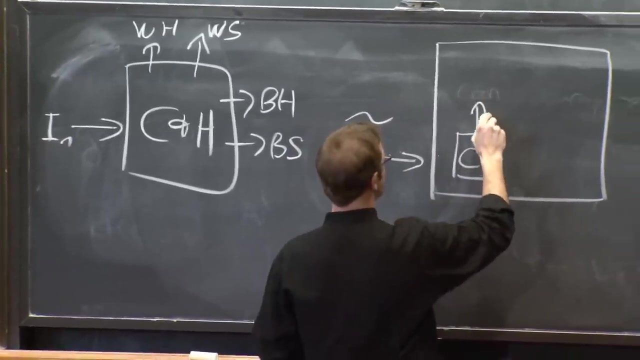 hardness box. So, for example, here's something that you might imagine: Take our incident electrons And first send them into a color box And take those white electrons, Oops, OK, I'll just draw it this way: Take the white electrons and send them into a hardness box. 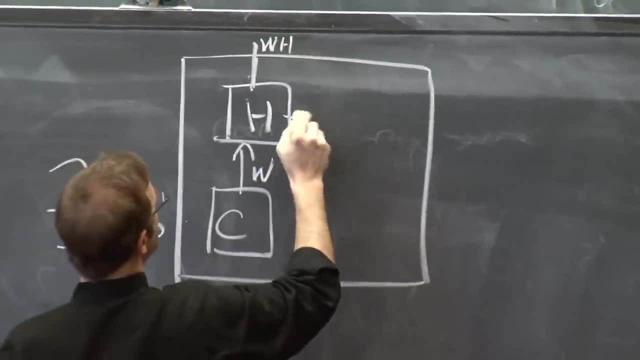 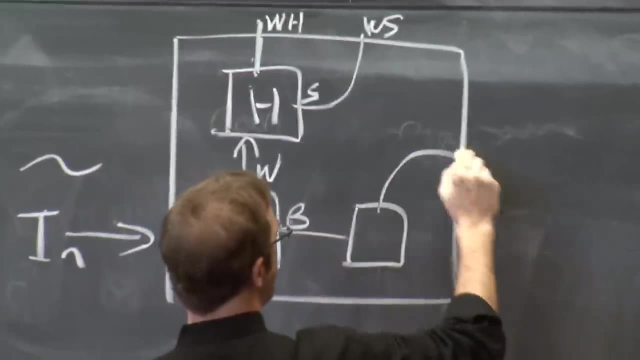 And take those electrons, And this is going to be white and hard, And this is going to be white and soft, And similarly, send these black electrons into a hardness box. And here's hard and black, And here's soft and black. 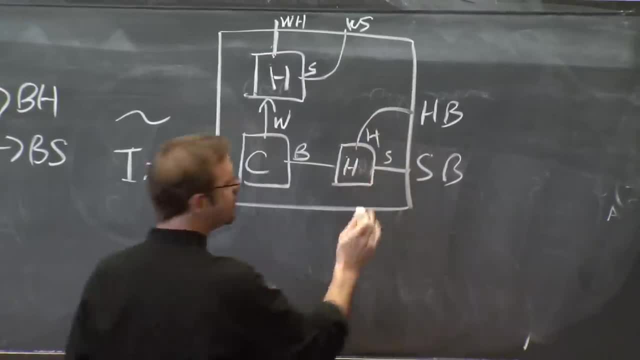 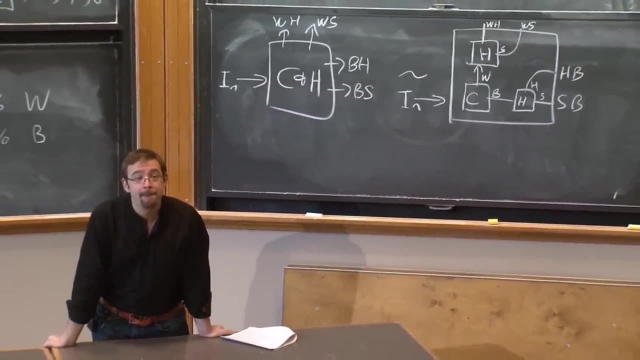 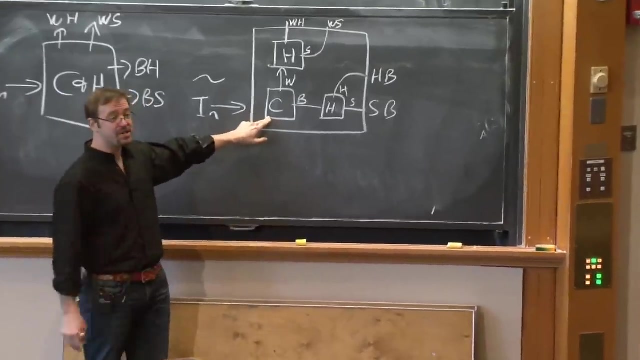 OK, Everyone cool with that. So this seems to do the thing I wanted. It measures both the hardness and the color. What's the problem with it? Yeah exactly, So the color is not persistent. So you tell me this is a soft and black electron, right? 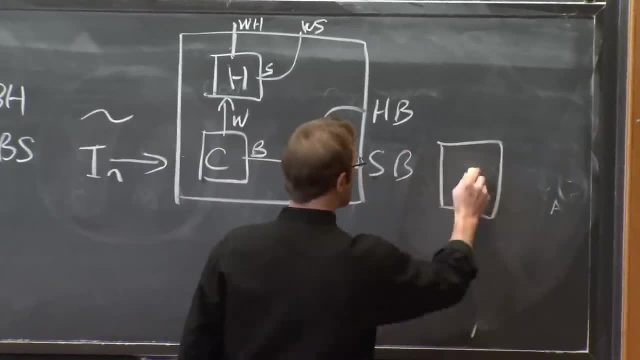 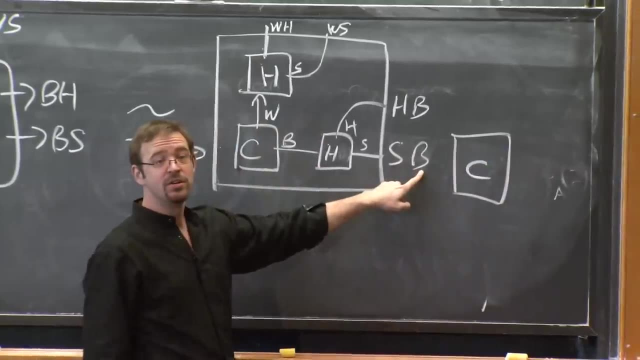 That's what you told me. Here's the box. But if I put a color box here, that's the experiment we just ran. And what happens? Does this come out black? No, this is a crappy source of black electrons. It's 50-50 black and white. 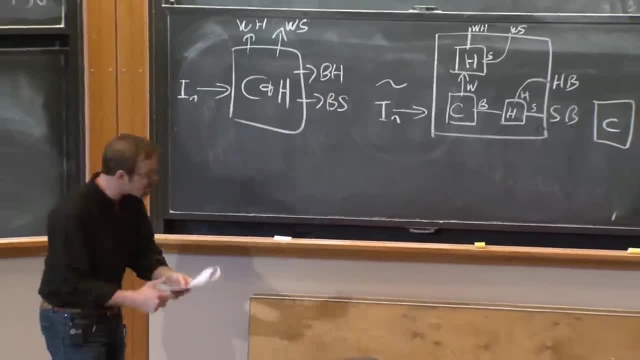 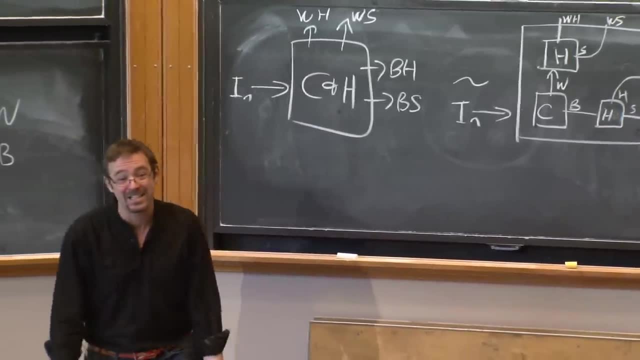 So this box can't be built, And the reason- and I want to emphasize this- the reason we cannot build this box is not because our experiments are crude And it's not because I can't build things, although that's true, I was banned from a lab one day after joining it, actually, 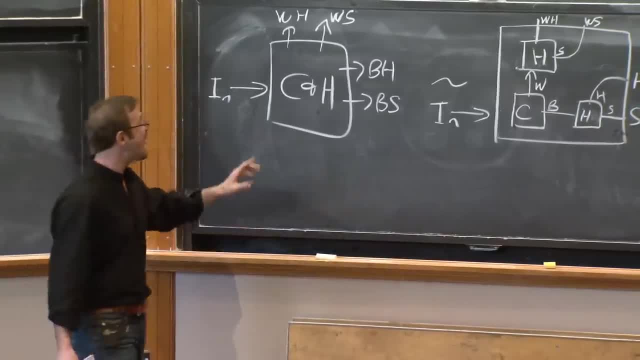 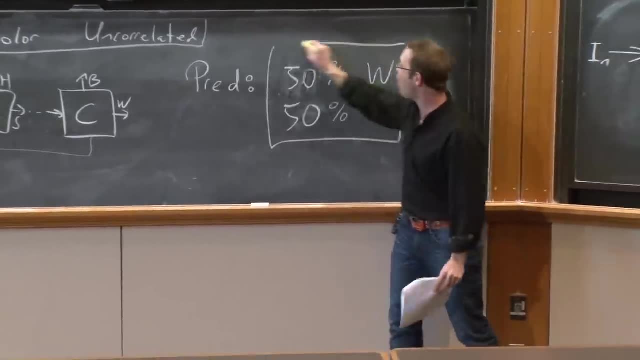 So I really can't build, But other people can. OK, And that's not why We can't, because of something much more fundamental, something deeper, something in principle, which is encoded in this awesome experiment. OK, This can't be done. 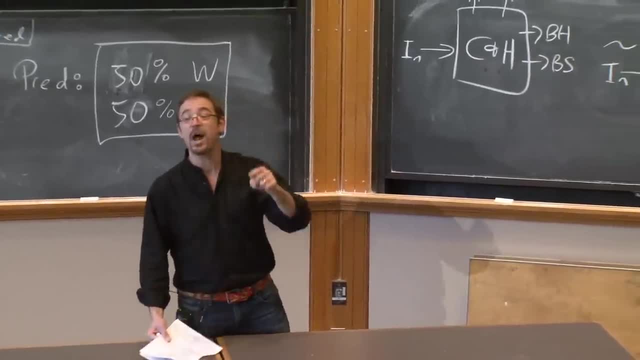 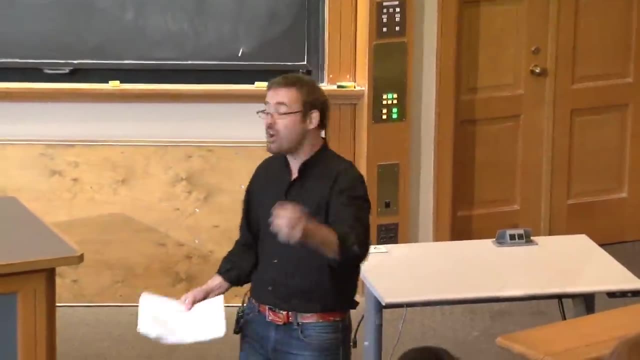 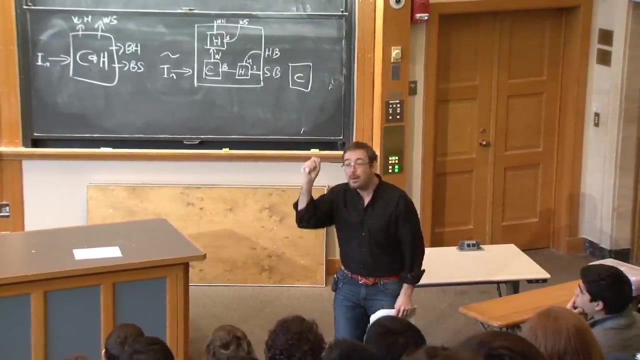 It does not mean anything. as a consequence, It does not mean anything to say this: electron is white and hard, Because if you tell me it's white and hard and I measure white, well I know that if it's hard it's going to come out 50-50.. 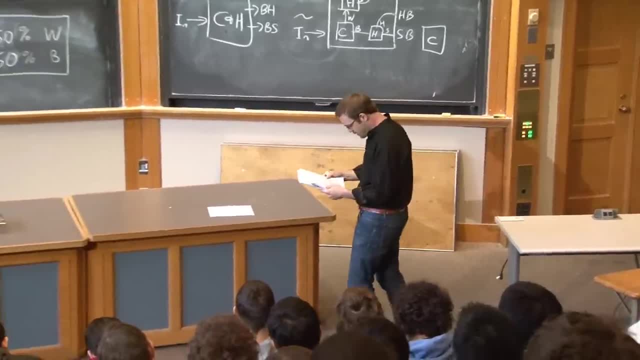 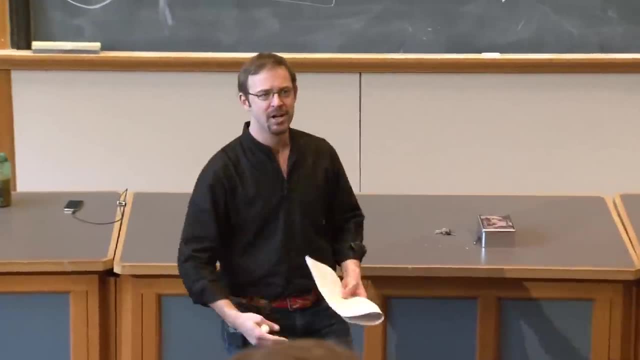 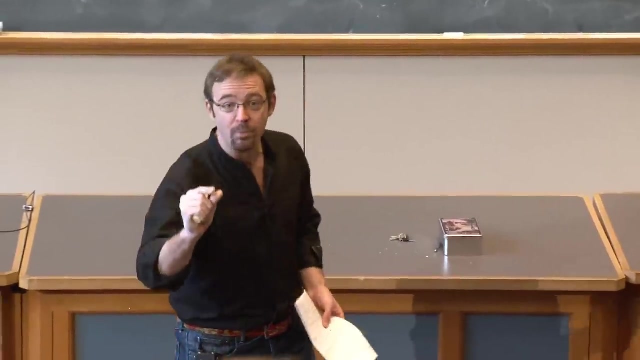 It does not mean anything. So this is an important idea. This is an idea which is enshrined in physics with a term which comes with capital letters: the uncertainty principle. And the uncertainty principle says basically that: look, there are some observable, measurable properties. 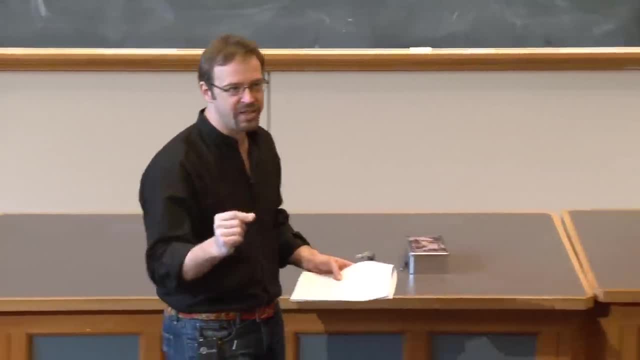 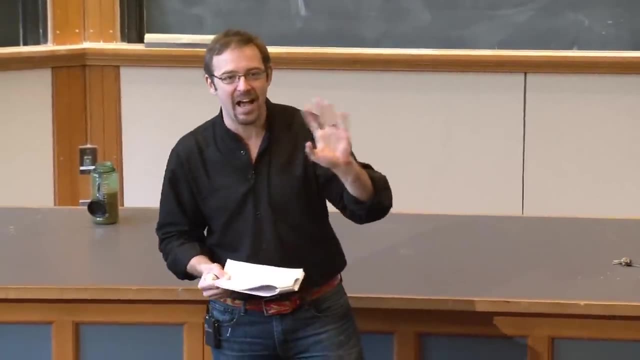 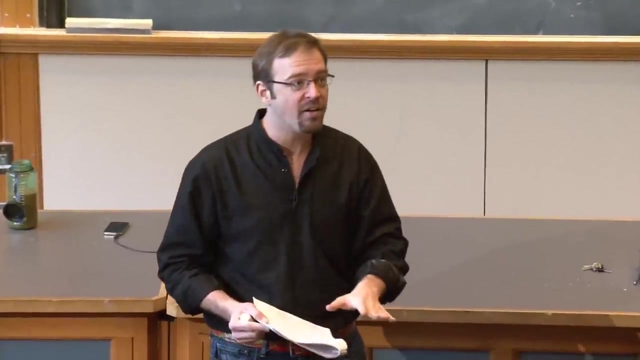 of a system which are incompatible with each other in precisely this way. Incompatible with each other in the sense that, not that you can't know, because you can't know whether it's hard and soft simultaneously, Deeper, it is not hard and white simultaneously. 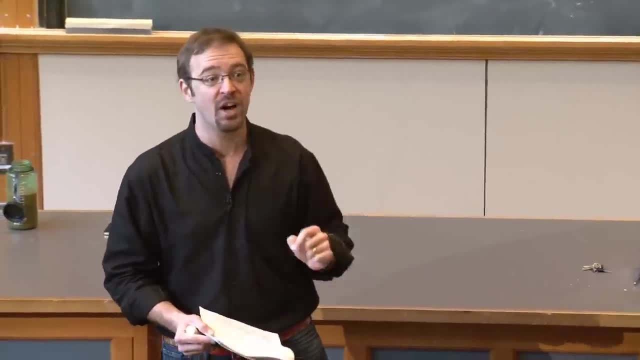 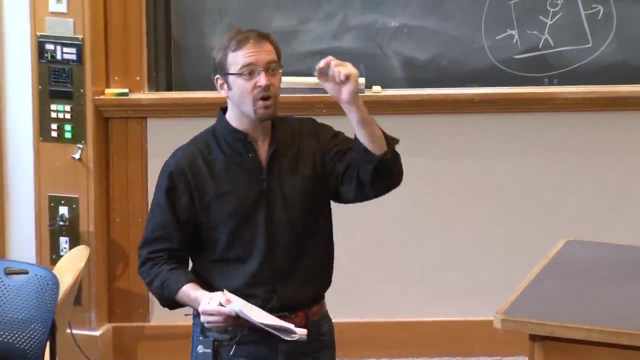 It cannot be. It does not mean anything to say. it is hard and white simultaneously. That is uncertainty. And again, uncertainty is an idea we are going to come back to over and over in the class, But every time you think about it, 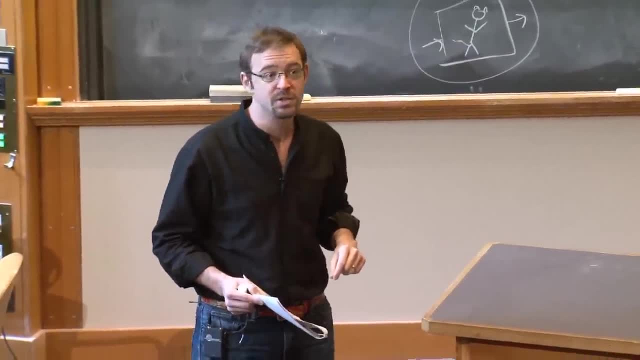 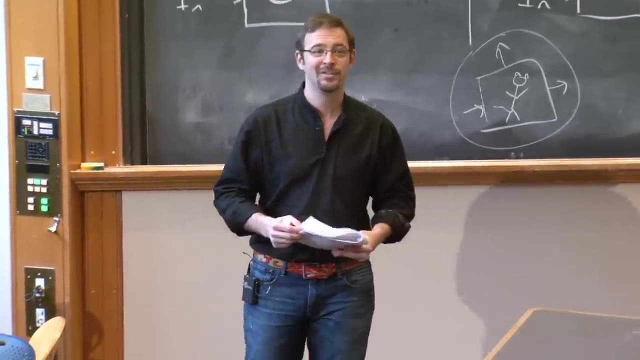 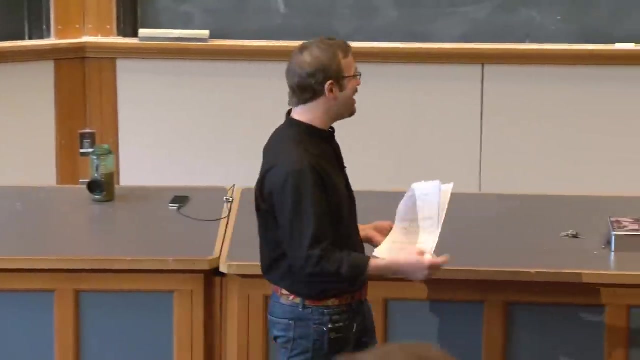 this should be the first place you start for the next few weeks. Yeah Questions, No questions, OK. so at this point it's really tempting to think: yeah, OK, this is just about the hardness and the color of electrons. 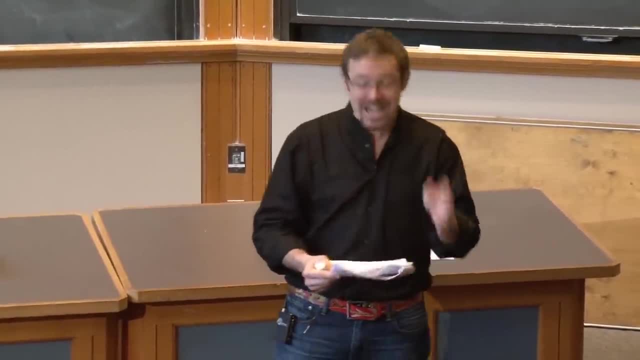 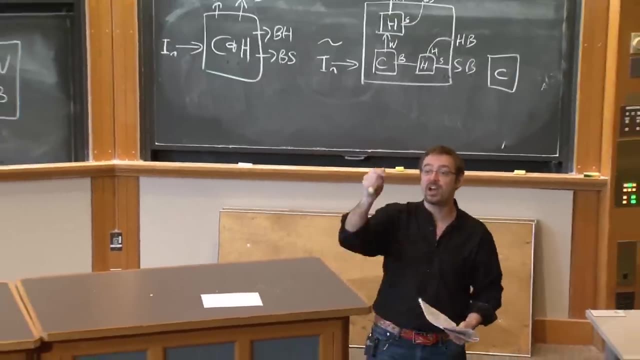 It's just a weird thing about electrons. It's not a weird thing about the rest of the world. The rest of the world is completely reasonable And no, that's absolutely wrong. Every object in the world has the same properties. If you take buckyballs and you send them, 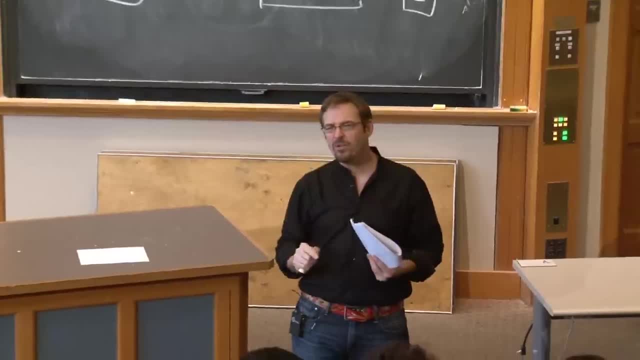 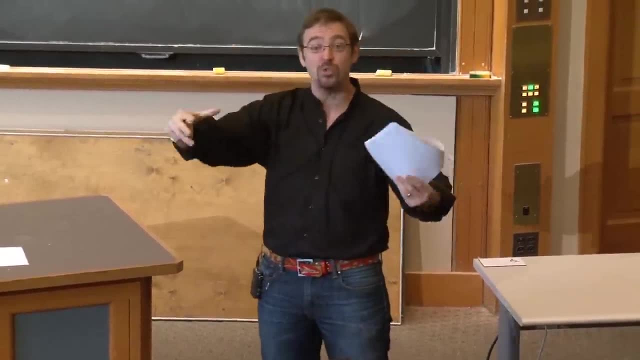 through the analogous experiment and I will show you the data. I think tomorrow, but soon I will show you the data. when you take buckyballs and run it through a similar experiment, you get the same effect. Now, buckyballs are huge, right? 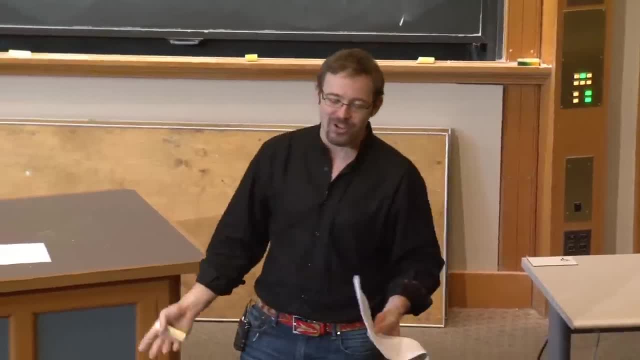 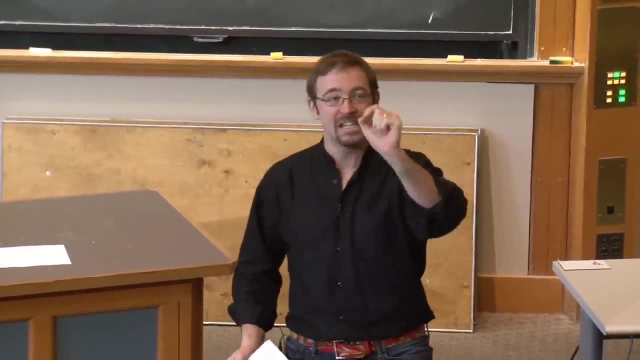 60 carbon atoms. But OK, at that point you're saying, dude, come on huge 60 carbon atoms. So there is a pendulum, depending on how you define building in this building. OK, OK, OK. 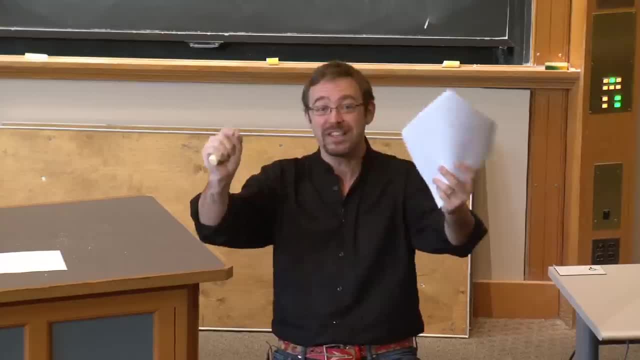 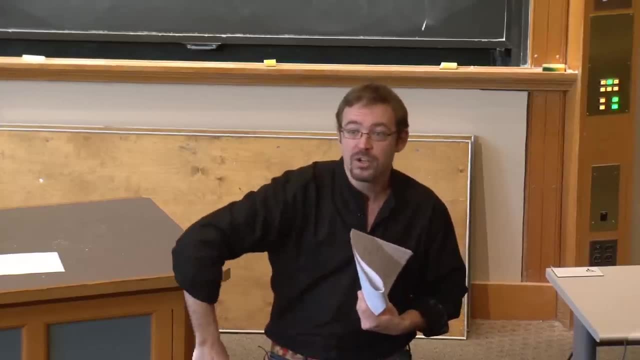 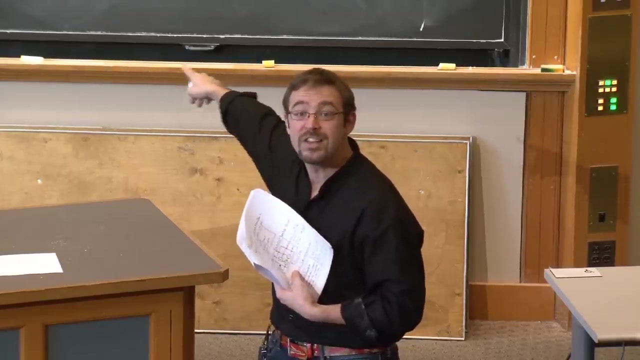 A pendulum which is used in principle, which is used to improve detectors to detect gravitational waves. There's a pendulum with a- I think it's 20 kilo mirror And that pendulum exhibits the same sort of effects here. 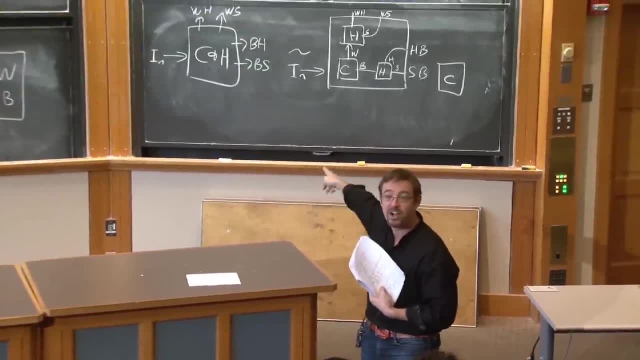 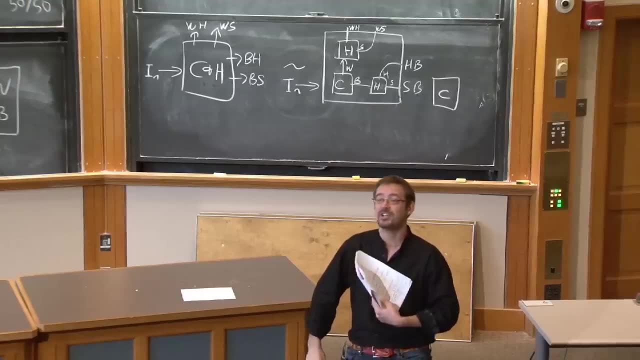 We can see these quantum mechanical effects in those mirrors. And this is in breathtakingly awesome experiments done by Anergis Malvalavala, whose name I can never pronounce, but who is totally awesome. She's an amazing physicist And she can get these kind of quantum effects. 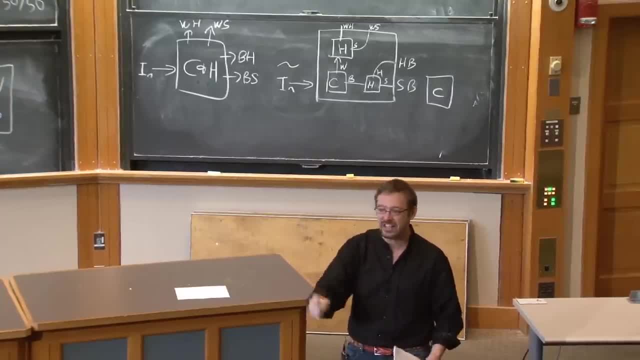 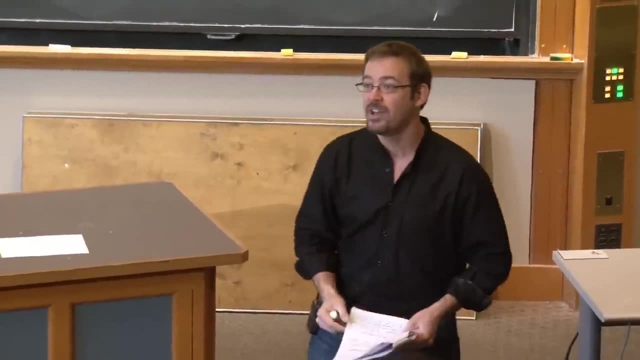 out of a 20 kilo mirror. So before you say something silly like, oh, it's just electrons, it's 20 kilo mirrors And if I could put you on a pendulum, that accurate it would be you OK. 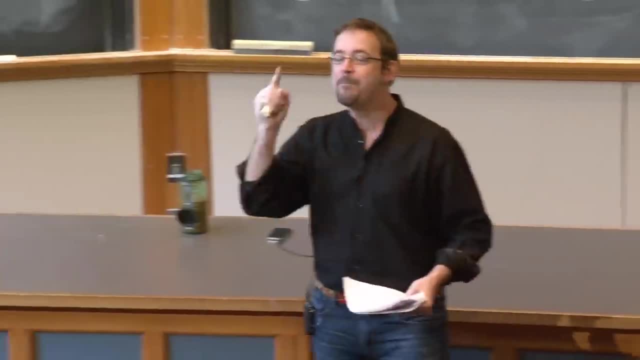 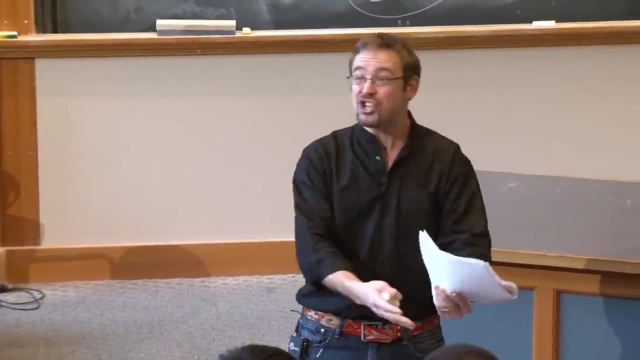 These are properties of everything around you. The miracle is not that electrons behave oddly. The miracle is that when you take 10 to the 27 electrons, they behave like cheese. That's the miracle. OK, This is the underlying correct thing. 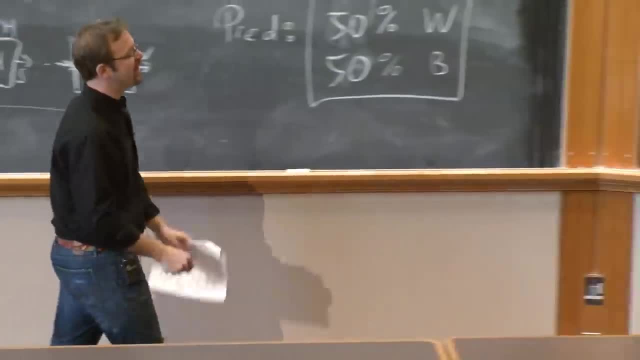 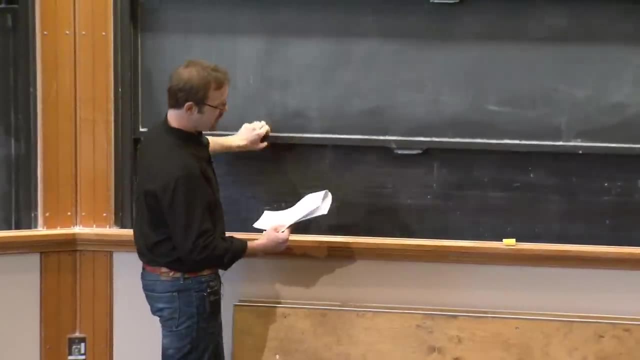 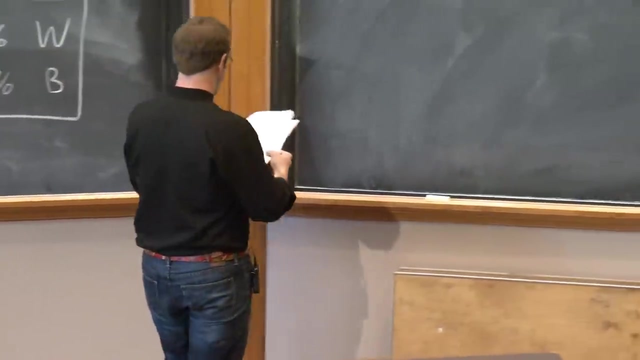 OK. So this is so far, so good, But let's go deeper, Let's push it. And to push it, I want to design for you a slightly more elaborate apparatus, Slightly more elaborate experimental apparatus, And for this I want you to consider the following device: 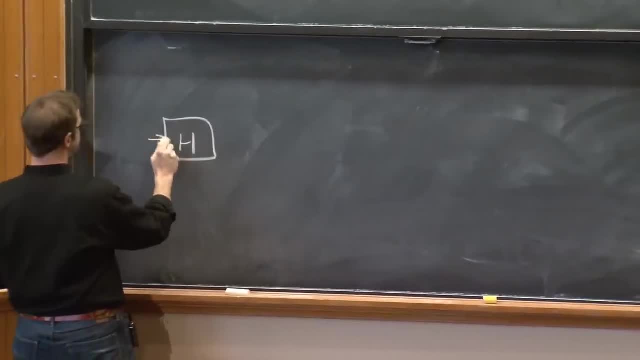 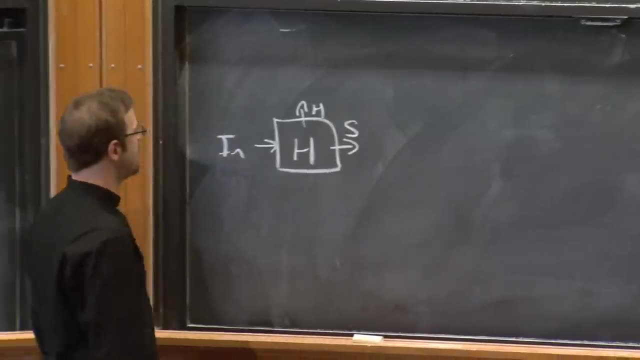 I'm going to need to introduce a couple of new features for you. Here's a hardness box And it has an import. And the hardness box, The hardness box, has a hard aperture And it has a soft aperture. And now, in addition to this hardness box, 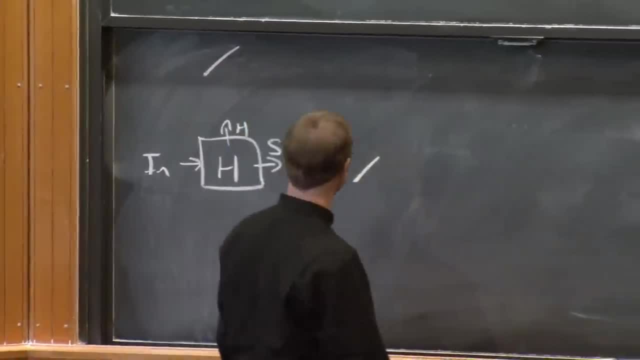 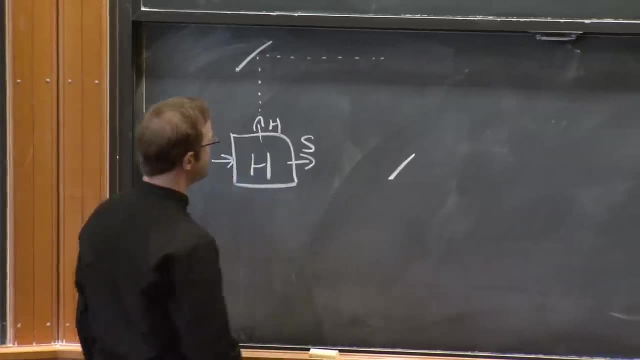 I'm going to introduce two elements. First, mirrors: OK, And what these mirrors do is they take the incident electrons, and nothing else. They change the direction of motion. OK, Change the direction of motion, And here's what I mean by doing nothing else. 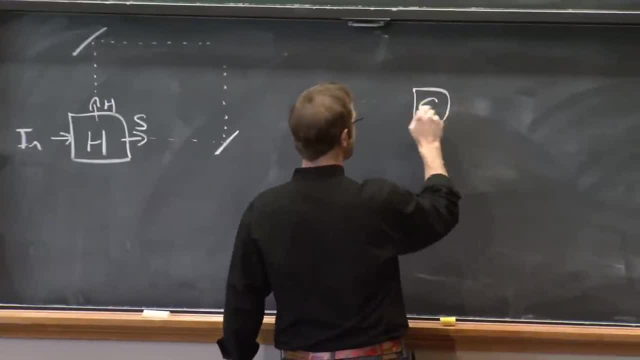 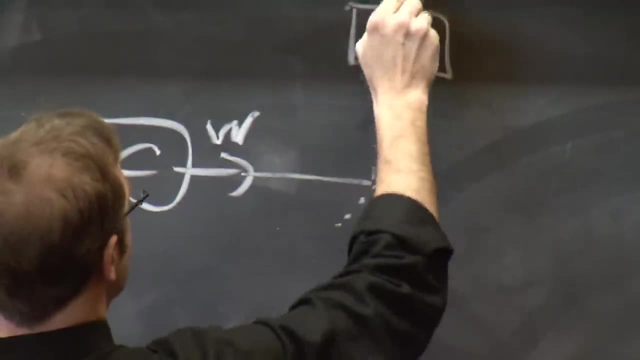 If I take one of these mirrors and I take, for example, a color box and I take the white electrons that come out and I bounce it off the mirror and then I send these into a color box, Then they come out white 100% of the time. 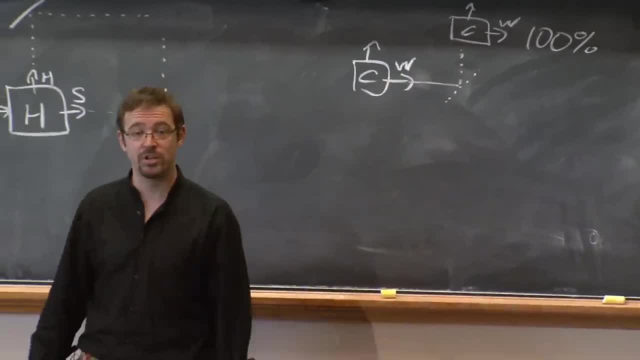 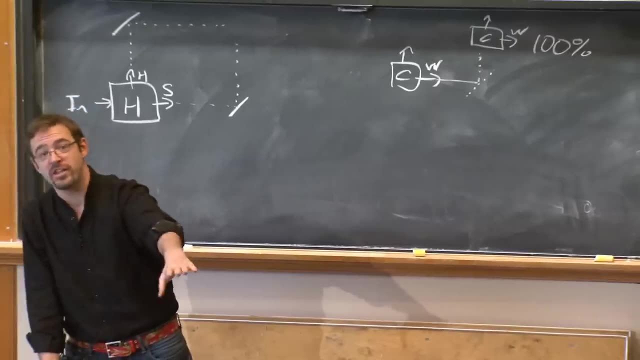 It does not change the observable color. All it does is change the direction. Similarly with the hardness box, It doesn't change the hardness, It just changes the direction of motion. And every experiment we've ever done on these guys changes in no way whatsoever the color or the hardness. 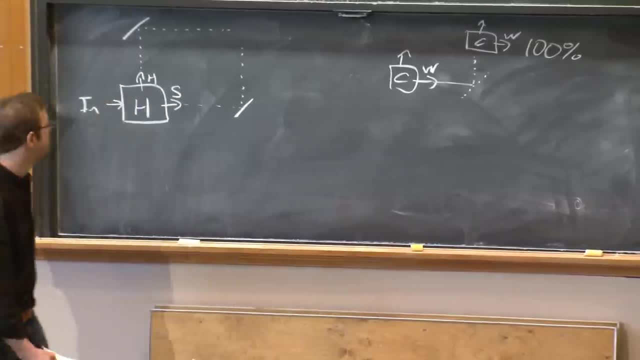 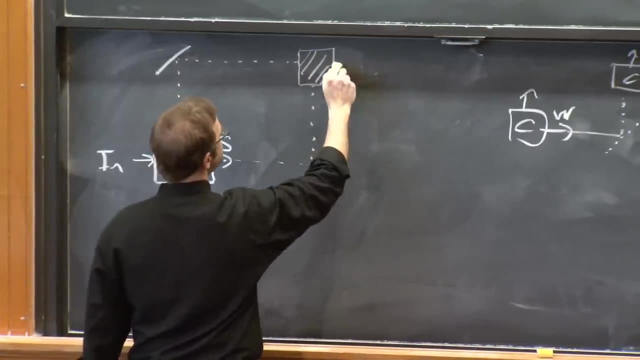 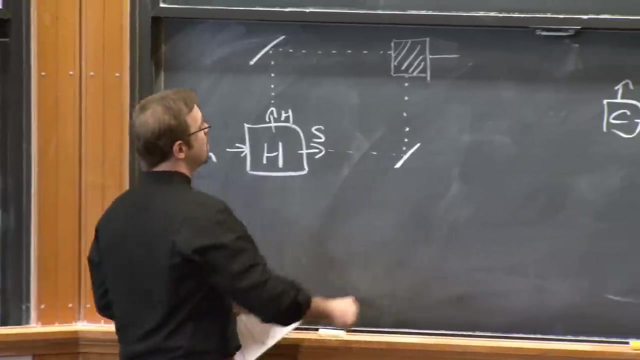 by subsequent measurements Just changes the direction of motion. And then I'm going to add another thing, Another mirror. It's actually a slightly fancy set of mirrors. All they do is they join these beams together into a single beam, And again, this doesn't change the color. 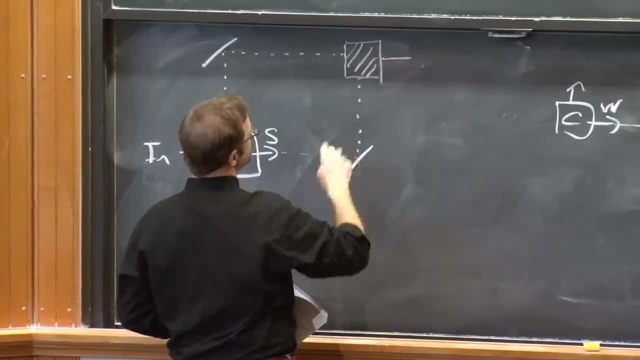 You send in a white electron, you get out And you measure the color. on the other side, you get a white electron. You send in a black electron from here and you measure the color. you get a black electron again out. Cool, 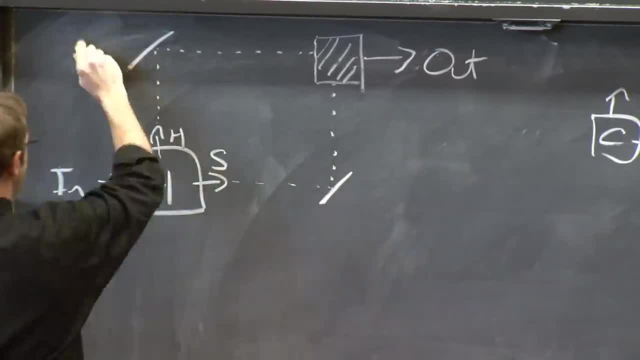 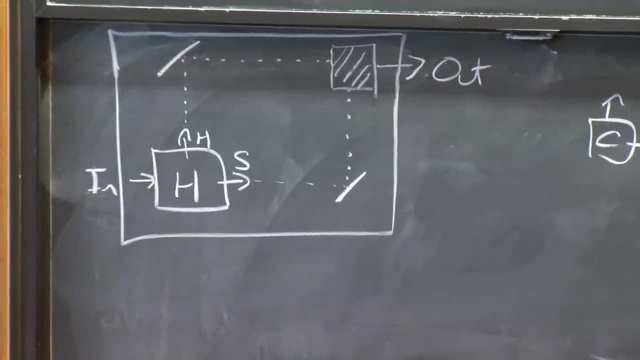 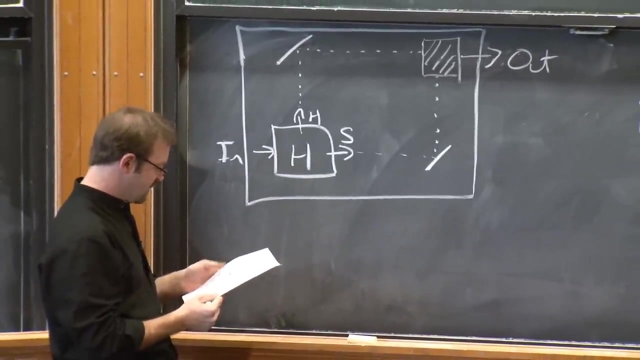 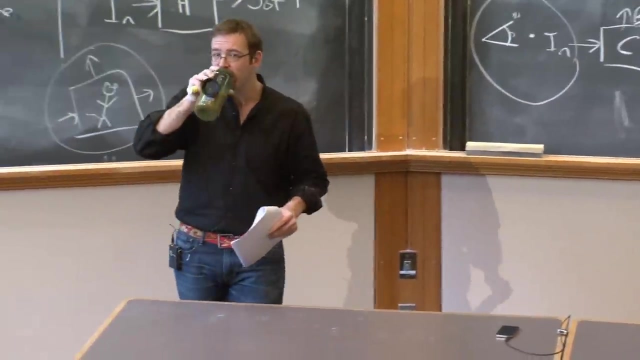 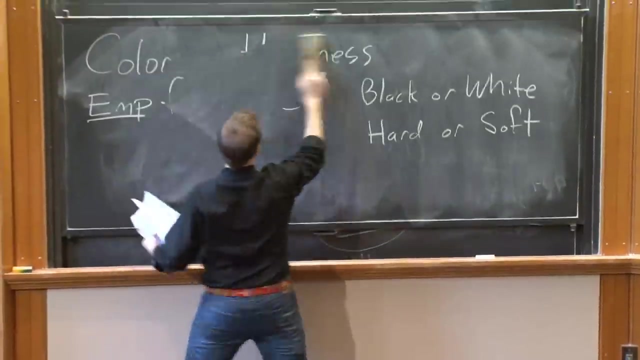 So here's my apparatus And I'm going to put this inside a big box And I want to run some experiments with this apparatus. Everyone cool with the basic design? Any questions before I cruise on? This part is fun The first. so what I want to do now 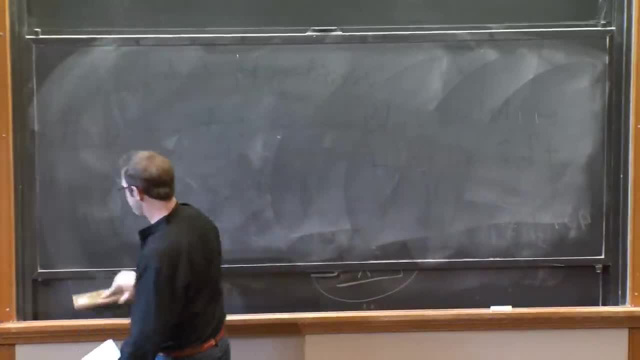 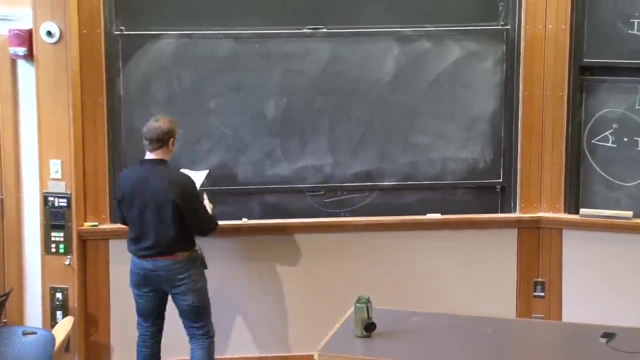 is. I want to run some simple experiments before we get to fancy stuff. And the simple experiments are just going to warm you up. They're going to prepare you to make some predictions and some calculations And eventually we'd like to lead back to this guy. 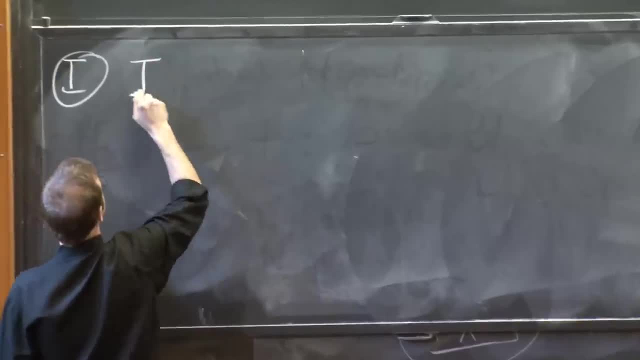 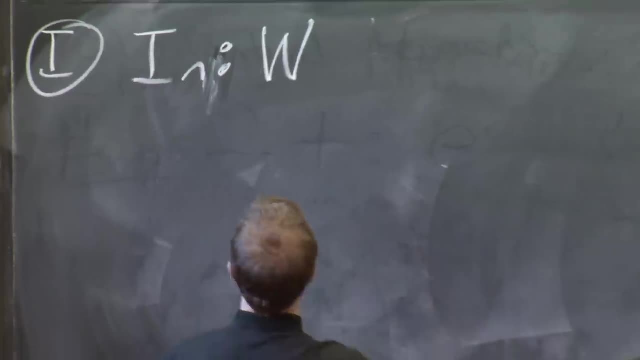 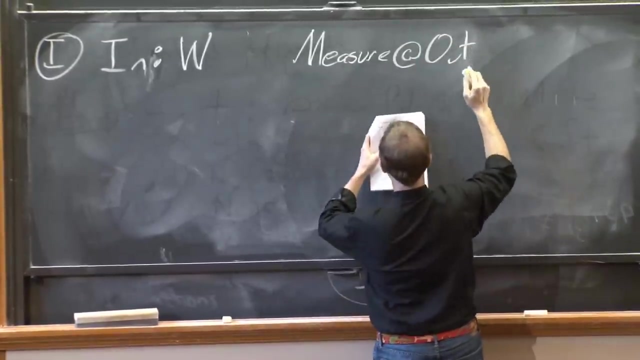 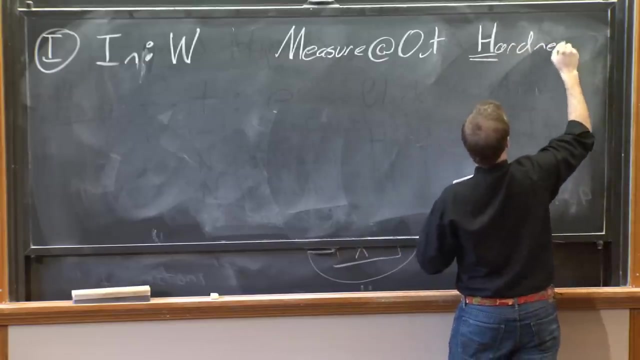 So the first experiment: I'm going to send in white electrons. Whoops, I'm going to send in white electrons And I'm going to measure at the end and in particular at the output, the hardness. OK, So I'm going to send in white electrons. 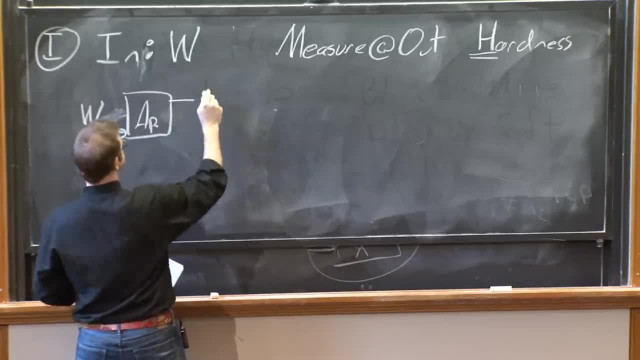 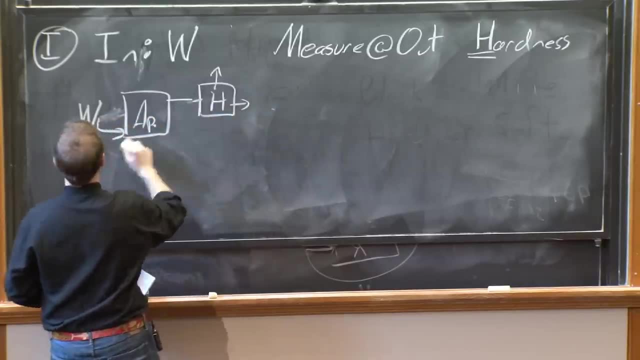 And I'm going to measure the hardness. So this is my apparatus: I'm going to measure the hardness at the output, And what I mean by measure the hardness is: I throw these electrons into a hardness box and see what comes out. So this is experiment one. 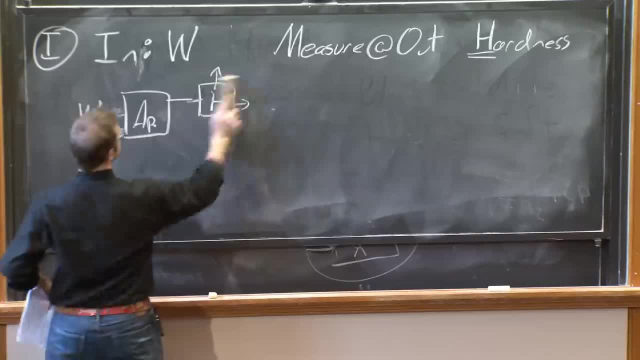 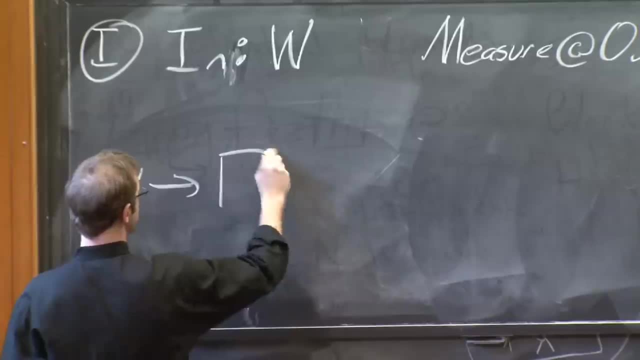 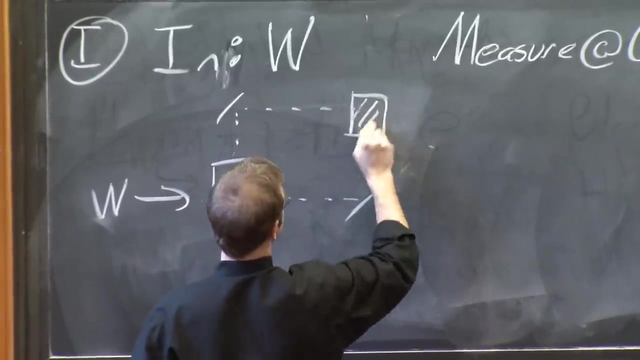 And let me draw this. OK, So this is experiment one And let me draw this, And let me draw this, Let me big in the diagram So you send white into. So the mechanism is a hardness box, mirror, mirror mirrors. 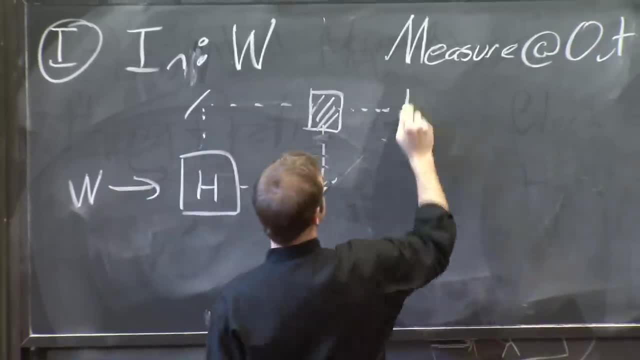 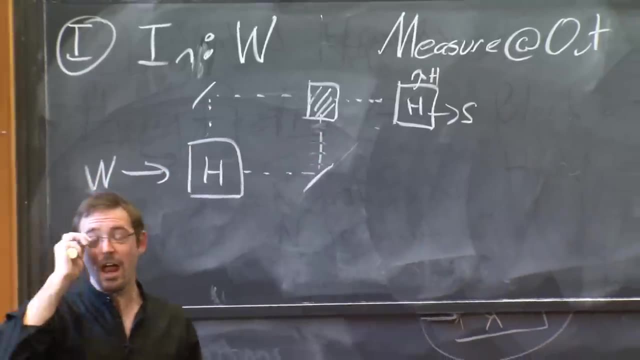 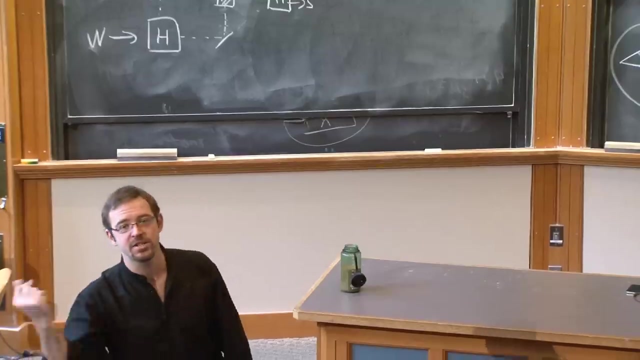 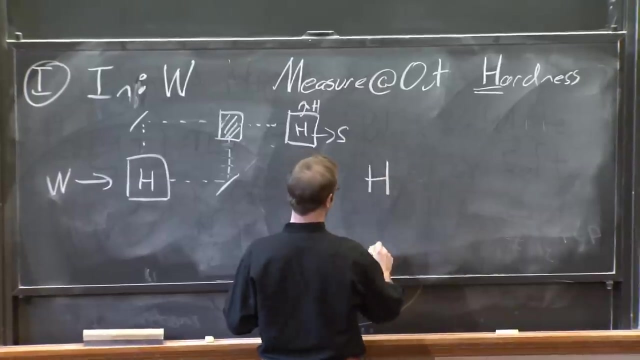 And now whoops, we're measuring the hardness out. So hardness, And the question I want to ask is how many electrons come out the hard aperture And how many electrons come out the soft aperture of this final hardness box? So I'd like to know what fraction come out hard? 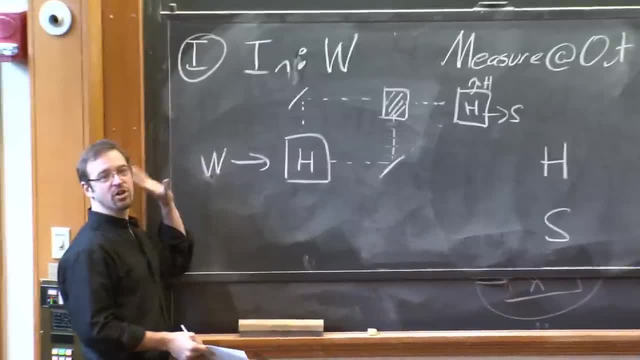 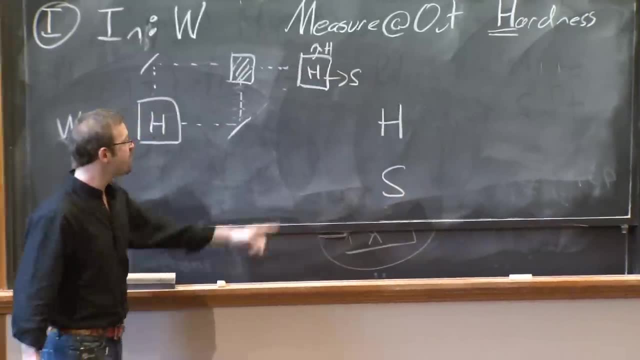 and what fraction come out soft. I send an initial white electron. For example, I took a color box and took the white output. Send them into the hardness box. mirror, mirror, hard, hard, soft, And what fraction come out hard and what fraction come out soft. 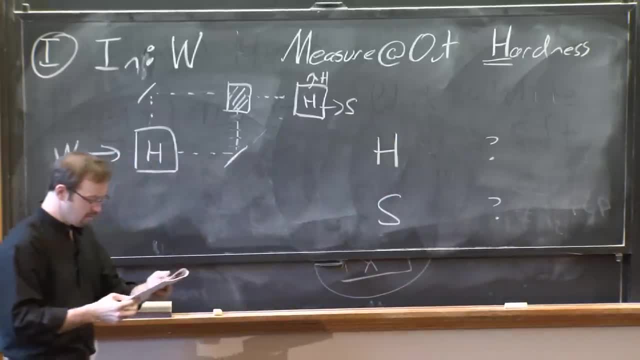 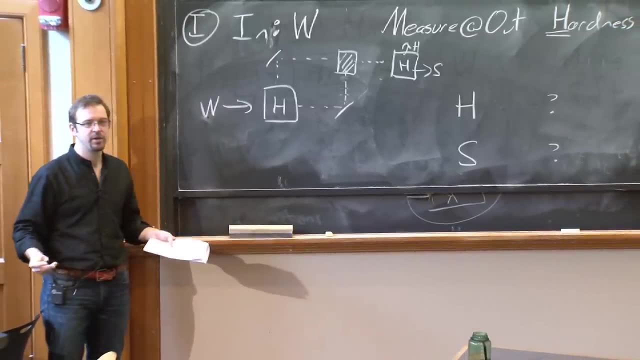 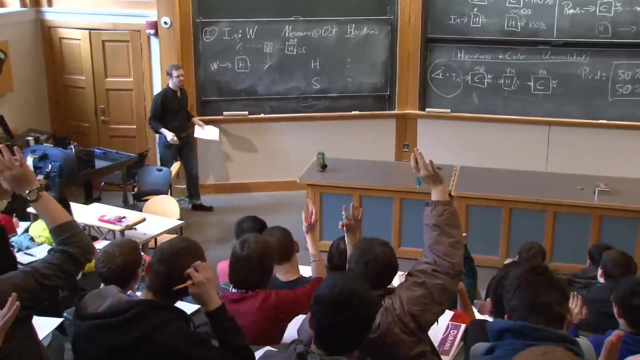 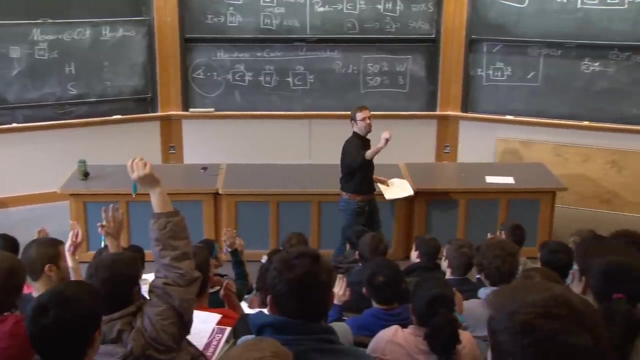 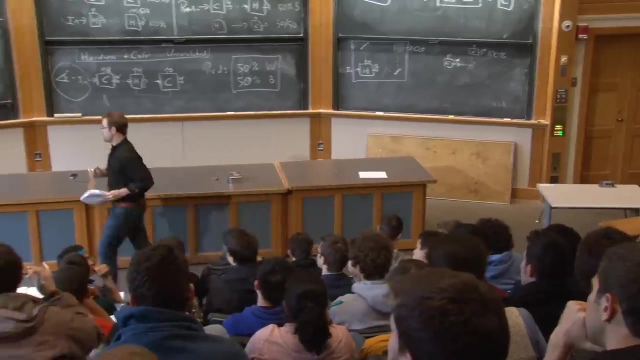 OK, So just think about it for a minute And when you have a prediction in your head, raise your hand. All right, Good, Walk me through your prediction. OK, 50-50.. How come I'm seeing four of the colors? 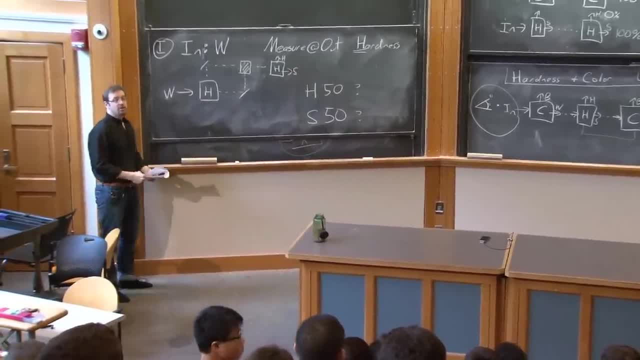 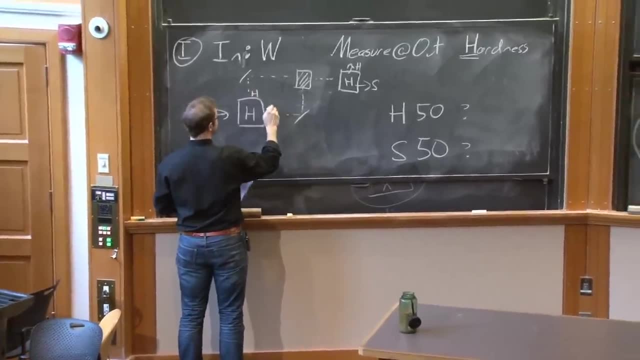 have a bearing on hardness. Good. So it's going to go to the hardness box, like we expected it to come out of there, And then, once again, it'll go to the other hardness box- Awesome. So let me say that again. 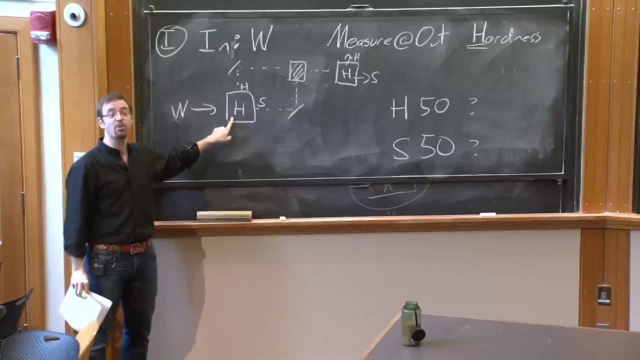 So we've done the experiment. You send a white electron into a hardness box And we know that it's non-predictive 50-50.. So if you take a white electron and you send it into the hardness box, 50%. 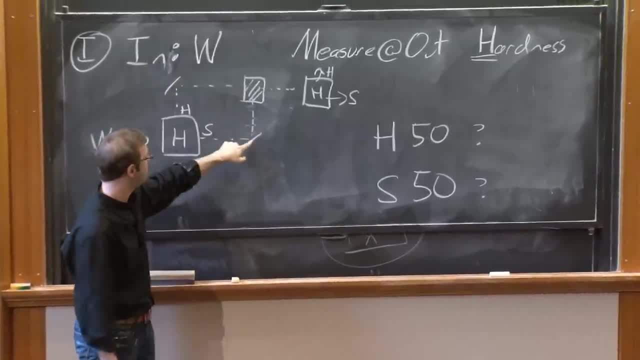 OK, OK, OK, OK, 50% of the time it will come out the hard aperture And 50% of the time it will come out the soft aperture. Now, if you take the one that comes out, the hard aperture- 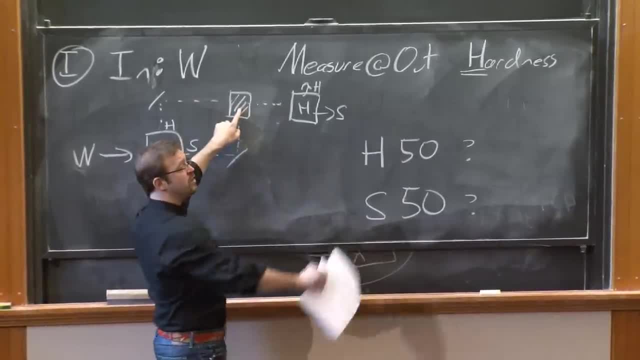 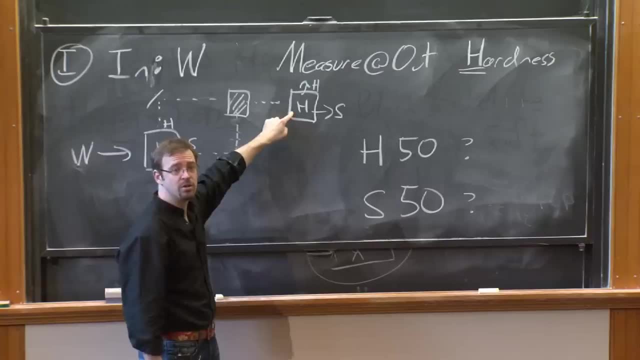 then you send it up here. send it up here. We know that these mirrors do nothing to the hardness of the electron except change the direction of motion. We've already done that experiment. So you measure the hardness at the output. what do you get? 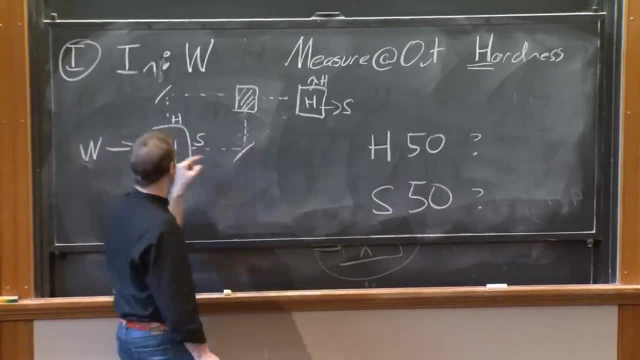 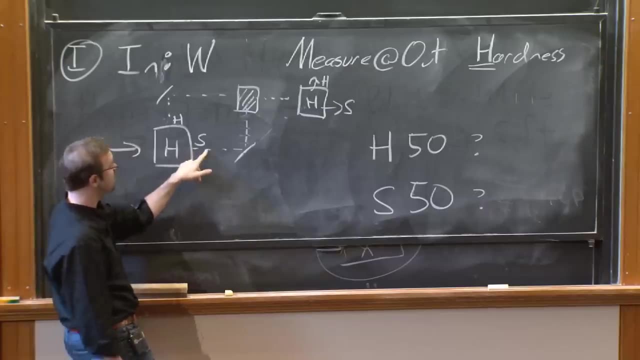 Hard because it came out hard. Mirror, mirror, hardness, hard. But it only came out hard 50% of the time because we sent in an initially white electron. Yeah, What about the other 50%? Well, the other 50% of the time it 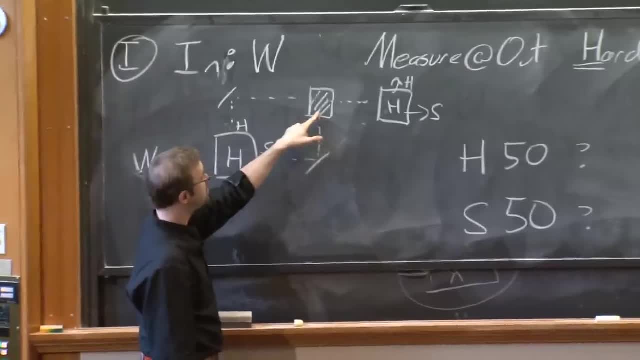 comes out the soft aperture and follows what I'll call the soft path to the mirror mirror hardness. And with soft mirror mirror hardness, you know it comes out soft 50% of the time it comes out this way. 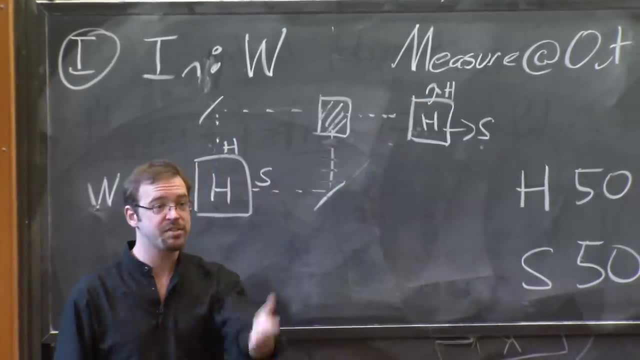 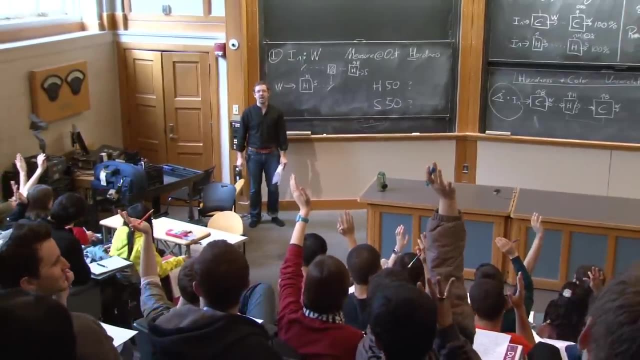 and then it will come out hard. 50%: it follows the soft path and then it will come out soft. Was this the logic Good? How many people agree with this? Solid? How many people disagree? No, abstention, OK. 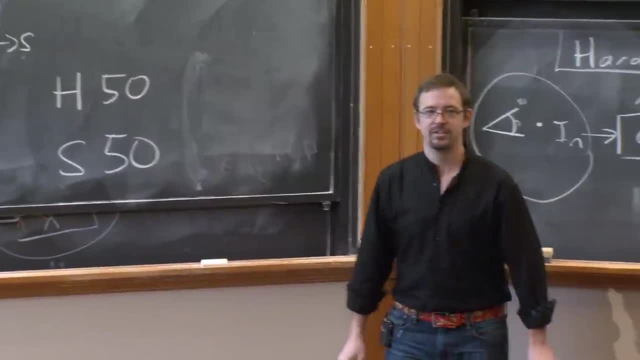 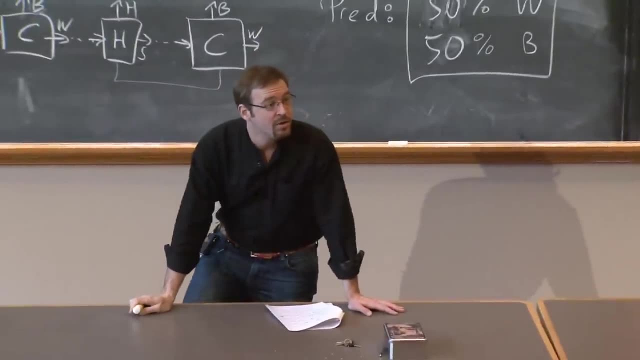 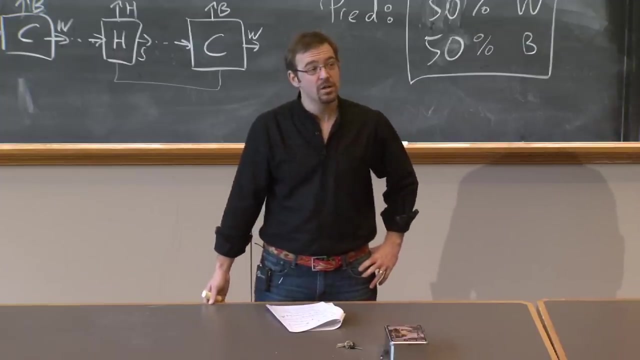 So here's a prediction: Surveys, Surveys, Oh yep, Just a question: Could you justify that prediction without talking about? oh well, half the electrons were initially measured to be hard and half were initially measured to be soft. 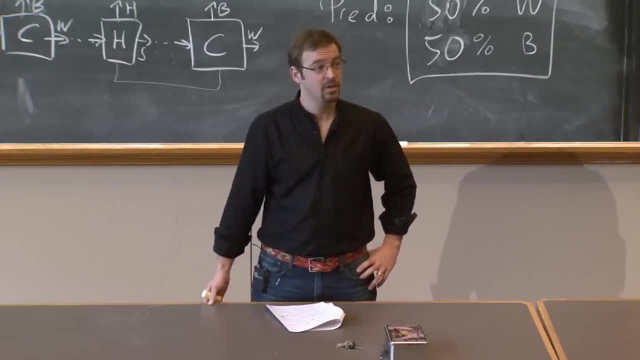 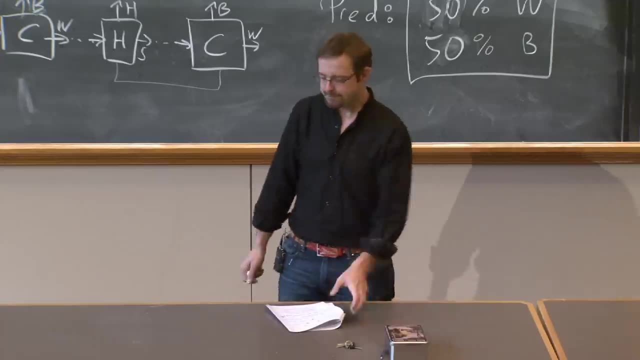 by just saying: well, we have a hardness box and then we join the beams of electrons together again, So we don't know anything about it. So it's just like sending white electrons into one hardness box instead of two. Yeah, That's a really tempting argument, isn't it? 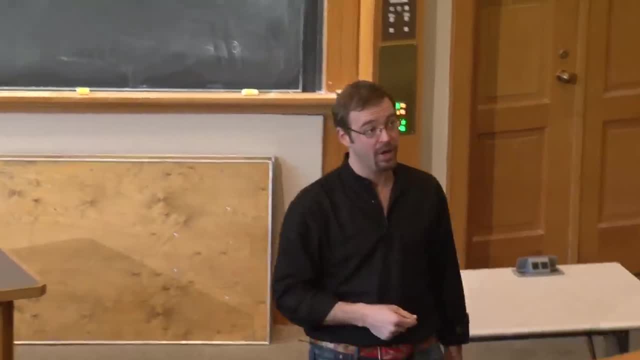 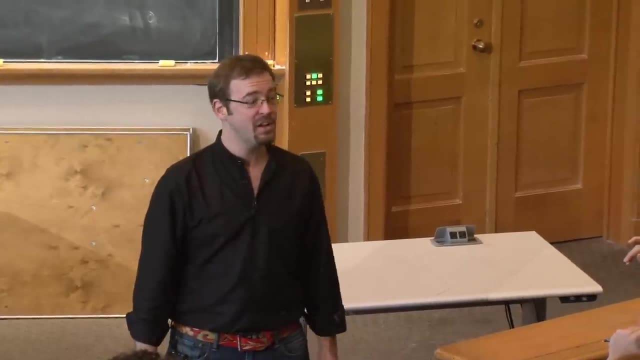 So let's see. We're going to see in a few minutes whether that kind of an argument is reliable or not, But so far we've been given two different arguments that lead to the same prediction: 50-50.. Yeah, Question. 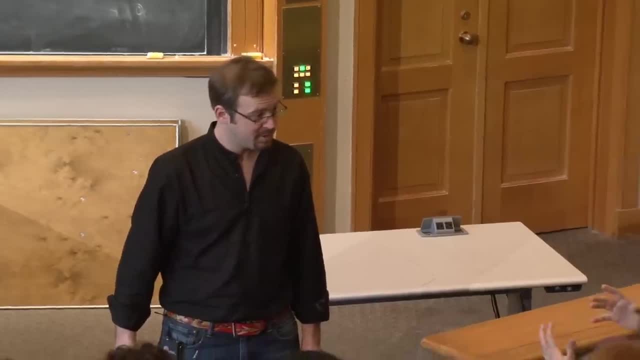 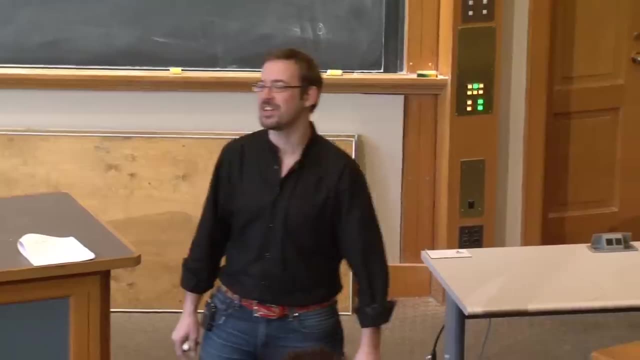 Those like those electrons interact between themselves, Like when you get them together. Yeah, This is a very good question. So here's a question. Look, you're sending a bunch of electrons into this apparatus, But if I take two, look I took 802, you know. 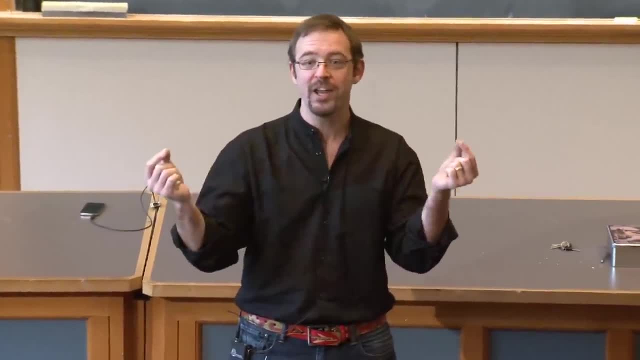 You take two electrons and you put them close to each other. what do they do? Pew Right, They interact with each other through a potential Right. So we're being a little bold here, throwing a bunch of electrons in and saying: 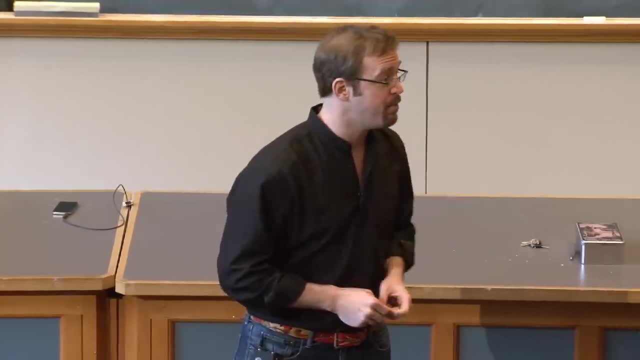 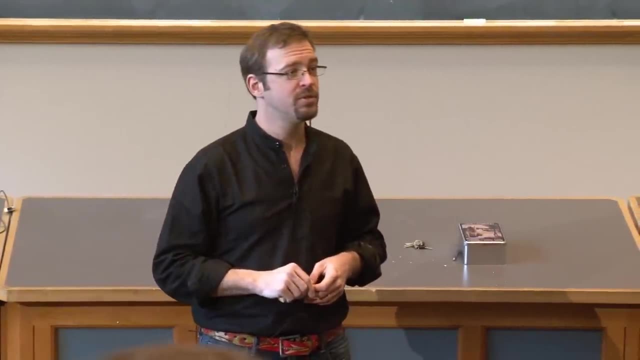 oh, they're independent. So I'm going to do one better. I will send them in one at a time, One electron through the apparatus, And then it will wait for six weeks, And then I'll say: see you guys, laugh. 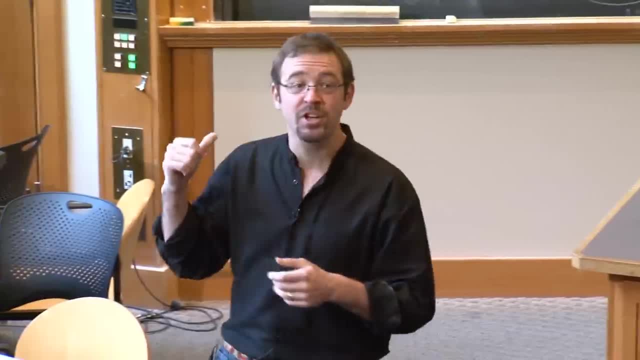 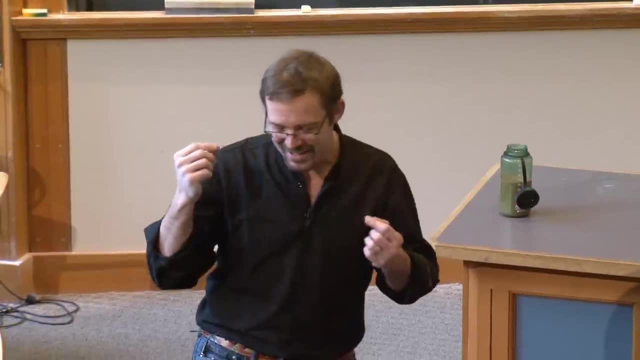 You think that's funny, But there's a famous story of a guy who did a similar experiment with photons. OK, French guy, I mean the French, they know what they're doing. So he wanted to do the same experiment with photons. 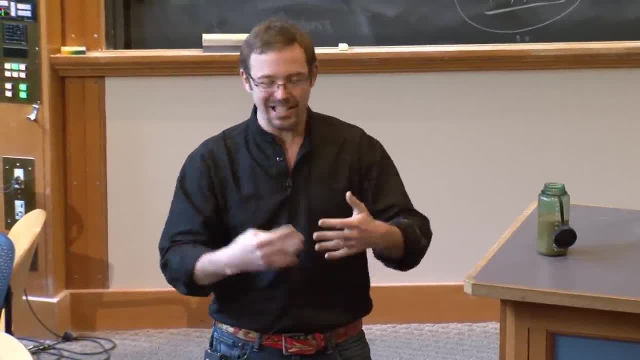 But the problem is, if you take a laser and you shine it into your apparatus, then there are like 10 to the 18 electrons in there, or photons in there at any given moment, And the photons who knows what they're. 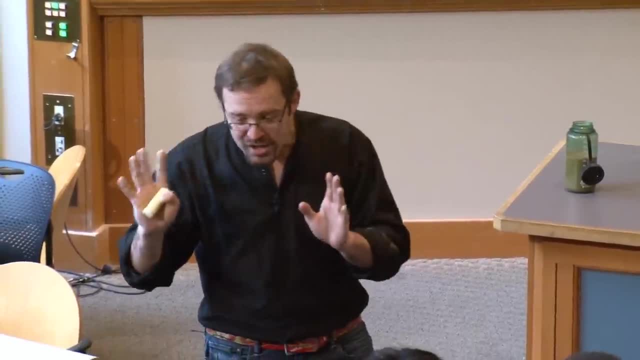 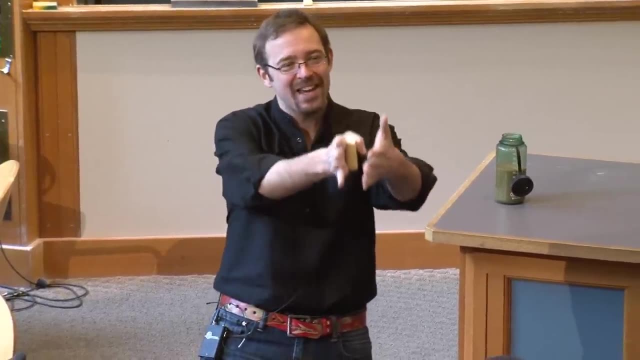 doing with each other, Right? So I want to send in one photon, But the problem is it's very hard to get a single photon, Very hard. So what he did, if you're not, he took an opaque barrier. I don't remember what it was. 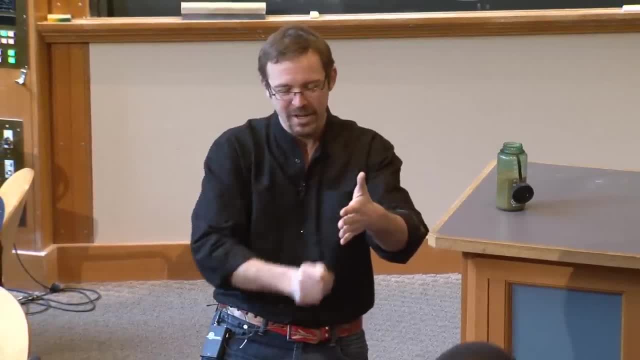 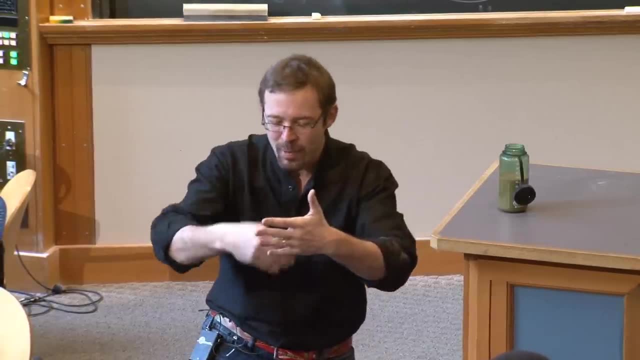 It was some sort of film on top of glass. I think it was some sort of oil tar film. Barton, do you remember what he used? OK, so he takes a film and it has this opaque property such that the photons that are incident on upon it. 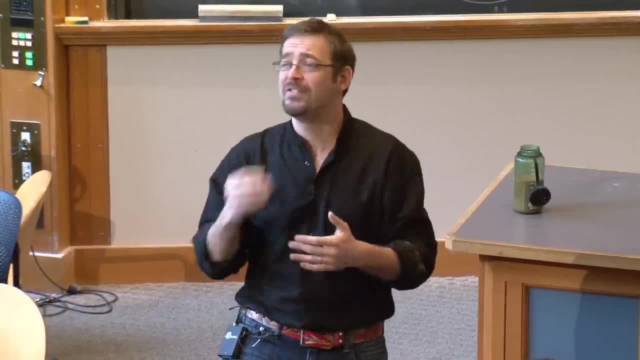 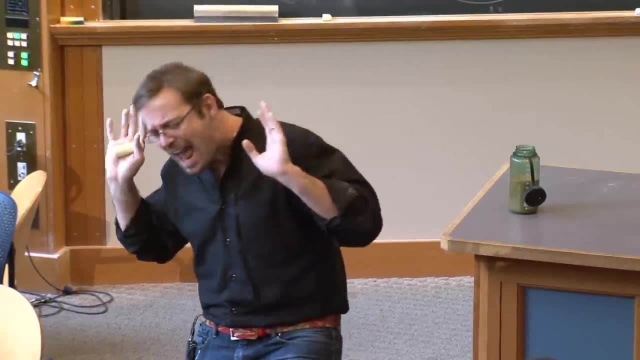 get absorbed. Once in a blue moon, a photon manages to make its way through, Literally like once every couple of days Now, or a couple of hours, I think. So it's going to take a long time to get any sort of statistics. 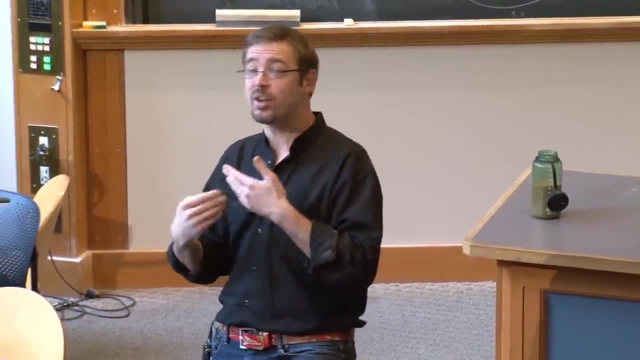 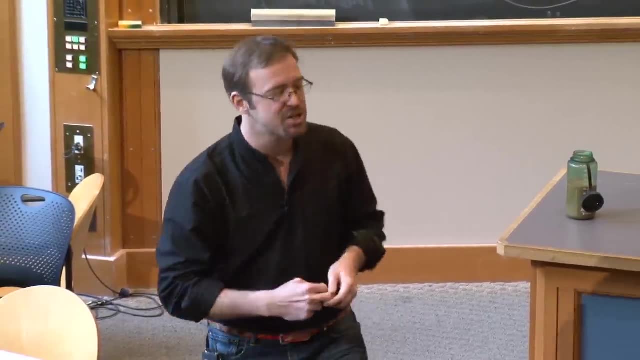 But he has this advantage that once every couple of hours or whatever, a photon makes its way through, That means inside the apparatus. if it takes a picosecond to cross, triumph Right, That's the week I was talking about. 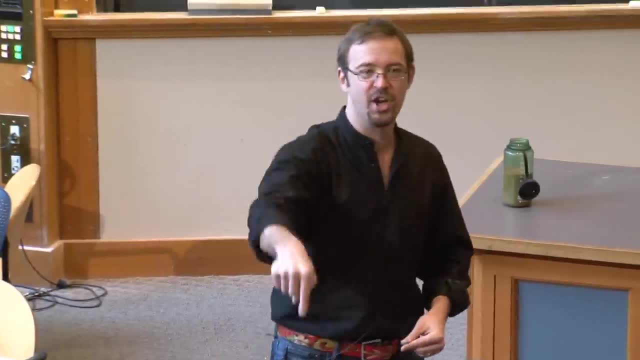 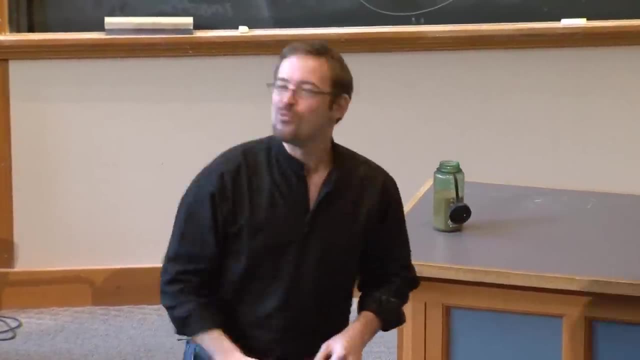 So he does this experiment, But, as you can tell, you start the experiment, you press go and then you wait for six months. Side note on: this: guy Liked boats, Really liked yachts, So he had six months to wait before doing. 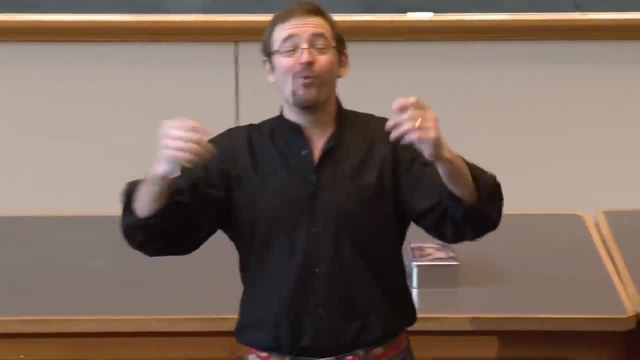 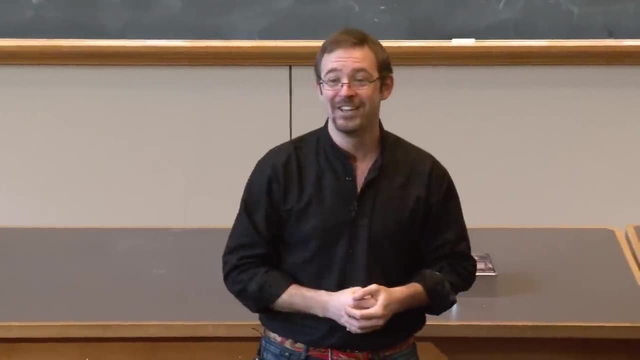 a beautiful experiment, having the results. and what did he do? Went on a world tour in his yacht, Comes back, collects the data and declares victory, Because indeed he saw the effect he wanted. So I was not kidding, We really do wait. 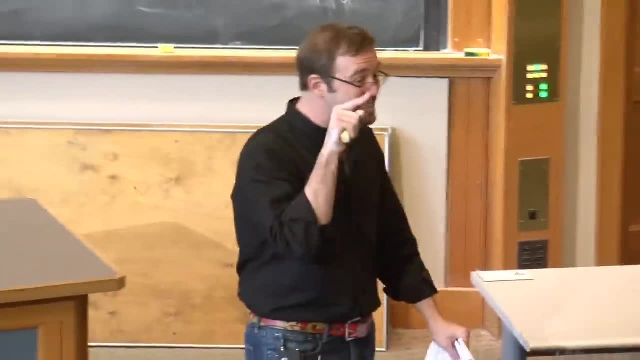 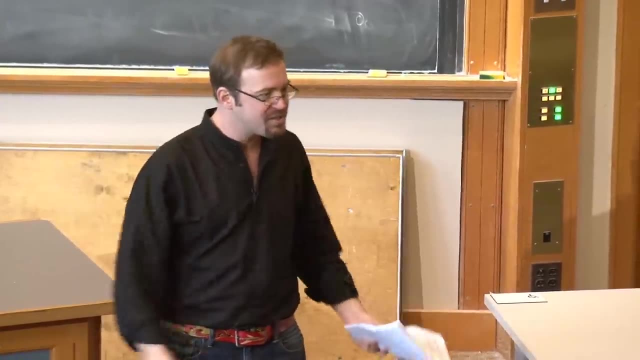 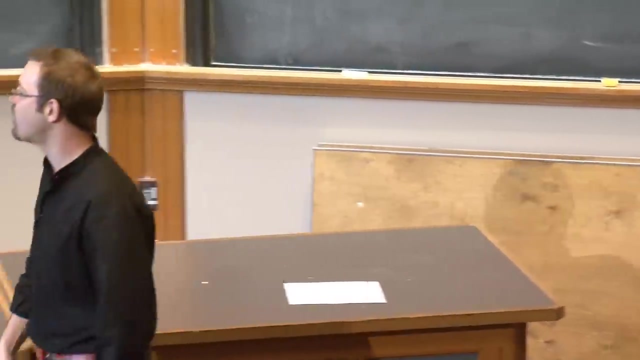 So I will take your challenge and single electron, throw it in, let it go through. the apparatus takes mere moments. wait for a week, send in another electron. No electrons are interacting with each other. OK, Just a single electron at a time going through this apparatus. 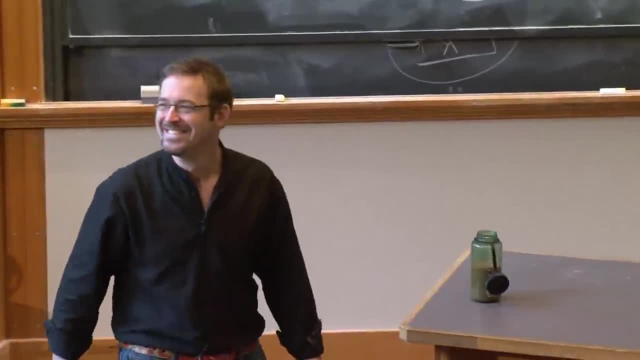 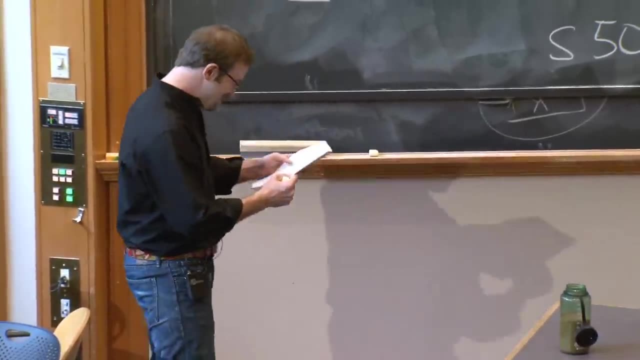 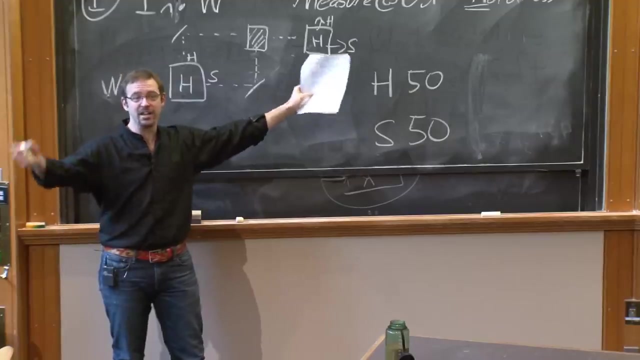 Other complaints. Sorry, More stories. Oh, you'll get them. I have a hard time resisting. So here's the prediction: 50-50.. We now have two arguments for this. So, again, let's vote after the second argument. 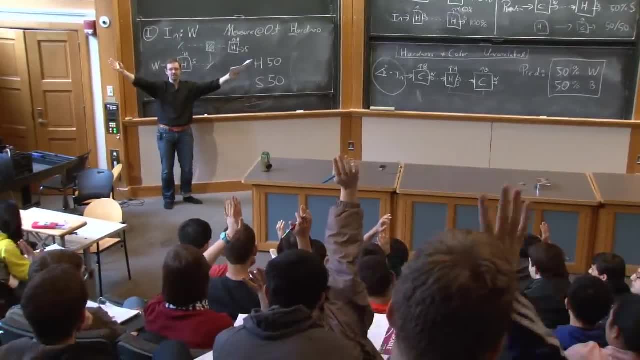 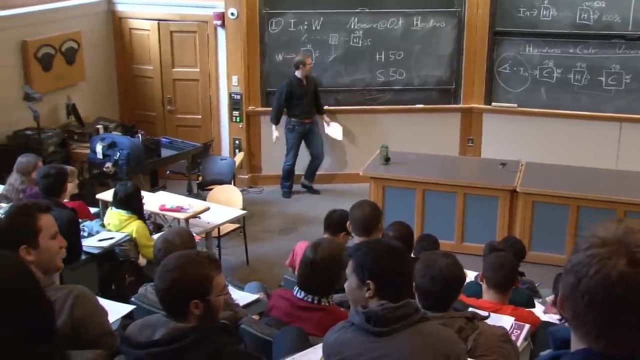 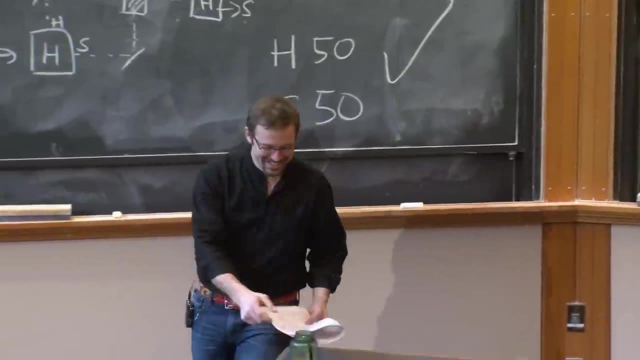 50-50,. how many people You sure Positive, Positive, OK. How many people don't think so? Very small dust, OK, It's correct. Yay, OK, So good. So I like messing with you guys. 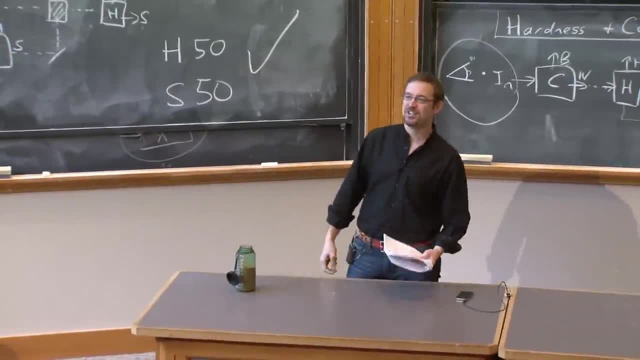 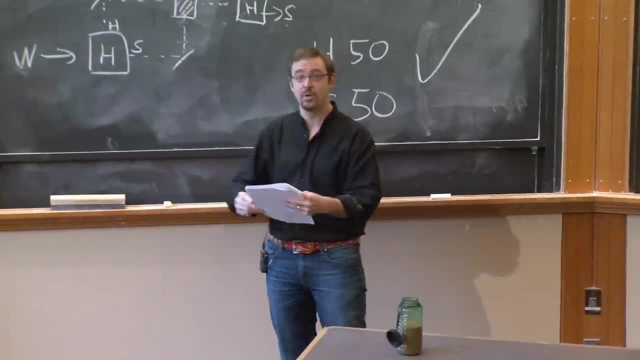 So, remember, we're going to go through a few experiments first, where it's going to be very easy to predict the results. We've got four experiments like this to do, And then we'll go on to the interesting examples. But we need to go through them so we know what happens. 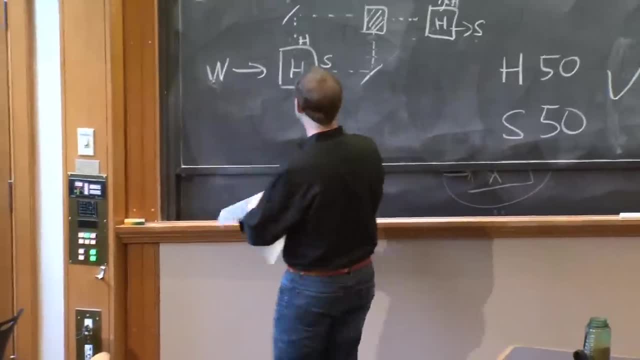 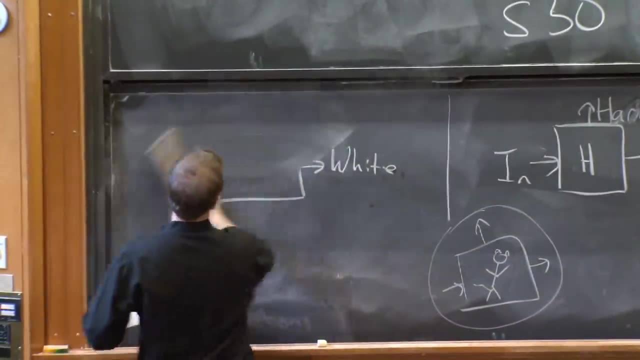 so we can make an empirical argument rather than an in-principle argument. So there's the first experiment. Now we want to run the second experiment. And the second experiment same as the first, a little bit louder, a little bit worse. 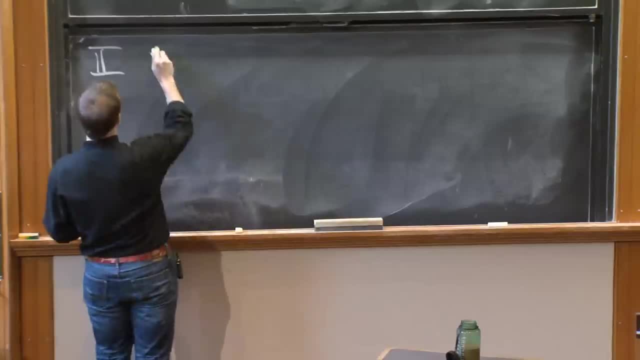 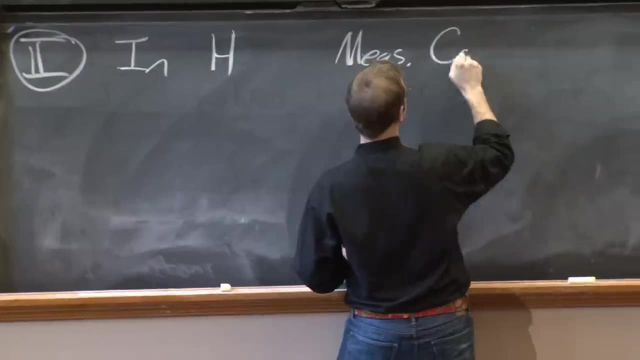 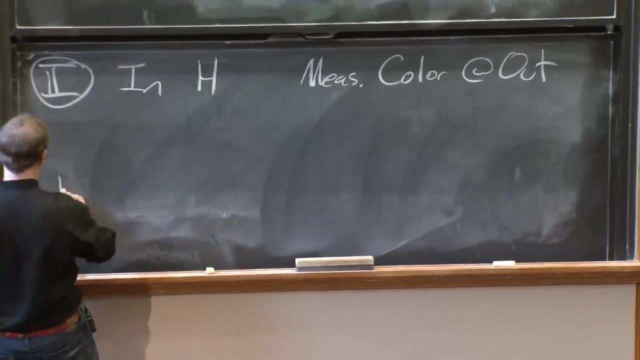 Sorry, The second experiment: we're going to send in hard electrons And we're going to measure color at out. OK, So again, let's look at the apparatus. We send in hard electrons And our apparatus is hard box, hardness box. 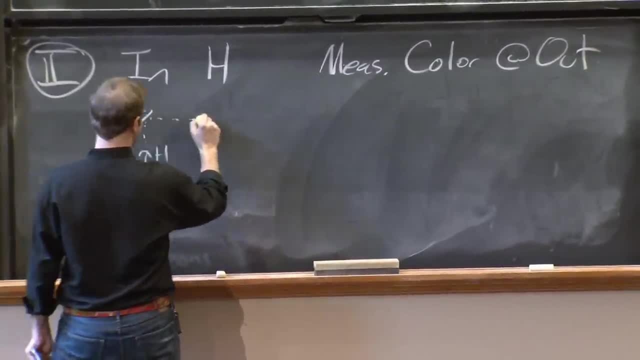 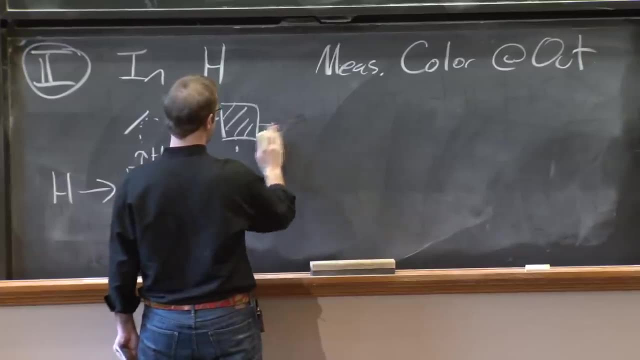 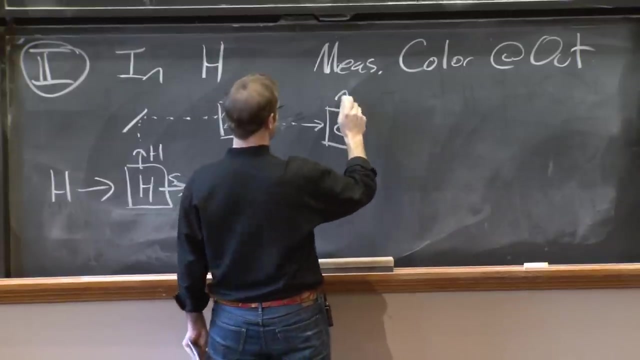 with a hard and a soft aperture, And now we're going to measure the color at the output Color. What have I been doing? Black, And now I want to know what fraction come up, OK, OK, OK. So black and white fraction come out white. 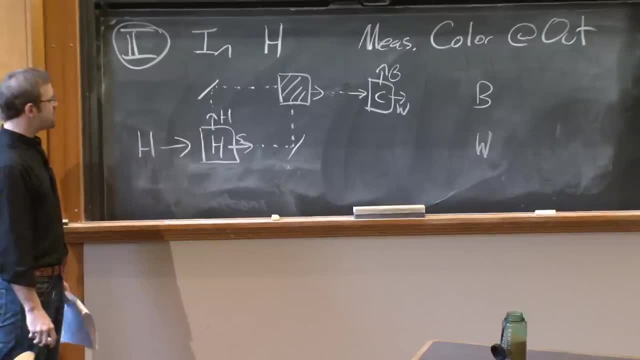 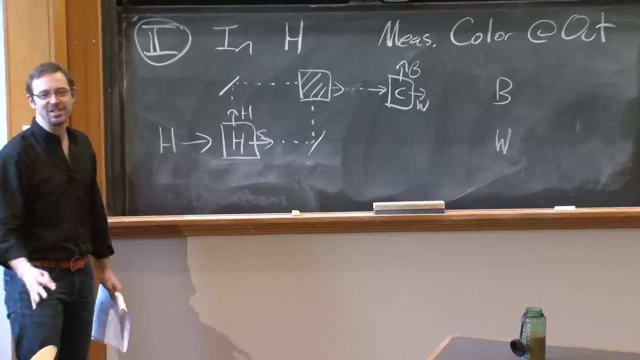 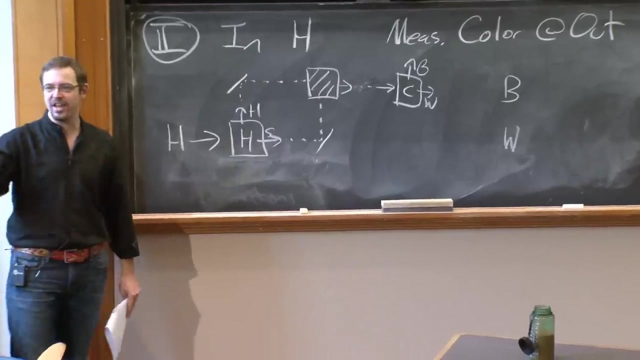 We're using lots of monkeys in this process. OK, So this is not rocket science. Rocket science isn't that complicated. Neuroscience is much harder. This is not neuroscience. OK, So let's figure out what this is. Predictions. So again, think about your prediction in your head. 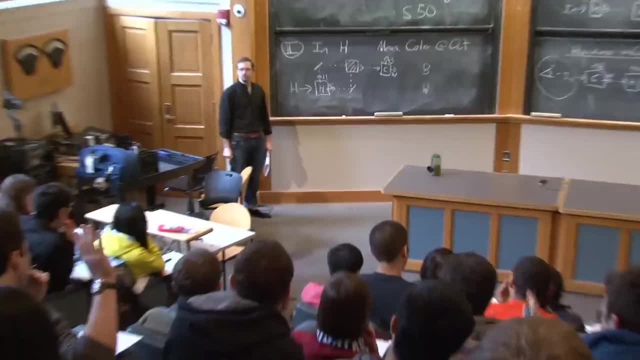 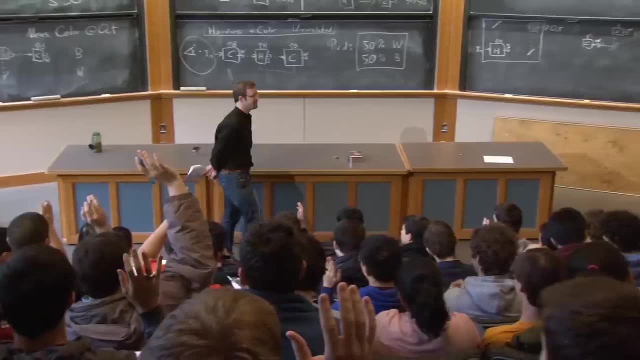 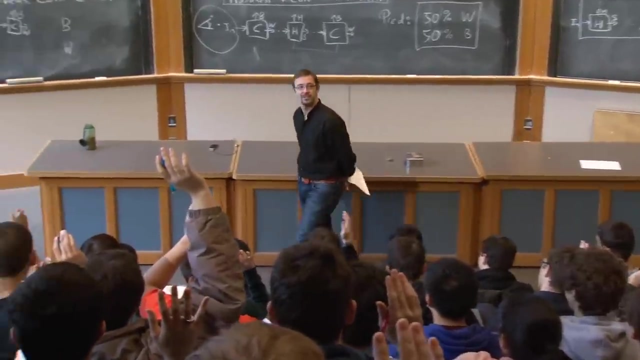 Come to a conclusion. Raise your hand when you have an idea. And just because you don't raise your hand doesn't mean I won't call on you. 50-50 black and white. 50-50 black and white. I like it. 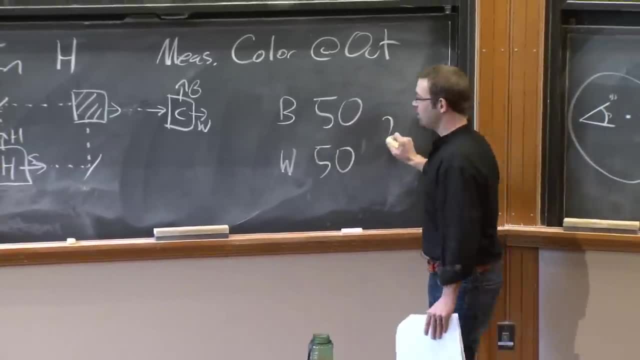 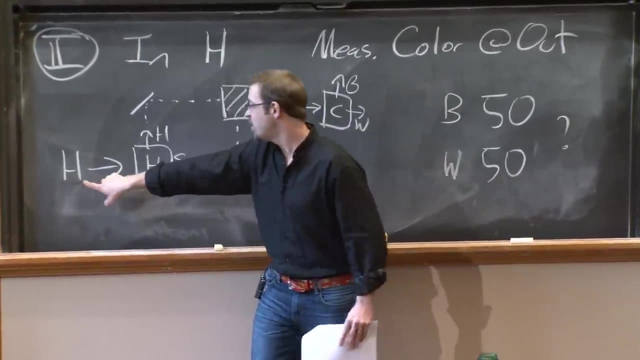 Tell me why It's done through a hardness box which should have a one color and then will have to be different colors. Great, So the statement- I'm going to say that slightly more slowly. That was exactly. That was an excellent argument. 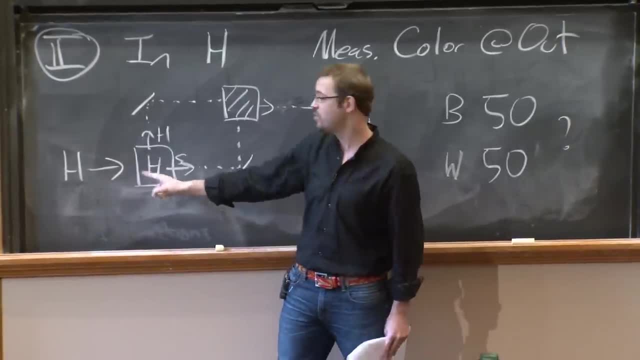 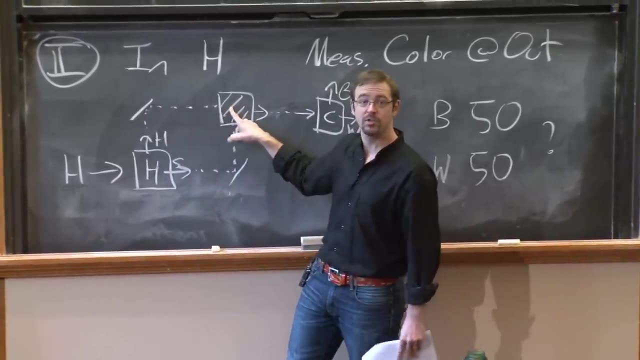 We have a hard electron. We know that hardness boxes are persistent. If you send a hard electron in, it comes out hard. So every electron incident upon our apparatus will transit across the hard trajectory. It will bounce. It will bounce, But it is still hard because we've already 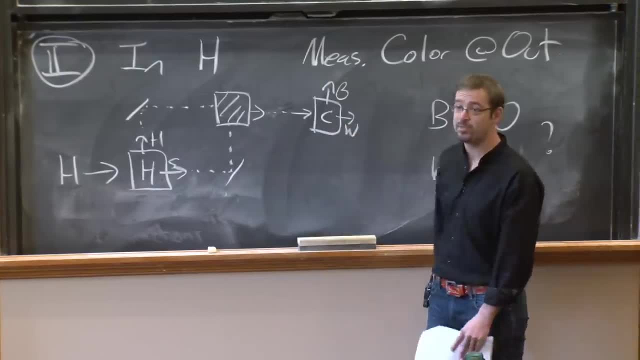 done that experiment. The mirrors do nothing to the hardness. So we send a hard electron into the color box And what comes out? Well, we've done that experiment too Hard into color 50-50.. The prediction is 50-50.. 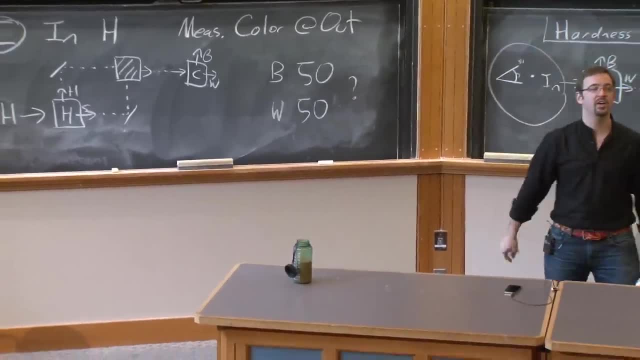 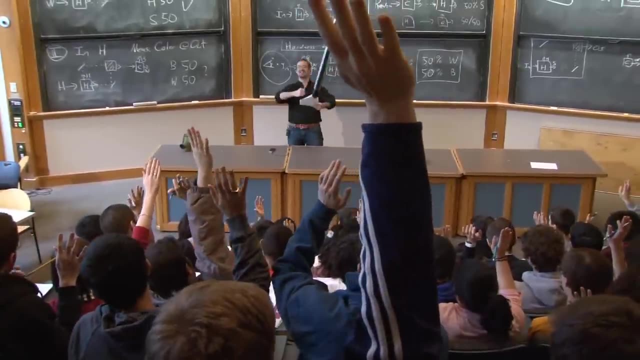 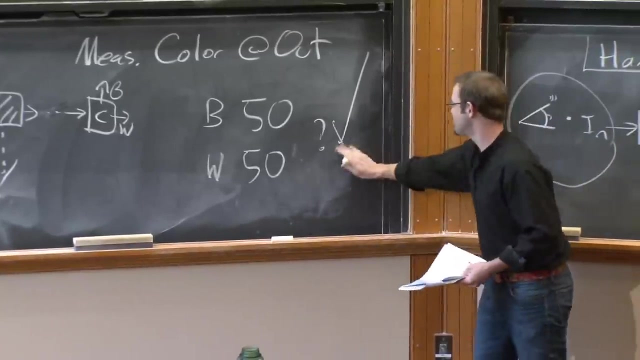 This is your prediction. Is that correct? Awesome, OK, OK. OK, Let us vote. How many people think this is correct? Gusto, I like it. How many people think it's not All right? Yay, This is correct. 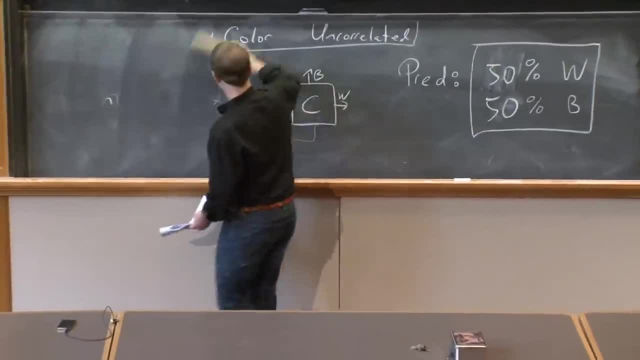 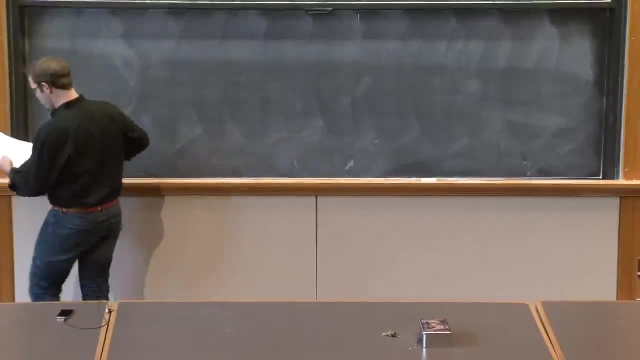 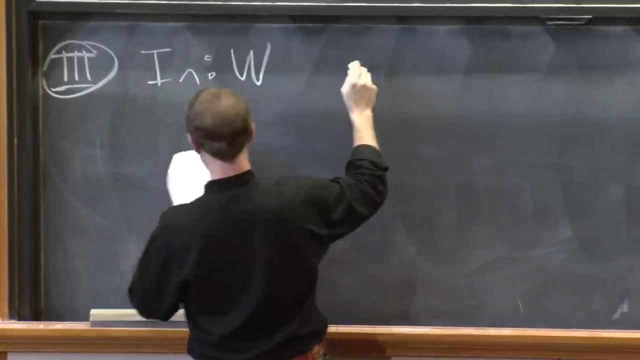 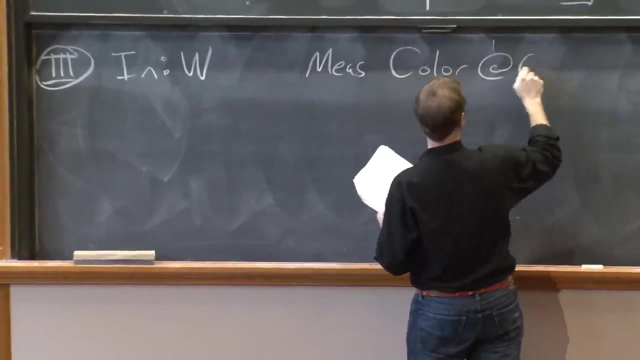 OK, Third experiment, slightly more complicated, But we have to go through these to get to the good stuff. So humor me for a moment. Third: Let's send in White electrons And then measure the color at the output port. So now we send in white electrons- same beast. 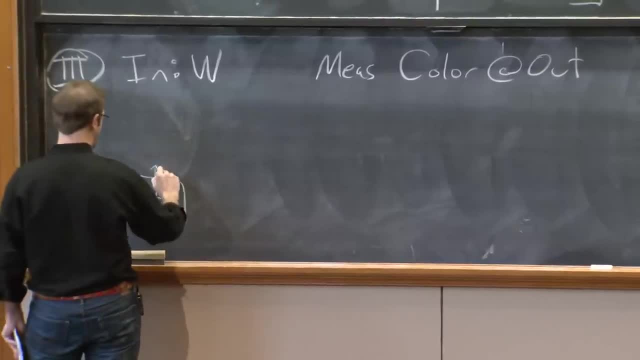 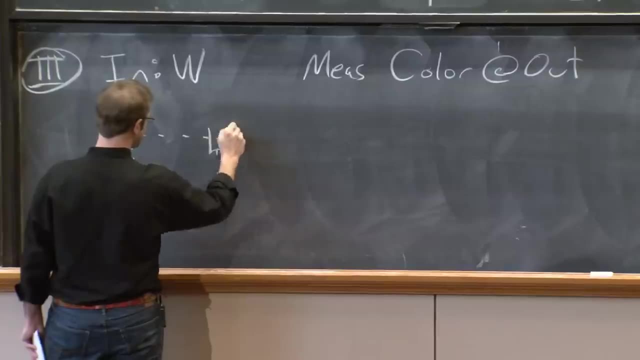 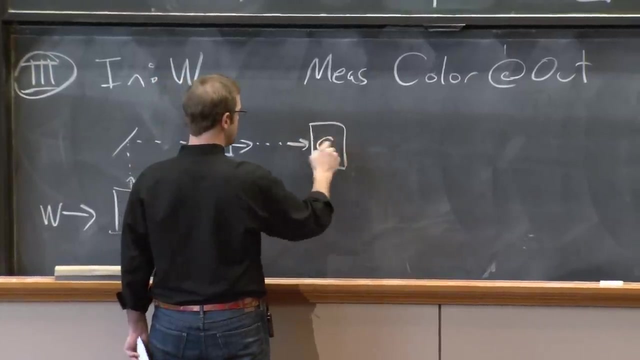 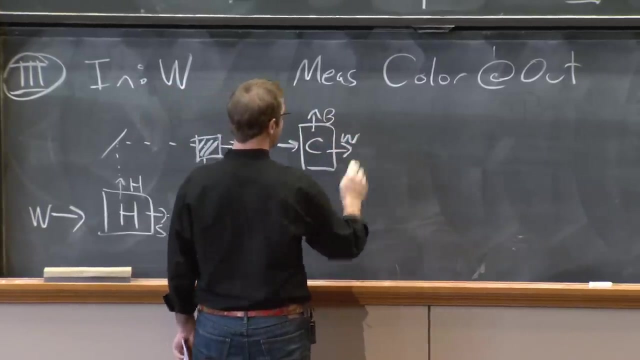 And our apparatus is hardness box with a hard path and a soft path. Doo doo doo mirror, doo doo doo mirror box joined together into our out And now we send those out electrons into a color box and our color box black and white. 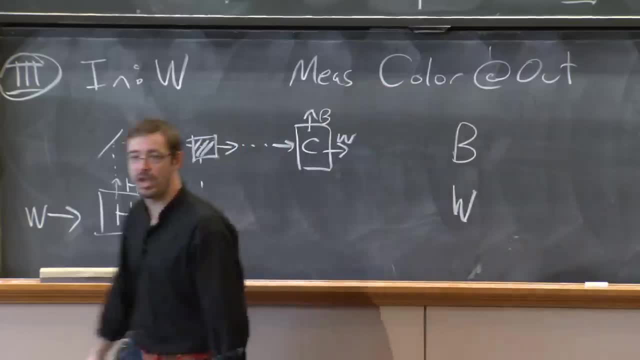 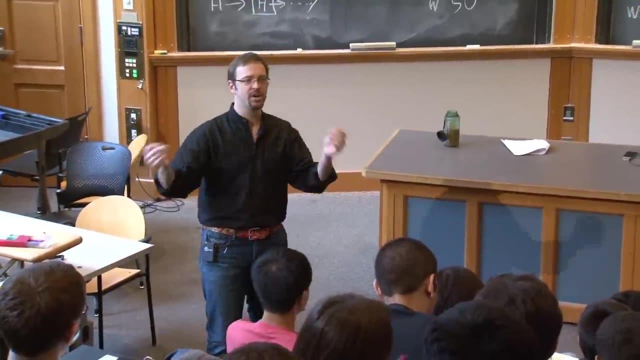 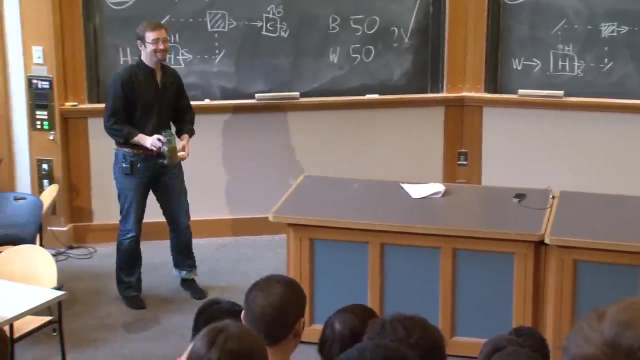 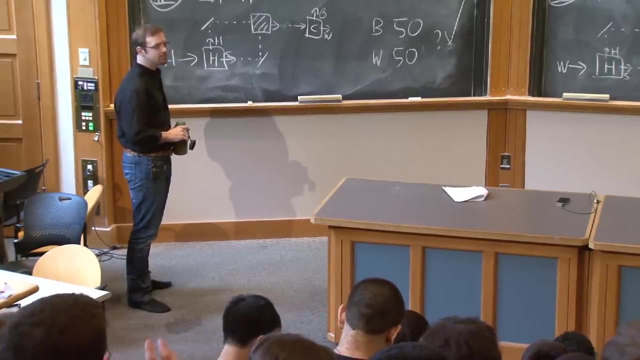 And now the question is: how many come out black and how many come out white? OK Again, think through the logic, follow the electrons, come up with a prediction. Raise your hand when you have a prediction, OK, OK. 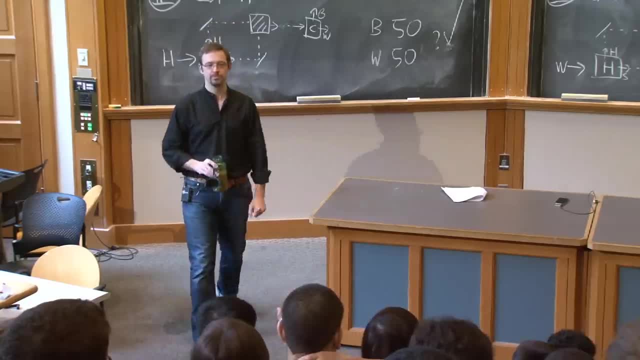 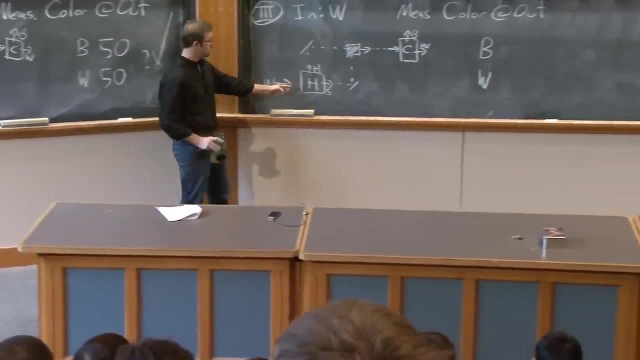 So if you're going to be taking all the color in the same place, you don't even need to use the other one. You just have to pick a color box- the original color box. You just have to pick a color box and then split it out. 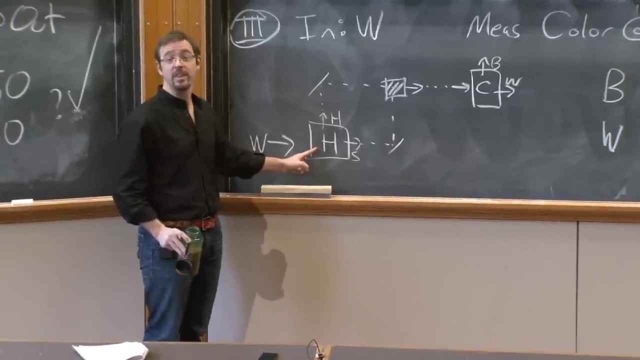 So the colors don't change. So if you're going to be using a random color box, you just have to split it out. So we just have to make sure that those colors are the same, And then you just put the color. 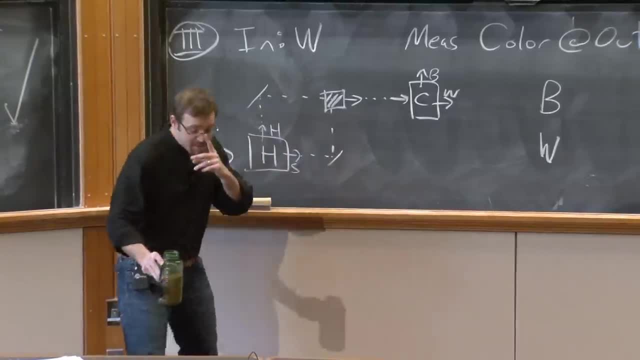 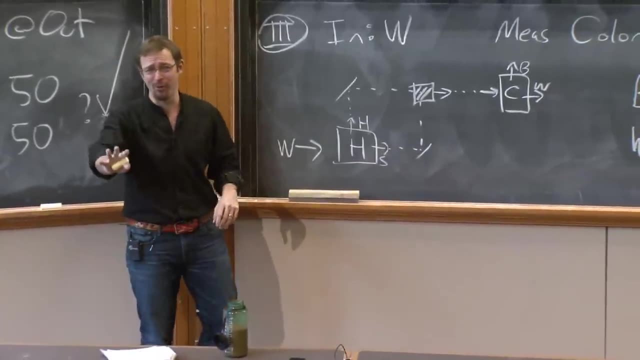 You can do the same thing with other colors. OK, I would say so, Great. So let me say that again out loud and tell me if this is an accurate sort of extension of what you said. I'm just going to use more words. 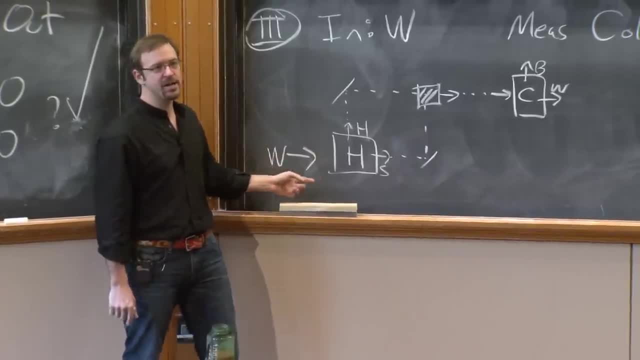 but it's, I think, the same logic. We have a white electron, initially a white electron. We send it into a hardness box. When we send a white electron into a hardness box, we know what happens. 50% of the time it comes out hard: the hard aperture. 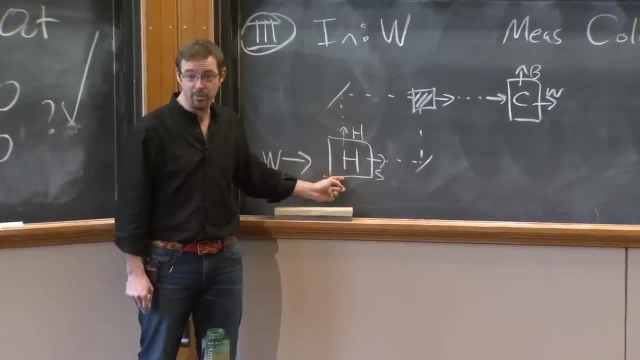 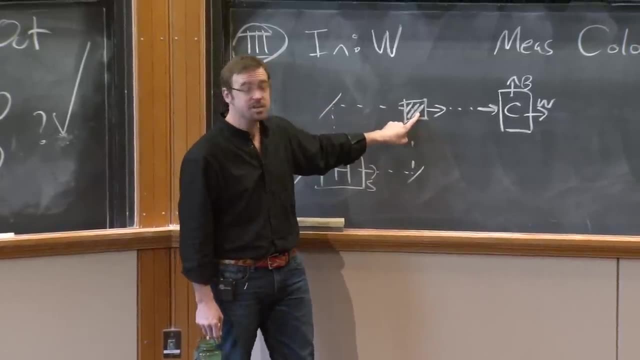 50% of the time it comes out the soft aperture. Consider those electrons that came out the hard aperture. Those electrons that came out the hard aperture will then transit across the system, preserving their hardness by virtue of the fact that these mirrors preserve hardness. 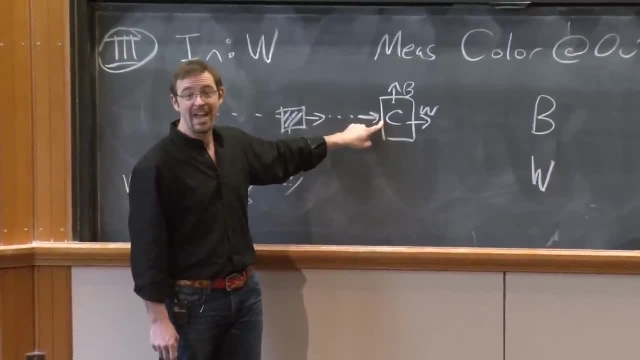 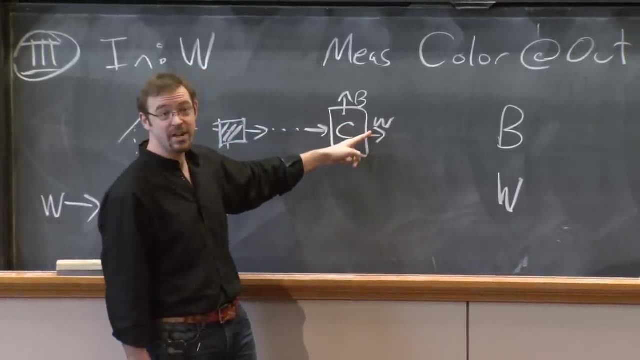 and end up in a color box. When they end at the color box, when that electron, the single electron in the system, ends at this color box, then we know that a hard electron entering the color box comes out black or white 50% of the time. 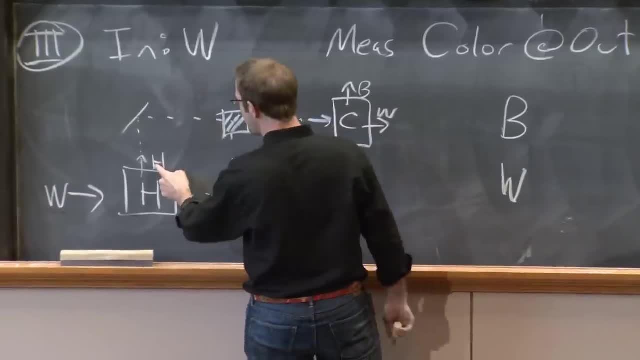 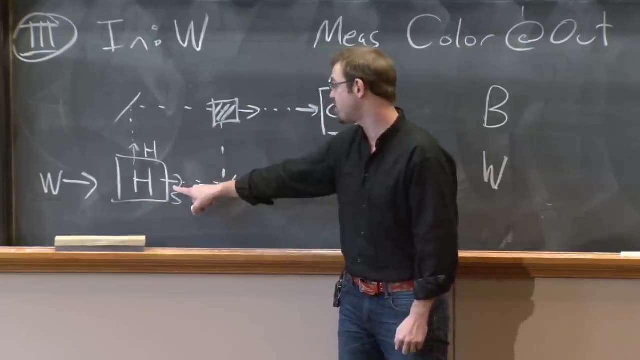 We've done that experiment too. So for those 50% that came out hard, we get 50-50.. Now consider the other 50%. The other half of the time the single electron in the system will come out- the soft aperture. 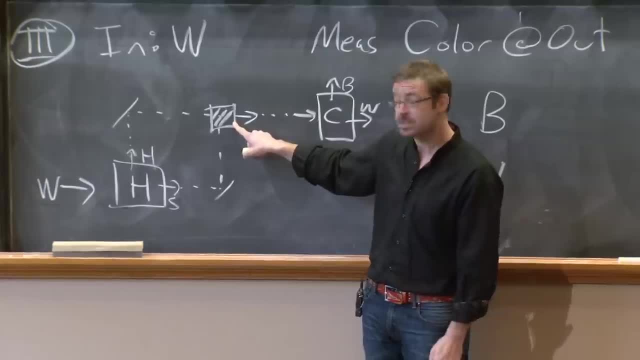 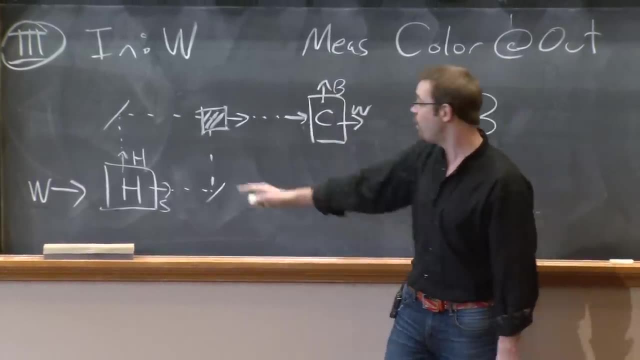 It will then proceed along the soft trajectory, bounce-bounce, not changing its hardness, and is then a soft electron incident on the color box. But we've also done that experiment and we get 50-50 out black and white. So those electrons that came out hard come out 50-50,. 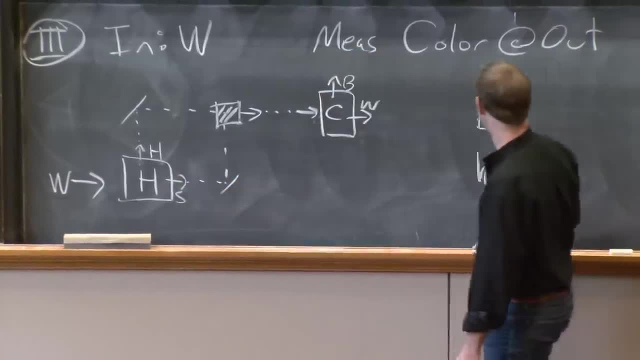 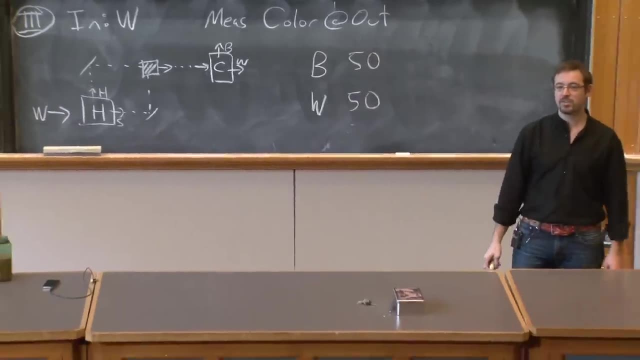 and those electrons that come out soft come out 50-50. And the logic then leads to 50-50 twice 50-50.. Was that an accurate statement? Good, Pretty reasonable extension. OK, let's vote. How many people agree with this one? 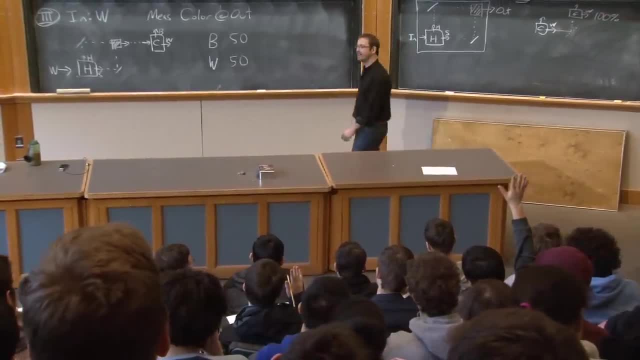 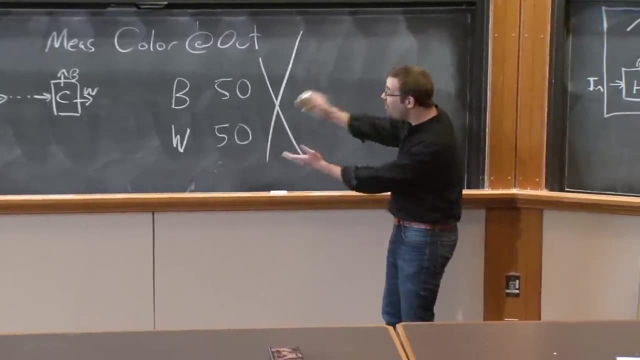 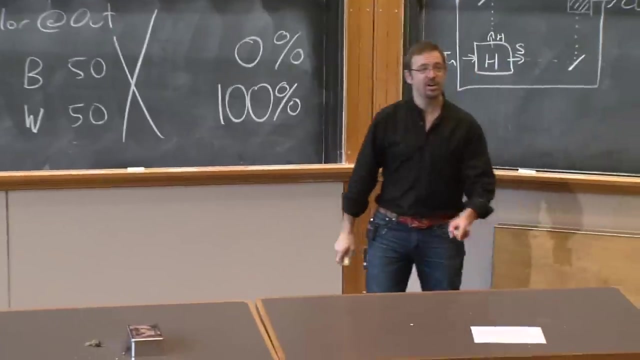 OK, and how many people disagree? Yeah, OK, so vast majority agree, and the answer is no. This is wrong. In fact, of these, 100% come out white and 0 come out black. Never, ever, does an electron come out the black aperture. 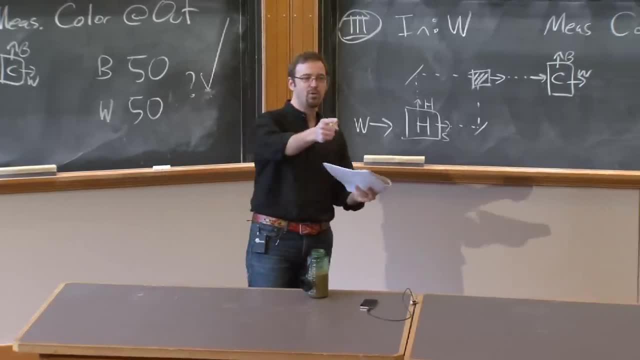 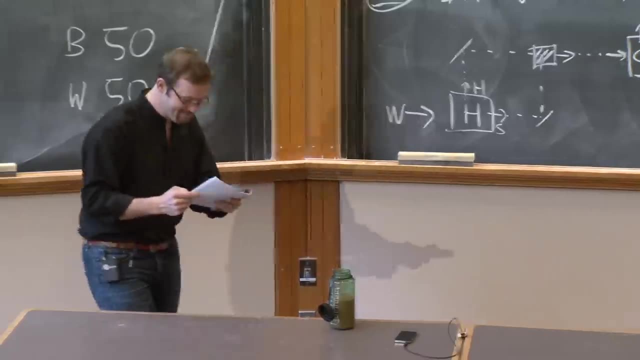 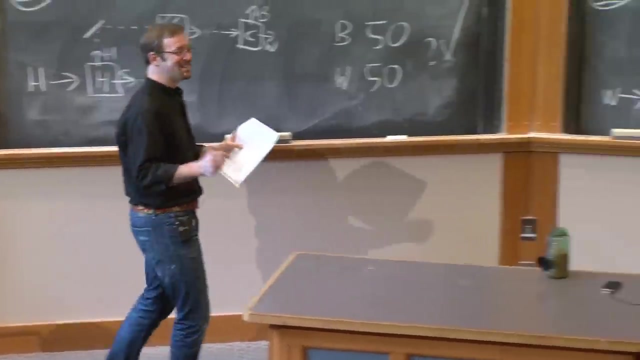 I would like to quote what a student just said, because it's actually the next line in my notes, which is what the hell is going on. So let's run a series of follow-up experiments to tease out what's going on here. 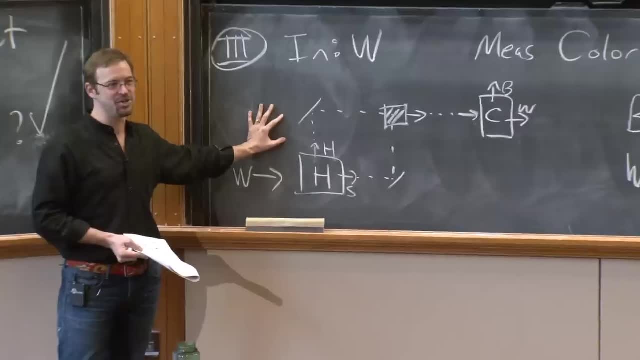 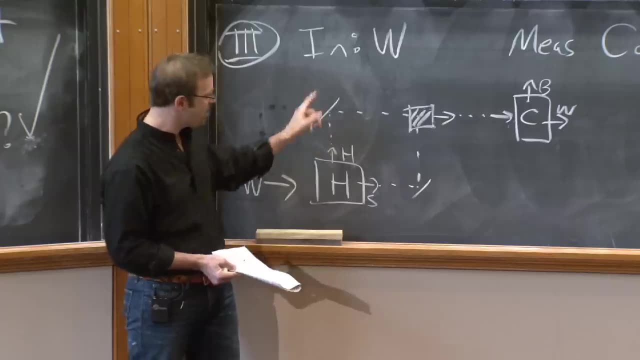 So something very strange, Let's just all agree. something very strange just happened. We sent a single electron in and that single electron comes out the hardness box. Well, it either came out the hardness box or it came out the softness. 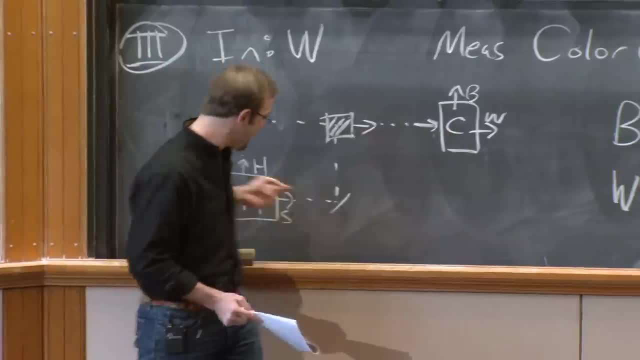 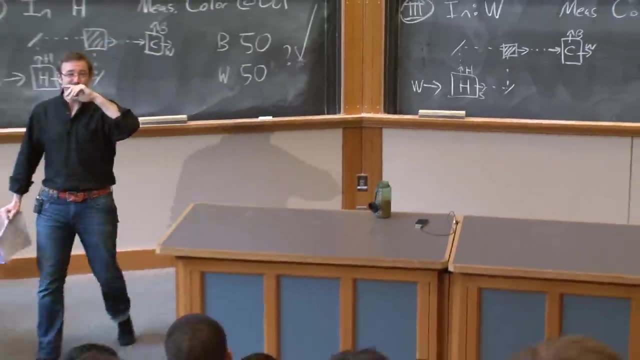 It either came out the hard aperture or the soft aperture, And if it came out the hard, we know what happens. If it came out the soft, we know what happens, And it's not 50-50.. So we need to improve the situation. 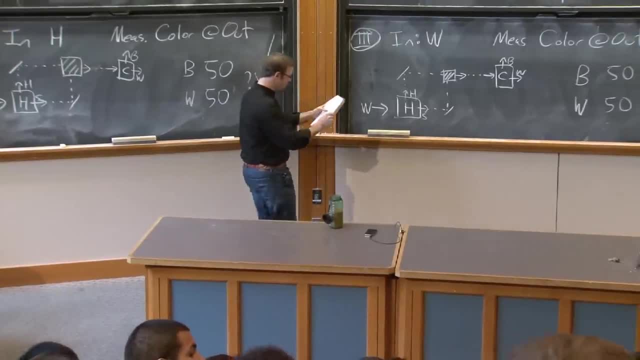 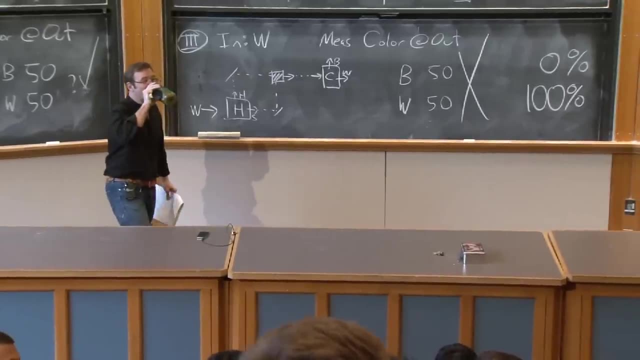 Hold on a sec. Hold on one sec, OK. So OK, go ahead. Yeah, I have a question about the setup. Yeah, So for the second hardness box, are we collecting both the soft and the hard aspects? The second: 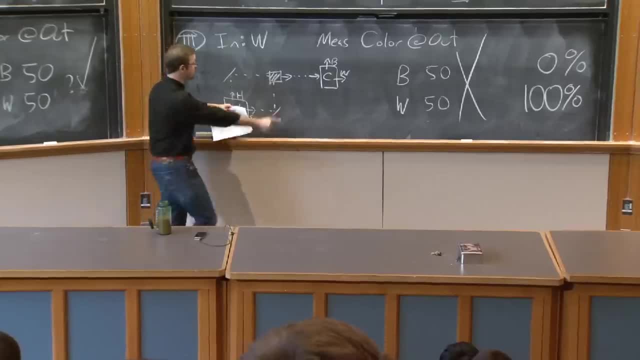 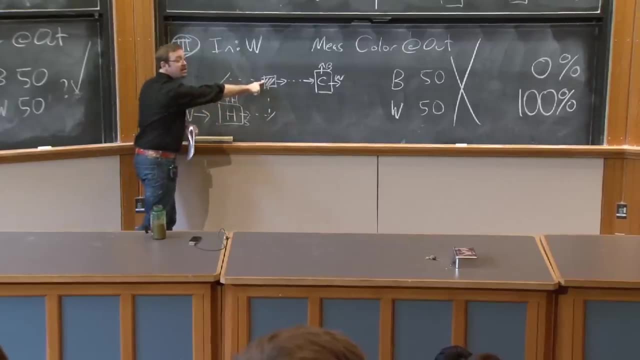 You mean the first hardness box, Or the one with the? This one? No, the Which one? Sorry, This series one, This guy? Yeah, Oh, that's a mirror, not a hardness box. So all this does is: oh, thanks for asking. 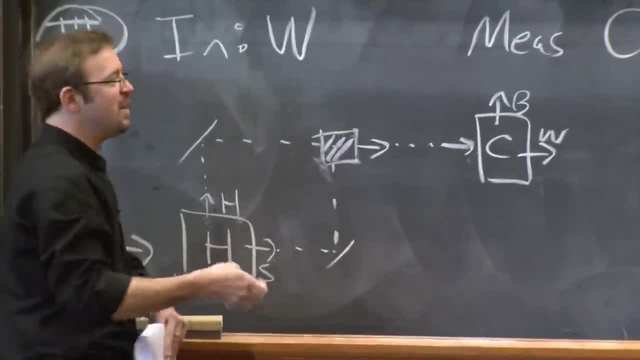 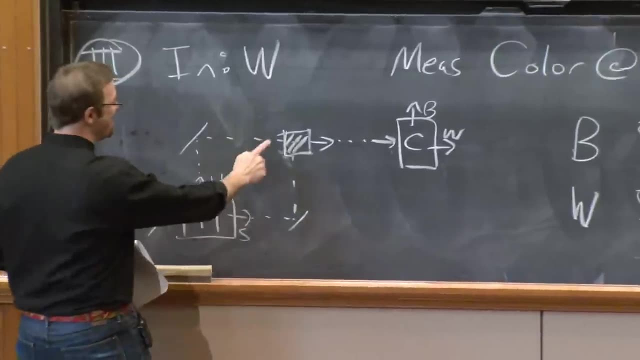 OK, yeah, sorry, I wish I had a better notation for this, but I don't. There's a classic. well, I'm not going to go into it. So remember that thing where I can't stop myself from telling stories. 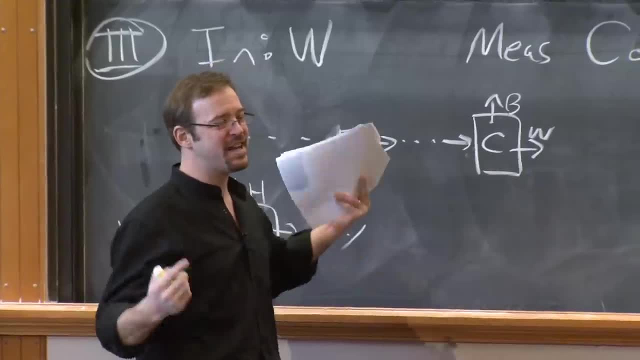 So all this does? it's just a set of mirrors, It's a set of fancy mirrors, And all it does is it takes an electron coming this way or an electron coming this way, and both of them get sent out in the same direction. 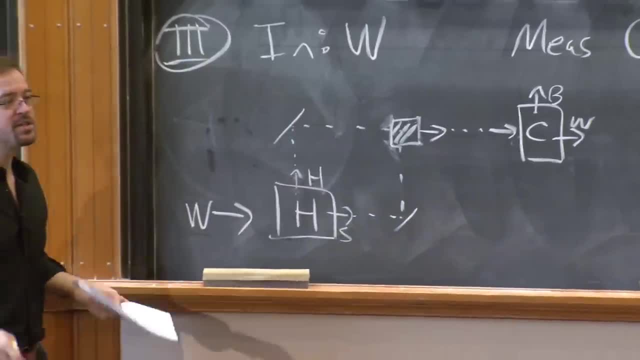 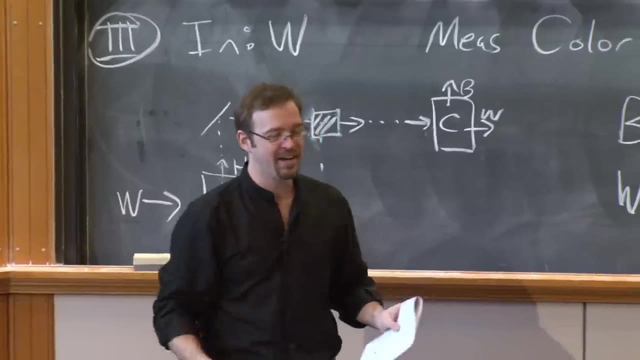 It's like a beam joiner, It's like a y-junction, That's all it is. So if you will imagine the box is a box and you take I don't know Professor's Weebok and you put him inside, 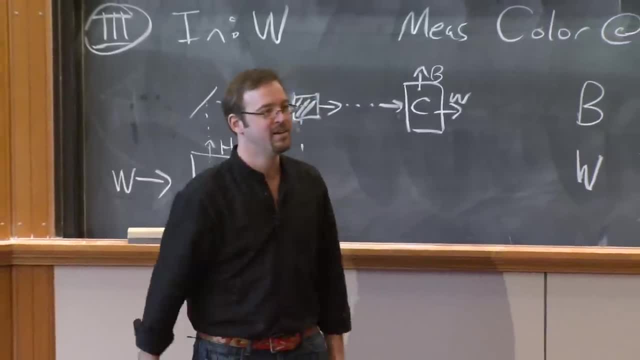 And every time an electron comes up this way, he throws it out that way. And every time it comes in this way, he throws it out that way, And he'd be really ticked at you for putting him in a box, but he'd do the job well. 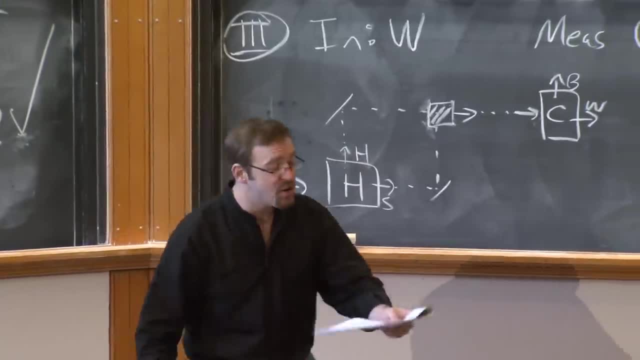 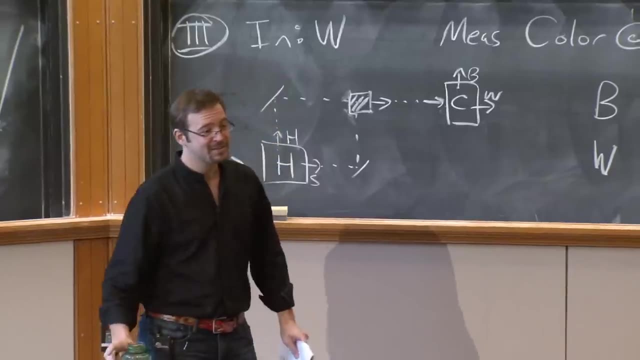 Yeah, And this also works. if you go one electron at a time, This works. if you go one electron at a time, This works. if you go 14 electrons at a time, It works. It works reliably. Yeah, Just maybe we spend just one second. 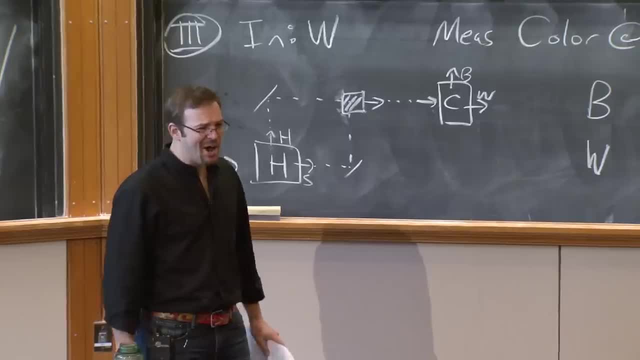 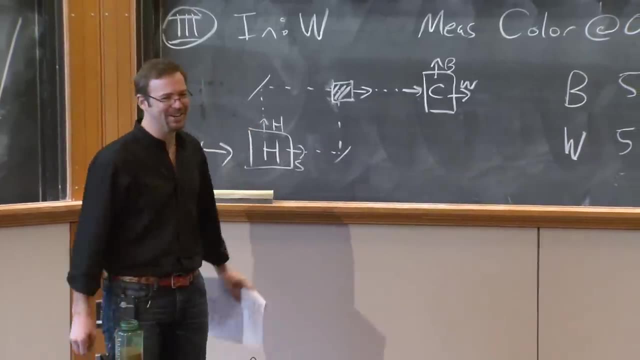 on: what's the difference between this experiment and that one? Yeah, I know, Right, Right, Yeah. So the question was: what's the difference between this experiment and the last one? Yeah, good question, So we're going to have to answer that. 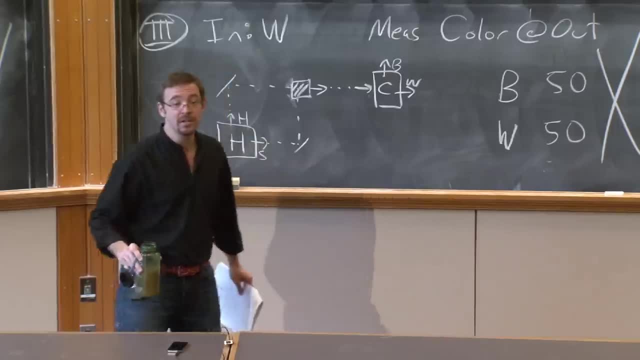 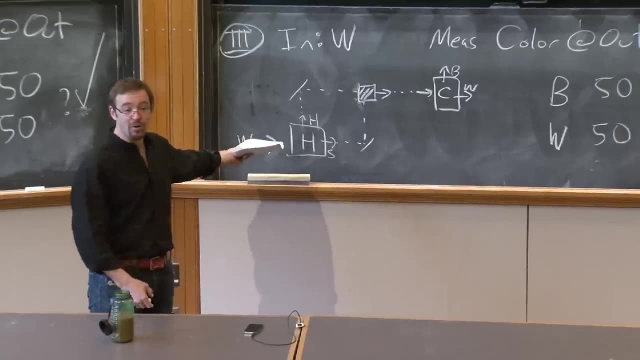 Yeah, Well, you're mixing again the harness. So it's like as you were measuring it. it's not white at all. right, Apparently, it's a lot like we were measuring it, Because we send in the white electron. 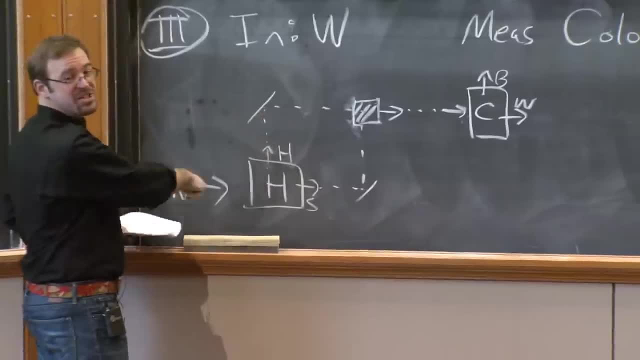 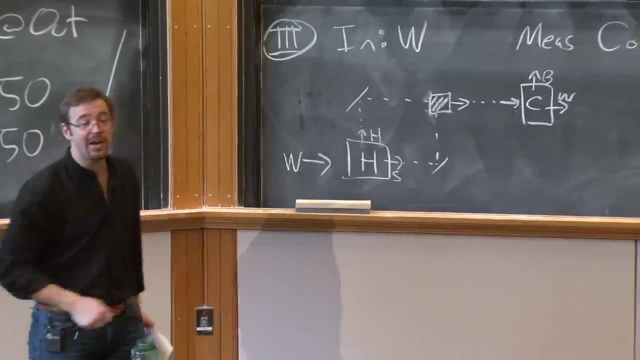 and at the end we get out that it's still white. So somehow this is like not doing anything. But how does that work? So that's an excellent observation, And I'm going to build you now a couple of experiments that tease out what's going on. 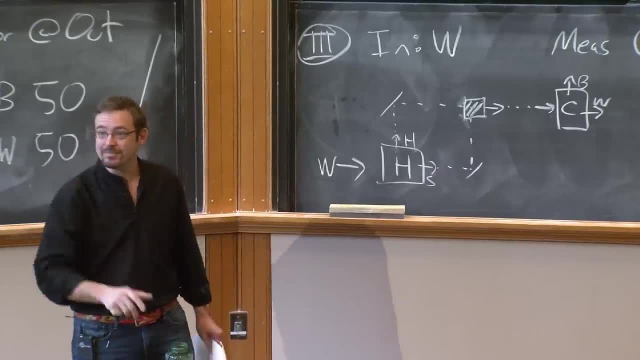 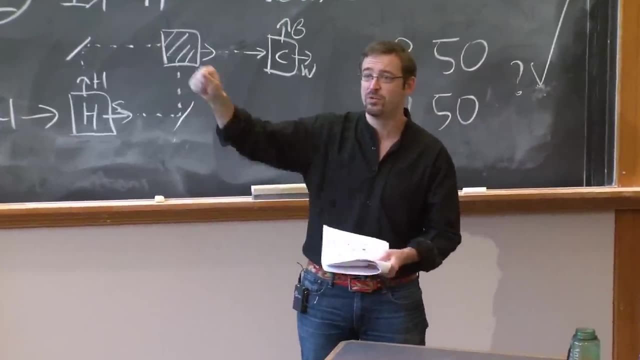 And you're not going to like the answer. Yeah, What were the white electrons that were generated in this experiment? The white electrons were generated in the following way: I take a random source of electrons, ie I rub a cat against a balloon and I charge it. 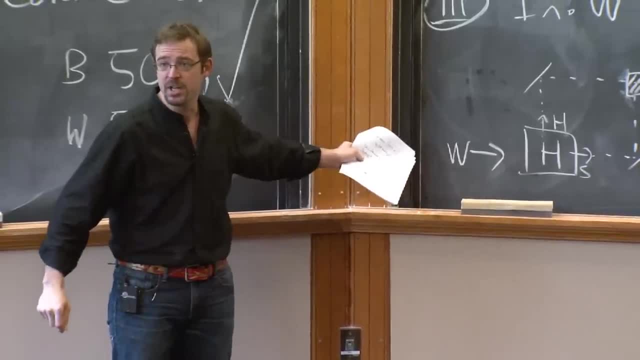 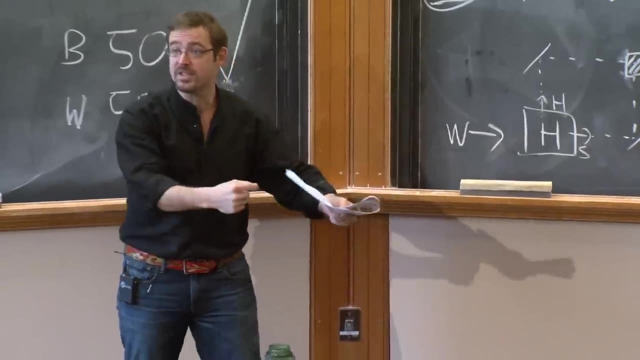 OK, And so I take those random electrons and I send them into a color box. And we have previously observed that if you take random electrons and throw them into a color box and pull out the electrons that come out, the white aperture, if you then send them into a color box again. 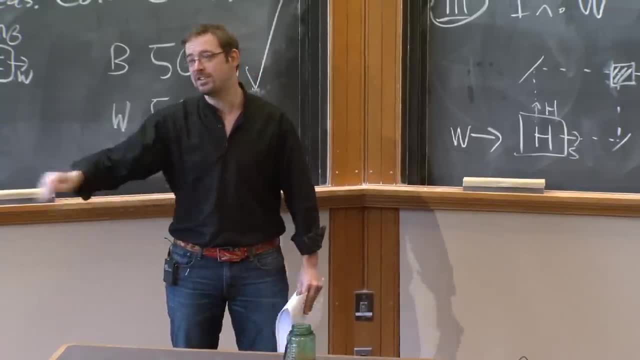 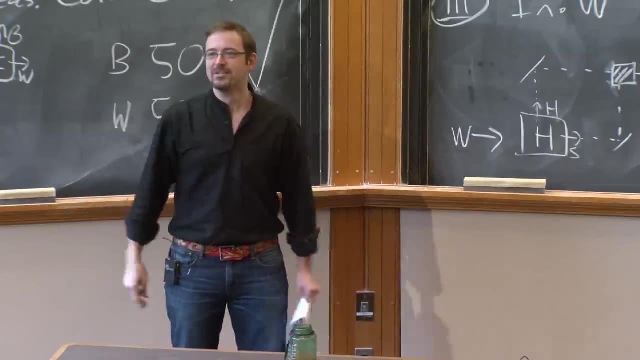 they're still white, So that's how I've generated them. I could have done it by rubbing the cat against glass or rubbing it against me right. Stroke the cat. But any randomly selected set of electrons sent into a color box and then from which you take the white electrons. 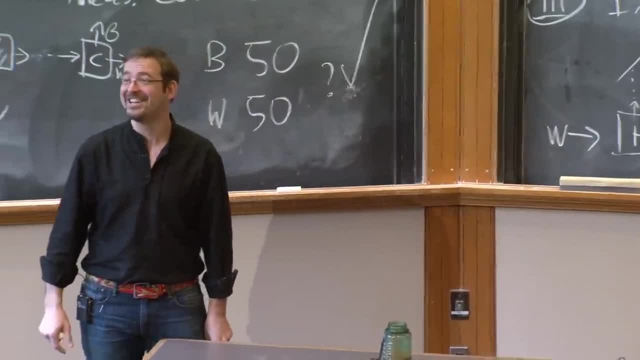 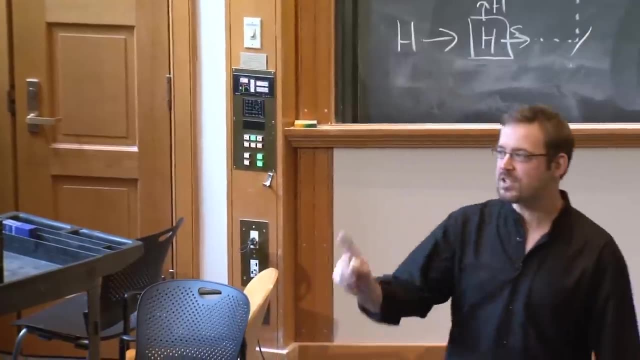 Yeah, Uh-huh, Exactly Yeah, It's the things that you never actually know about the electrons by yourself. That's a really good question. So here's something that I'm going to be very careful not to say in this class, to the degree. 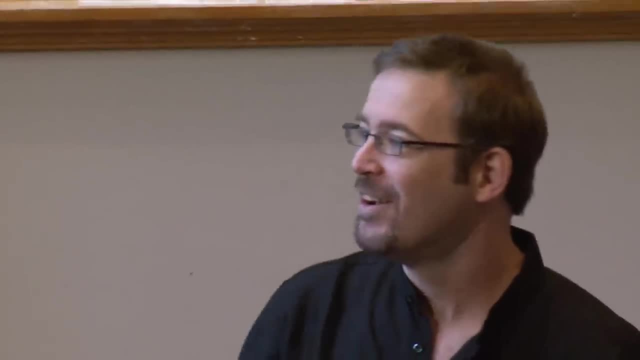 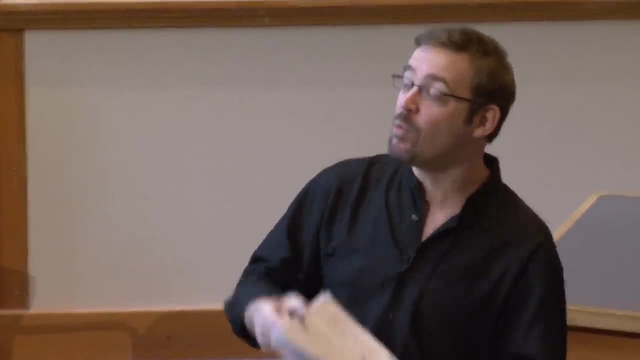 possible. I'm not going to use the word to know. Oh to measure. You get to know to measure. Good, Measure is a very slippery word too. I've used it here because I couldn't really get away with not using it. 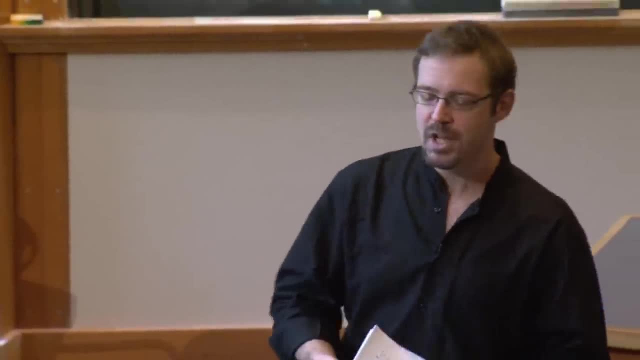 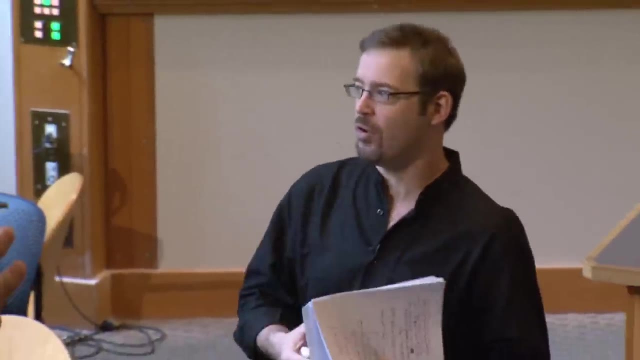 But we'll talk about that in great in some of the other some detail later on in the course. For the moment I want to emphasize that it's tempting but dangerous at this point to talk about whether you know or don't know, or whether someone knows or doesn't know. 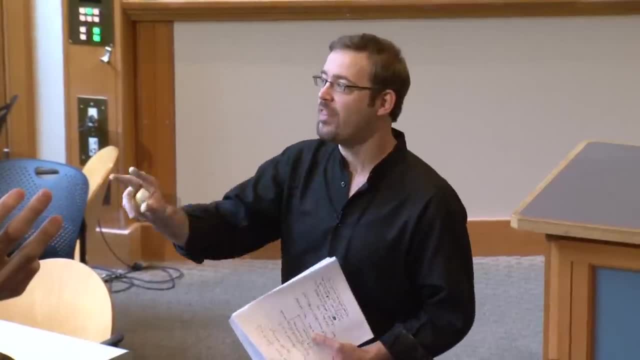 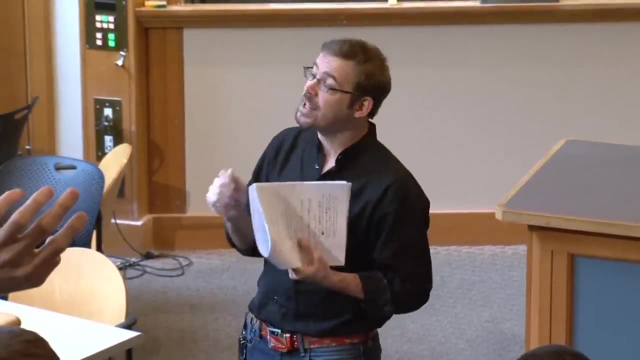 For example, the monkey inside knows or doesn't know. So let's try to avoid that and focus on just operational questions of what are the things that go in, what are the things that come out and with what probabilities. And the reason that's so useful is that it's something. 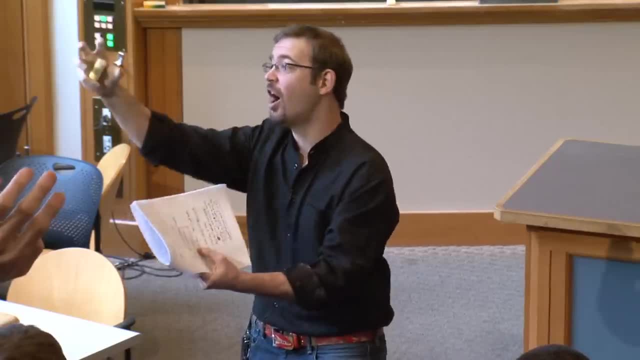 that you can just do. There's no ambiguity about whether you've caught a white electron in a particular spot. Now, in particular, the reason that it's so useful in this case, The reason these boxes are such a powerful tool, is that you don't measure the electron. 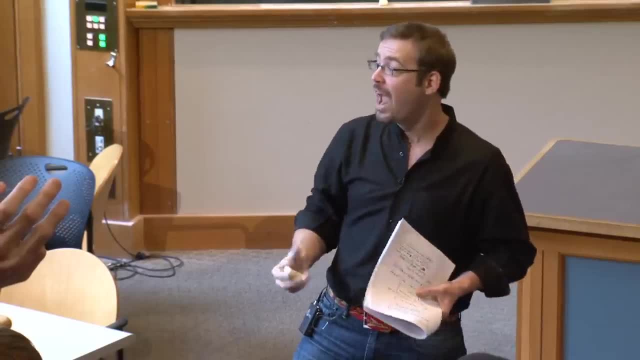 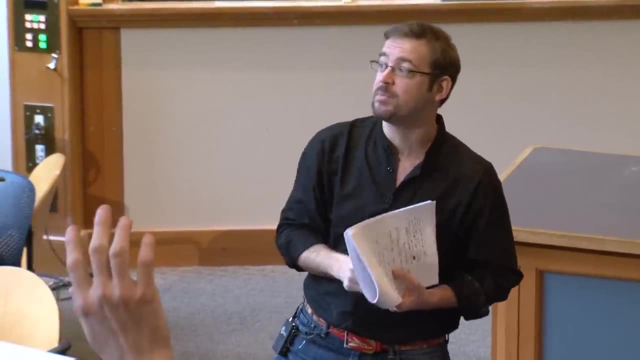 you measure the position of the electron. You get hit by the electron or you don't. And by using these boxes we can infer from their position the color or the hardness, And that's the reason these boxes are so useful. So we're inferring from the position. 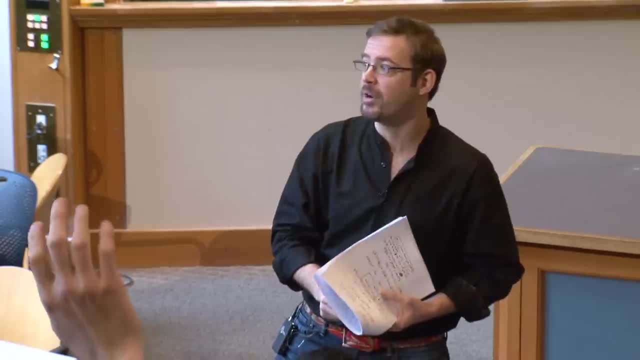 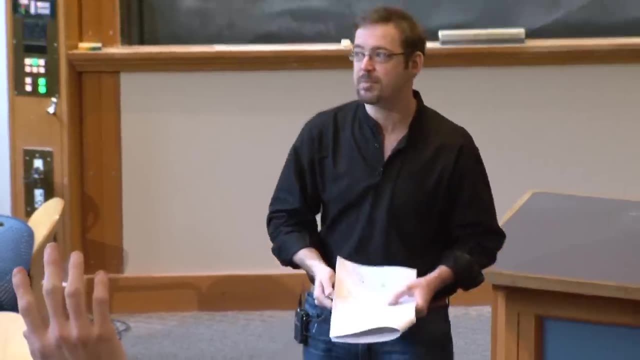 which is easy to measure. if you get beamed or you don't, We're inferring the property that we're interested in. So it's a really good question, though Keep it in the back of your mind and we'll talk about it on and off for the rest of the semester. 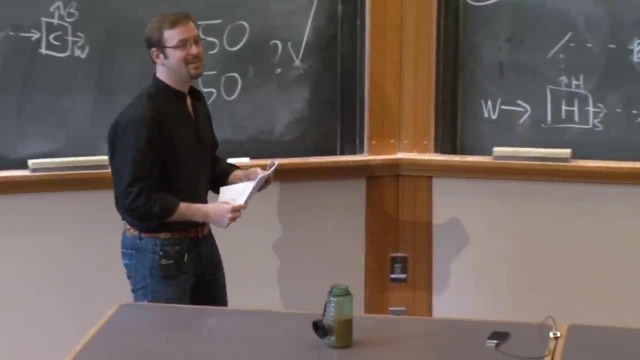 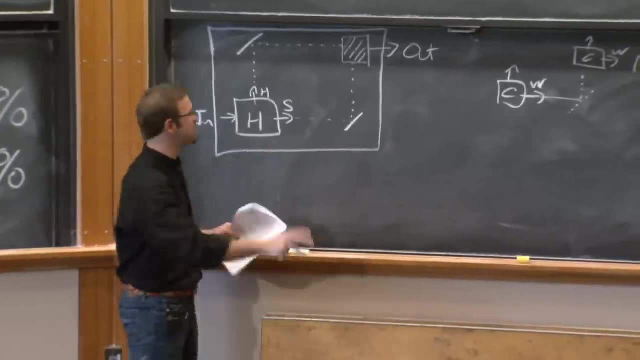 Yeah, So what happens if you have the setup and you just take away the bottom right here? Perfect question. OK, this leads me into the next experiment. So here's the modification that. thank you, That's a great question. Here's a modification of this experiment. 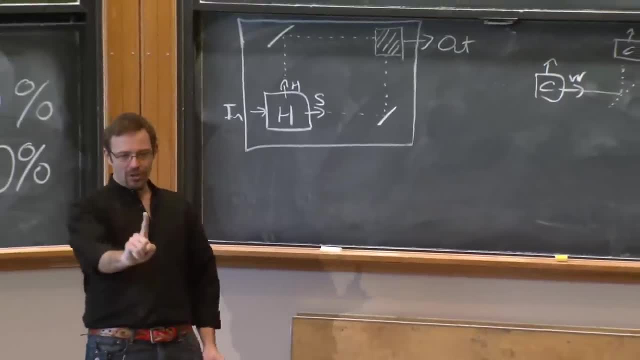 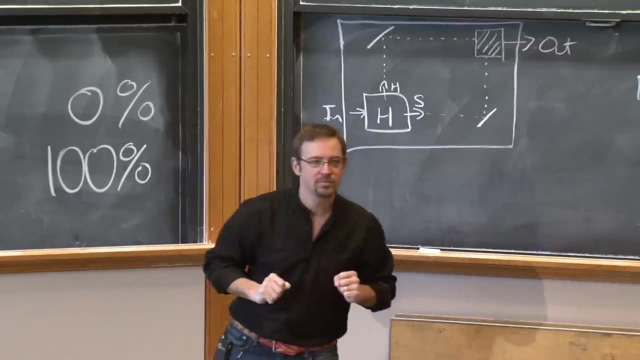 So let's rig up a small hold on. I want to go through the next series of experiments and then I'll come back to questions, And these are great questions. So I want to rig up a small movable wall. A small movable wall. 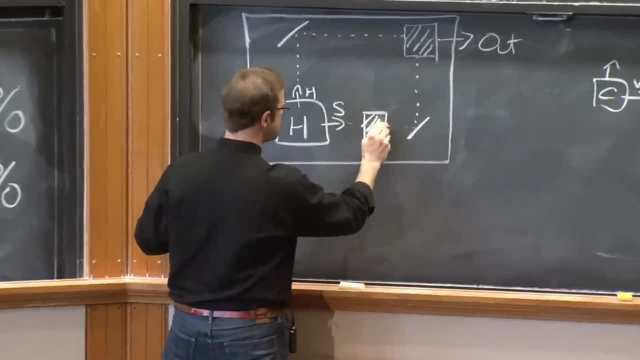 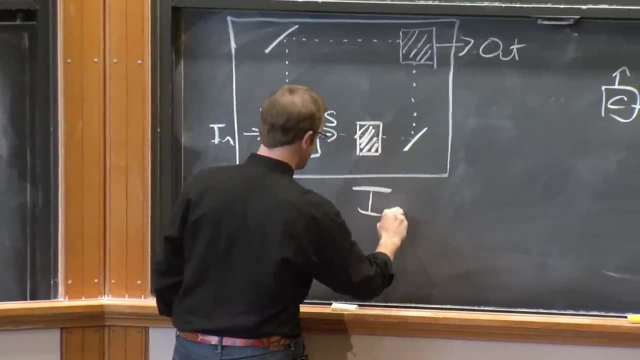 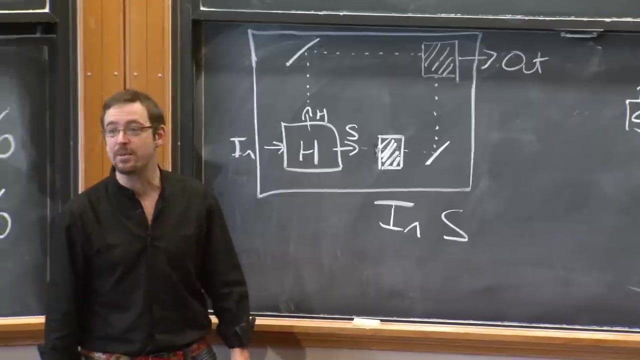 A movable barrier. And here's what this movable barrier will do. If I put the barrier in so this would be in the soft path. When I put the barrier in the soft path, it absorbs all electrons, incident upon it and impedes them from proceeding. 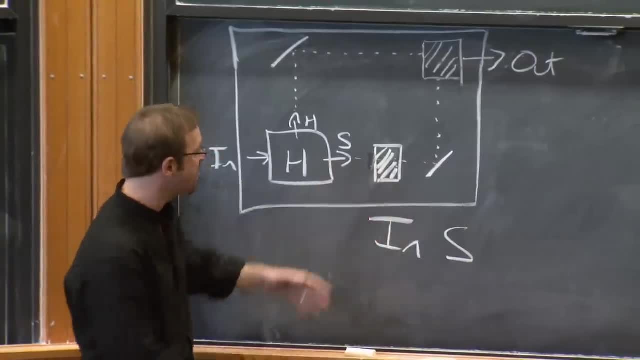 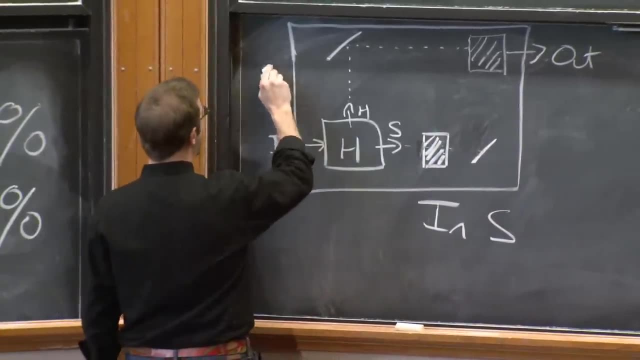 So you put a barrier in here. we put our barrier in the soft path. no electrons continue through it. An electron incident cannot continue through it. OK, When I say that the barrier is out, what I mean is it's not in the way. 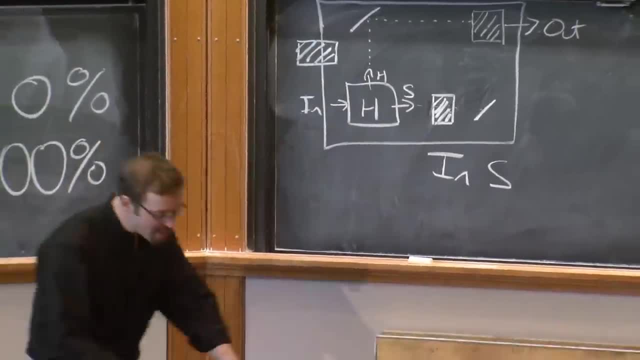 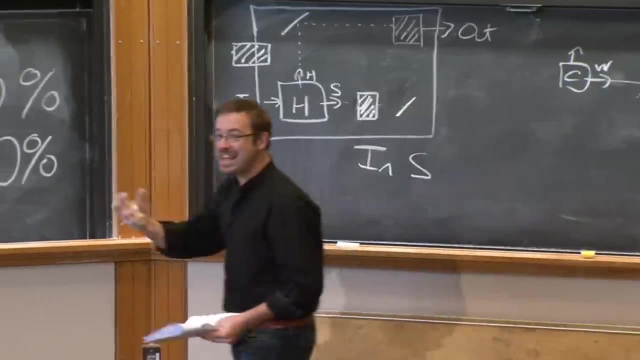 I've moved it out of the way, Cool. So I want to run the same experiment, And I want to run this experiment in the following way: I'm going to run the experiment using the barriers to tease out how the electrons transit through our apparatus. 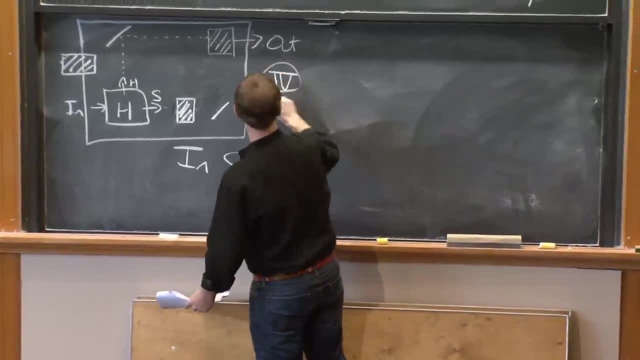 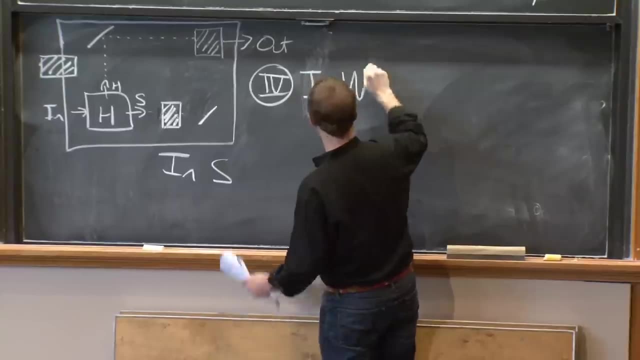 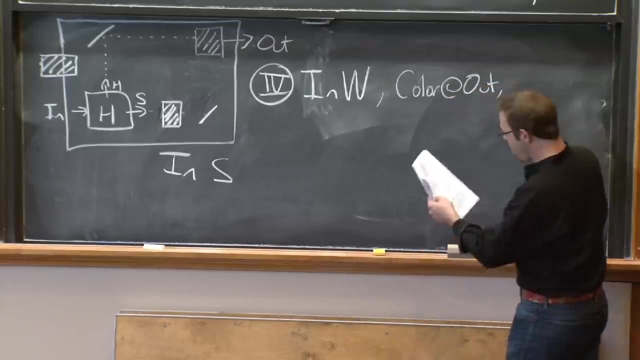 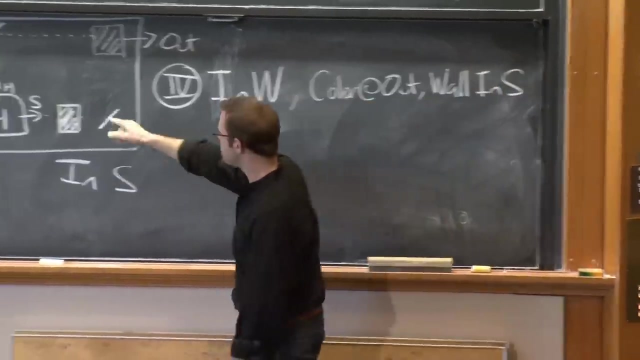 OK. So experiment four: Let's send in a white electron again. I want to do the same experiment we just did And color at out, but now with a wall in the south path, Wall in soft. OK, So that's this experiment. 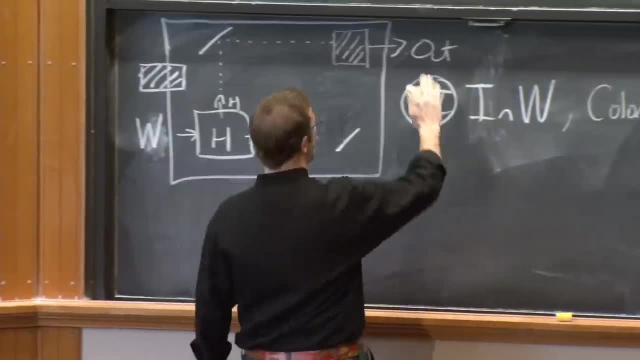 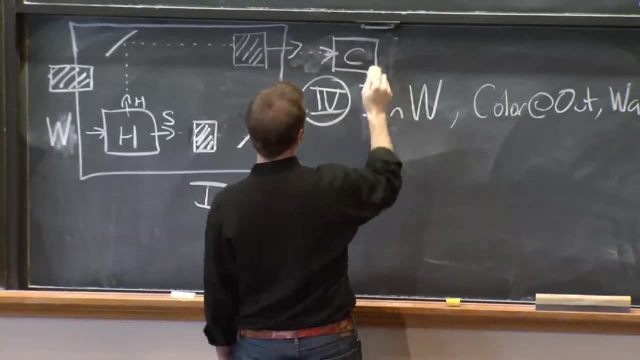 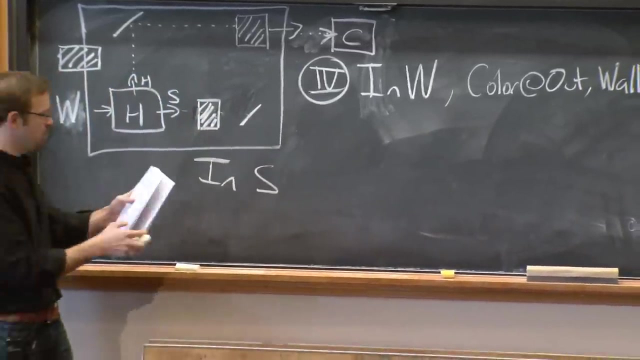 So we send in white electrons And we send out Soft Soft And at the output we measure the color, as before, And the question is what fraction come out? What fraction come out Black And what fraction come out? 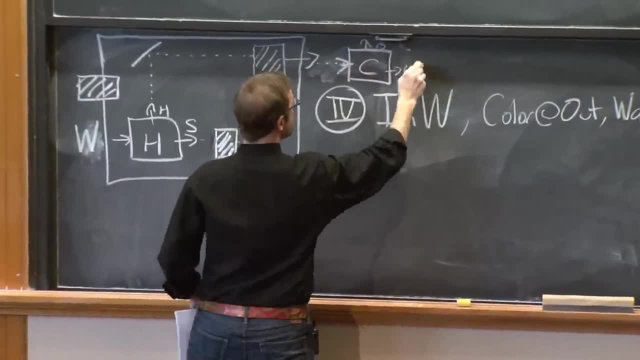 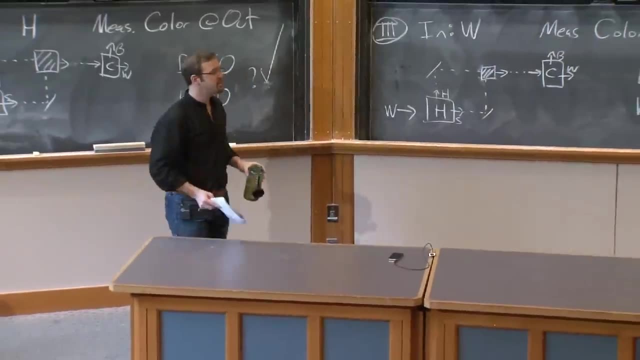 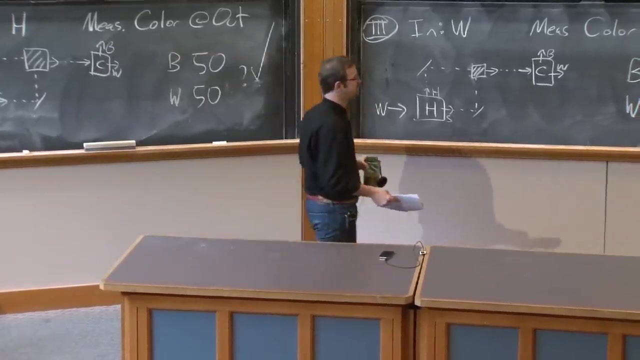 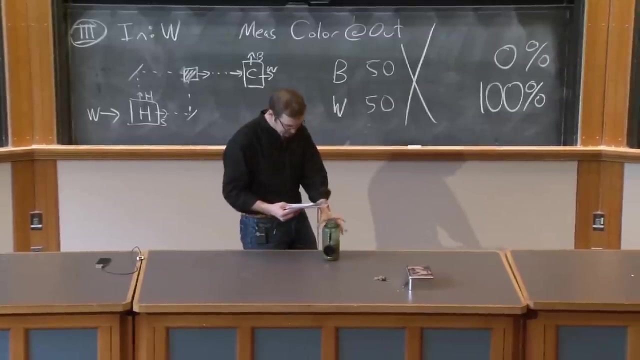 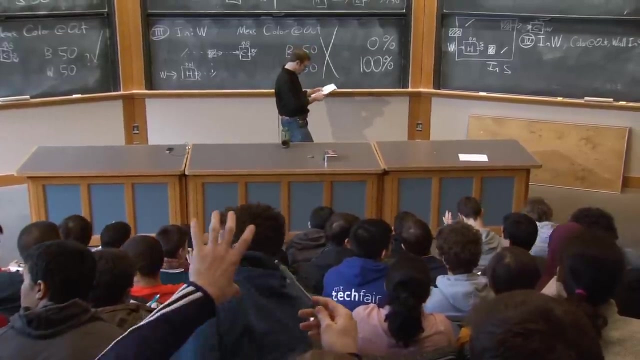 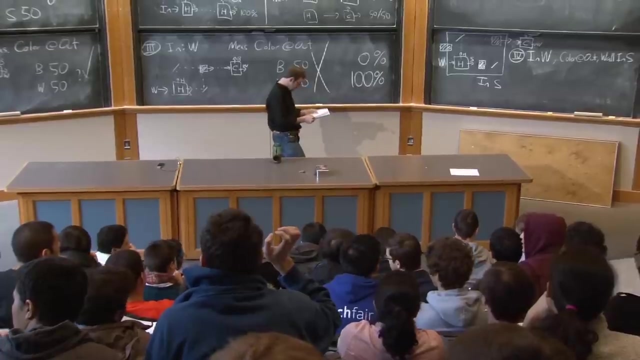 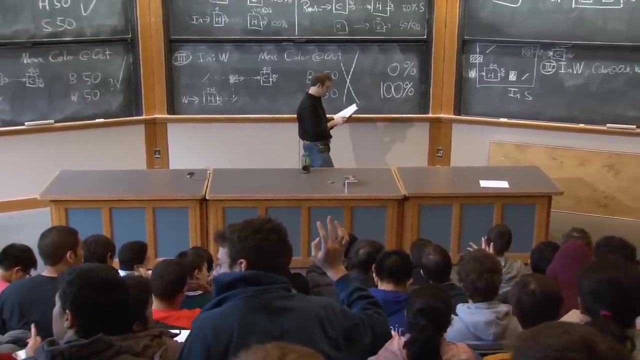 White. OK, So again, everyone think through it for a second. Just take a second, And this one's a little sneaky, So just feel free to discuss it with the person sitting next to you. OK, Just take a second and you're welcome to use your phone. 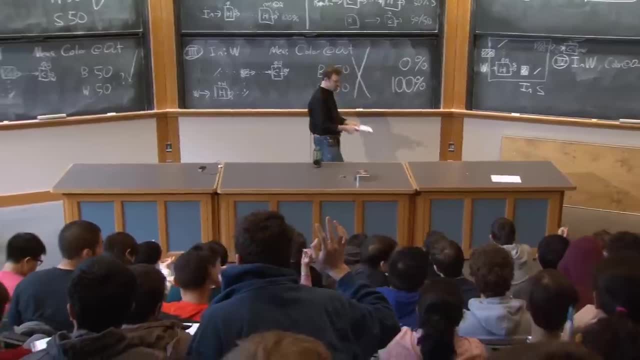 Just take a second And then we're going to come back to the next experiment. OK, OK, OK, All right. So let's go ahead and start And we're going to have a quick test run And I'm going to say: OK. 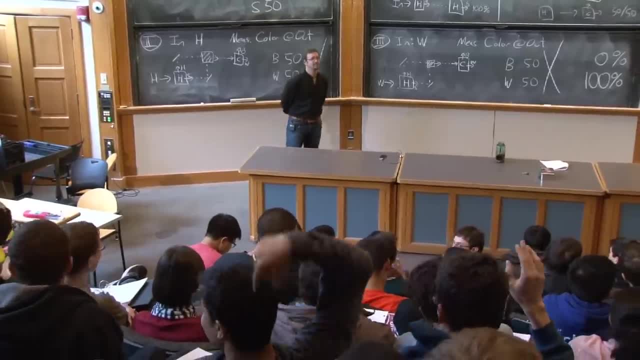 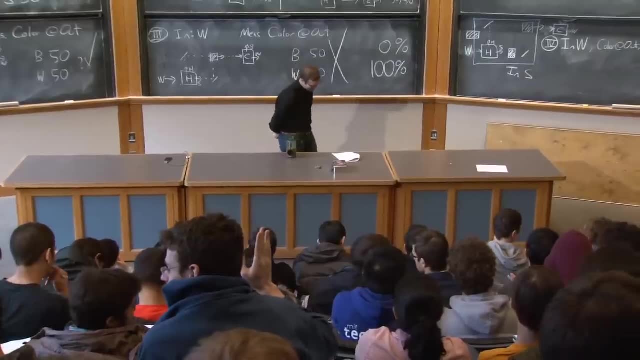 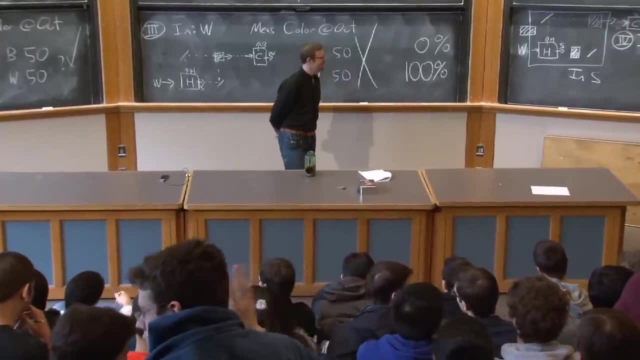 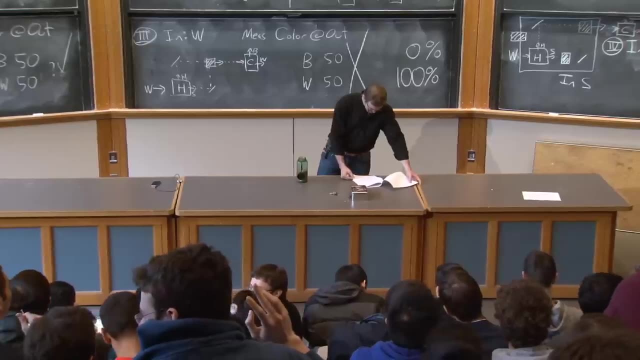 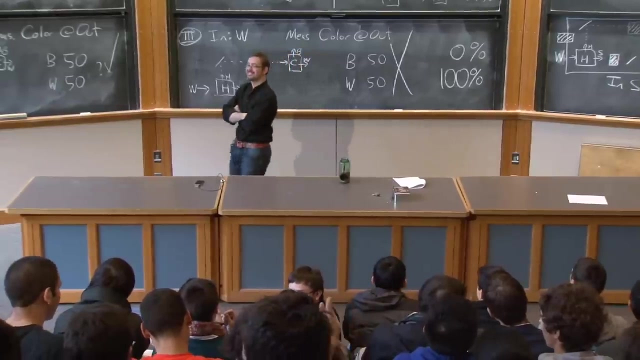 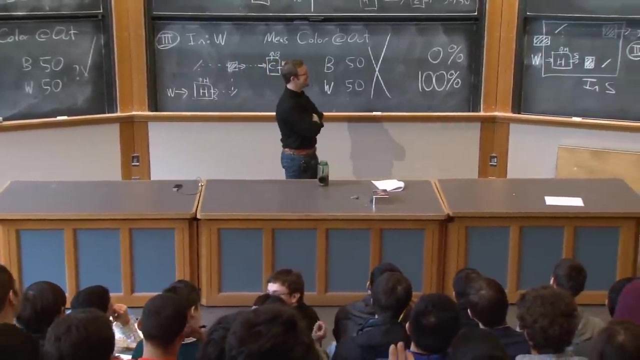 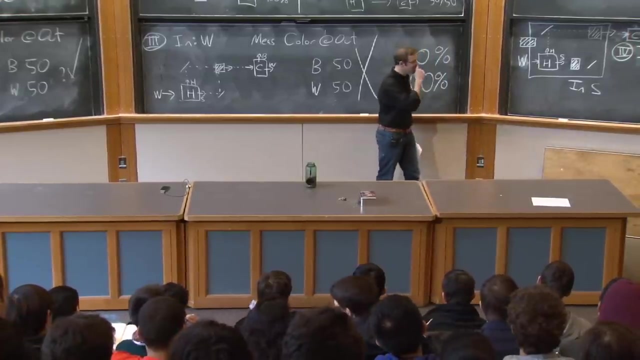 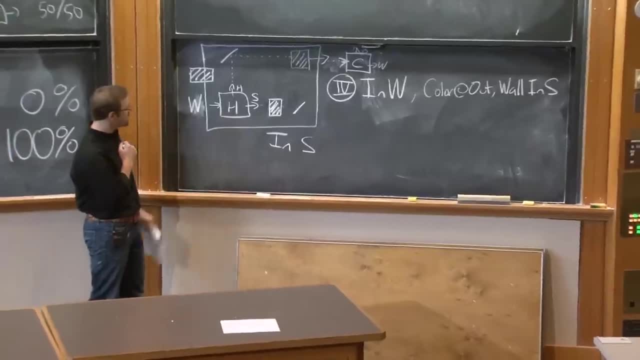 So the first thing I expect is that, look, if I send in a white electron and I put it in a hardness pass, I know that 50% of the time it goes out hard and 50% of the time it goes out soft. 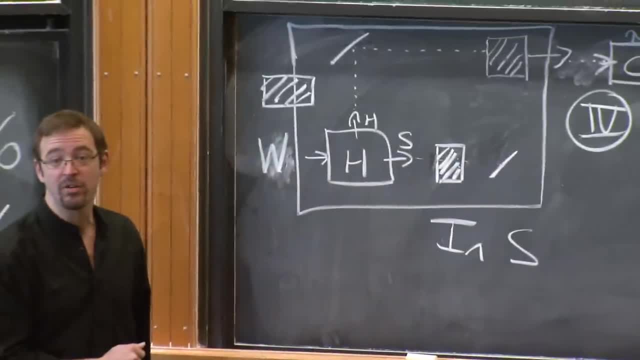 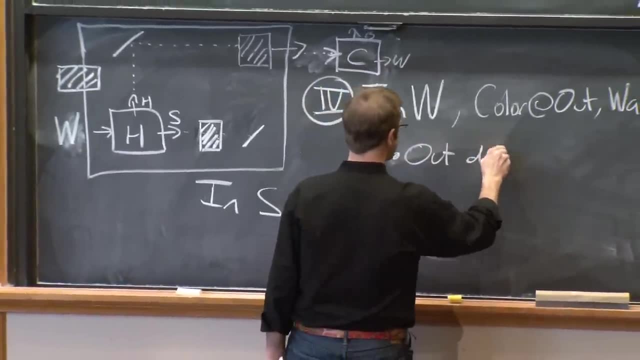 If it goes out the soft aperture, it's going to get eaten by the barrier. Right, It's going to get eaten by the barrier. So first thing I predict is that the output should be down by 50%. However, here's an important bit of physics: 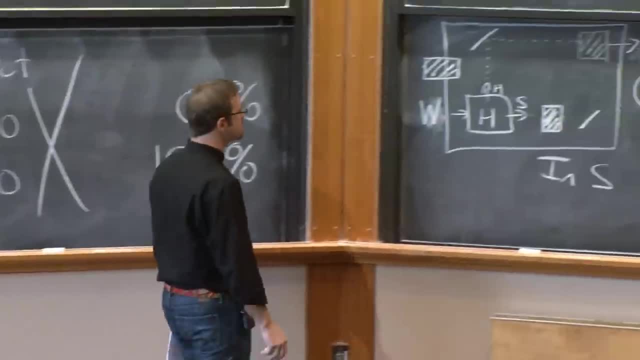 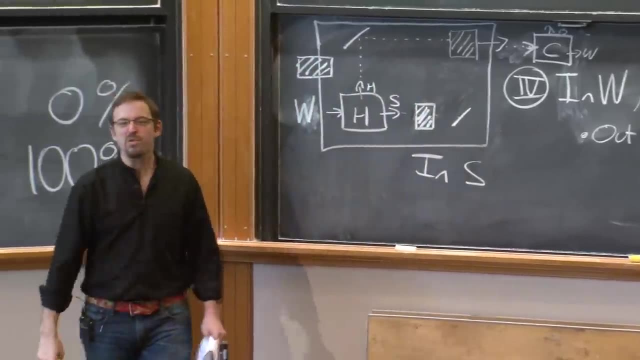 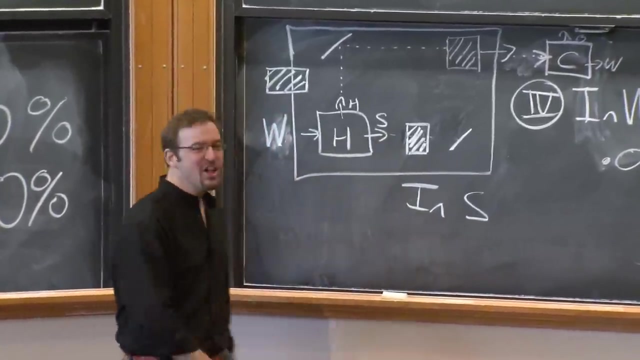 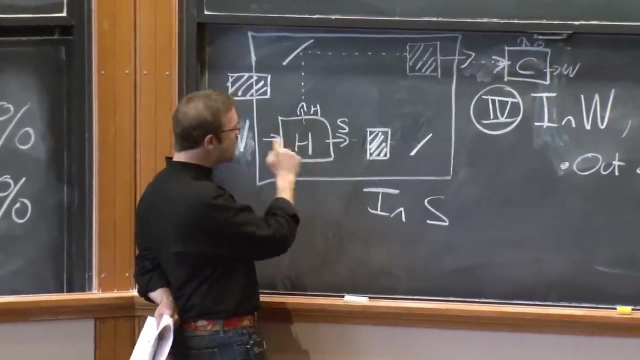 And this comes to the idea of locality. I didn't tell you this, but these arm lengths- in the experiment I did, 3,000 kilometers long. 3,000 kilometers long, That's too minor. 10 million kilometers long, really long, very long. 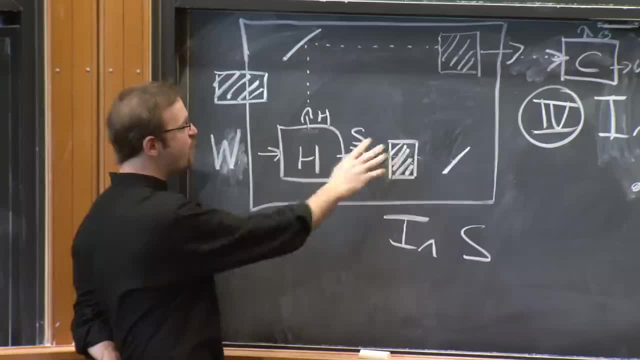 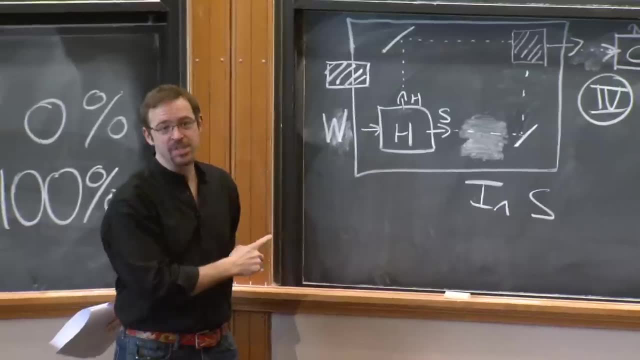 Now imagine an electron that enters this, an initially white electron. If we had the barriers out. if the barrier was out, what do we get? 100% white, right, We just did this experiment to our surprise. So if we did this, we get 100%. 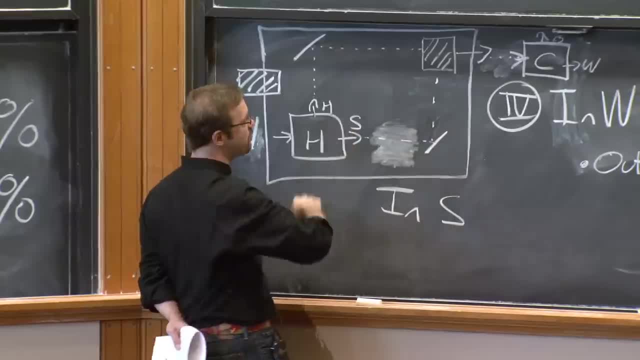 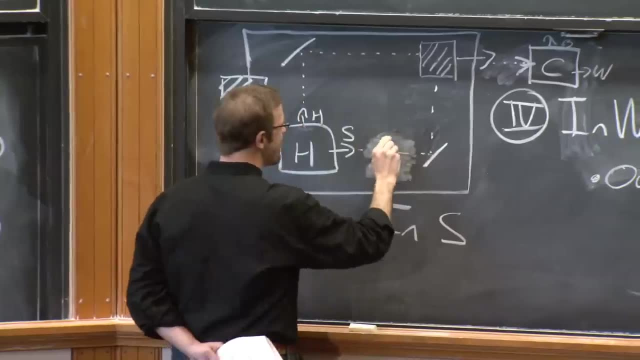 That means that any electron going along the south pass comes out white. Any electron going along the hard path goes out white. They all come out white. So now imagine I do this, Imagine I put a barrier in here, 2 million miles away from this path. 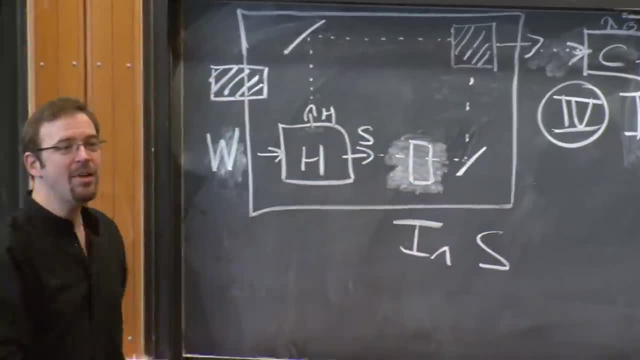 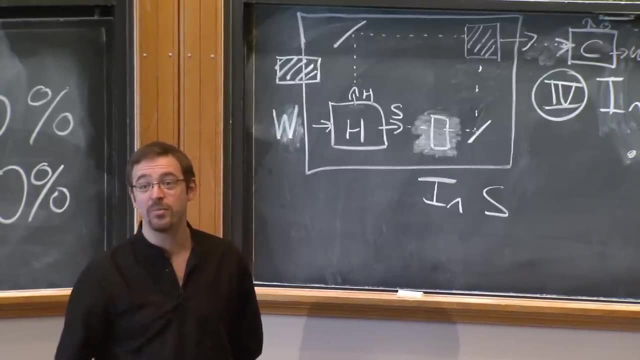 How does a hard electron along this path know that? I put the barrier there And I'm going to make it even more sneaky for you. I'm going to insert the barrier along the path after I launch the electron into the apparatus And when I send in the electron I 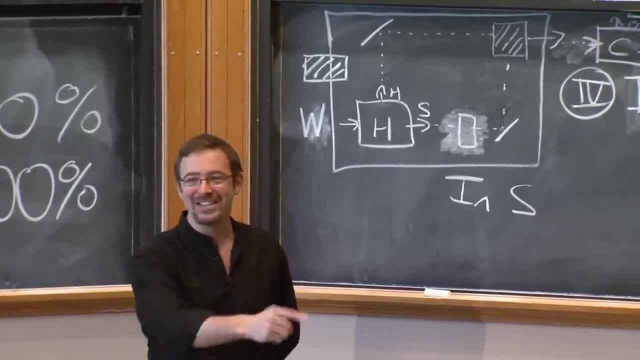 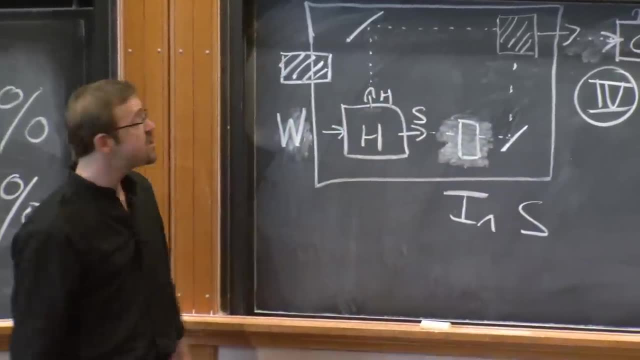 will not know at that moment whether, nor will the electron know, because they're not very smart- whether the barrier is in place, And this is going to be millions of miles away from this guy, So an electron out here can't know. 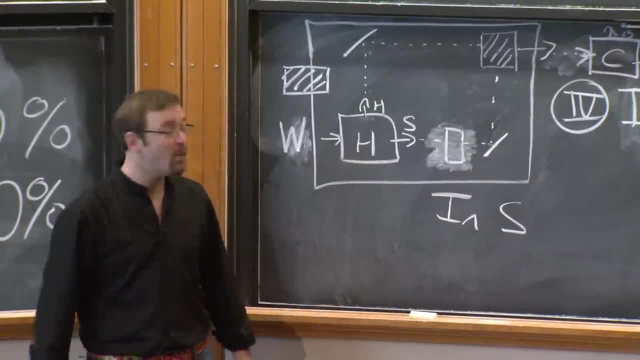 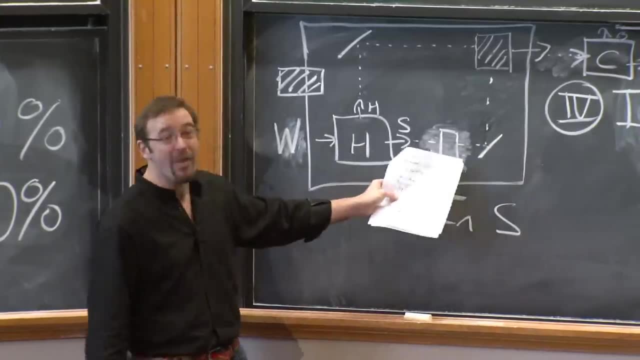 It hasn't been there. It just hasn't been there. It can't know. But we know that when we ran this apparatus without the barrier in there it came out 100% white. But it can't possibly know whether the barrier's in there. 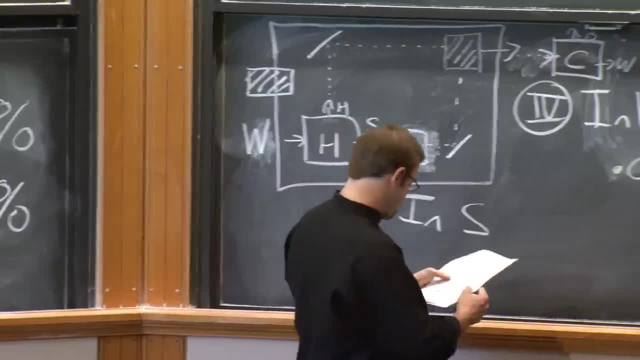 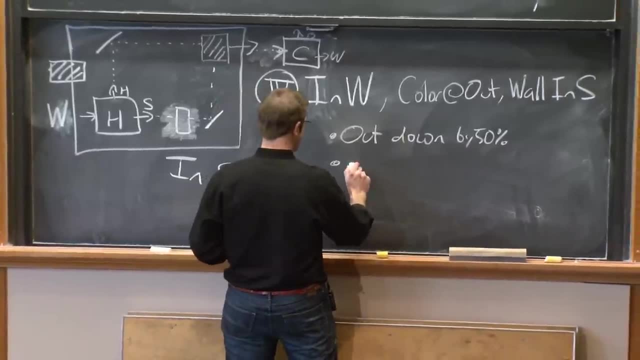 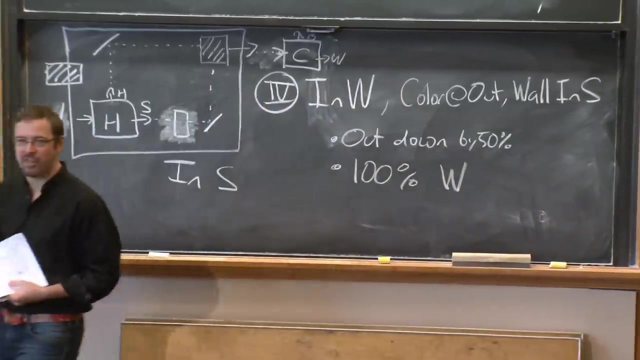 or not, It's over here. So what this tells us is that we should expect the output to be down by 50%, But all the electrons that do make it through must come out white, because they didn't know that there was a barrier there. 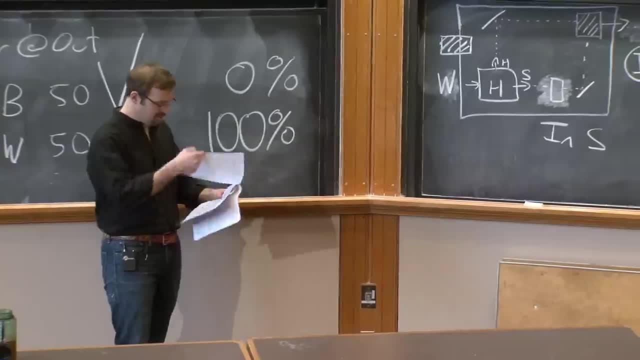 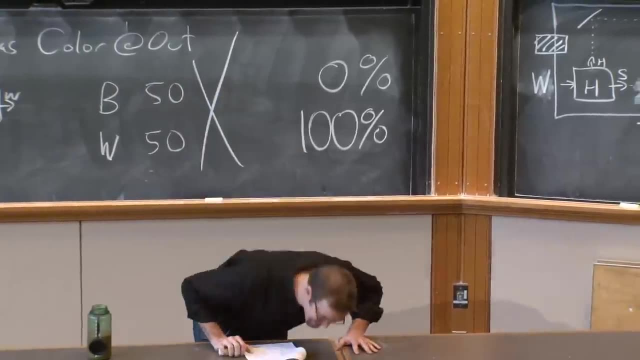 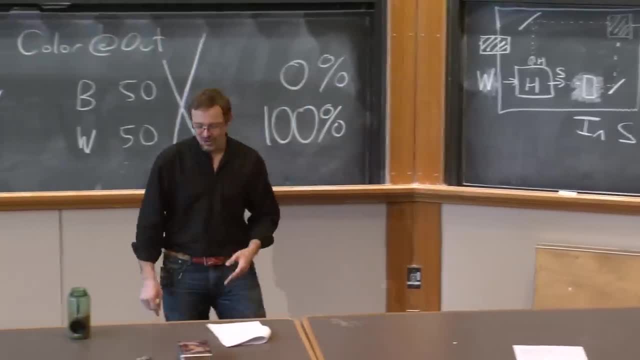 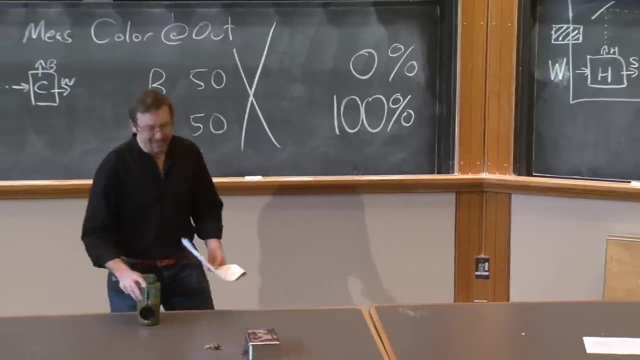 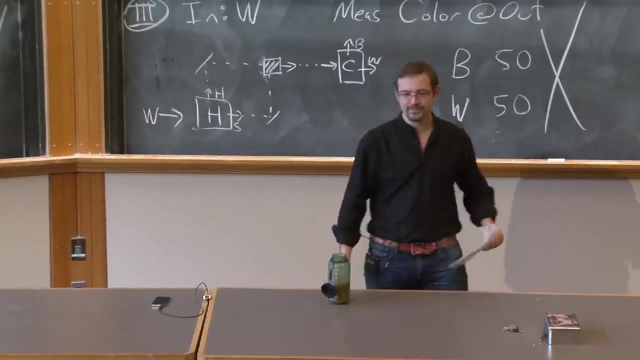 I was making fun of the electron. So in that particular case I was not referring to my or your knowledge. I was referring to the electron's tragically impoverished knowledge. Yeah Well, but if they come out 100% white, then wouldn't we know then that the electrons both are? 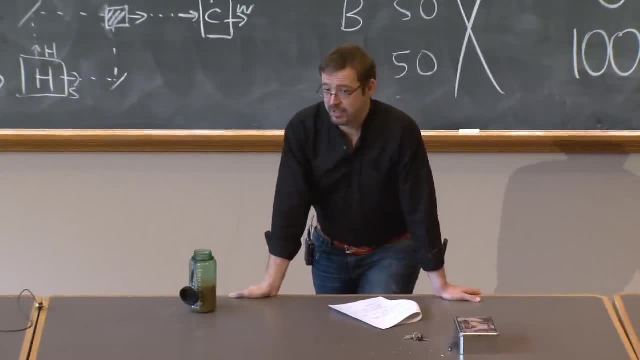 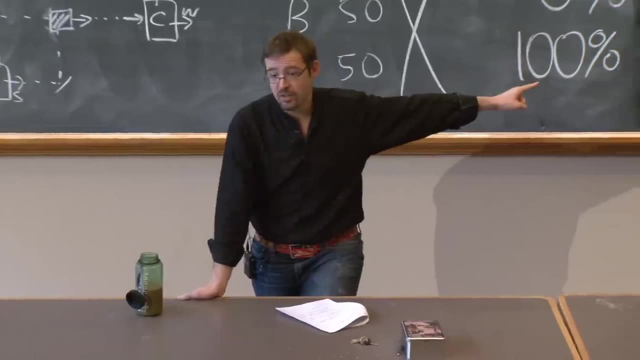 white, It's like a violet. Yeah Well, here's the more troubling thing. Imagine it didn't come out 100% white. Then the electron would have demonstrably not gone along the soft path, It would have demonstrably gone through the hard path. 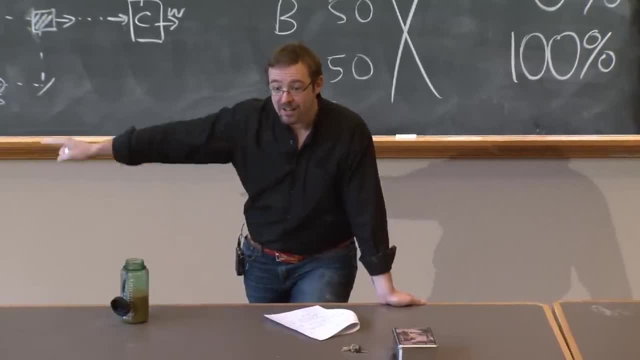 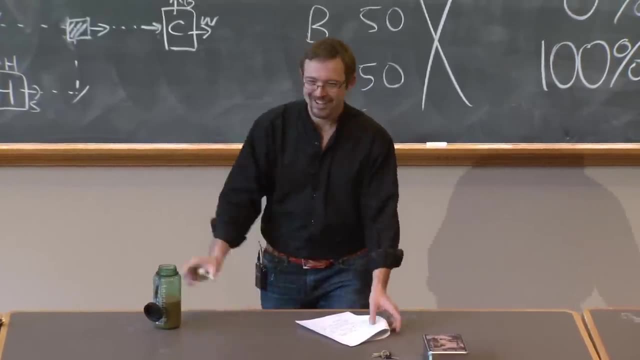 because that's the only path available to it. And yet it would still have known that millions of miles away there's a barrier on a path it didn't take. So which one's more upsetting to you? And personally I find this one the less upsetting of the two. 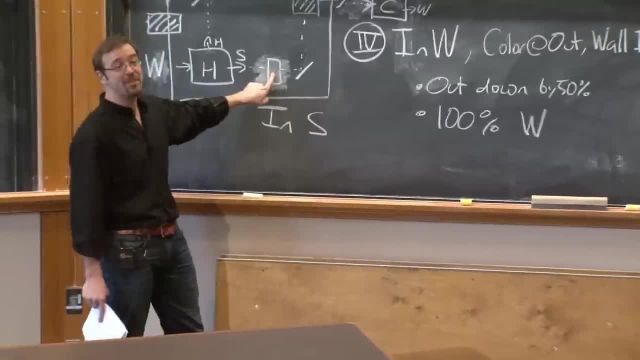 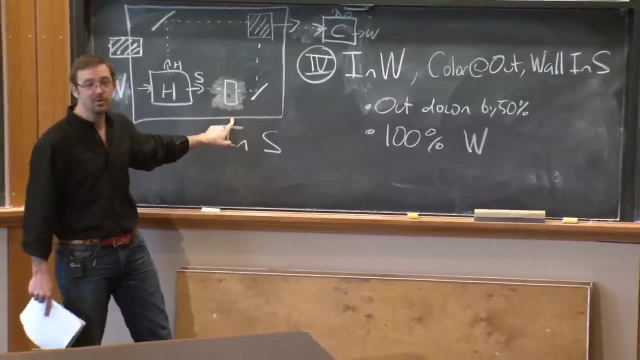 OK, So the prediction is our output should be down by 50%, because half of them get eaten, But they should all come out white, because those that didn't get eaten can't possibly know that there was a barrier here, Millions of miles away. 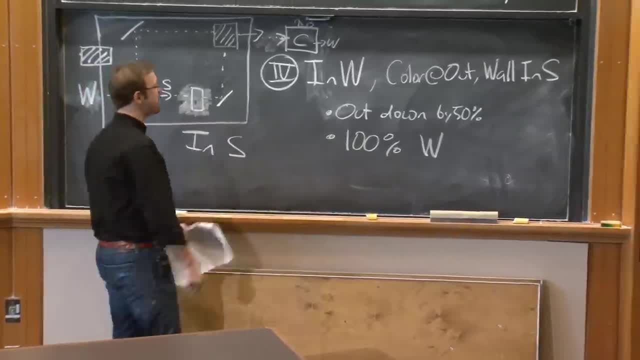 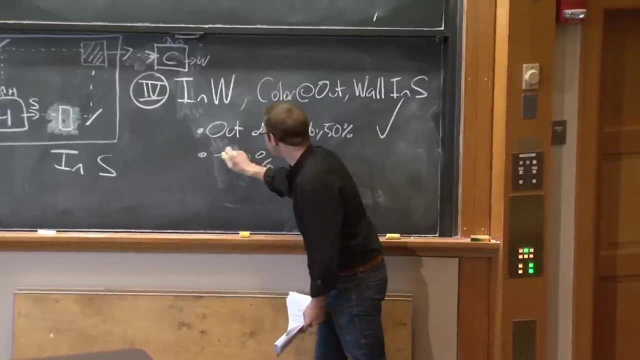 OK, So we run this experiment and here's the experimental result. In fact, the experimental result is: yes, the output is down by 50%, but no, not 100% white, 50% white, 50% white. 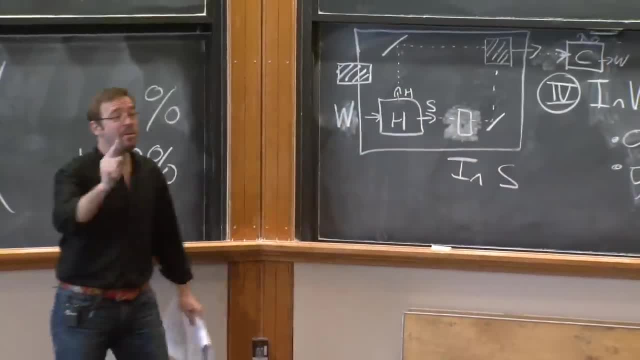 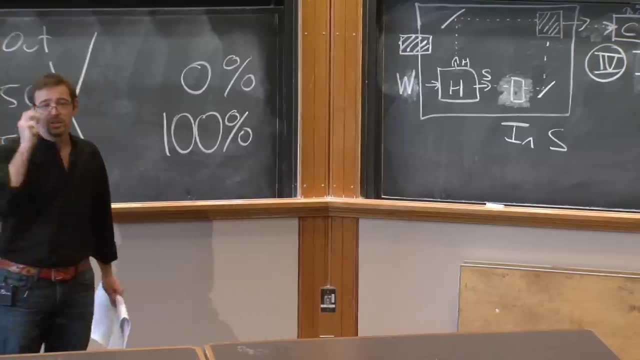 The barrier, if we put the barrier in the hardness path, If we put the barrier in the hardness path still down by 50% and it's at odds 50-50.. How could the electron know I'm making fun of it? 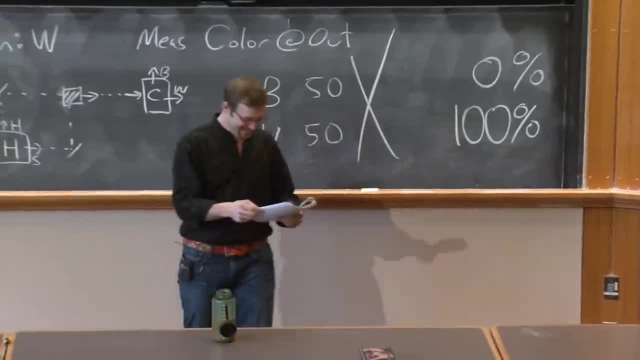 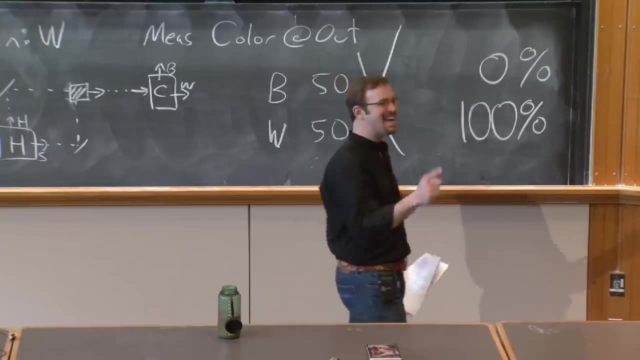 Yeah, I guess my question is before we asked how it knows there's a plot in one of the paths, how did it know before over there that there were two paths that combined them? Excellent, Exactly. So actually this problem was there already. 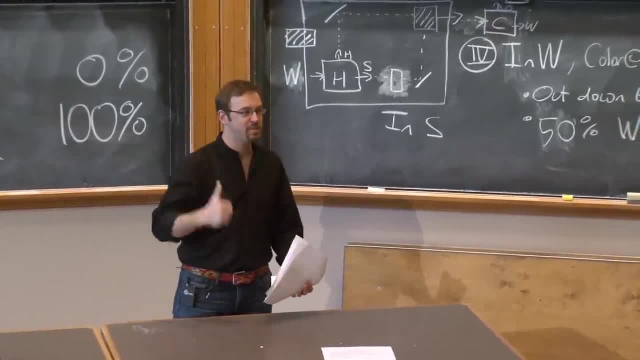 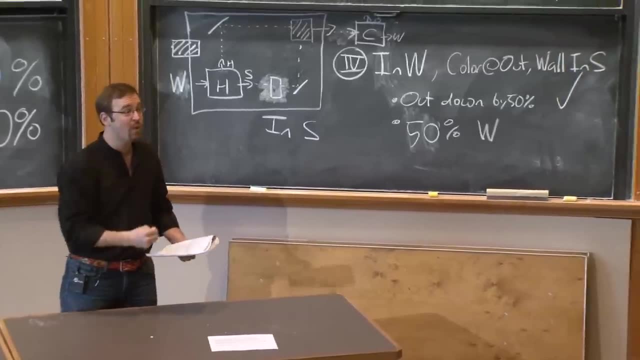 in the experiment we did. All we've done here is tease out something that was existing in the experiment, something that was disturbing. The presence of those mirrors and the option of taking two paths somehow changed the way the electron behaved. How is that possible? 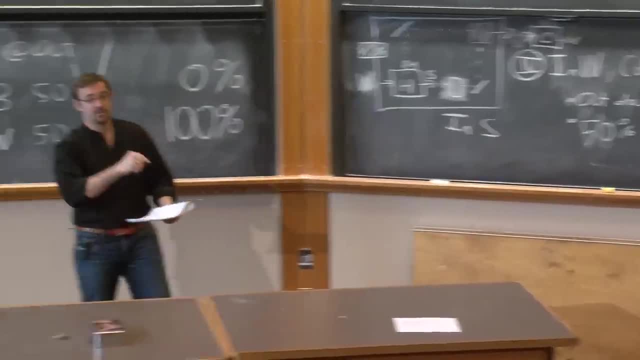 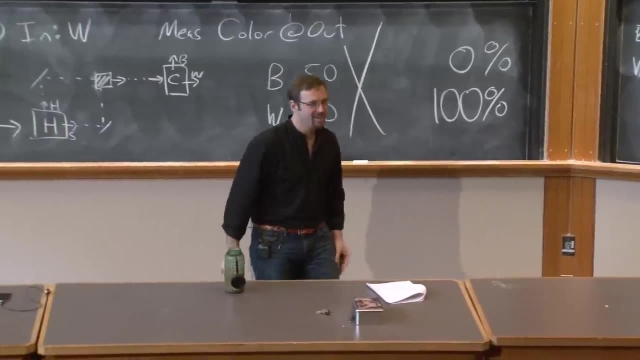 And here we're seeing that very sharply. Thank you for that excellent observation. Yeah, What if you replaced the two mirrors with color boxes, so that one, like both color boxes, had their hard or soft, and then you would refine all the organs and then put it in that last color box. 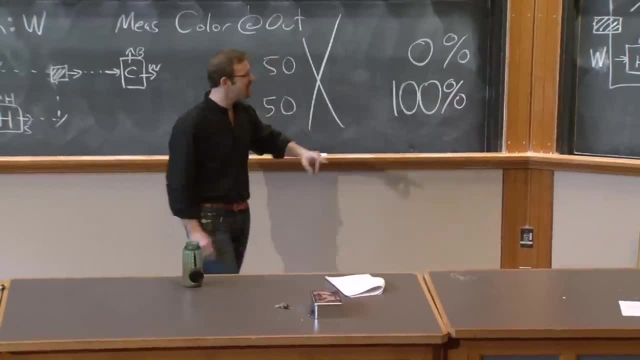 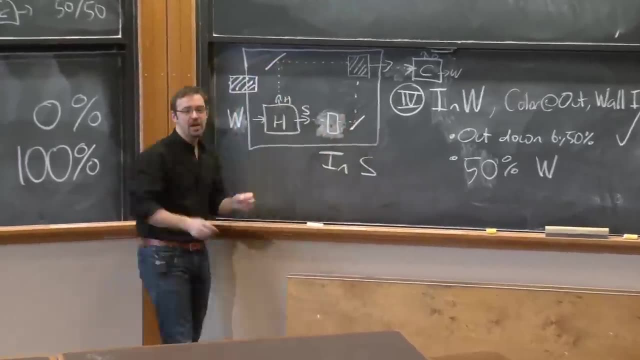 Yeah, so that's a totally reasonable question. So the question is basically: let's take this experiment and let's make it even more intricate by, for example, replacing these mirrors by color boxes. OK, so here's the thing I want to emphasize. 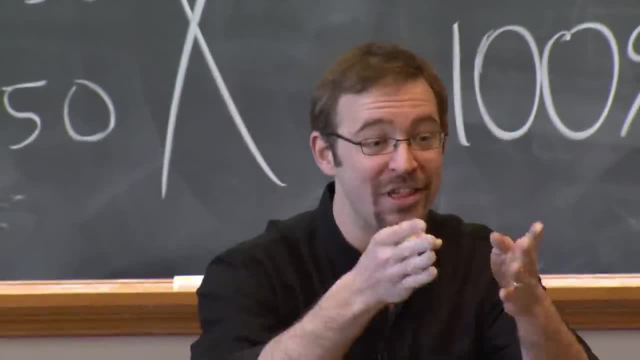 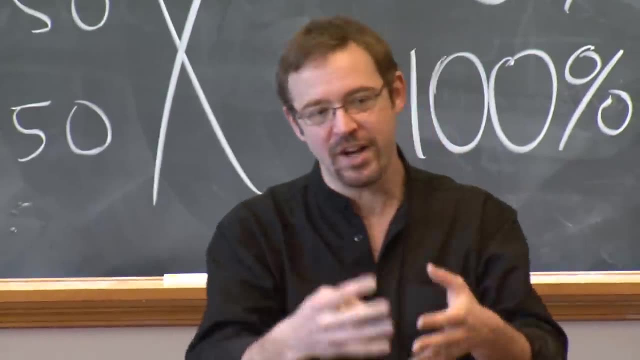 Something that- well, how do I say it? I strongly encourage you to think through that example And, in particular, think through that example. Come to my office hours and ask me about it. So that's going to be studying a different experiment. 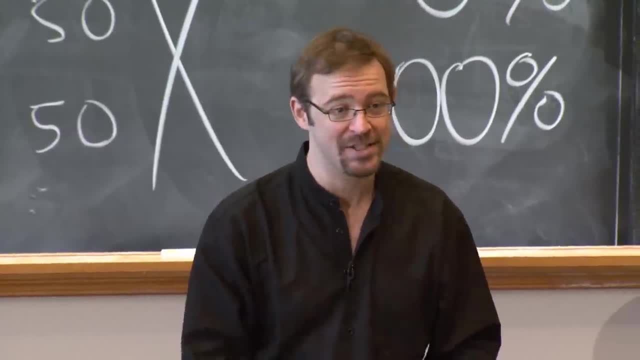 And different experiments are going to have different results, So we're going to have to deal with that on a case-by-case basis. It's an interesting example, but it's going to take us a bit afar from where we are right now. But after we get to the punchline from this, 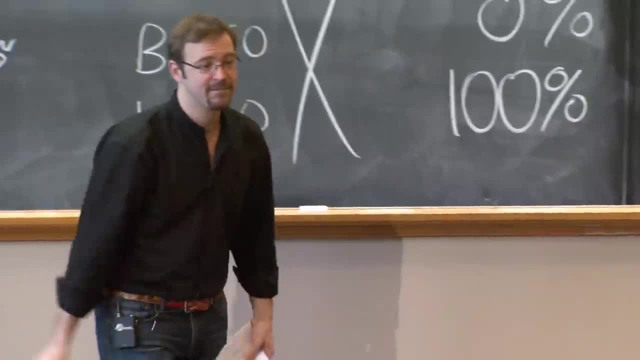 come to my office hours and ask me exactly that question. OK, Yeah, So we have a color box to put it in white. There's like electrons And we've got this and this and like brown and stuff. Yeah, 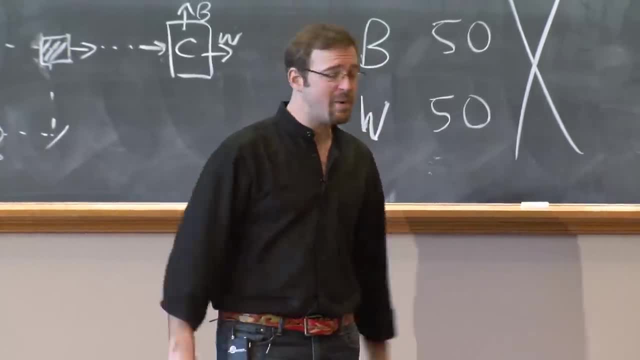 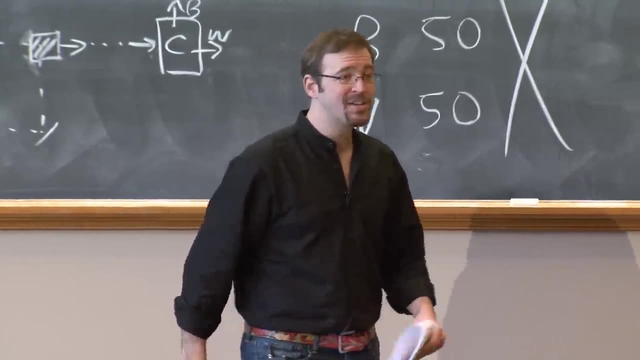 How do you know the boxes work? How do I know the boxes work? These are the same boxes we used from the binning. We tested them over and over. How did you first check it if it worked, Because it's always kind of maybe different, you know. 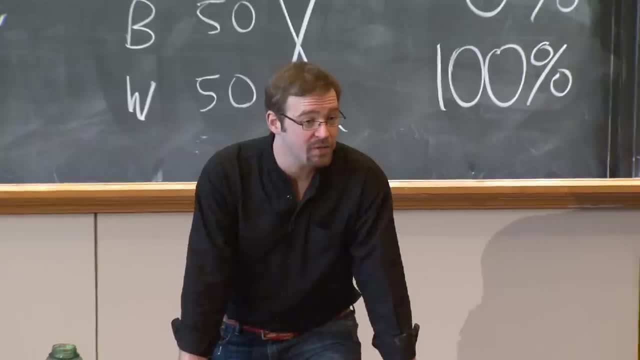 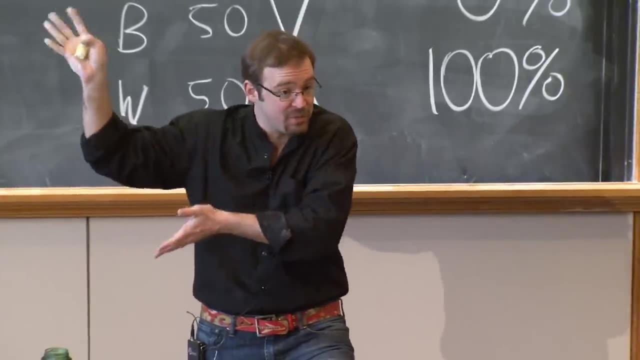 How to say There's no other way to build a box that does the properties that we want, which is that you send in color and it comes out color again and the mirrors behave this way. There's any box that does those first set of things, which. 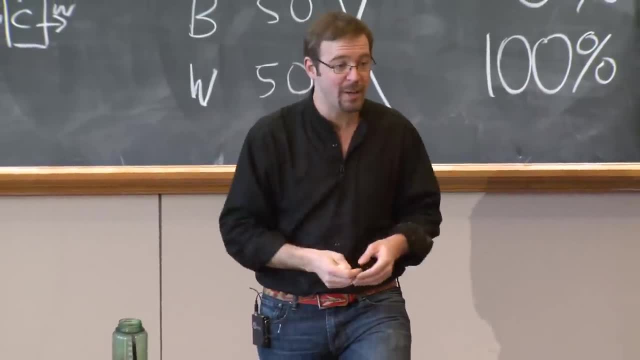 is what I will call a color box, does this too. There's no other way to do it. I mean, I don't mean this, because like no one's you know testing, Because you can't actually check it. 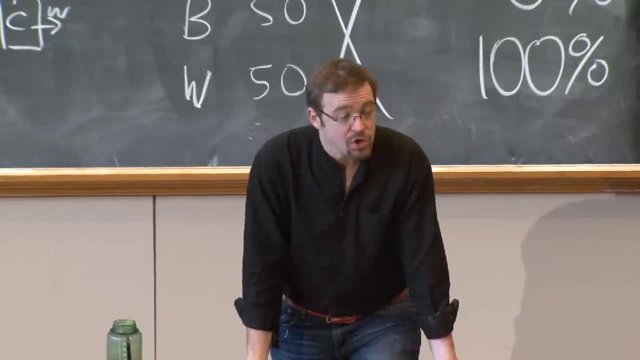 You can't actually send an electron you know is white. Oh sure you can. You take the electron that came out of the color box. That's what we mean by saying it's white, Yeah, but it's a box, yeah. 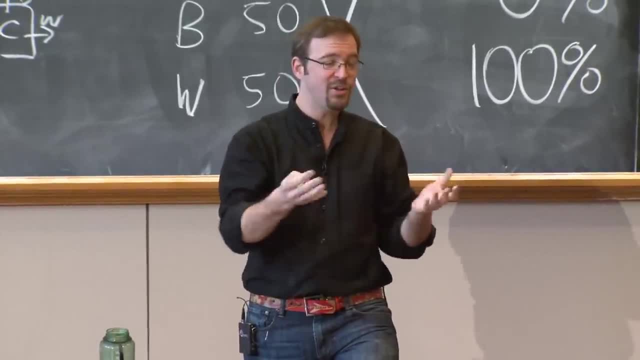 Well, but that's what it means to say: the electron is white, Right? It's like how do you know that my name is Alan? You say Alan and I go, what Right? But you might feel like, look, that's not. 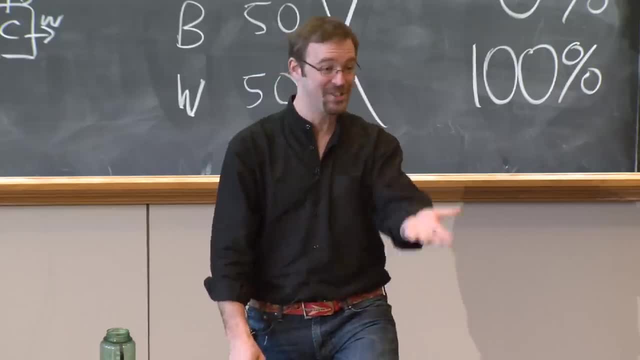 a test of whether I'm Alan. It's like, well, what is a test of what you? That's how you test What's your name. I'm Alan, Oh great, That's your name. So that's what I mean by white. 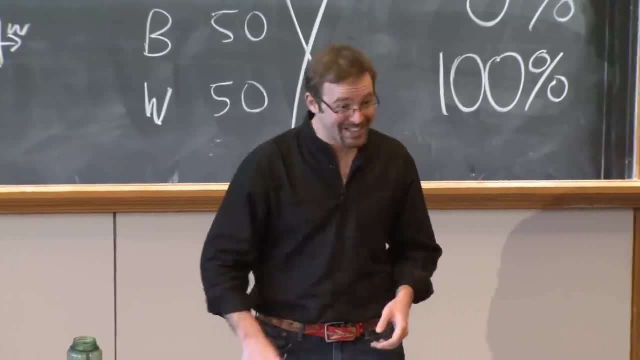 Now you might quibble that that's a stupid thing to call an electron, and I grant you that, But it is nonetheless a property that I can empirically engage. OK, I've been told that I never ask questions from the people on the right. 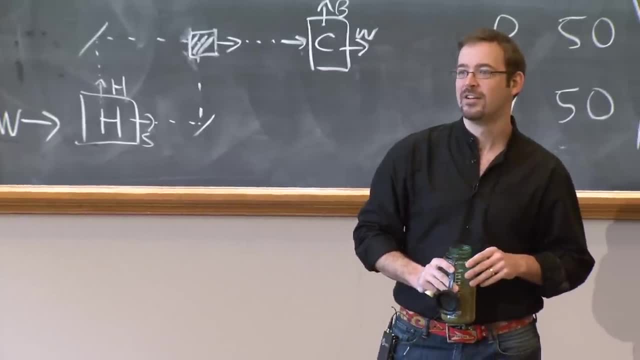 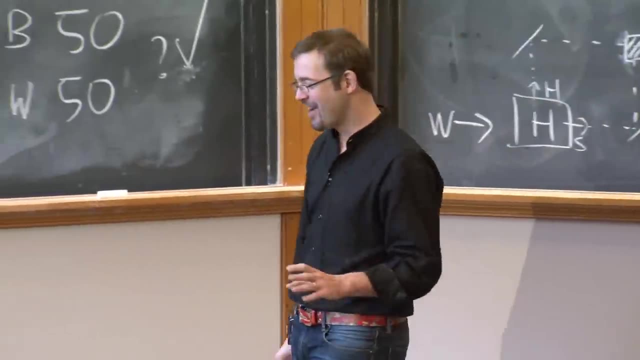 Yeah, Is it important whether the experimenter knows what all is there? No, This experiment has been done again by some French guys. There's this, The French Look dude. So there's this guy, Alain Aspey. 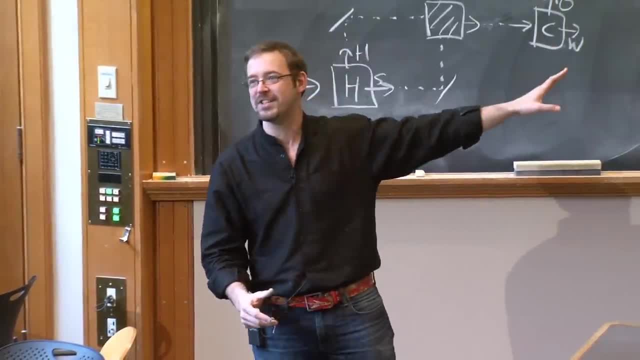 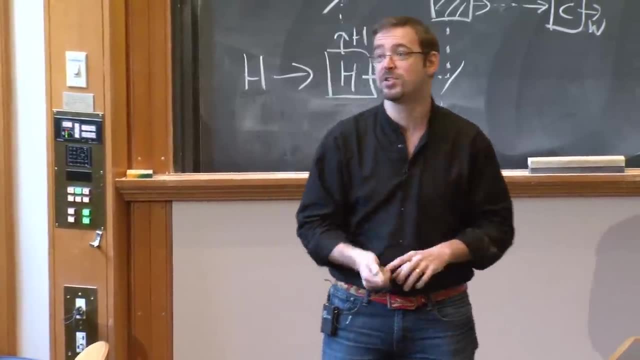 Great experimentalist, great physicist, And he's done lots of beautiful experiments on exactly this topic. And send me an email and I'll post some example papers and reviews by him. And he's a great writer on the web page. So just send me an email to remind me of that. 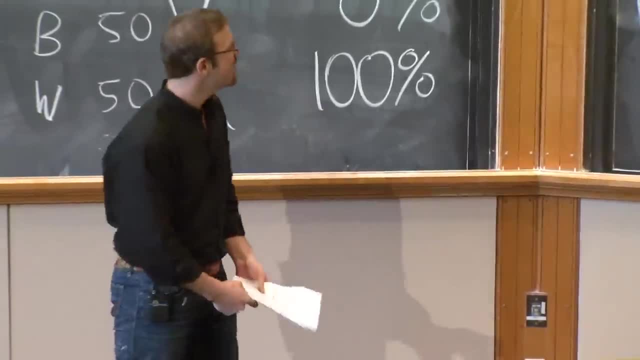 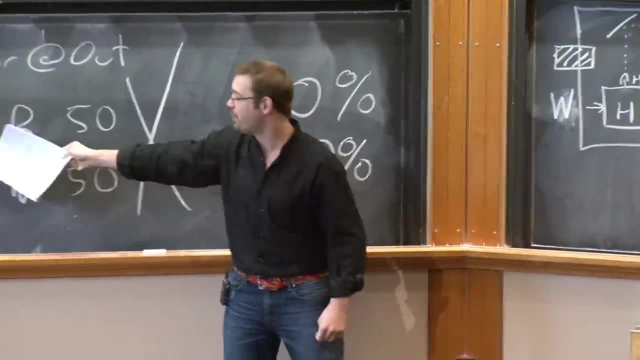 OK, so we're lowish on time, so let me move on. So what I want to do now is I want to take the lesson of this experiment and the observation that was made a minute ago that in fact, the same problem was present when we ran. 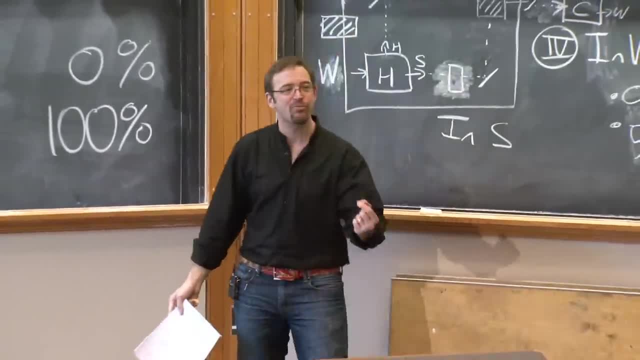 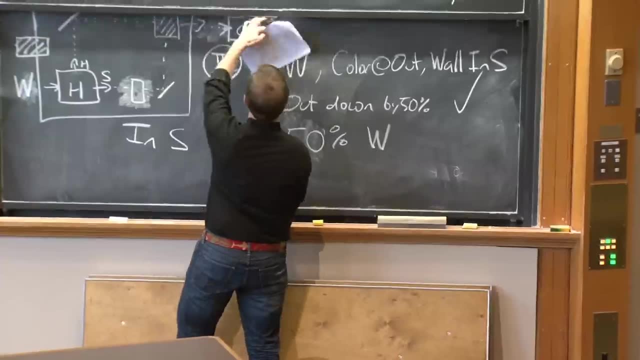 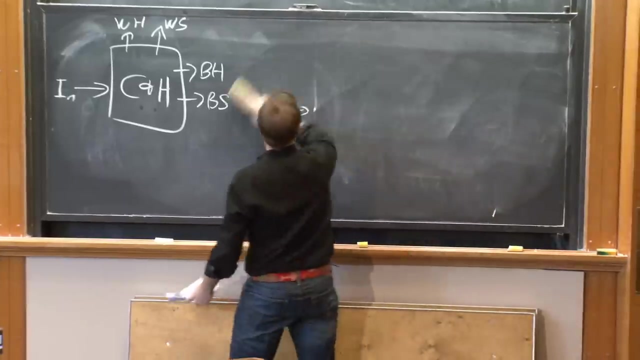 this experiment and got 100%. We should have been freaked out already And I want to think through what that's telling us about the electron, the single electron, as it transits the apparatus. The thing is, at this point we're in real trouble. 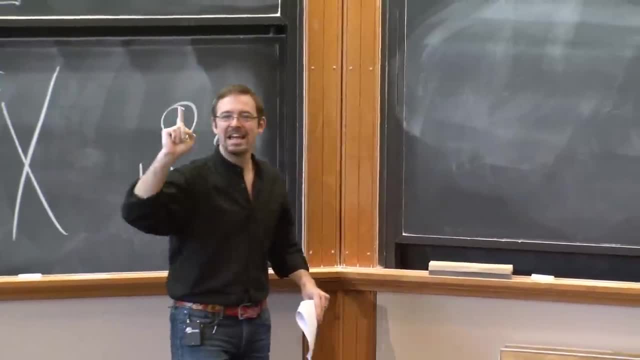 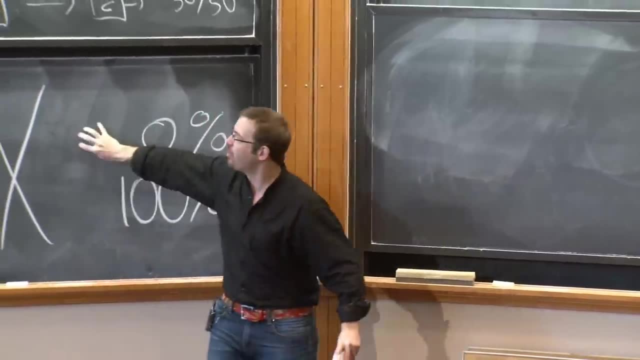 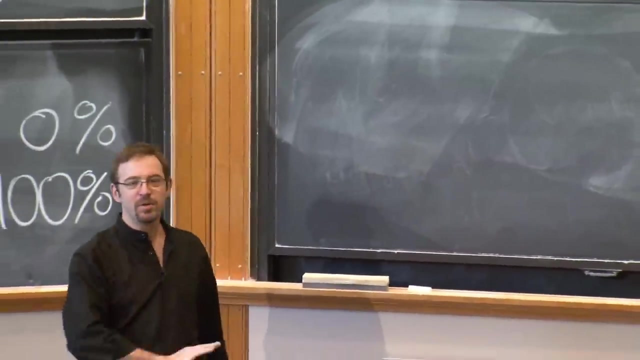 And here's the reason: Consider a single electron inside the apparatus. And I want to think about the electron inside the apparatus while all walls are out. So it's this experiment: Consider the single electron. We know, with total confidence, with complete reliability. 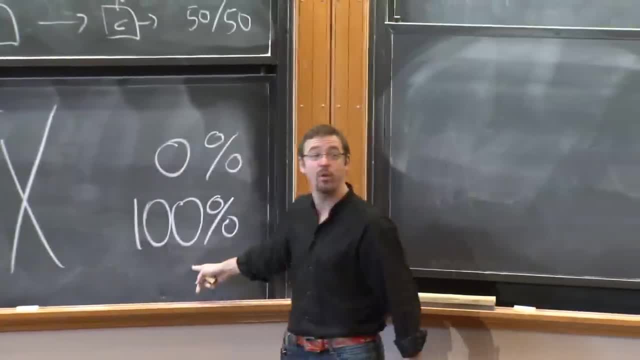 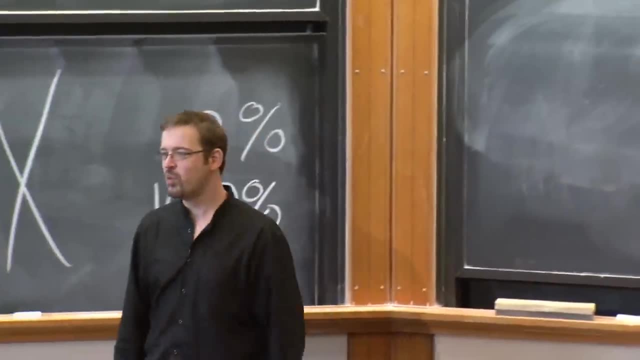 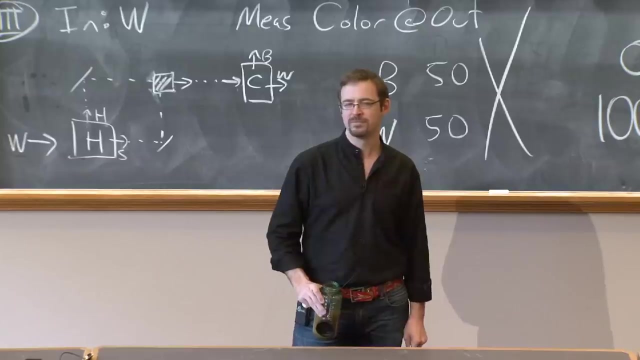 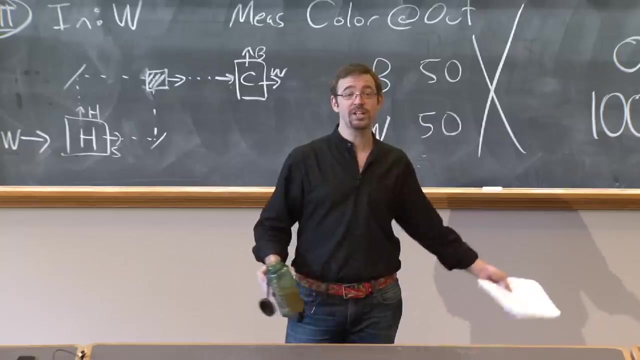 that every electron will exit this color box, out the white aperture. We've done this experiment. We know it will come out white. Yes, Here's my question. Which route did it take? Spoiler, Not a spoiler. Which route did it take? 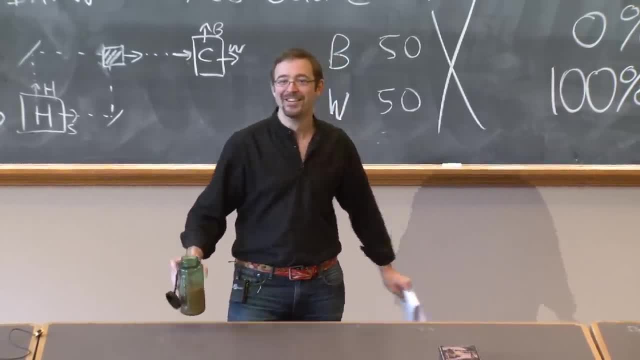 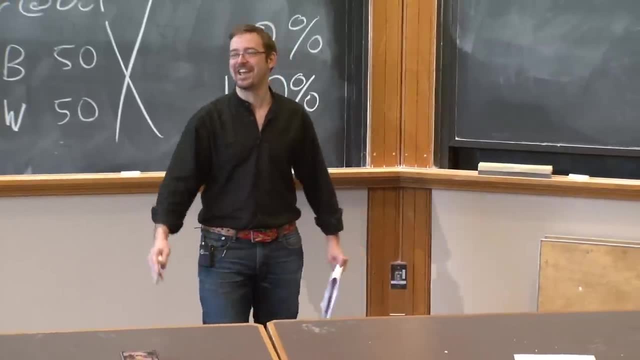 Why do you care what route it took? I'm asking you the question. That's why you care. I'm the professor here. What is this? Come on? Which route did it take? We don't know, We don't measure it. 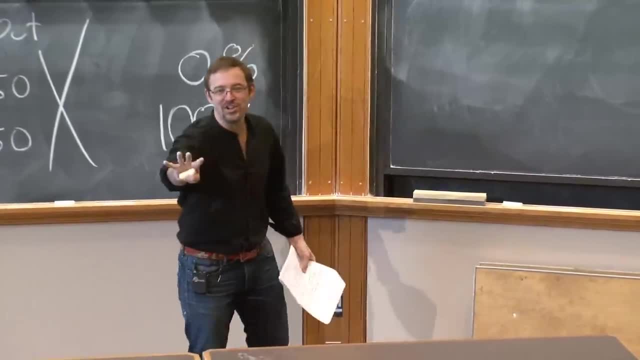 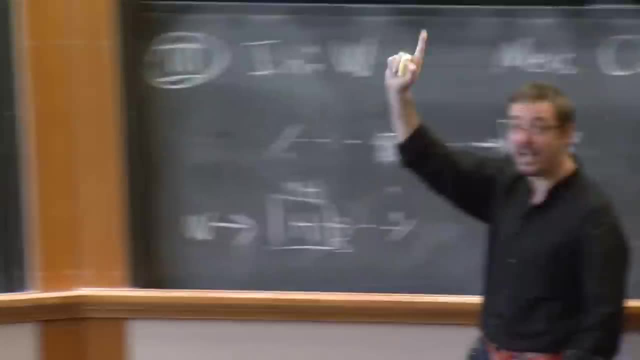 OK, let's think through the possibilities. Grapple with this question in your belly. Let's think through the possibilities. First off, did it take the hardness path? So, as it transits through, It's a single electron transiting through this apparatus. 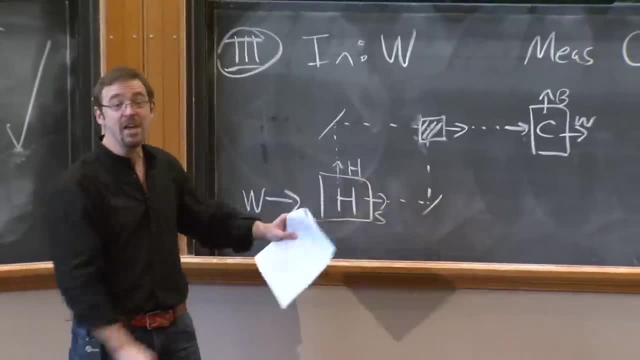 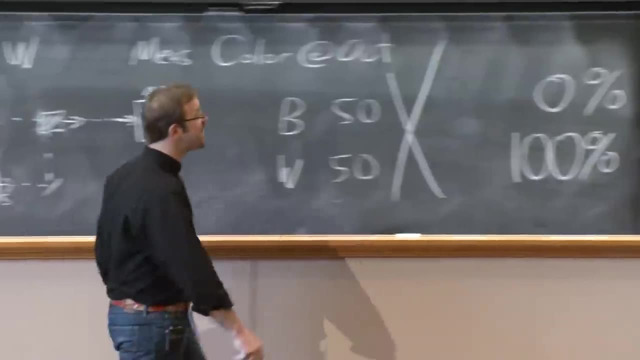 Did it take the hard path or did it take the soft path? These are millions of miles long, millions of miles apart. This is not a ridiculous question. Did it go millions of miles that direction, millions of miles that direction? Did it take the hardness path? 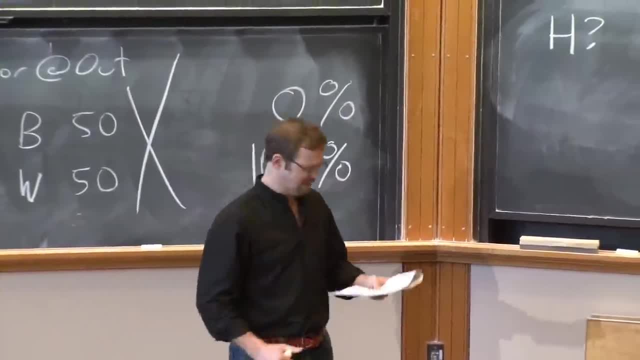 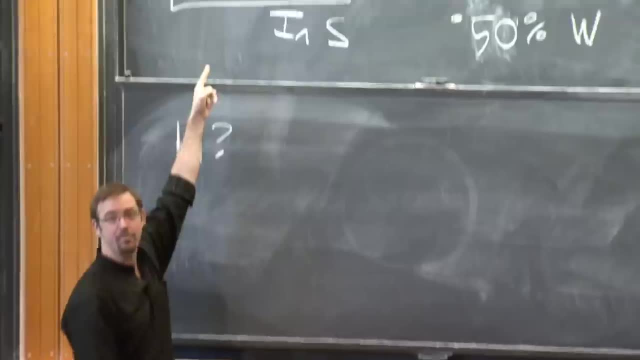 Ladies and gentlemen, did it take the hardness path? the hard path? Well, we ran this experiment by putting a wall in the soft path, And if we put a wall in the soft path, then we know it took the hard path, because no other electrons 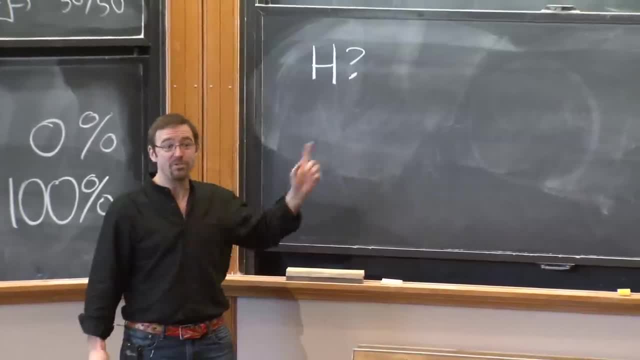 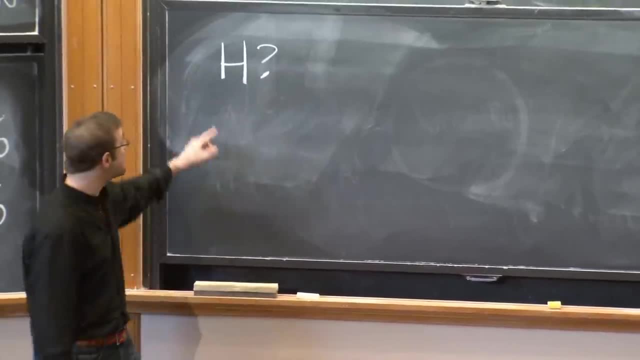 come out except those that went through the hard path, correct? On the other hand, if it went through the hard path, it would come out 50% of the time white, 50% of the time black, But in fact, in this apparatus it comes out always 100% white. 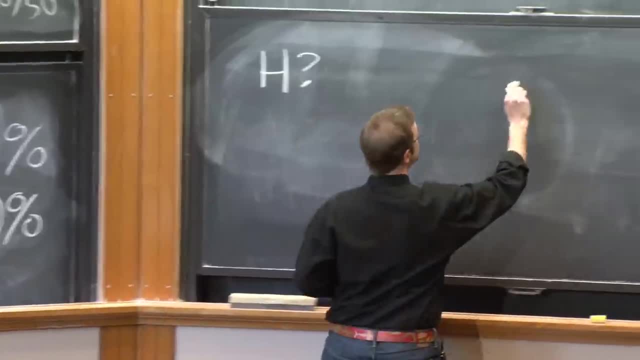 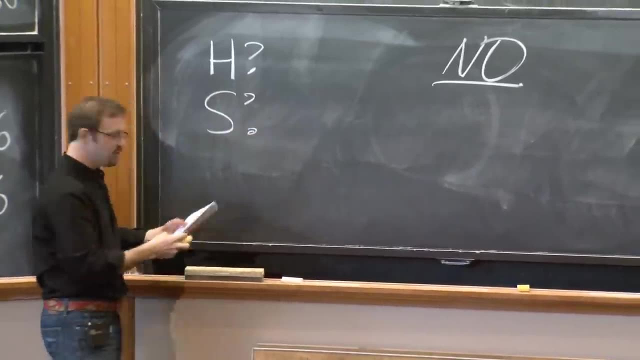 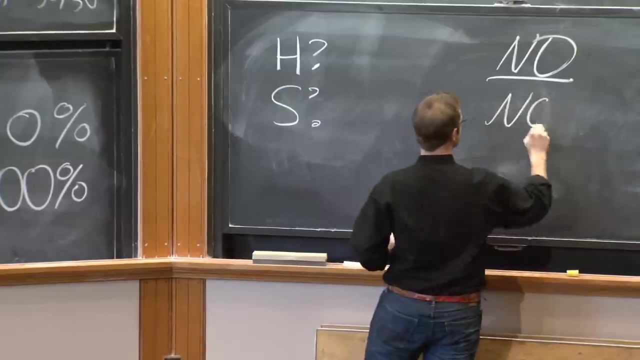 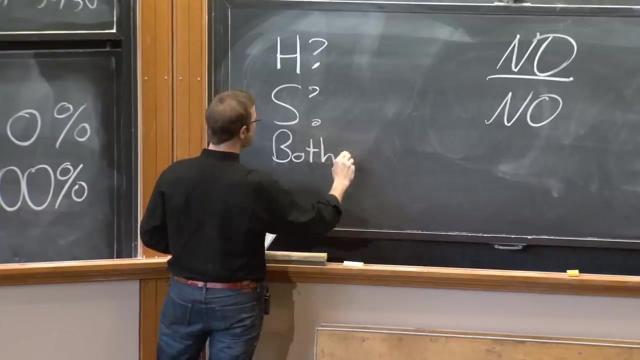 It cannot have taken the hard path? No, Did it take the soft path? Same argument, Different side, right? No, Well, this is not looking good. Well, look, maybe this was suggested. Maybe it took both. Maybe electrons are sneaky little devils that split and do. 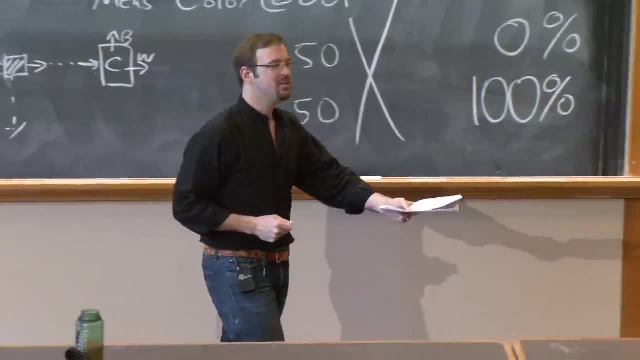 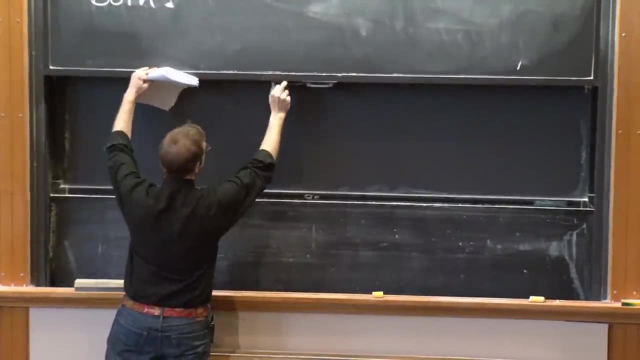 and part of it goes one way and part of it goes the other. Maybe it took both paths. So this is easy, We can test this one. And here's I'm going to test this one. Oh sorry, Actually I'm not going to do that yet. 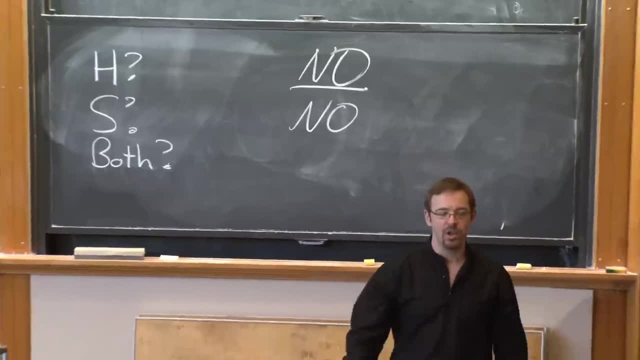 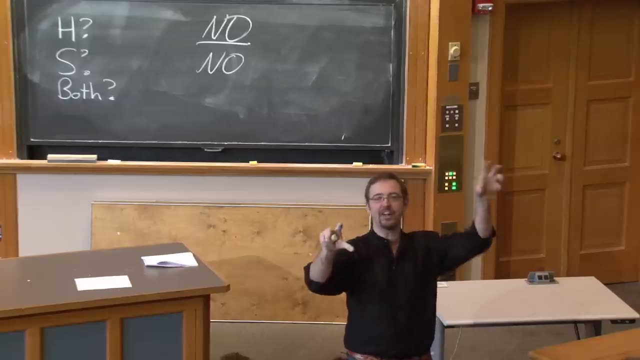 So we can test this one. So if it took both paths, here's what you should be able to do. You should be able to put a detector along each path and you'd be able to get half an electron on one side and half an electron on the other. 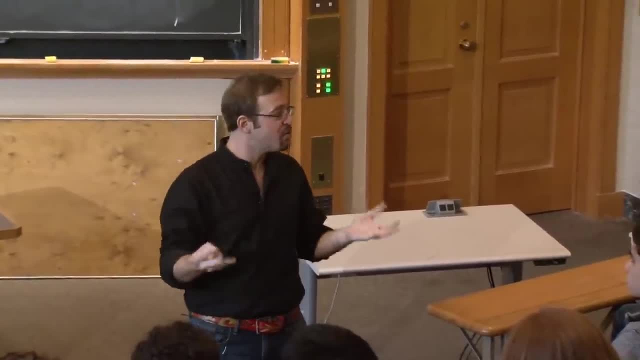 Or maybe two electrons, one on each side and one on the other right. So this is the thing that you'd predict if you said it went both. So here's what we'll do: We will take detectors, We will put one along the hard path. 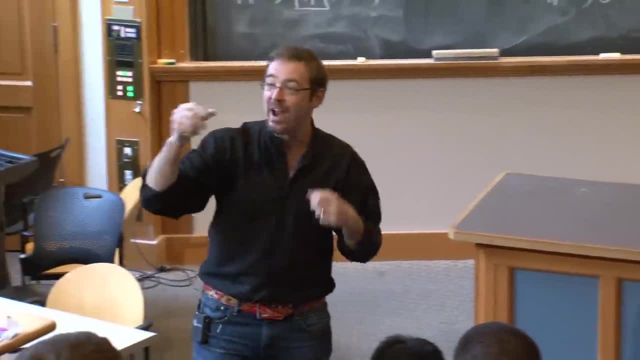 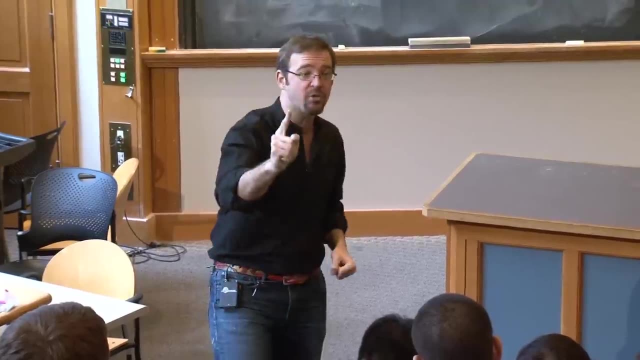 and one along the soft path. We will run the experiment and then observe whether and ask whether we see two electrons. we see half and half. What do we see? And the answer is: you always, always- see one electron on one of the paths. 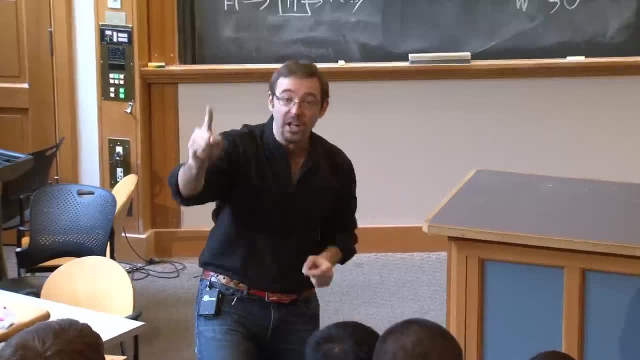 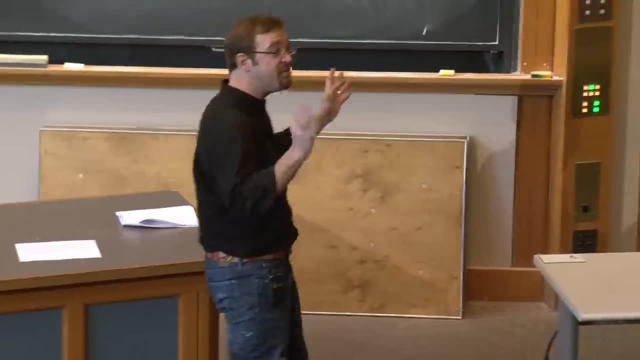 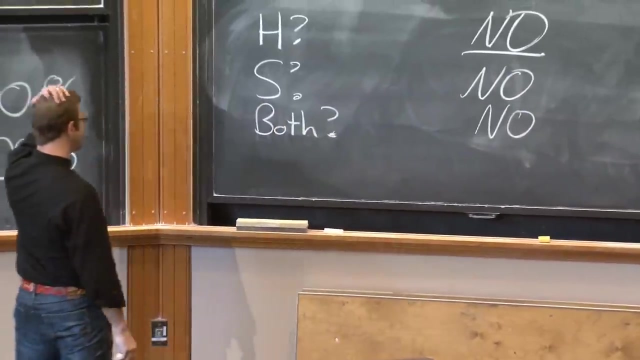 You never see half an electron, You never see a squishy electron. You see one electron on one path period. It did not take both. You never see an electron split in two, divided, confused. No Well, it didn't take the hard path. 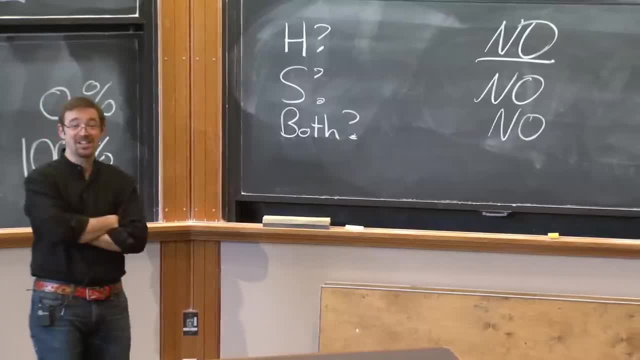 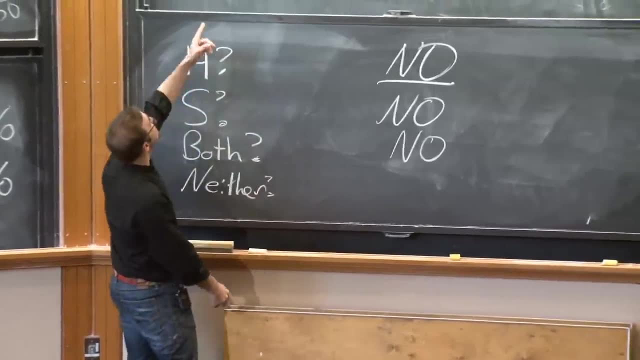 It didn't take the soft path, It didn't take both. There's one option left: Neither. Well, I say neither, but So what about neither? And that's easy. Let's put a barrier in both paths. And then what happens? 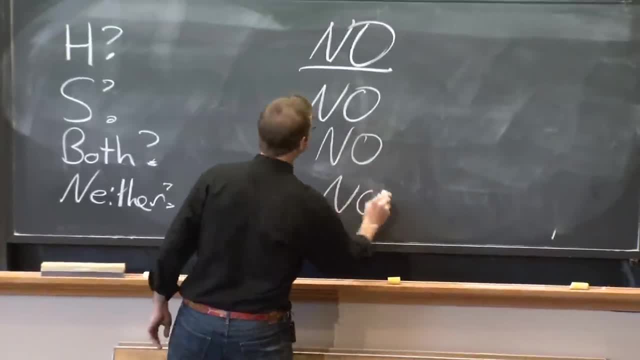 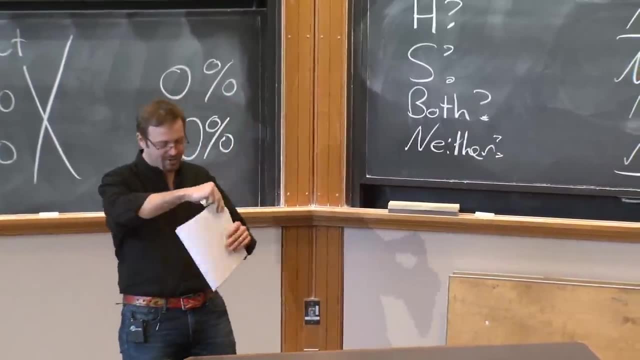 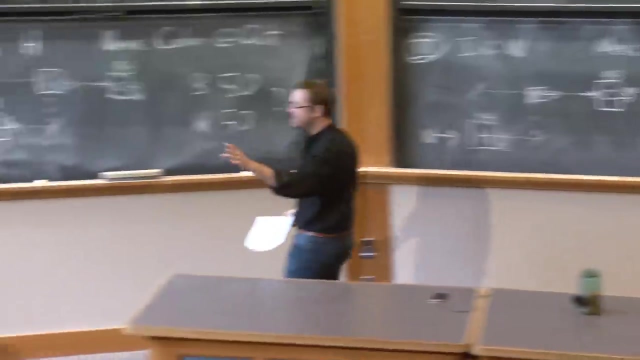 Nothing comes out right, So no, OK. So now to repeat an earlier prescient remark from one of the students: what the hell? So here's the world we're facing. I want you to think about this. Take this seriously. 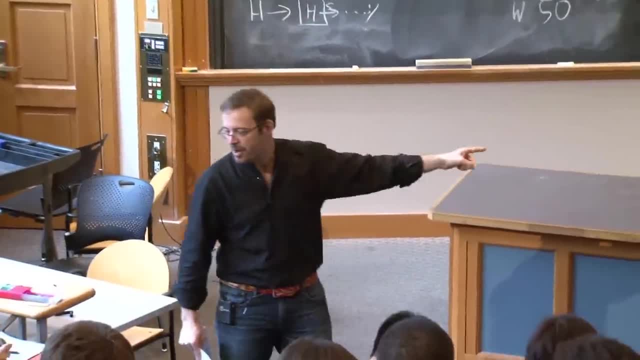 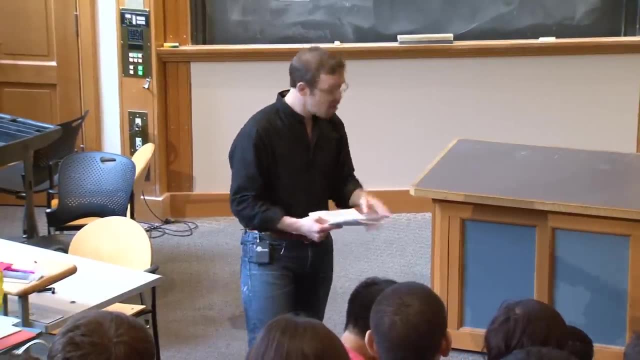 Here's the world we're facing. And when I say here's the world we're facing, I don't mean just these experiments, I mean the world around you. 20 kilo mirrors, buckyballs- Here is what they do. 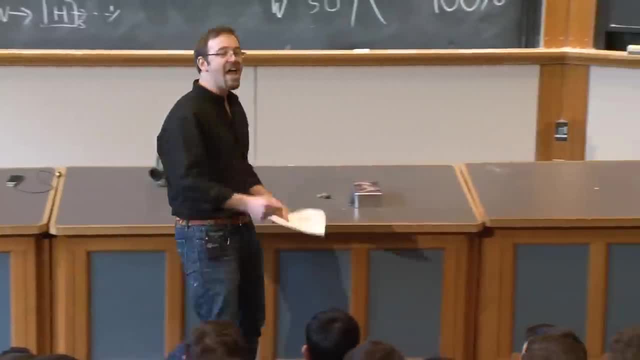 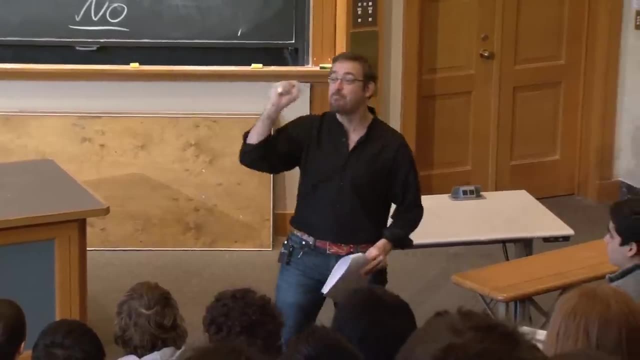 When you send them through an apparatus like this. every single object that goes through this apparatus does not take the hard path, It does not take the soft path, It doesn't take both And it does not take neither. And that pretty much exhausts the set. 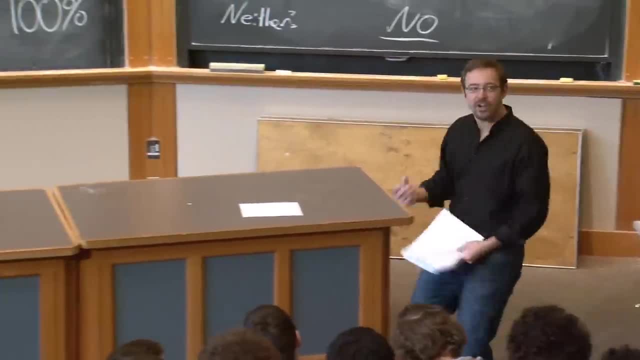 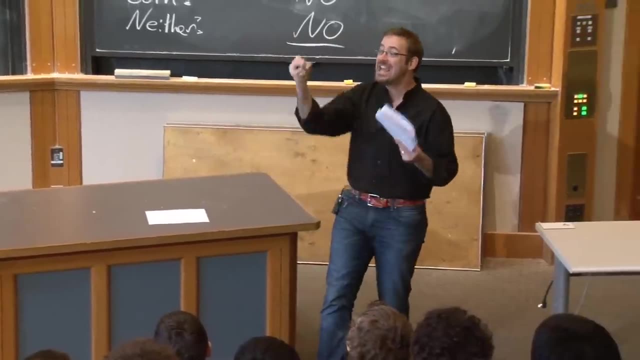 of logical possibilities. So what are our electrosystems? So what are our electrosystems? What are the electrons doing when they're inside the apparatus? How do you describe an electron inside the apparatus? You can't say it's on one path. 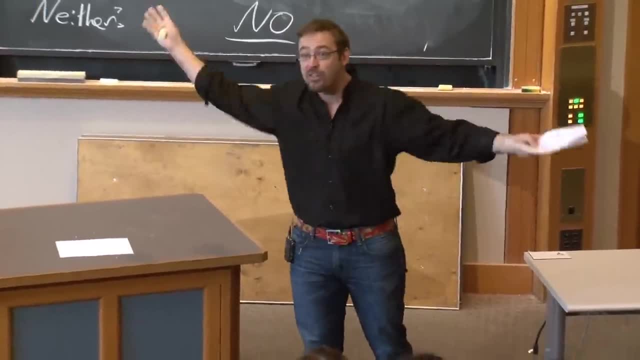 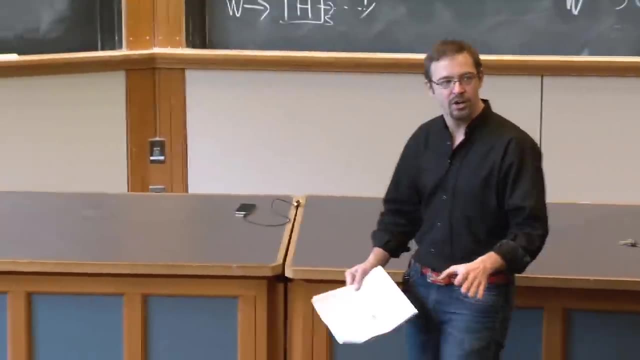 You can't say it's on the other, It's not on both and it's not on either. What is it doing halfway through this experiment? So, if our experiments are accurate, to the best of our ability to determine they are, and if our arguments are correct- and that's on me- 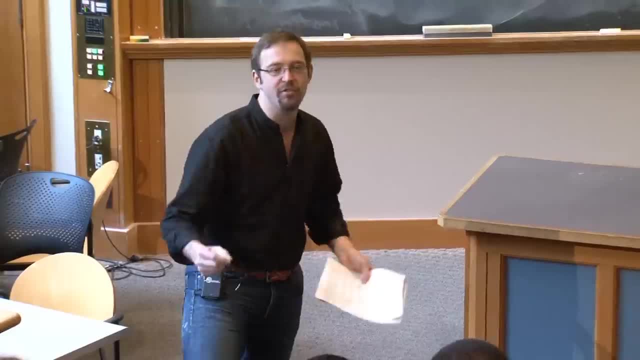 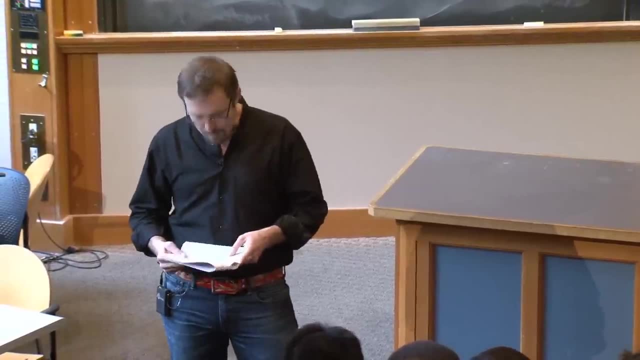 then they're doing something. These electrons are doing something we've just never thought of before, something we've never dreamt of before, something for which we don't really have good words in the English language. Apparently, empirically, electrons have a way of moving. 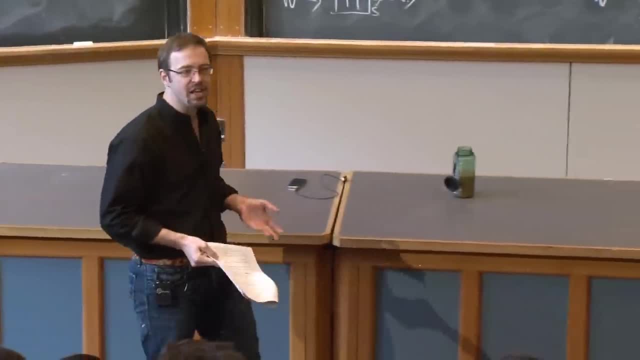 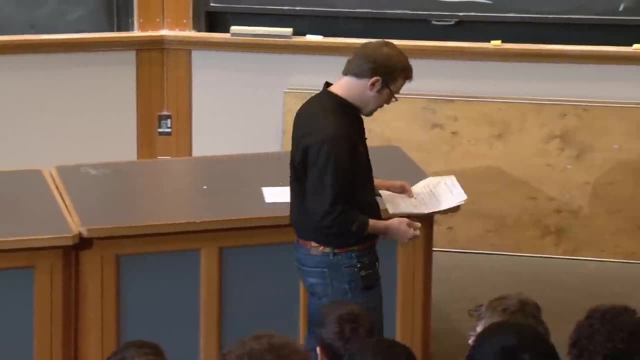 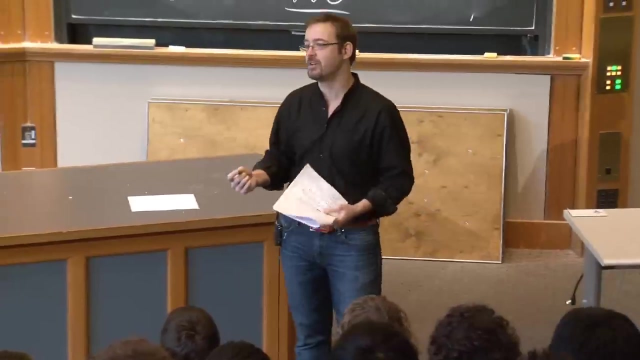 Electrons have a way of being which is unlike anything that we're used to thinking about, And so do molecules, And so do bacteria. So does chalk. It's just harder to detect in those objects. So physicists have a name for this new mode of being. 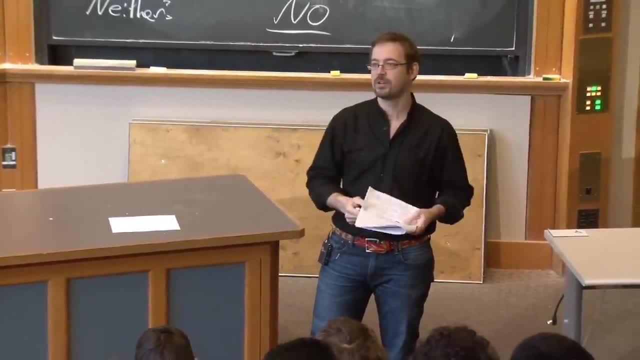 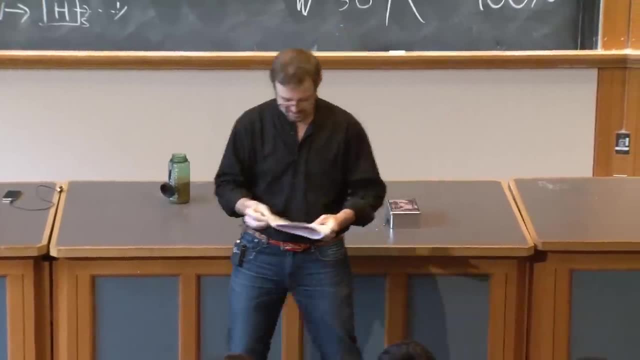 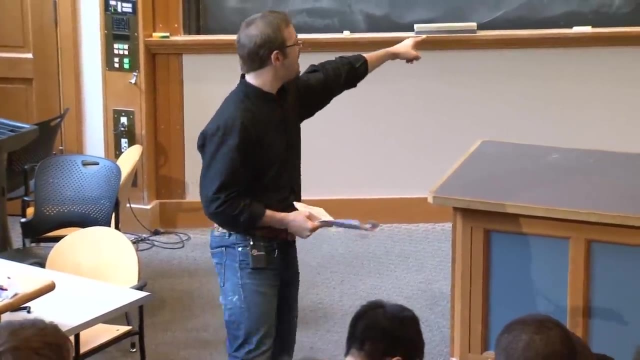 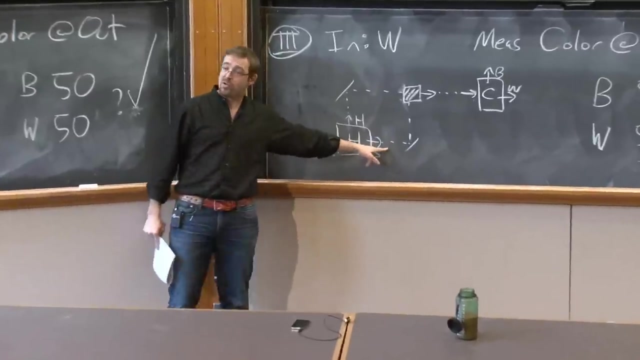 And we call it superposition. Now, at the moment, superposition is code, for I have no idea what's going on. The usage of the word superposition would go something like this: An initially white electron inside this apparatus, with the walls out, is neither hard nor soft, nor both. 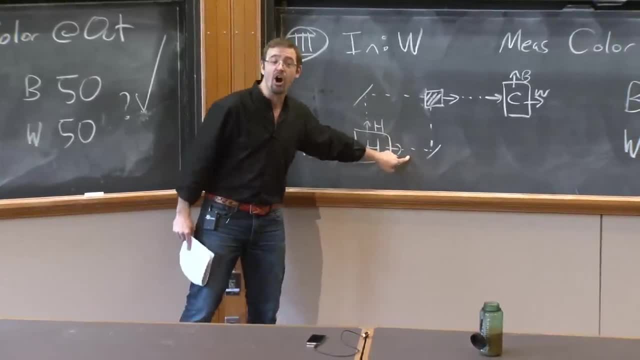 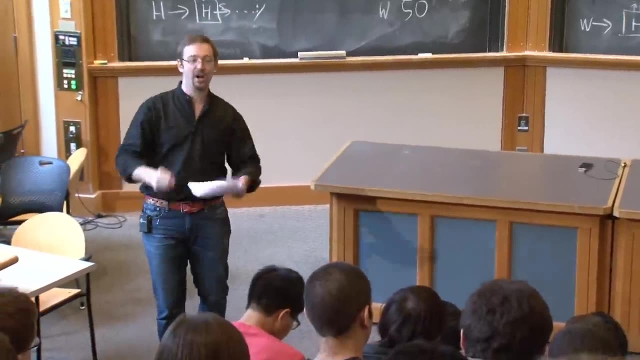 nor neither. It is, in fact, in a superposition of being hard and of being soft. This is why we can't meaningfully say this electron is some color and some hardness, not because our boxes are crude and not because we're ignorant. 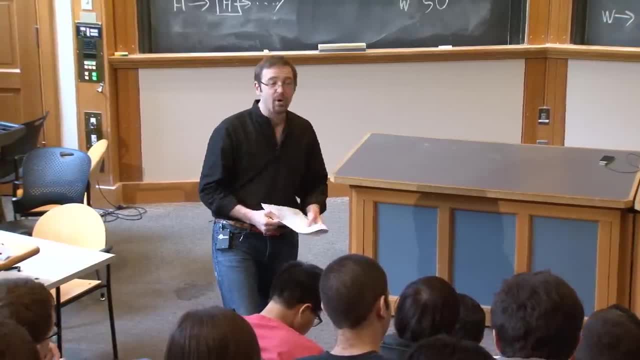 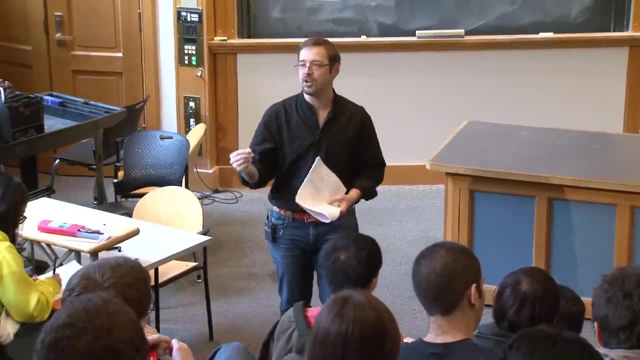 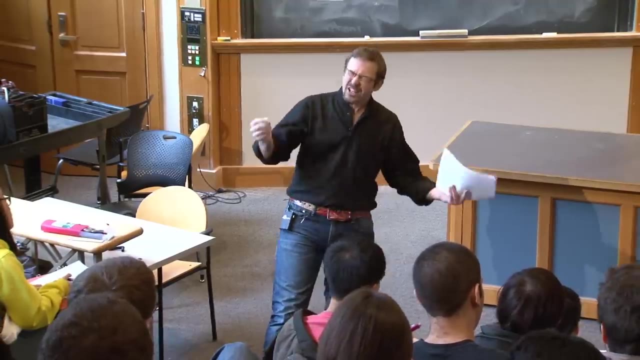 Though our boxes are crude and we are ignorant, it's deeper. Having a definite color means not having a definite hardness, but rather being in a superposition of being hard and being soft. Sorry, Every electron exists, Every electron exits a hardness box, either hard or soft. 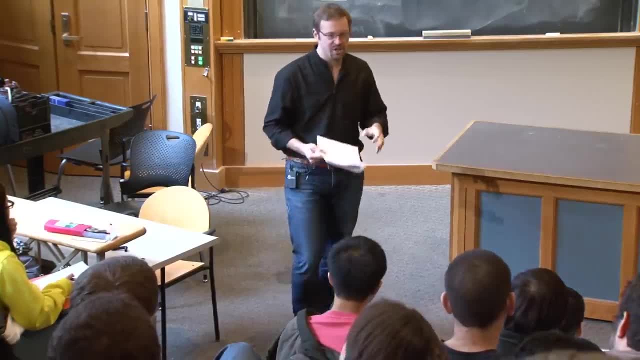 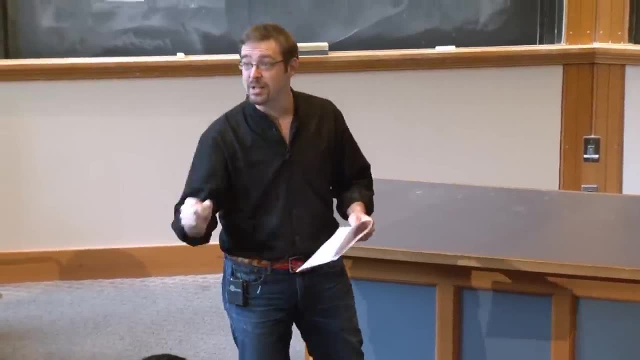 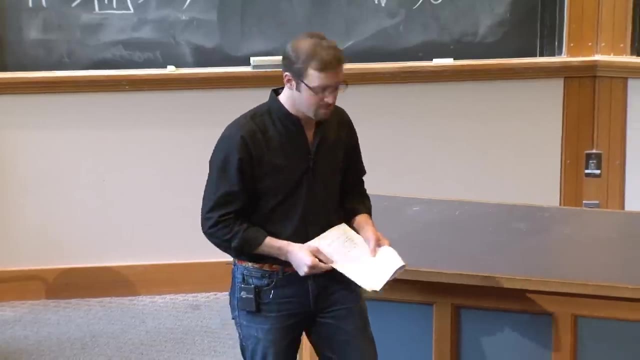 But not every electron is hard or soft. It can also be a superposition of being hard or being soft. The probability that we subsequently measure it to be hard or soft depends on precisely what superposition it is. For example, we know that if an electron 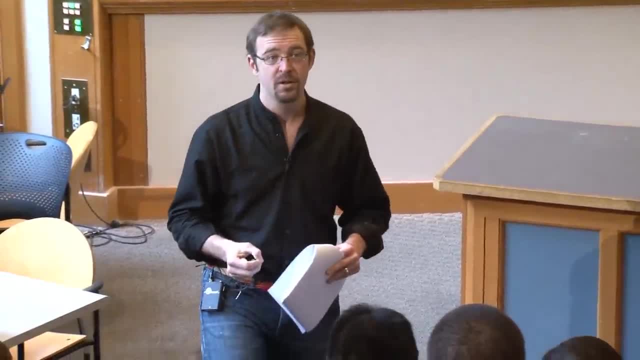 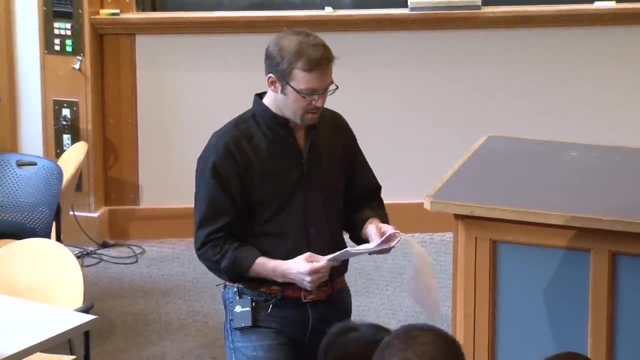 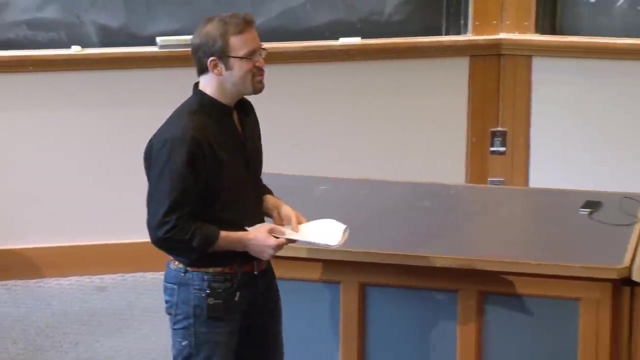 is in the superposition corresponding to being white, then there are even odds of it being subsequently measured to be hard or to be soft. So to build a better definition of superposition than I have no idea what's going on is going to require a new language. 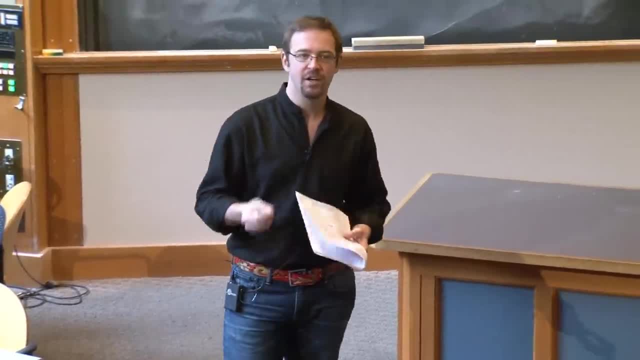 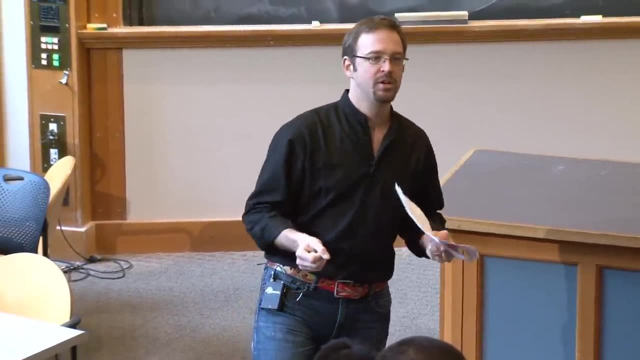 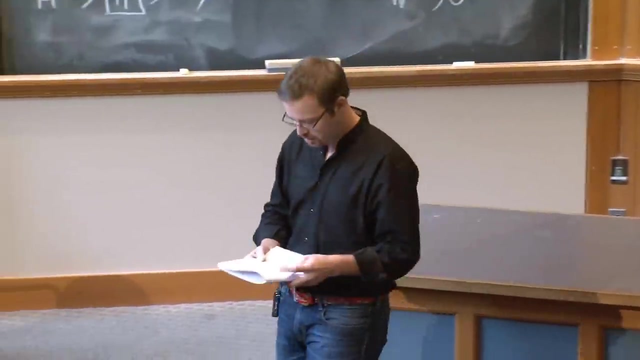 And that language is quantum mechanics And the underpinnings of this language are the topic of the course, And developing a better understanding of this idea of superposition is what you have to do over the next three months. Now, if all this troubles your intuition,